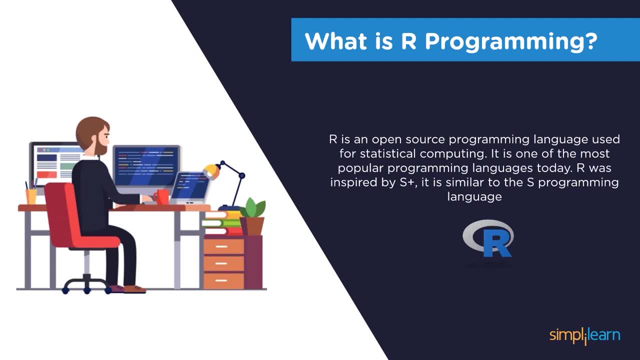 It was inspired by S plus and it is similar to S programming language. So, when it comes to data science, what we can say is: R is a popularly used programming language across the globe. It is free and open source. as I mentioned, It is optimized for vector operations, which we will 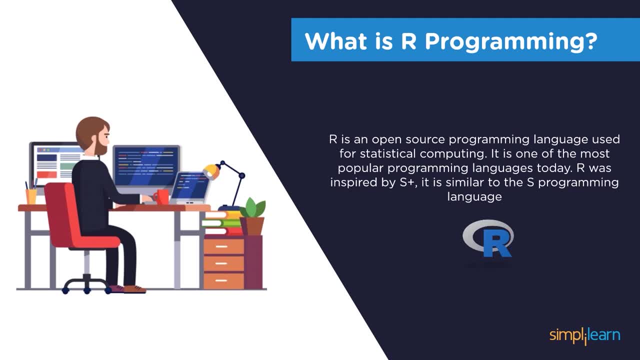 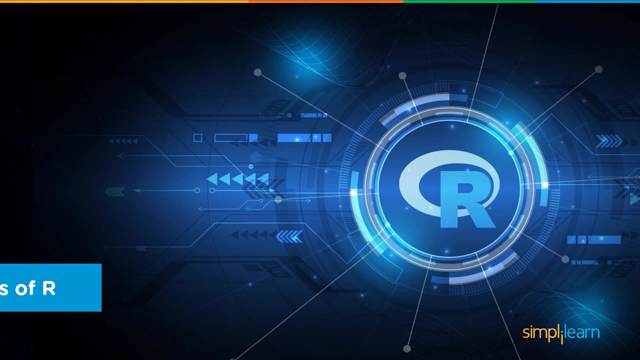 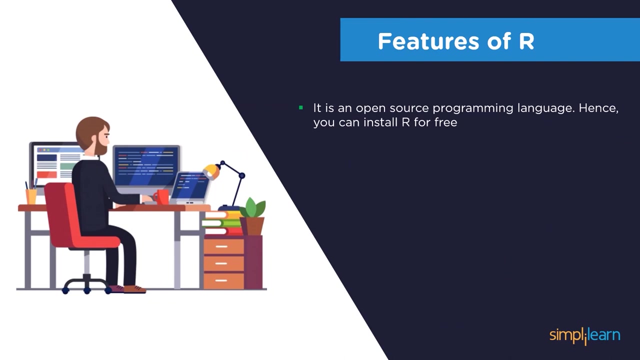 learn about later. It has an amazing community, has, in fact, 9000 plus encoded or community packages allowing us to do almost anything or everything using R. Now, when we talk about features of R, as I said, it's open source programming language, so you can. 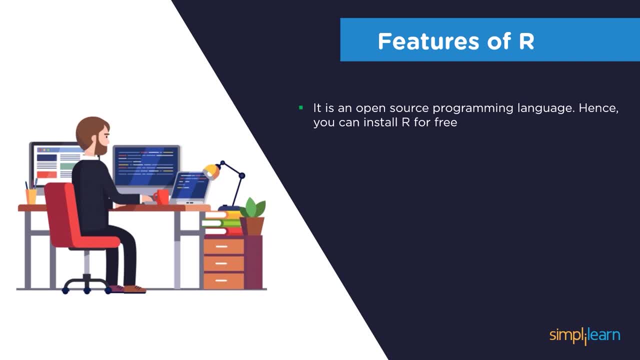 install R for free and you can straight away start working. You wouldn't have to really go for a licensed version or pay for the software. Non-coders can also understand and perform programming in R and it has various data structures and operators. It can be integrated with other programming. 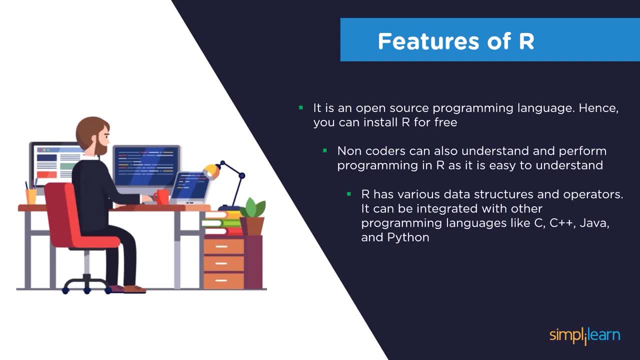 languages like C, C++, Java and Python. It consists of various inbuilt packages, a lot of sample data sets which can be used, and that makes reporting the results of an analysis easier by using R. Now, before we start learning about variables, loops, how you work with R and 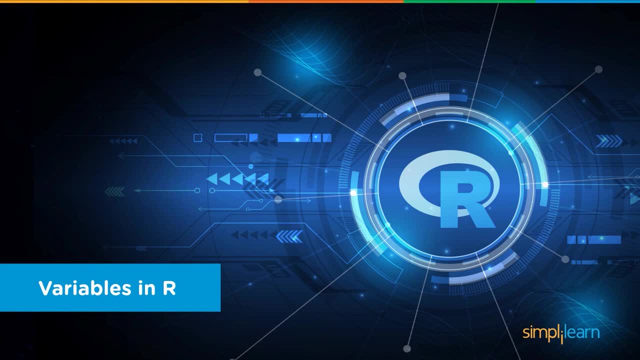 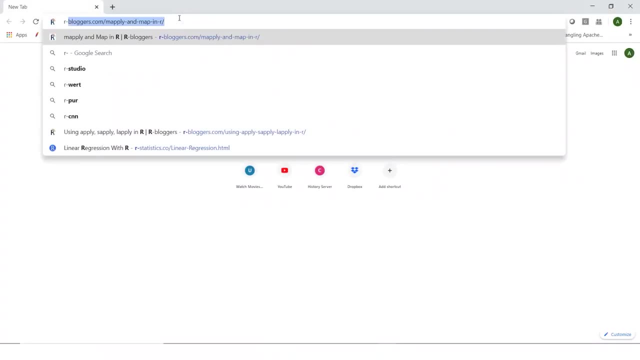 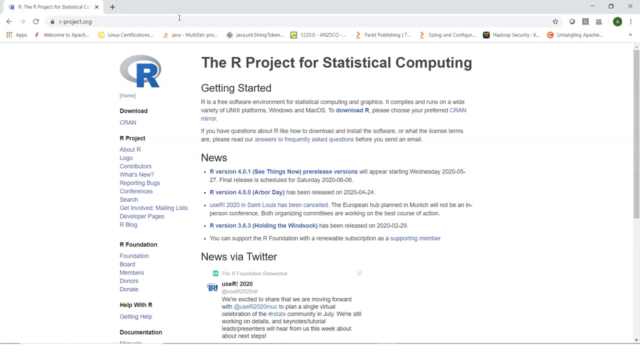 so on. it would be good to know how you can set up R and work on R. So for that, what you can do is you can just go to r-projectorg, and once we get to the home page of R project for statistical computing using this link, we can click on download R here. Now, that brings you to a. 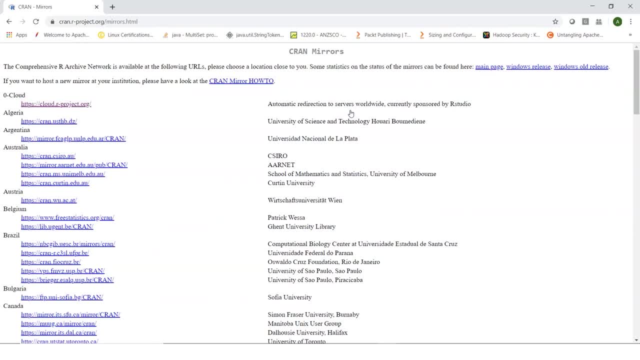 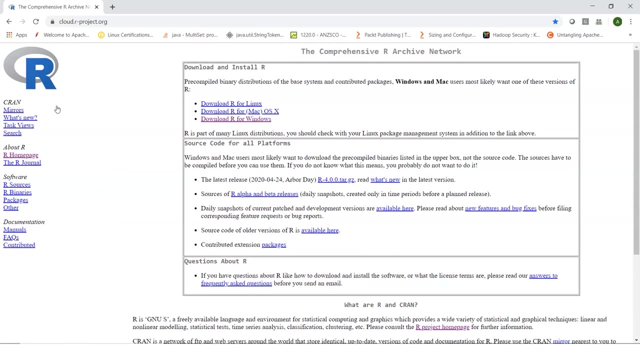 page to download it Now. there are various links here, So it shows you the comprehensive R archive network that is, CRAN mirrors, and it is available at different URLs. However, I would choose the first one, which is zero cloud. You can just click on this one and then, based on your operating. 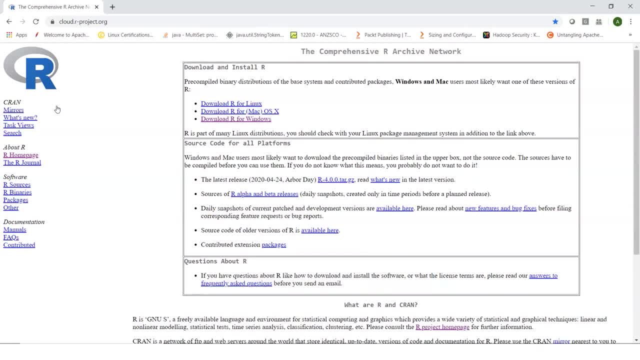 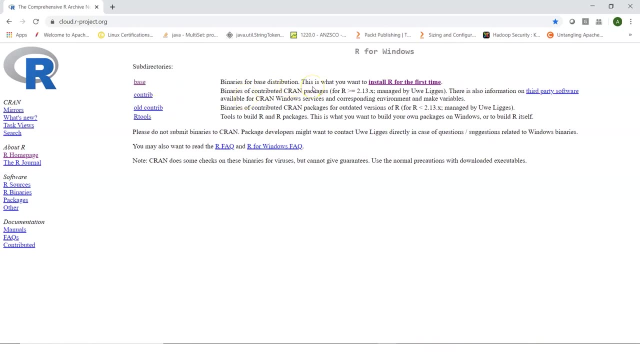 system. whether you are working on a Linux machine, on a MacBook or Windows, you can install it, So you can just click on this one. As of now, I'm using a Windows machine, so I can click on download R for Windows, and that takes me to this link, which says binaries for base distribution. Now, this is 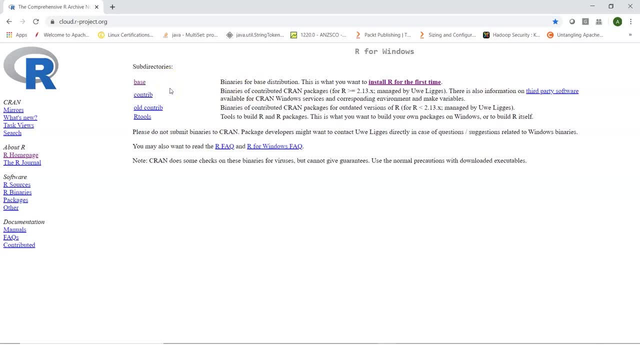 what we can use to work with R straight away. However, there is one more package, that is R studio. We will see how we can set up that Now. this one takes us to the best mirror possible for our location, from where we can download R, So you can click on this base and then you can. 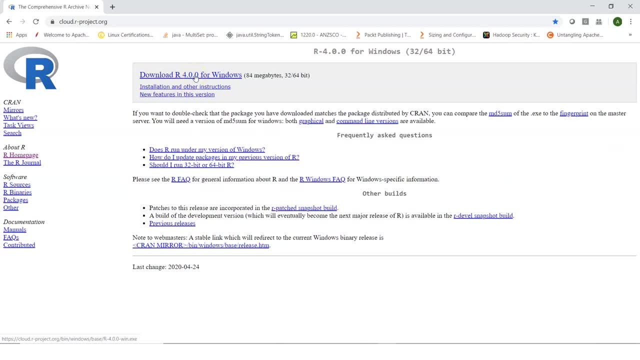 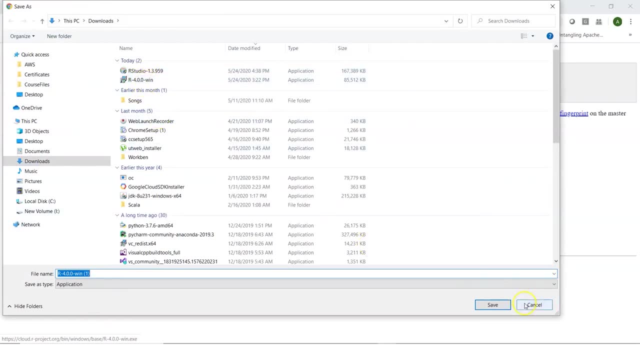 download by clicking on this link. I have already downloaded R for Windows and I have already downloaded this. So once you click on this one, you can just save it. So I have it here already in my downloads and that's more than enough. Then you can just double-click on it and you can go through. 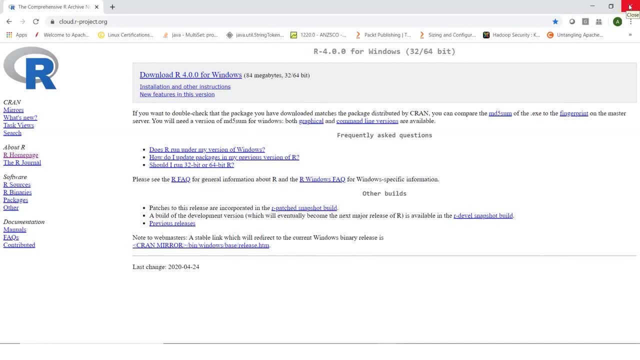 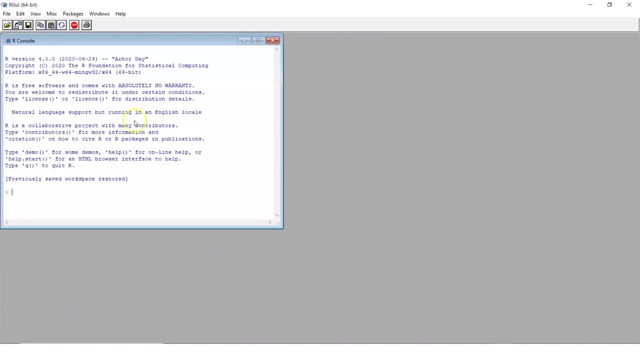 the instructions to set up R. That would also allow you to basically set up a desktop shortcut, which I have already done here on my machine, and if I go in here I see our base. You can click on this one and that will take you to the best mirror possible. So I have already downloaded this. so 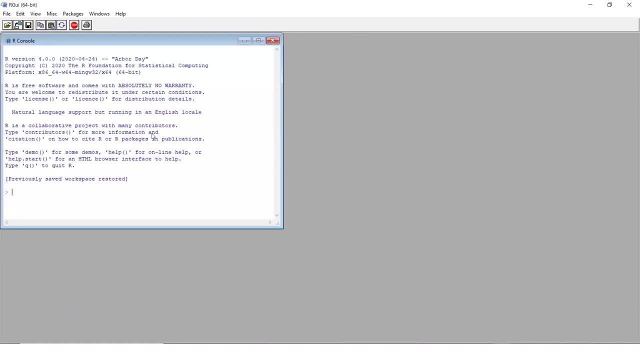 brings you to the page which you can use to straight away start working with R. now, yes, there is one more package called R studio, which is set up on top of base R, which makes working with R easier. now, here also, you can start working. so it shows you R console and you can click on file. 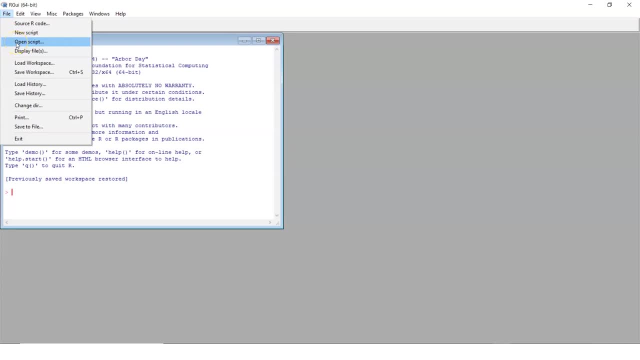 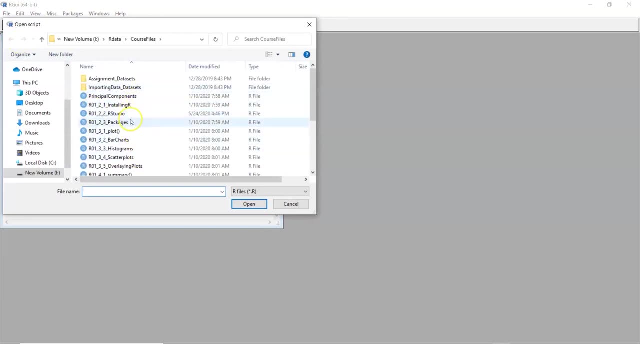 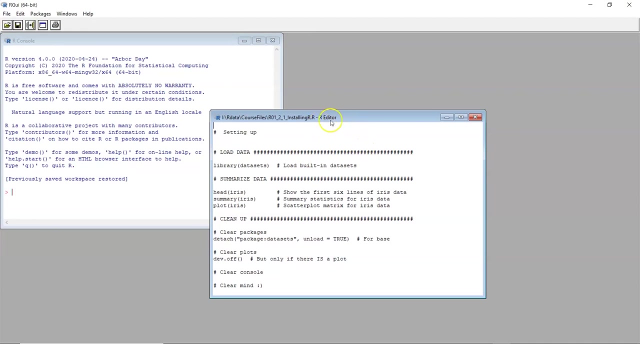 and if you have some scripts or files already written in the format of R, you can use those. so I can click on open script and that takes me to a page where I have some files which are already existing. I can just select this one and click on open and that shows me some options here. so I have 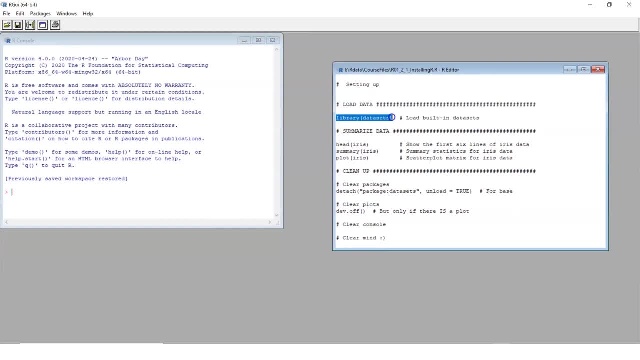 an editor which shows me, say, if I want to get a library to use built-in data sets, I could summarize the data, I could do a cleanup and we'll see all of this, but I would suggest using R studio rather than just using base R. however, install it and then you can start working with R and you can. 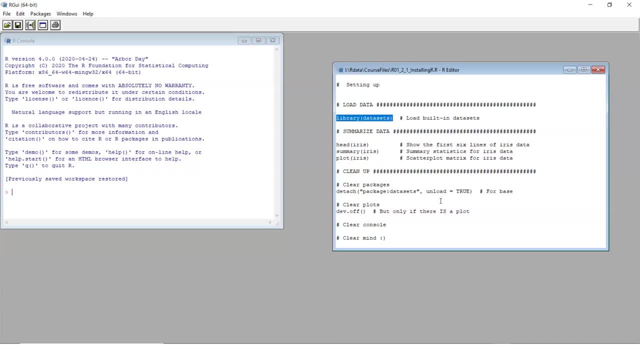 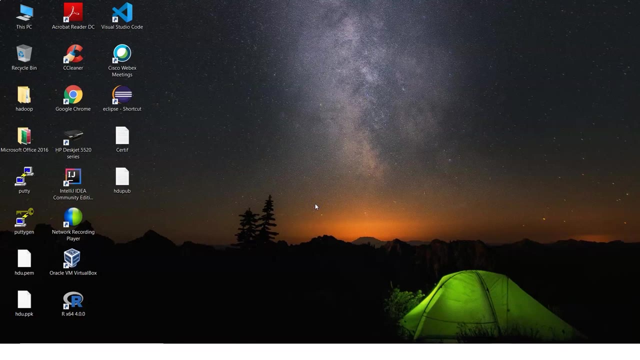 start installing base R would be required and, depending on your machine configuration- like mine is a 64-bit- I have chosen 64-bit while I was setting up base R. now, when it comes to R studio, it is basically a package which makes working with R easier. so, to install R studio, what you 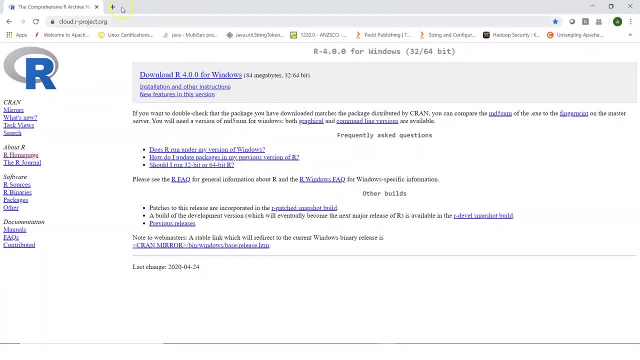 can do is you can go to the R studio home page or you can just go to google and say type R, and then you can start working with R, so you can start working with R and then you can start R and then you can start working with R and then you can start working with R and then you can start. 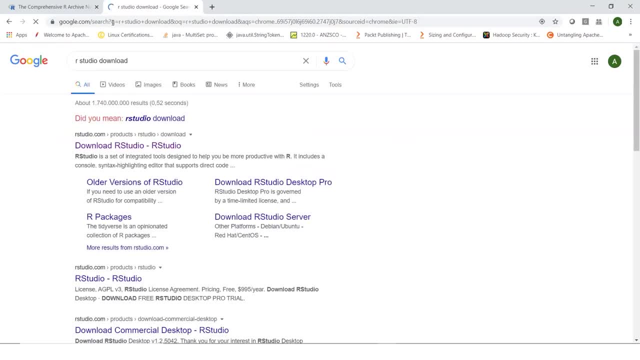 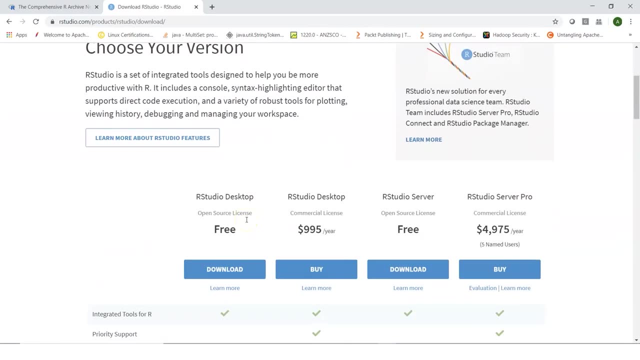 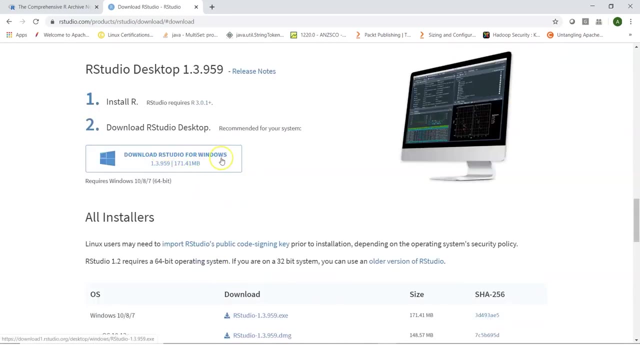 clicking on R studio download and then it takes you to this page. you can click on this, which says download R studio. you can choose your version. you can go for the free version, that is, R studio desktop, and you can click on this download and then you can download R studio for windows, which 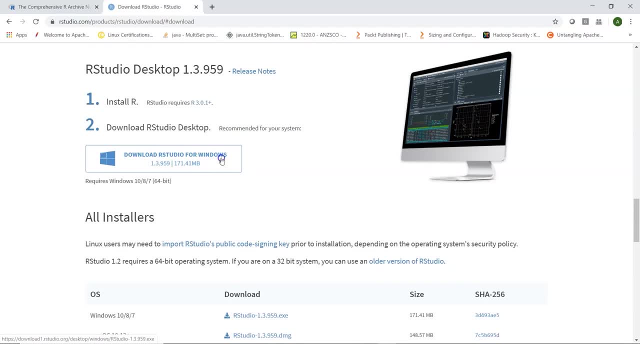 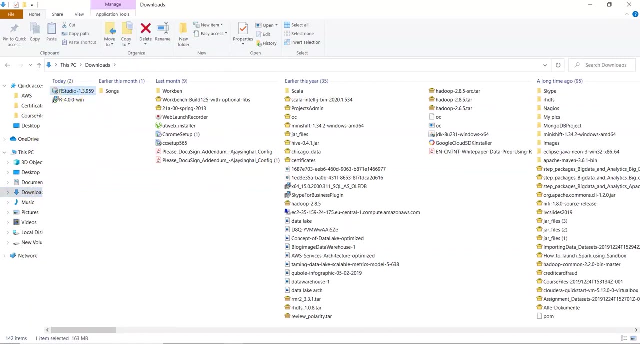 I have already done and then you have to run through the steps. so just click on this one and I already have R studio here right now. I can just basically use that. so, for example, if I go to downloads and if I look for RStudio, if I do a double click. 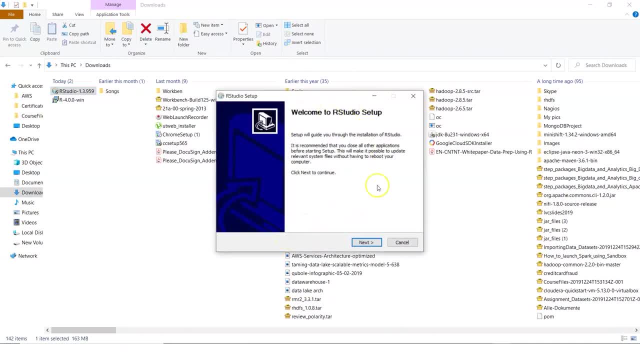 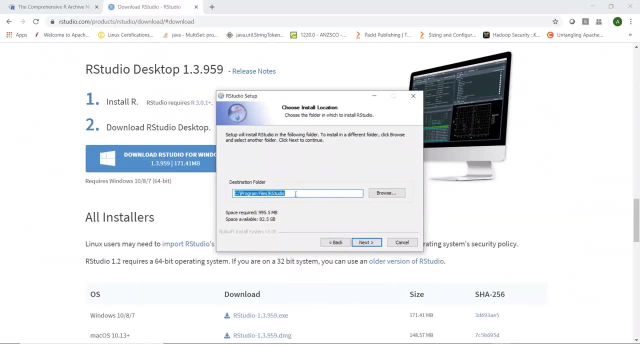 I can say yes, and then it takes me to the RStudio setup. just click on next and here you can choose the location. if you would want to place it in a specific location, click on next and then it says: select the start menu folder. so let RStudio be chosen here. click on install and then it will. 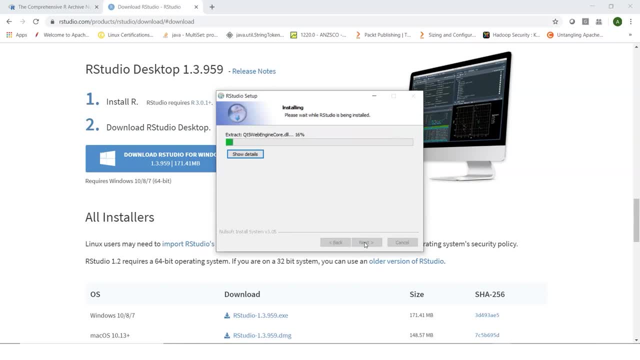 basically start installing this in a particular location now. in my case it is already existing right, so we can even click on show details and see what it is doing, what packages or what executables it is extracting now. once this is done, then you will be able to use RStudio. you can also 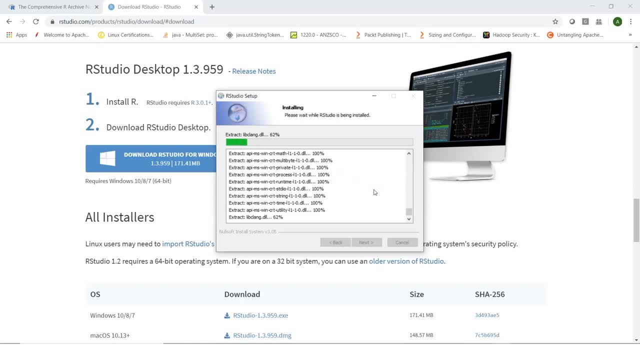 add a shortcut to your taskbar and you can continue using it. so I've already done this. this might take couple of seconds. just wait for this to complete you and you would have RStudio, which is an easier way of working with R. so a lot of developers. 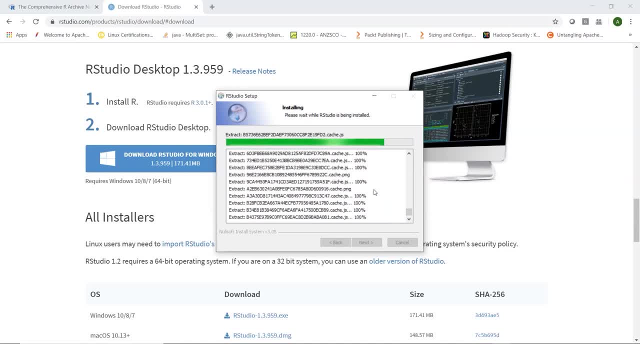 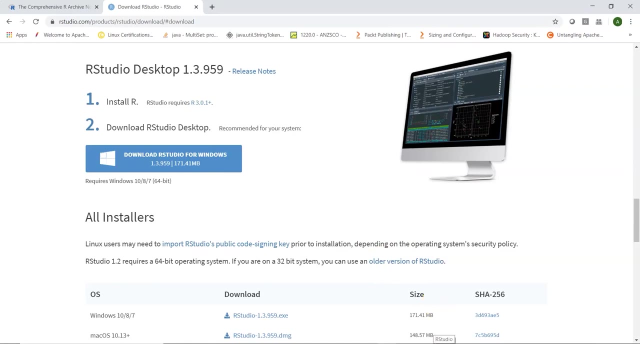 across the globe would be using RStudio when they are working with R to work on their data science or programming requirements. now, let's just wait. it is almost done and now I can click on finish, so so that part is done. you can add it as a shortcut, so RStudio has consistent commands. 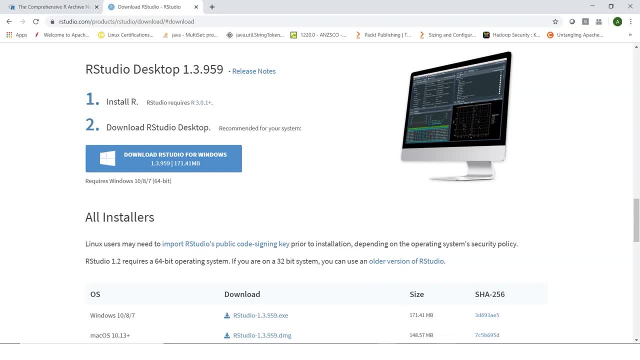 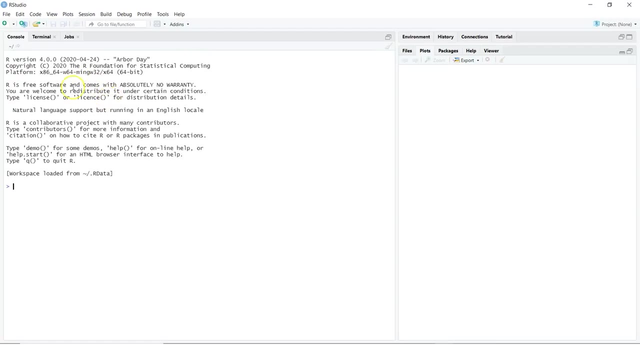 it has unified interface, it makes easy to navigate and manage through R and it is set up on top of your R base. now if I click and open on this, so that's my RStudio which is coming up now. here you see console which will show you the result where you can give your commands, so where we can get text output. now 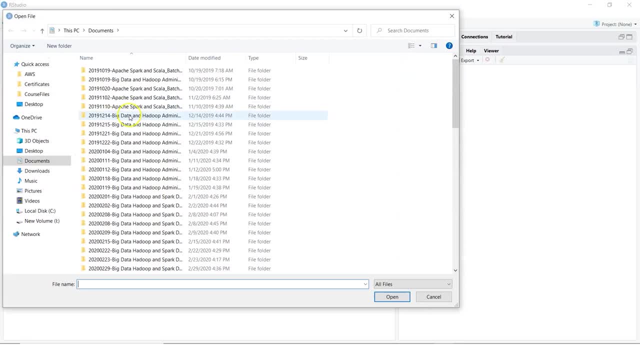 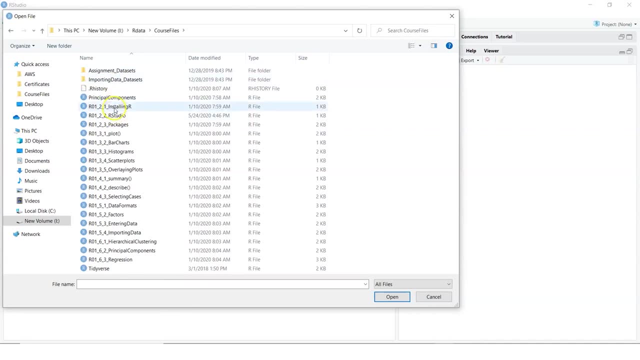 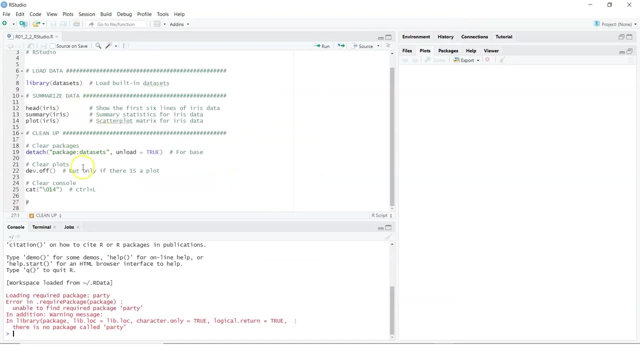 again, I can choose a file, so I can just say open file, and then I can go into my RStudio and I can go to a particular location where I have downloaded some data, and then basically I can choose, say for example RStudio, and that brings me here. so now you have your script, which has some commands. 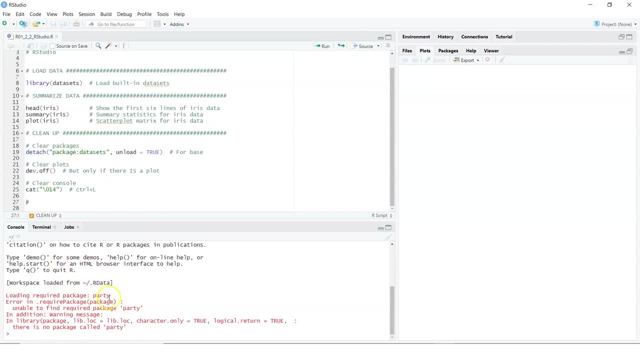 right on the left bottom you have console where you can see the output. on the right side you also have environment now that is, to use or provide variables. and then we can also have plots where you can see the output. on the right side you also have environment now that is, to use or provide. 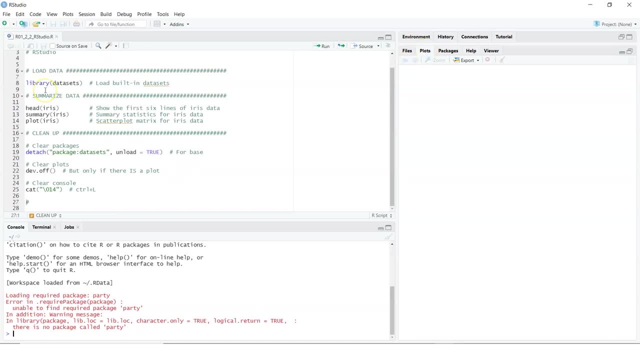 variables, and then we can also have plots, which we can see here now we can look at this as an example. so here I am loading the built-in data sets. so what I can just do is I can place my cursor here and I can just do a control enter, and that basically loads the built-in data sets, which 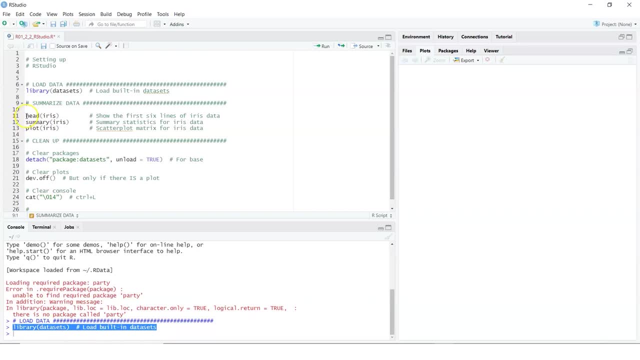 we can see here that has been done. now there is an inbuilt iris data set and we can just use head option to look at the first six lines of iris data set. so just place your cursor and do a control, enter and that shows you a summary. 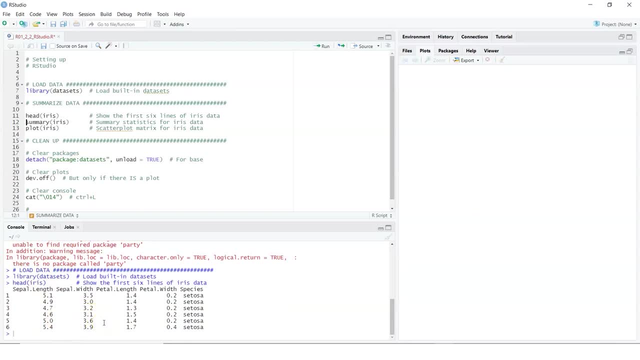 basically the first six lines of this data set what it contains. we will look into this data set later. this is a default data set which you can easily find when you are working with R. you can also have your cursor placed on summary and then just do a control enter so that basically shows. 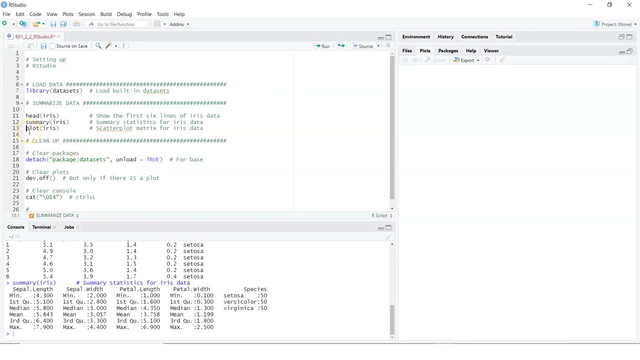 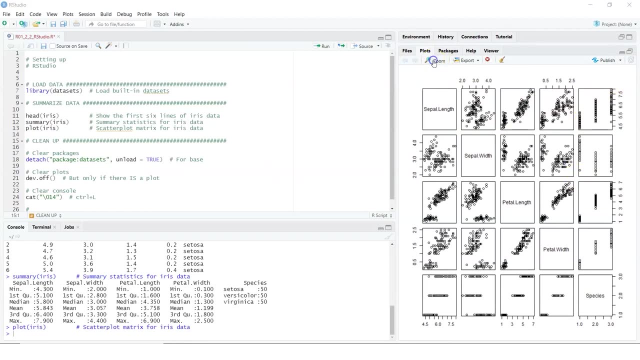 you summary statistics for iris data. you can do a plot and that basically shows you the plot, which you can also maximize and look at it in full screen. you can just do a zoom if you are interested in looking into this, and we will discuss how or what kind of information we can infer from. 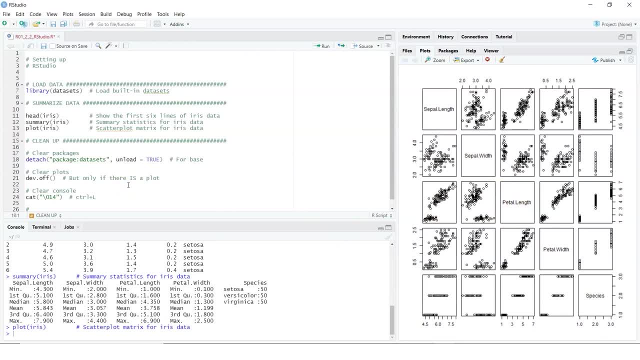 the plots. now, when it comes to cleaning up, you can just do detach and then we can say package data sets. and here we had loaded those data sets. so we are just doing a detach and we can say unload equals true. so I'll just do a control enter. I can also clear of the plots. 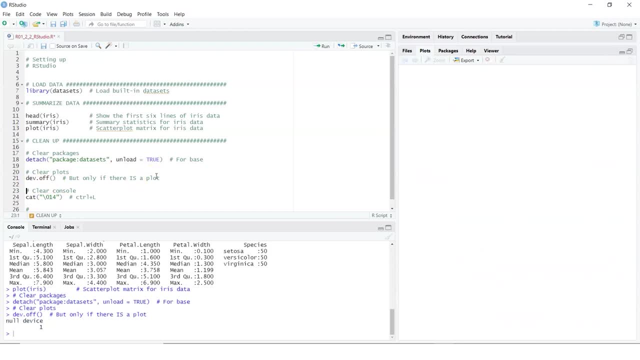 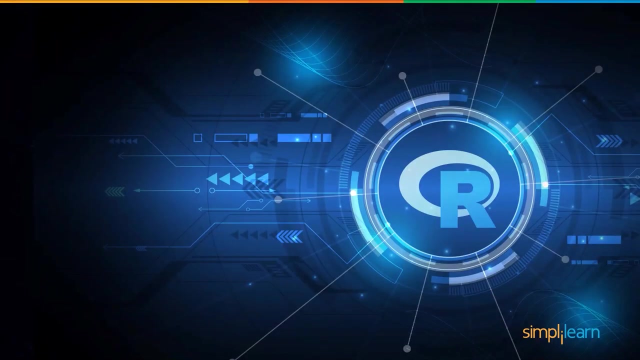 plots by doing this, for whatever plots we had, and we can either do a edit and then we can do a clear console from here, or the shortcut is ctrl r and you can clear off the console. so that's a simple way of starting your working with r by installing r studio. so let's continue learning about working. 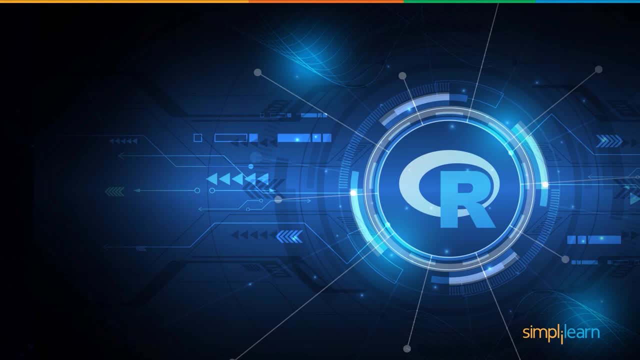 with r and basically, the first thing which we should learn here is about variables in r. so variables, as in any programming language, is a way to store your data value, factor of list values or a data set or object. in r. it allows us to conveniently reference the variable name. 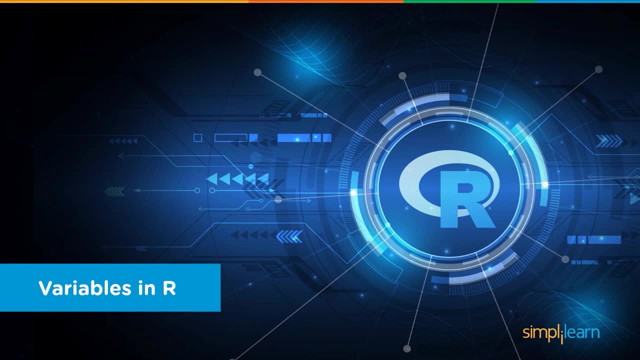 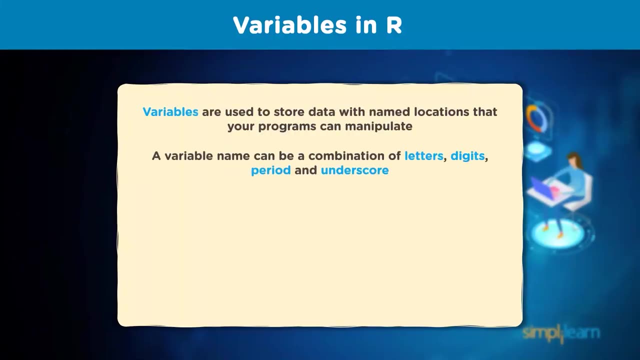 basically saving us from rewriting the data value of the variable name. and then we can start working with r and basically the first thing is about variables in r. so variables, as in any programming language, is a way to store your data, value or object many times in our program. so when we talk about variables in r, they are mainly used. 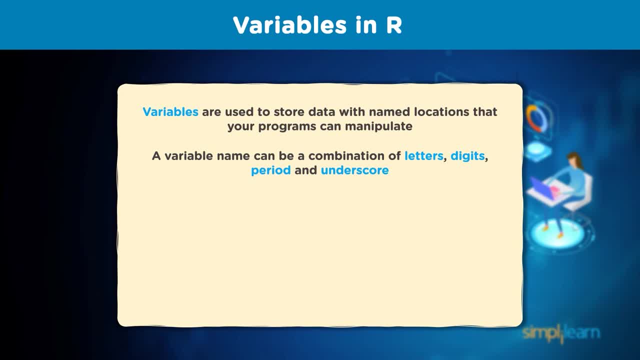 to store data with named locations that your programs can manipulate. a variable can be a combination of letters, digits, period and underscore, so you can have some valid variables as total sum. you can also have dot notation, so there are different naming or style conventions in r and we can use dot to separate names in description of a variable. we can also start a variable with: 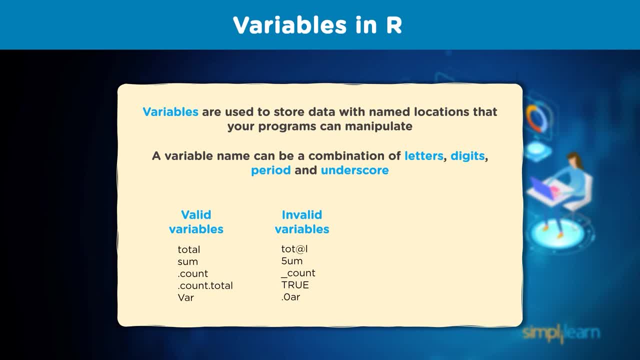 dot. we can include numbers in a variable and remember r is case sensitive, so we have to. whenever we declare a variable, we need to remember what case was used as in in the name of the variable. and there can be other conventions also, such as using an underscore or even using 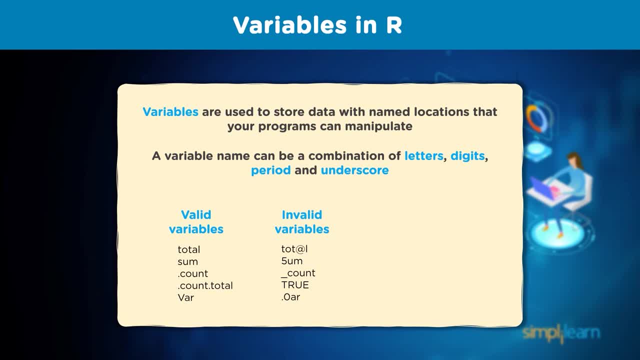 a case in between the variables. so variables can only consist of letters, numbers, periods, underscores your dot, followed by a letter, not a number, and we can declare our variables. we can also look at the type of the variables and the class to which it belongs, so there are some invalid. 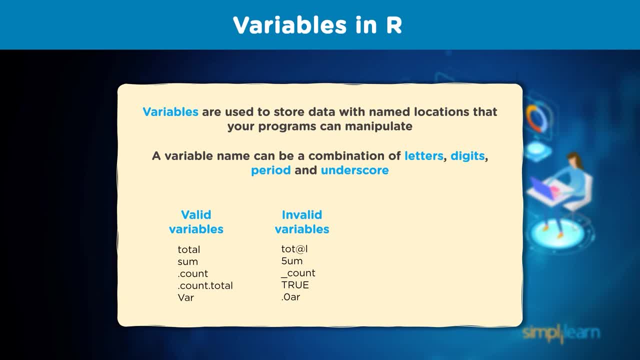 variables which we are seeing here, so that also needs to be remembered. so this is an example where you can use an assignment operator, which you see here between x and 10, to assign a value to a variable. you could also do that by doing a dot y and then assign a value. you could be doing that by using a. 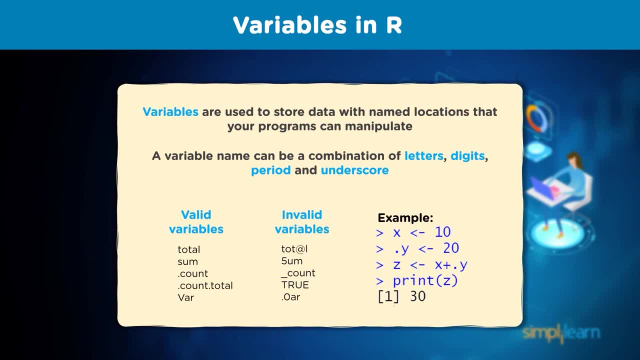 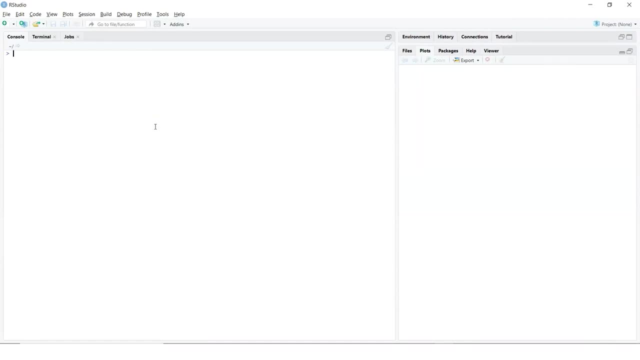 z and then having a computation done between x and y and finally you could do a print. so let's see some example here before we move further, and for that i can bring up my r studio here. so, as i said, we can basically have different kind of variables or naming conventions, for example. i could do something 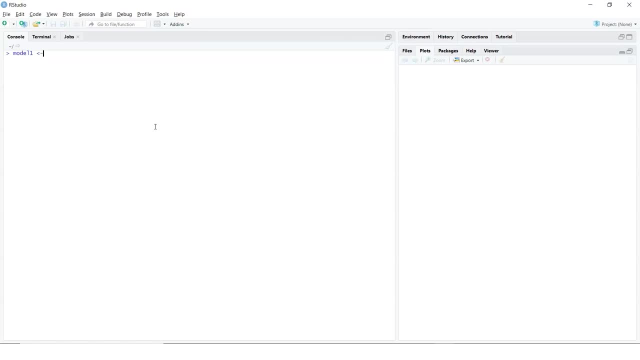 like model one, and then i can basically assign this. so this is just a variable and i could be assigning anything to it. i could be assigning different data types, which are available here. for example, i could do something like this and i could do a control enter. so 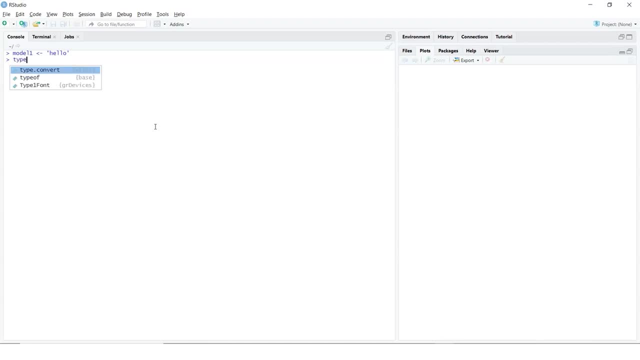 that's my variable. i can always do a type of and then basically i can check what is the type of my variable, so it tells it's a character. i can also do a class and then i can basically say: show me the class and that shows me it belongs to the character class. we'll learn about data types later, but we 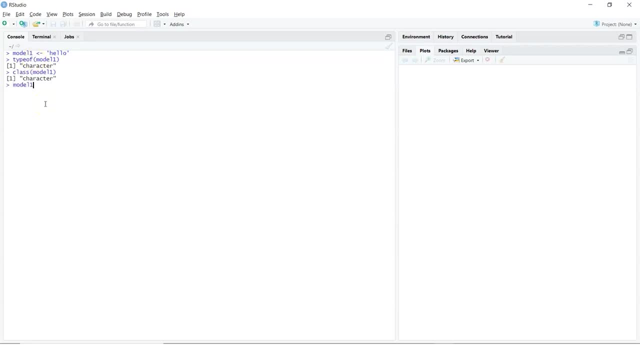 are using assignment operator. now, if i say what is model one, it shows me the value. but if i would do something like this, then it says object model not found. and why? because it is case sensitive. the variable which we had created was all in lowercase and the one which we tried to call 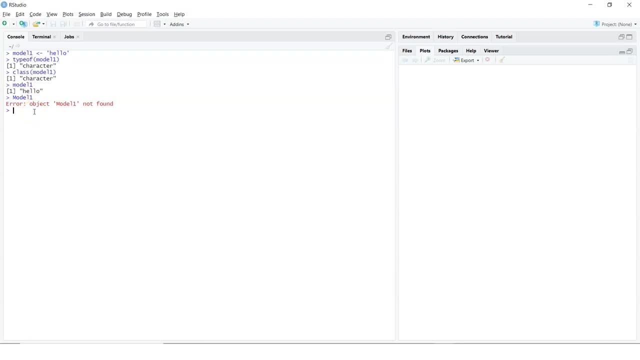 was starting with an uppercase, so you could have variables created. in such way. i could also do something like hello- underscore string and this could be my variable, where we are using an underscore, and then we can just give in something here and that becomes my variable, which you can. 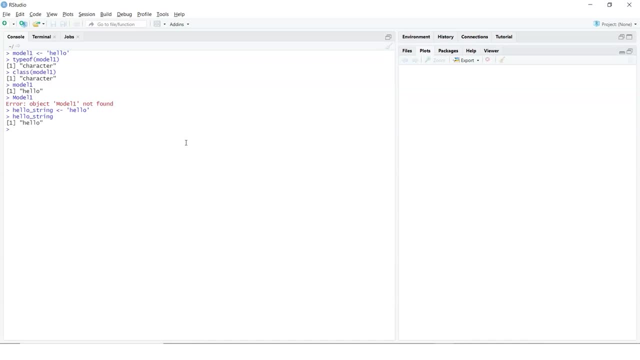 always call and check what is the value of that? you could also be doing something like this, so you could be using different cases, and then i could say something like this: and that's also my variable, and then i can basically look at the value of this variable. 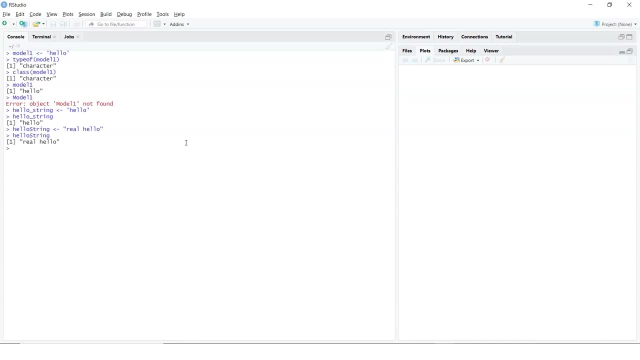 now, if we try to create a variable where we start the variable name with a number, what would happen? so if i say something like this and then if i try to assign a value to it, for example, let's say hundred, now this one will throw an error message because you cannot have your variable start. 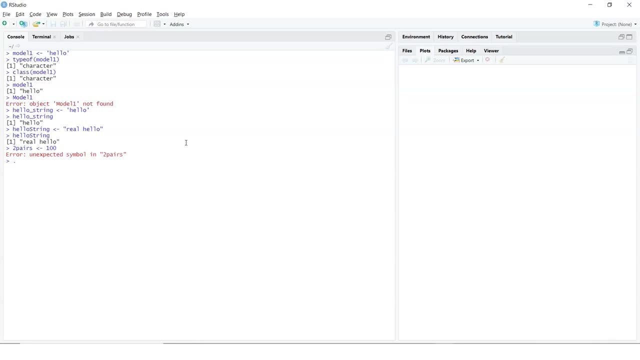 thing with a number, but if i used period and then basically give something like this: and let's try doing this by giving it a number. so if you see, here, since we gave a period, the rule is that it should be followed always by a letter and not a number, so i could just remove this and that. 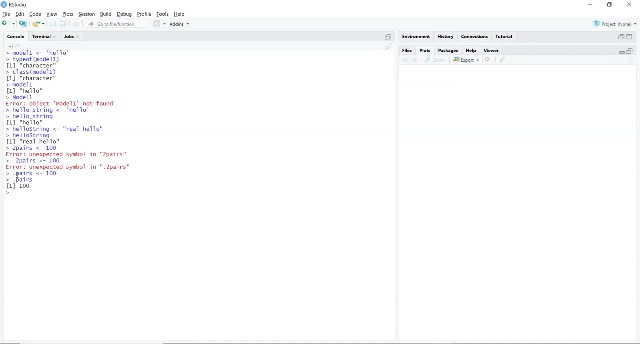 works perfectly fine. so these are some naming conventions which, when you practice, you will learn about. so now i can assign a variable by just doing a dot pairs and then assign any value to it. but always remember if you are using a period, if you are using a notation, then in that case that should always be followed. 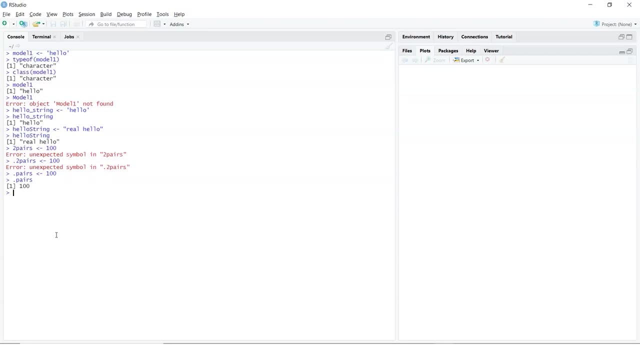 by a letter. one more thing which is always practiced in a real-time environment is that we cannot have spaces when we are creating variables. so, for example, if i say first num and then i try to assign this a value, it basically fails. but obviously i could have done this by doing a underscore and that perfectly. 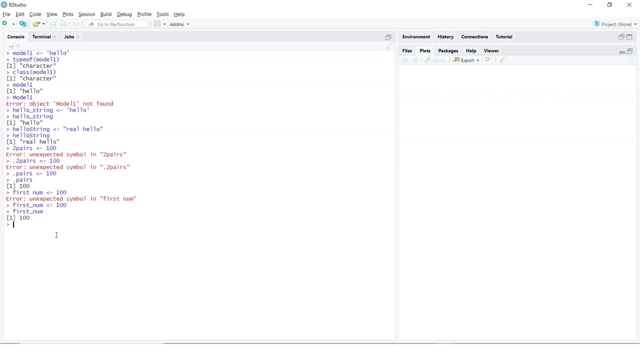 works fine and you can basically then call the value for this one always remember. one more standard practice which is followed in real time environment is you will try to have variable names with a little meaning to them. so, for example, if i would create a variable and i would say, for example: 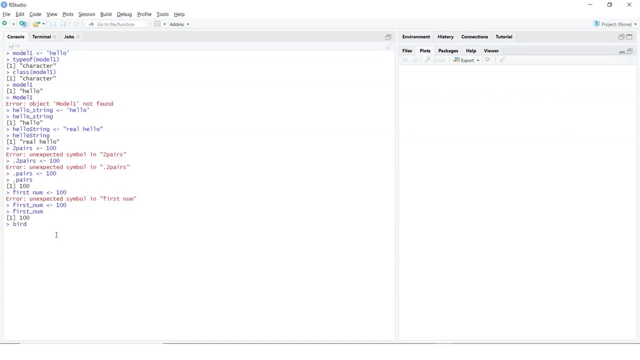 let's say bird, that's my variable name, and then if i assign this a value tiger, it works fine, but then it really does not make sense and that would basically create a lot of ambiguity in our coding. so it is always good to say, for example, animal. 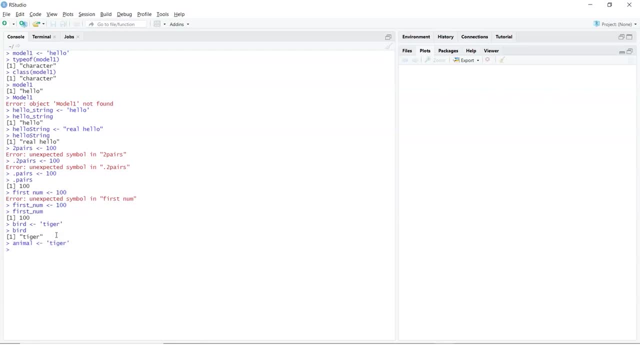 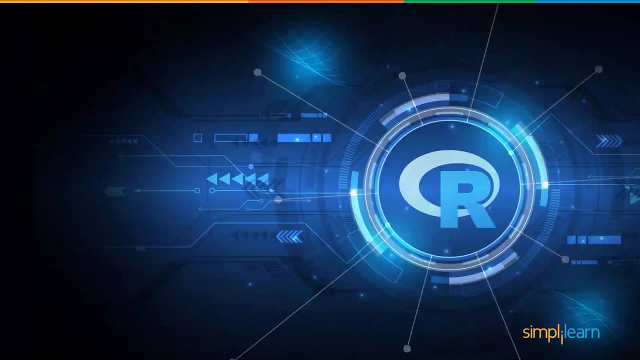 and then i would say, okay, so tiger is an animal, and that basically not only allows me to assign a value to the variable, but it is also a little bit more meaningful. now, when we talk about variables, it is also good to know the different data types which are available. 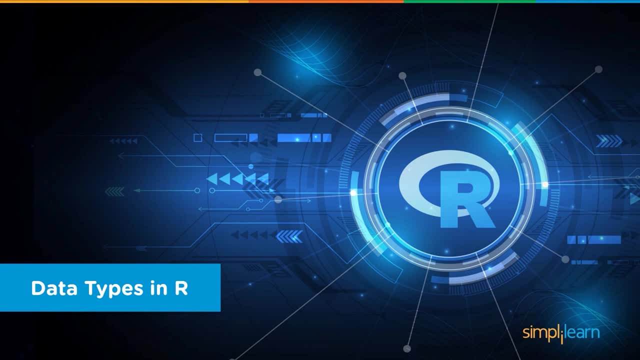 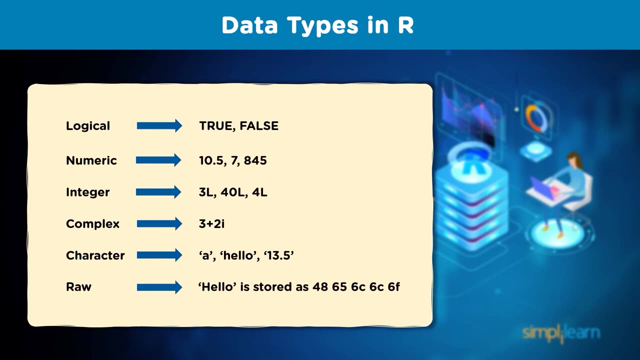 in R. now, like any other programming language, R also supports different data types: logical data types, such as true and false. you have numeric values, which is say these numbers. you could also be creating an integer which is 3l and 40l, 4l and so on. you can have a complex number. 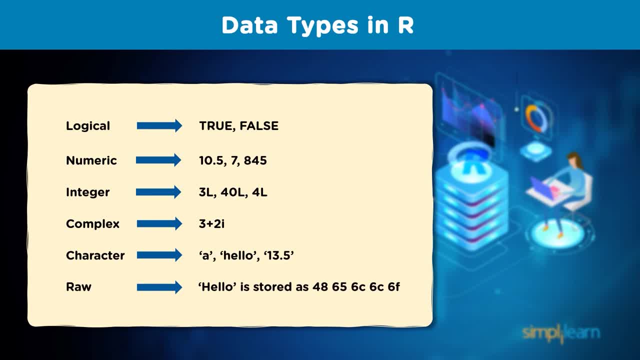 you can have characters, which can be just letters, or a set of letters, or anything which is within the quotes, or you can even have raw data. so these are different data types. we can again see quick examples here on data types. let me come out of this one. and as we saw already when we created 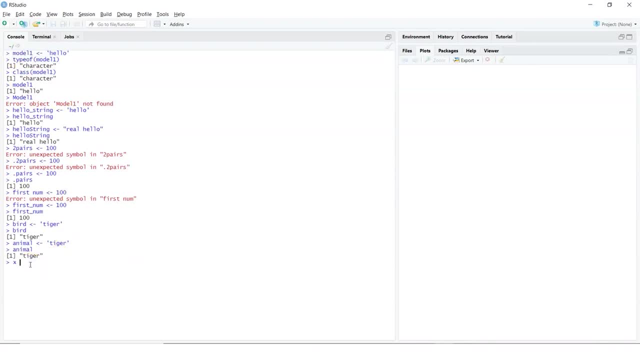 model one. this was character. now i can just say x and let's say 100, and obviously this is going to be not my integer, okay, so let's see this. what is this one? this one, by default, is double. it is by default double. so if i would want an integer, then 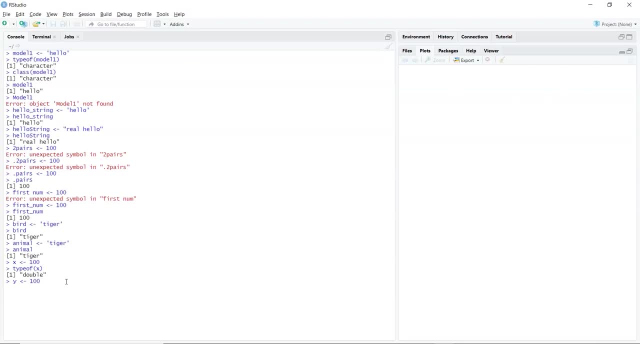 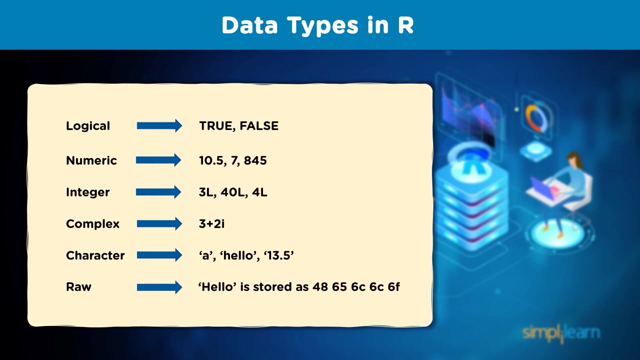 i would say, for example, something like like this: and this one you can check by using type off and you can see the value for this one. so this is an integer. so, similarly, you can have character, you can have complex, you can have raw data, you can have numeric. 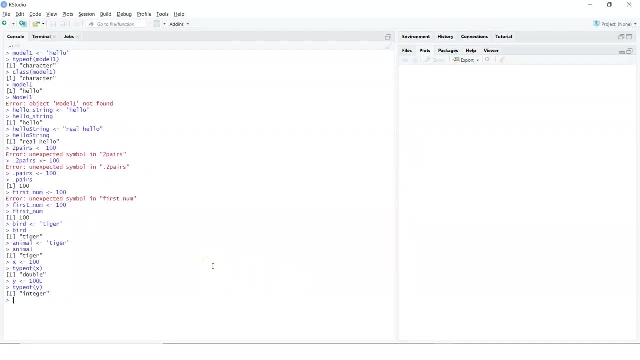 values. so all these are different data types. you could also be saying, for example, i would want to check the boolean so i can check this and select this one. and now, when i check the value for a, it is true, and we will learn about logical operators where we can basically be using these values assigned. 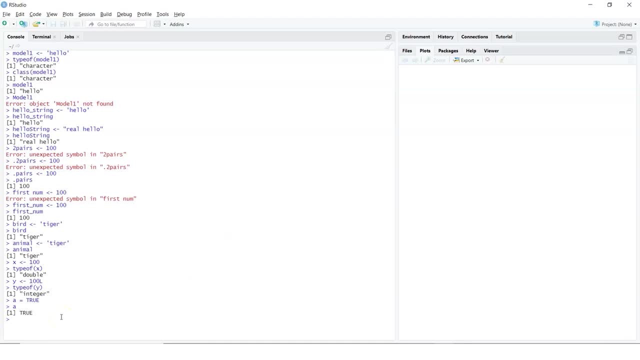 to the variables, to compare, to compute between different variables. so this is a simple, small example of using variables. so we have seen here using variables and also using the assignment operator and then assigning values to the variables and different naming conventions. we can also be using different data types which are supports and work with the. 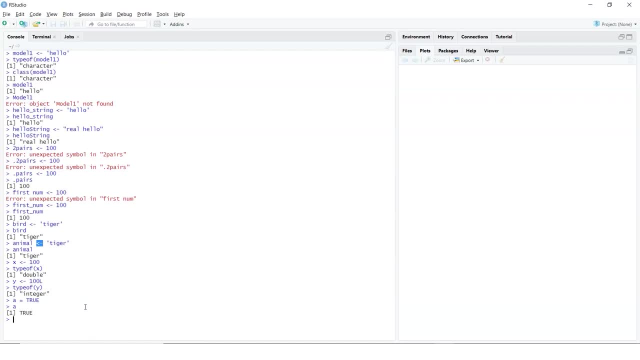 variables. now, once we have learned about variables or data types, let's also just first learn about your operators and how they can be used in your r programming language. now we might be intending to do some calculations on numeric values, find out differences between values or say, for example, compare values, so in that we can be using different kind of operators. 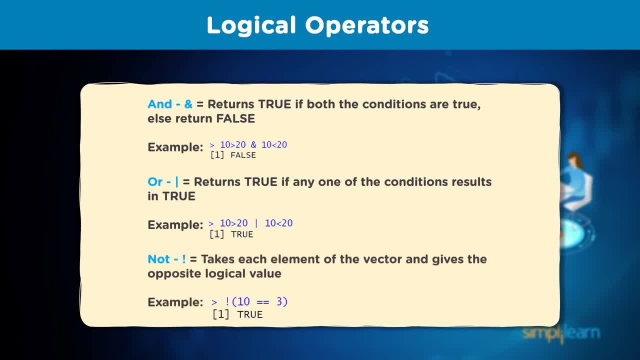 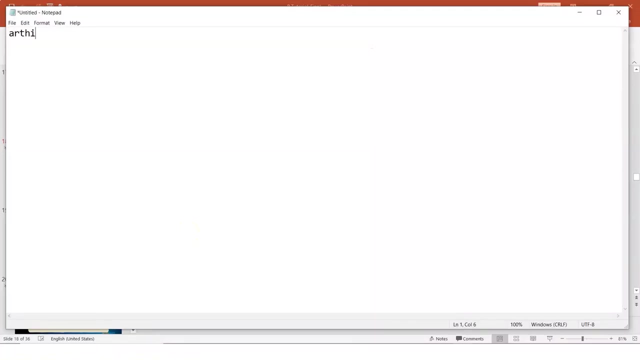 so we have various operators. we have arithmetic operators, we have rational operators, we also have logical operators. so before we straight away look into logical operators, let's also understand about the basics, such as your arithmetic operators, which supports, for example- let me pull up a notepad file here- and when we talk about arithmetic operators here, we are talking about your. 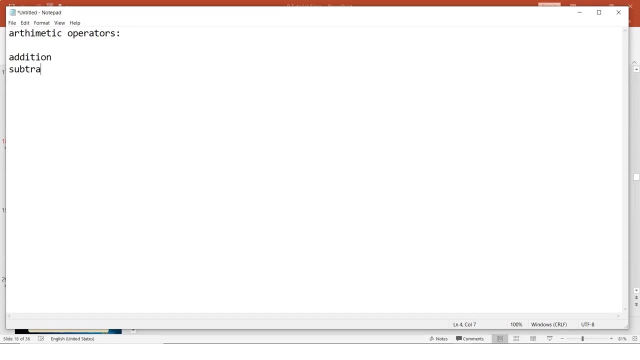 addition, you have subtraction, you have multiplication, you have division and you have remainder or modulus and you have exponent. and what makes it also important is that when you are using arithmetic operators you also need to know about the order of operations. so when you say order of operations, always the priority is to parenthesis, so that takes the priority. 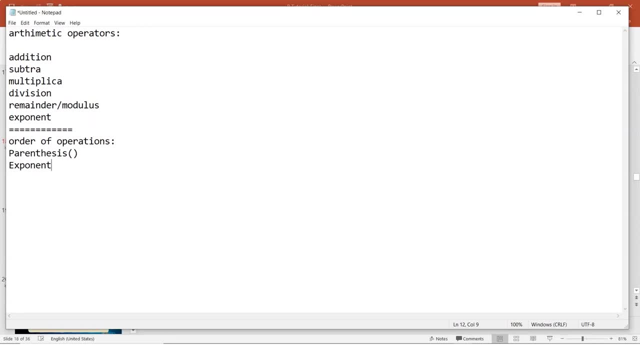 have then exponent or your computation, if that would involve exponent. so let's say exponent here, which is then followed by your multiplication and division, and that one also follows an order of left to right, whichever comes first when we talk about multiplication and division, and similarly, when we talk about addition and subtraction, it is left to right, whichever comes first. so these 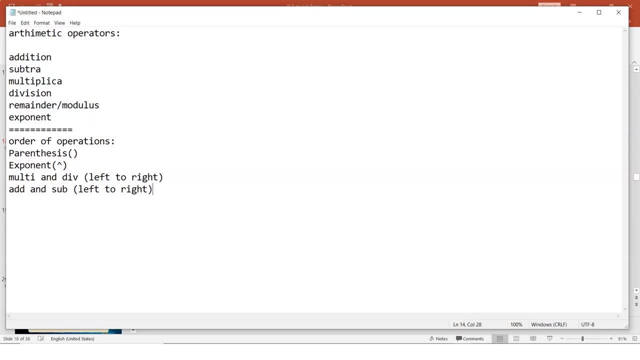 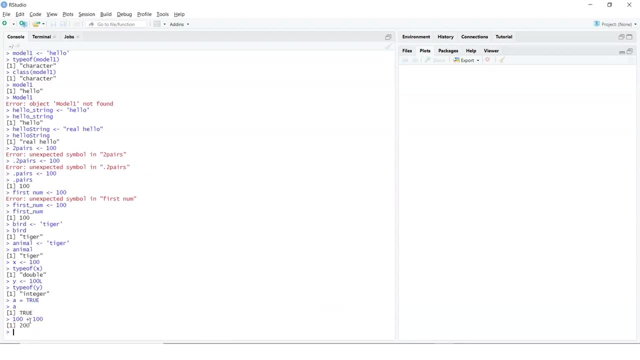 are some of the arithmetic operators. now we can see some examples here quickly, although these are some simple examples. so, for example, i can say 100 plus 100 and that gives me the value right. you can always do a 100 minus 50. you can do a 100 multiplication. 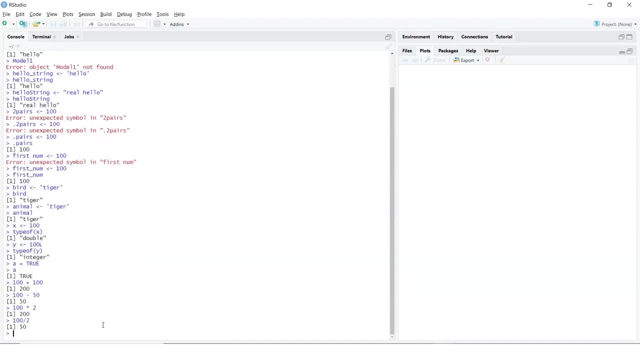 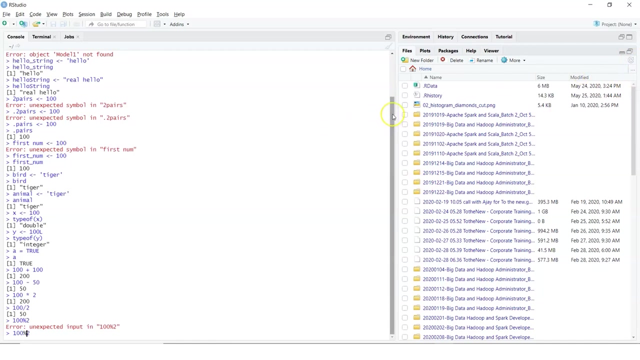 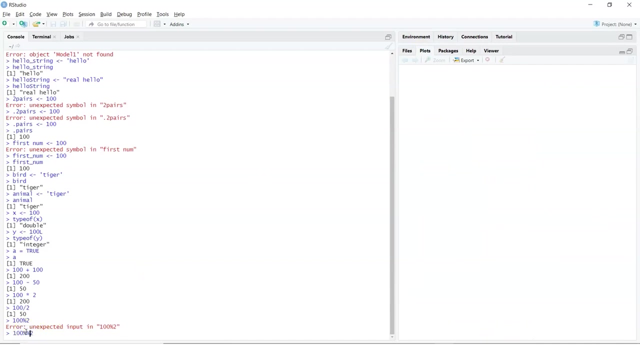 you could do a 100 division 2, or you could also use modulus 2, which basically gives you an error here. so i will, oh, just give me a minute. so let's give here one more percentage sign and that basically says what would be the remainder. so if we would want to look at the ordering when we are using 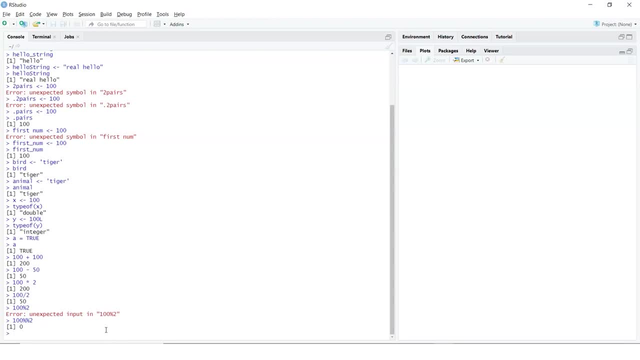 this arithmetic operators. we can see an example. so, for example, if i say 34 plus 46 divided by 2 gives me 57. however, if i use 34 plus 46- in parenthesis, which gets the priority, and then i divide, my result is different. so, understanding what arithmetic operators you can use and also the ordering in which, 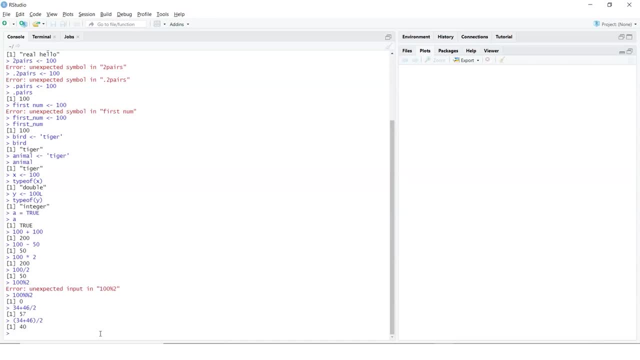 that leads to the computation is very important. so we can use all of these arithmetic operators and to control the ordering we can be using parenthesis or we can have our computations ordered with what kind of operation we would want, whether that would be multiplication or division, addition or subtraction. now, at any point of time, i can always do a control l and that allows me to. 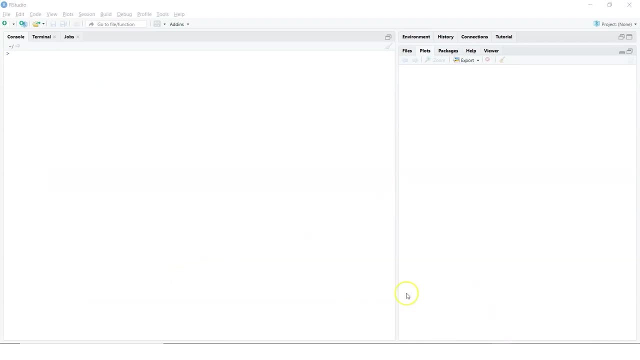 clear my console. let's continue our learning and let's learn about operators. so when we speak about arithmetic operators, we see that allows us to do computations. but we have also rational and logical operators which help us in doing our computations or comparing values or sometimes finding difference between different values, whether those are group. 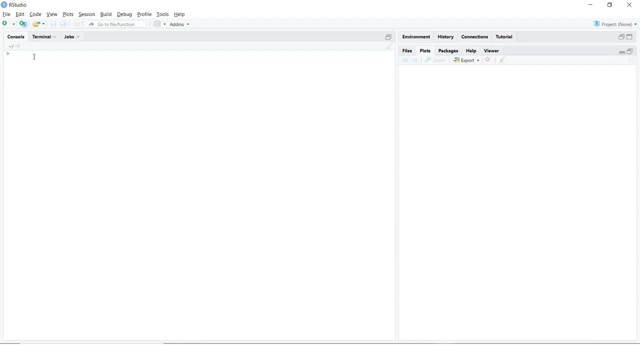 of values or whether those are individual values. so with your rational and logical operators you can compare data values. so if we would want to see if the values match or not match, or if the values are above or below equal to something, and so on. so when we talk about your rational operators, 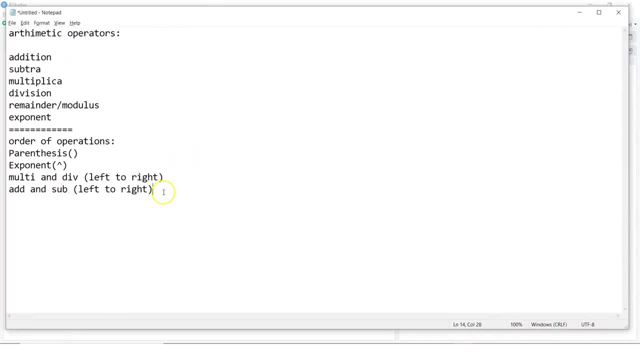 we basically have, in case of rational or logical operators, rational or logical operators. so we obviously have greater than. you have less than. you have greater than or equal. you have less than less than or equal. you have equal to and you have not equal. These are some of your. 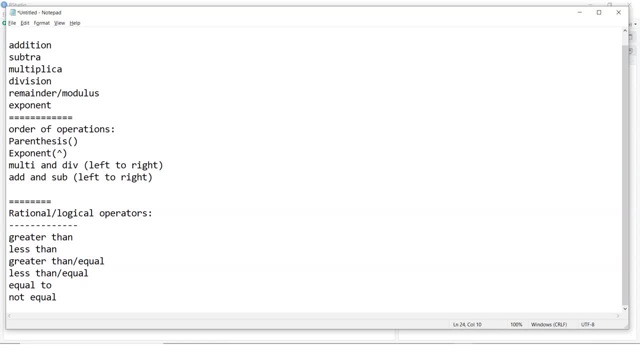 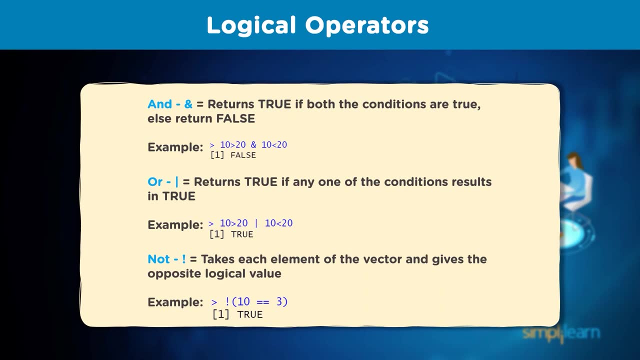 rational operators. we can say: And when you talk about your logical operators, then you have and you have or and you have not. So and is when it compares two values, So it returns true if both the conditions are true, else it will return a false. So for example, 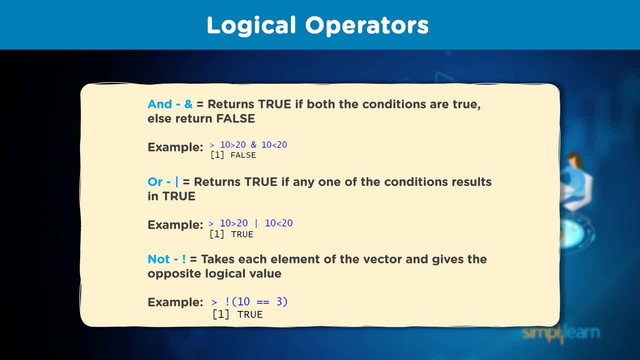 if I have 10 greater than 20 and 10 is less than 20, now that's not possible And we are comparing the result of both of these, So we are checking if both the conditions are true. and that's not really true here, So we see the value as false. Now, if I would, 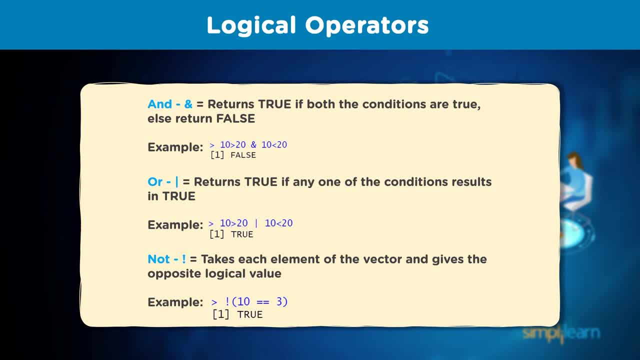 have replaced this one, this and with or. it would check. Even if one of the conditions is true, it would basically show me a result as true. You can also use a not operator, which takes each element of the vector and gives the opposite. 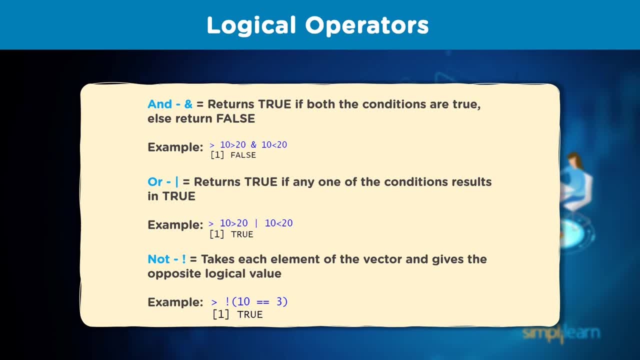 value. So we can be using any one of these operators and then basically do our computations. So let's see some examples about these logical operators Now. either you could just be assigning values to your variables and check, Or you could also do the same thing. So let's see some examples about these logical operators Now. either you could just be assigning values to your variables and check, or you could. 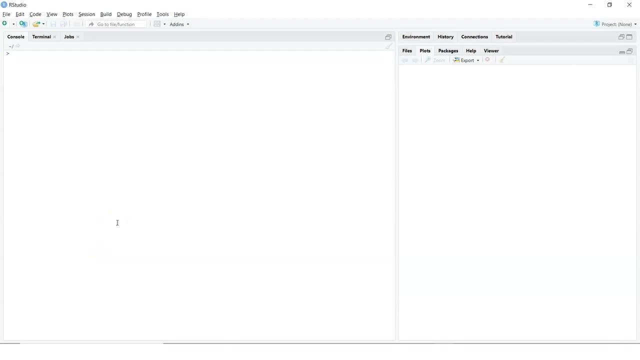 also be picking up a data set from your machine and then try to use these logical operators. So, for example, if I say x has been assigned 100,, y has been assigned 200, and if I try to say x equals y, so that already checks. 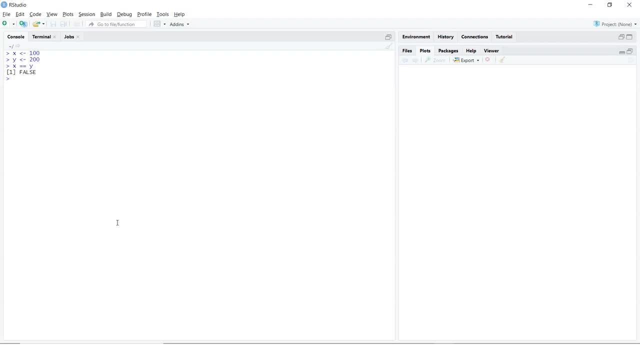 The value in comparison tells me that's not true, it is false. and if I would have used a not operator, for example, if I would have said something like this one, so it tells me true. So I can just check simple conditions like this. I can say: is my y greater than? 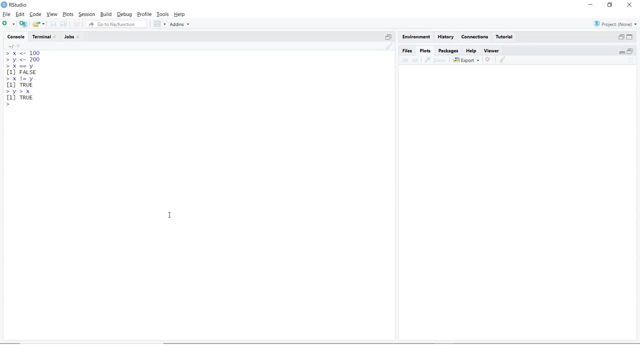 x And that tells me, yes, it is true. If I say y is greater than or equal to x, well, it would still say true. Well, it would still say true, Because when you are saying greater than or equal to x, so when you're saying this one, it works fine. 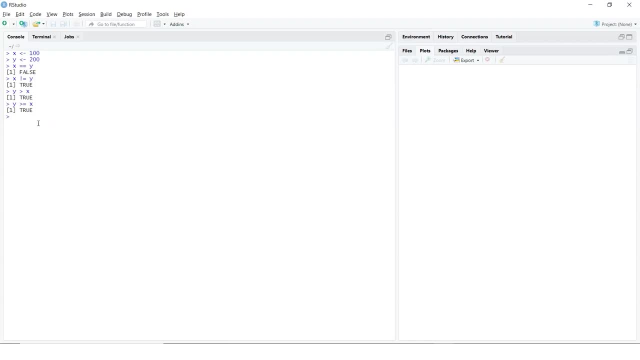 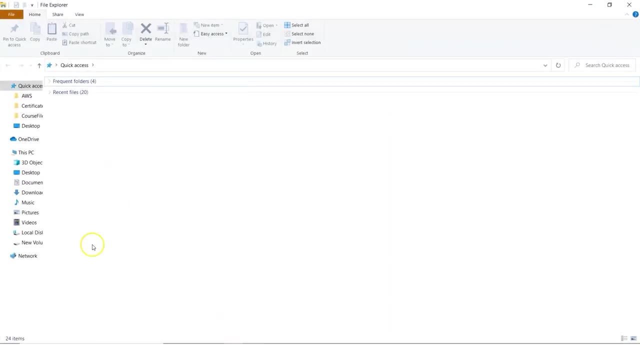 Now we can also be picking up some data set, and for that, what I can do is I can pick up one of the data set from my machine so I can go in here and I have the exception. Okay, I said I'm going to check and I learned this. 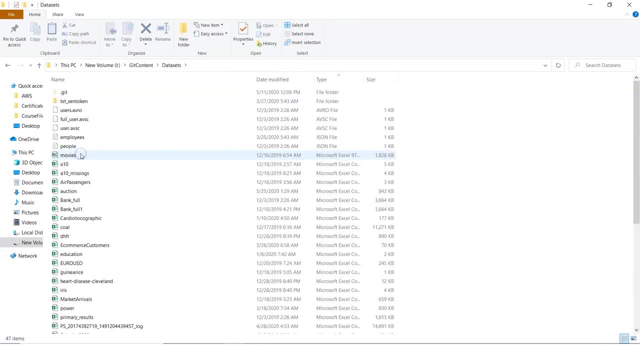 Okay, Here's y. Okay, Now that gives me the data set values. I can add this up to scores and this is the number of variables, some data sets. let's look into that and I would be interested in taking this auction data set and loading the values here. so I'll get this path and I will 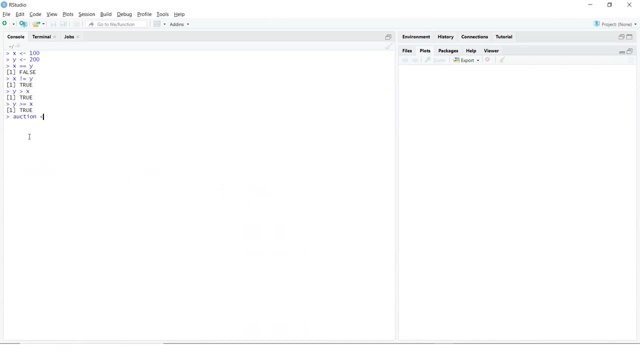 come here. I can use auction as my variable name. you could have given a dot separated name. for example I could have said auction, dot data, if this is what you want to do, and then you can assign variable a value. so here I'll say: read dot CSV and I intend to pick up a file. so I give this path and when we are 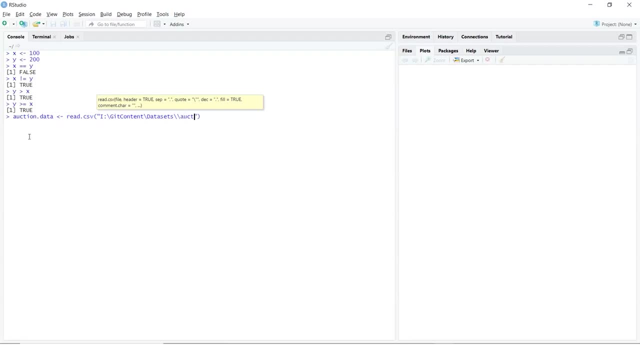 working on Windows machine we need to give a double slash, so I'll say auction dot CSV. now I could give other things, like header being true. what is the separator? if you would want to fill values to take care of missing values, we can look at all of those. so here I'll just add a backslash, I will add a. 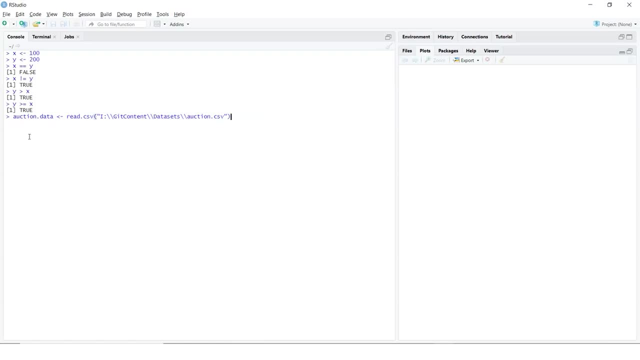 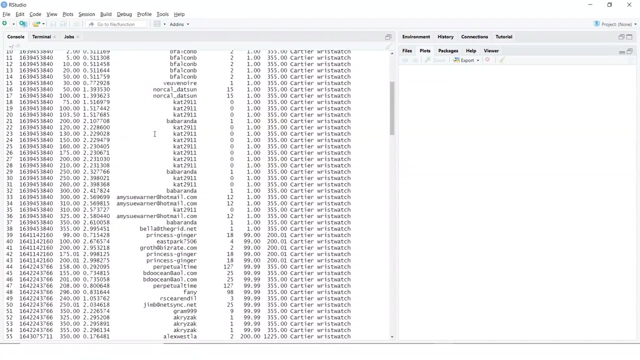 backslash and I will basically just do a control enter. now I can look at the values of this by just doing a auction dot data and I can see what values it has. so it has a lot of data here. it has a lot of your data here. you could have used some. 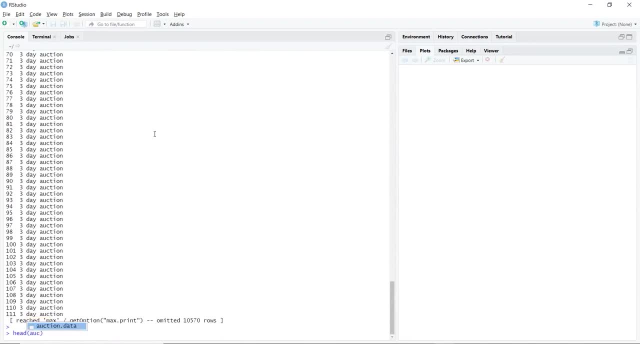 other functions, which we can see later, where I can choose head and I can see the first top five values. so we can basically assign data to the variable and continue working on this. now we can keep it simple, so let me repeat this step and here I will say auction as my variable. 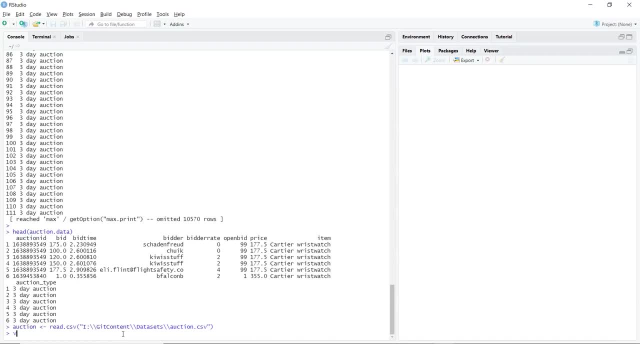 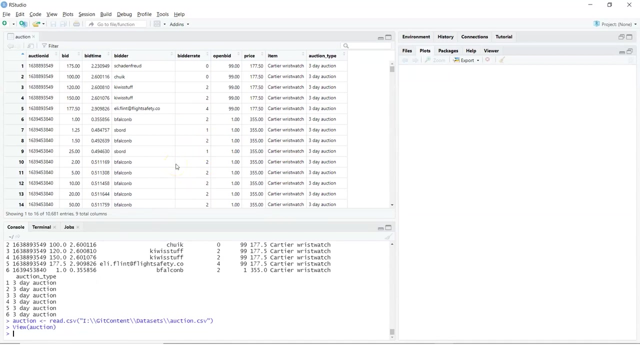 name and I'll assign this so I can basically do a, also a view on auction. so auction, and then basically that shows me a tabular form map of the data which allows me to look into the data and basically understand it, and then I can, you know, use this to work on variables. so what I 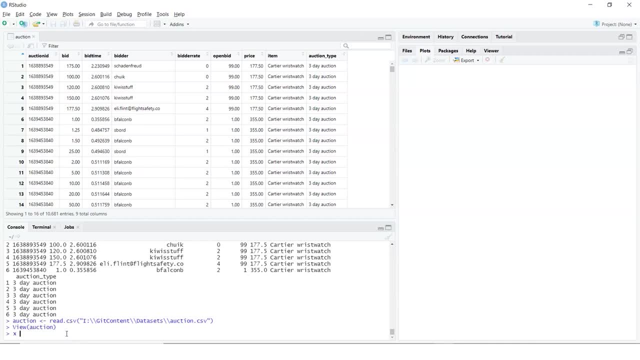 can do here is: I can say X and let's say, assign some value to this, for which I would want to work on my data set, which is auction. now, what do I want to do here? so let's use auction, and then I can use a dollar symbol and I can choose which column I'm interested in. so for 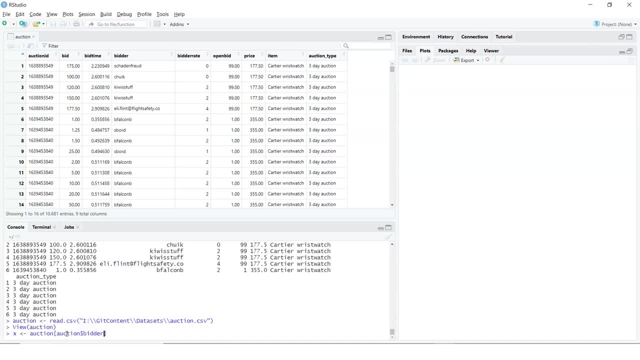 example, let's choose bidder and I can just give a value to this one. and let's pick up a name. so let's say tweak and that's the name, and I can be assigning all the values to this, or I could say I would want to use another. 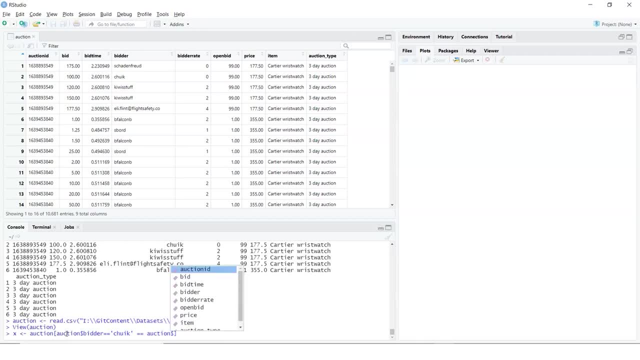 condition. so I'll say auction dollar, and then let's take this value of bid and let's say it is equals to hundred, and then I ended up with comma and I can try doing this now here. it gives me a problem because what we did was we did. 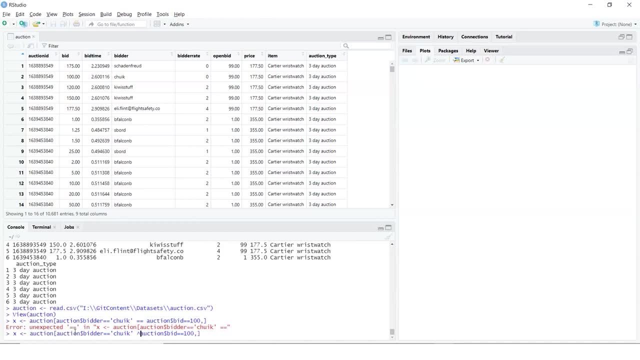 not use the right operator. so we will say, for example, and so I will say: X is being assigned, the value of auction bidder being tweak and auction bid value being hundred. so now, once we do this, I can look at the value of X and that shows me the value. so this is just a simple example of using a logical. 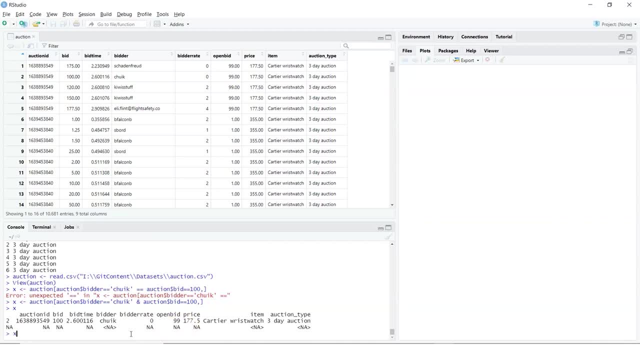 operator. now I could have just said instead of: and I could have used or, which is basically a, a pipe which you have to use, and that gives you or condition. and now hit on enter and if I now look at the values of X, it will show me a lot of values because we have given a or. 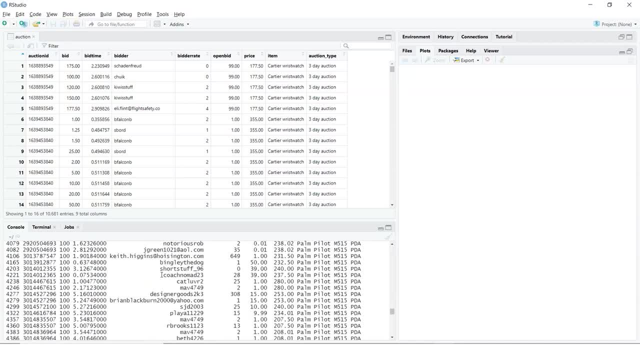 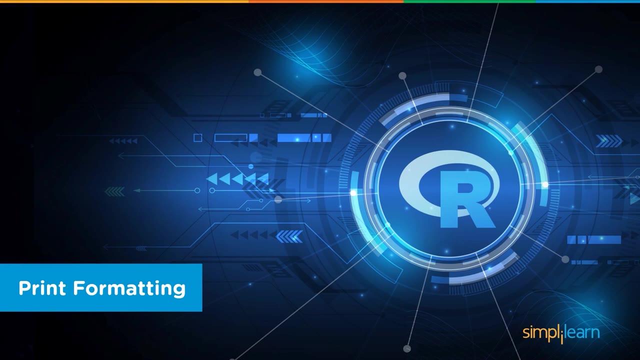 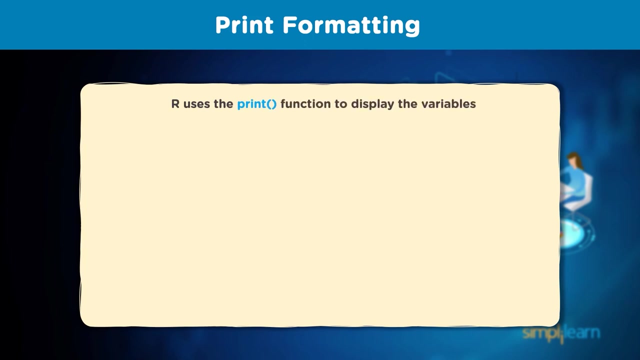 condition which basically matches one of the conditions. so in this way we can use logical operators and continue working and continue doing our computations. let's learn about print formatting and how print can be used to view your data. when you talk of what are our uses, print function to display the variables. so, for example, if 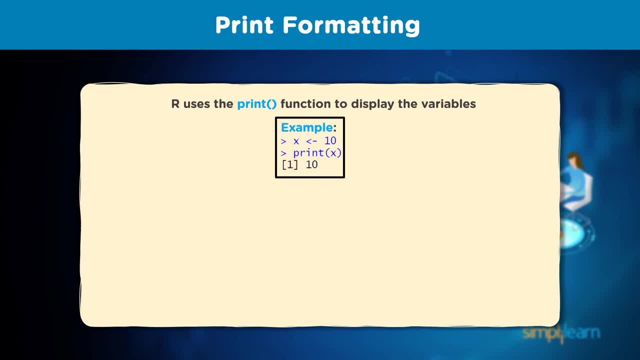 I have assigned number ten to X. i can do it print X and that will show me the value of x. what we see here, with one in square brackets, that also has a meaning, which basically means it is a vector, and we'll learn about vectors later. So R uses the paste and paste zero functions to format strings. 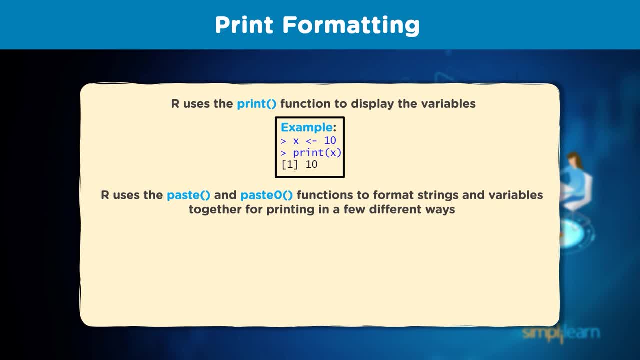 and variables together for printing in few different ways. For example, if I would do this, which I say is print paste, and then pass in two strings here or two words here, such as hello and world, that would be printed as follows: Now I could also do a print paste and then use a separator. 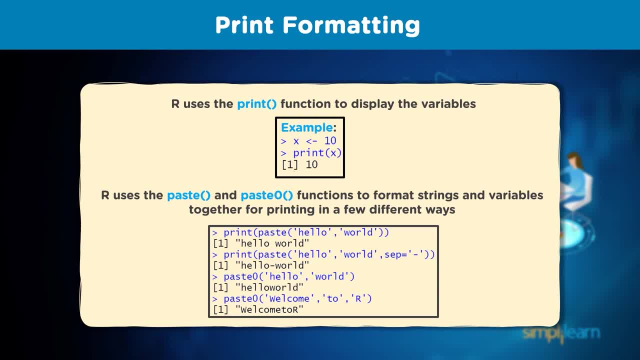 so my print would look something like this: If I use paste zero, then that avoids any space between these two words or, for example, these three words. So let's see some basic examples here when we talk about print. So, for example, if I bring up my R studio, here is an example. 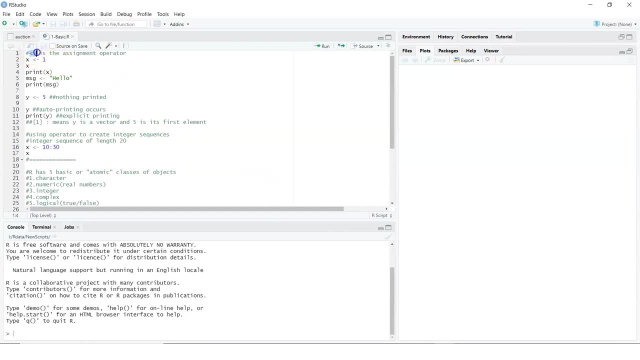 So X, as we say now. this is your assignment operator, which we already discussed. Now I can be assigning a value to this, So I can just place my cursor here and I can just hit on control enter. So value has been assigned. Now let's look at the value of X. Now I could also be doing a print X. 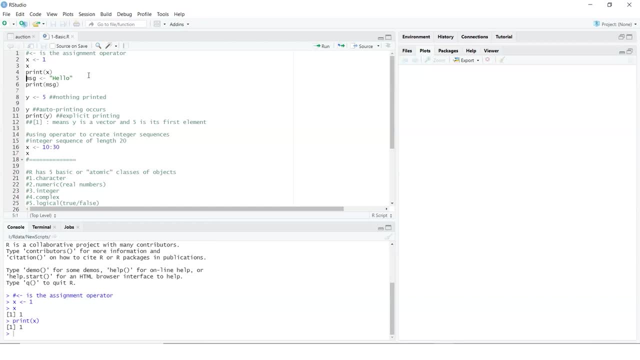 explicitly by using print function. For example, if I do similarly for messages hello, and then I can print the message by using print. Now if, for example, I do something like this, this is not going to print anything until I call the variable or I use a print function. So, for example: 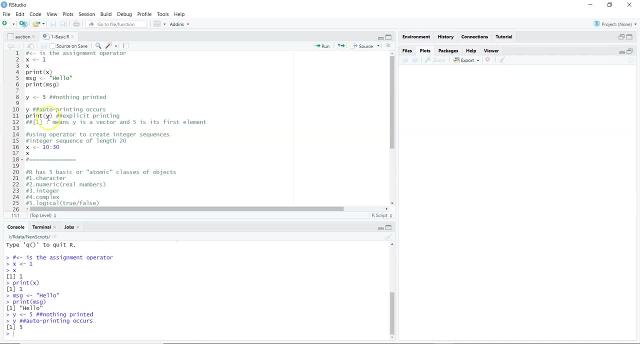 if I do a Y, we see auto printing shows us the value. or I could do explicitly by using the print function, by explicit printing. Now, whenever we look at this number one, as I mentioned, it means why is a vector and five is its first element. Now you can also use operator to create integer sequences, and we'll learn about. 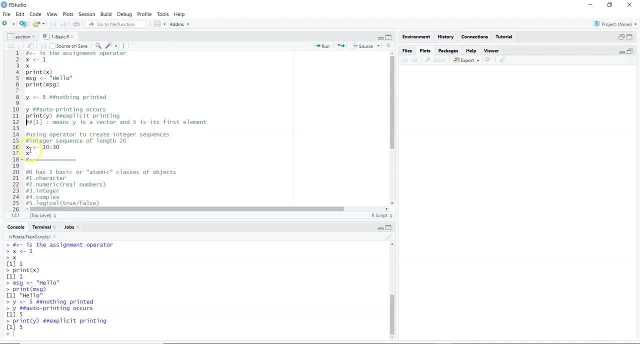 sequences or list later, But this is just a simple example. So I'm creating an integer sequence of length 20.. I can place my cursor here, which would start with 10.. 30. So let's look at this: values for our sequence of integers. Now, at any point of time you can 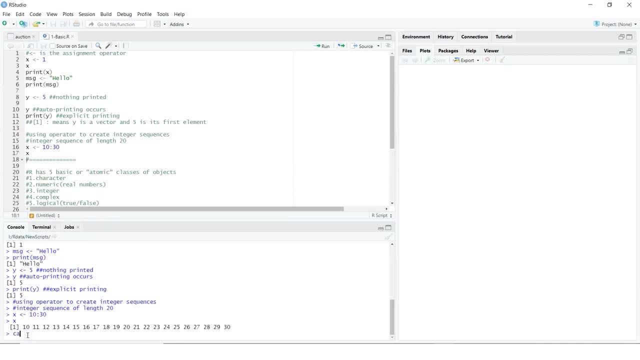 always use a class to look at the class of, say, x, and that shows me the classes of integers. Now, looking further, when we talk about different data types, as we learned few minutes before, So R has basically five basic or atomic classes of objects. So you have character numeric values. 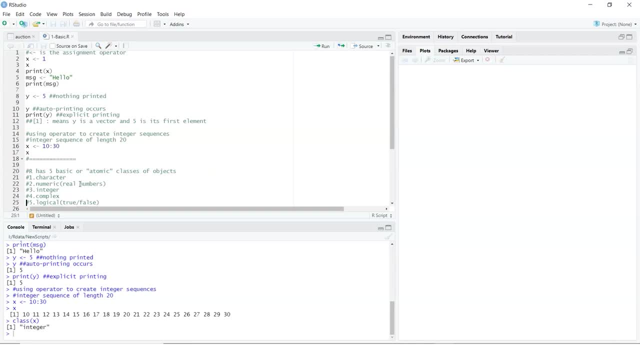 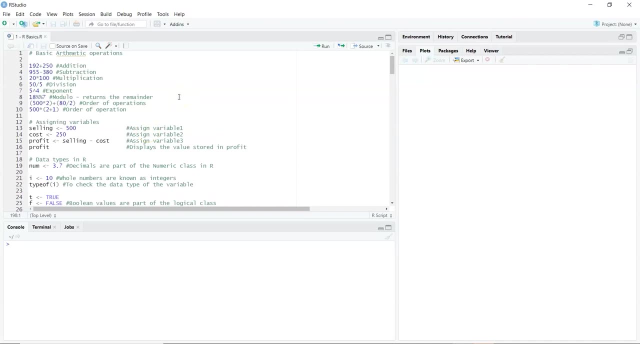 that is real numbers, you have integers, you have complex and you have logical values. Let's spend some time in understanding some basic arithmetic operations and how you can do it in using your R programming language. Now here I've opened up R studio and these are some basic. 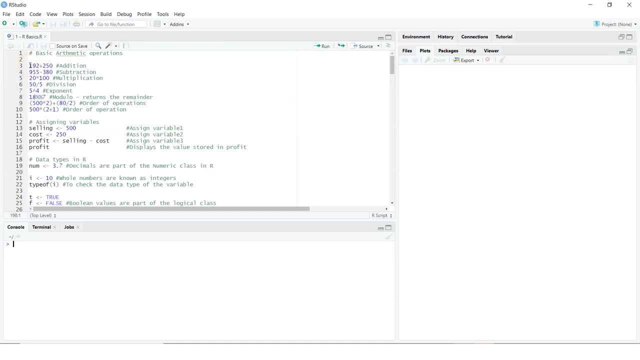 examples such as performing arithmetic operations. Now, for example, we can add two numbers and I can just place my cursor here and please press ctrl enter. That shows me the addition. I can do a subtraction, I can do multiplication, division, also going for exponential power, or use modulo. 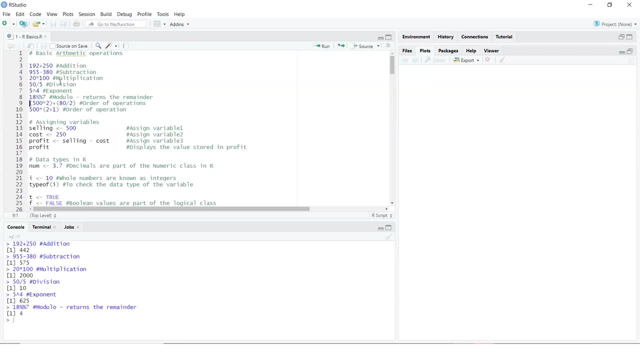 which is the number of integers. So I can do that, So I can do that, So I can do that, So it returns the remainder. Now, when we are performing operations, what we can also do is we can change the order of operations, and in this case we are using parenthesis, So I am putting 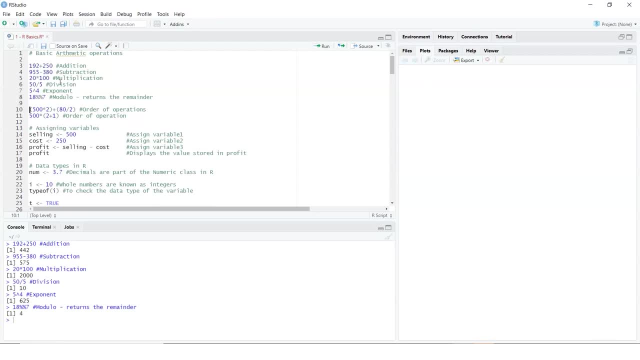 in 500 into 2 in a parenthesis, plus 80 divided by 2.. So first it operates what is given in parenthesis and that's why I get a result 1040.. Similarly I can change the order of operations, So here I can give 500 into and 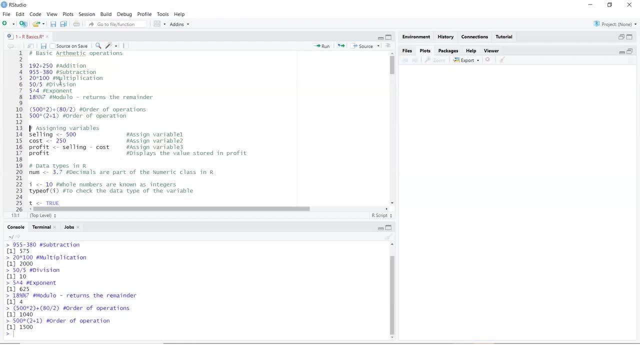 then something in the parenthesis, So that gets operated first, and hence you get result of 1500.. Now we have already discussed about the assignment operator, and what we can do here is we can assign variables some value. So for example, I create a variable called selling and then I would assign: 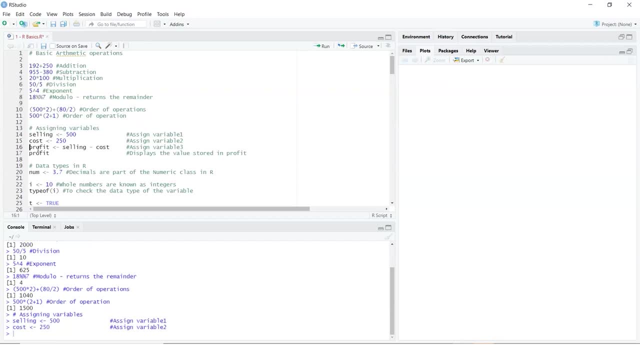 it a value, Similarly for cost, and then we can do some calculation So we can say profit is selling minus cost. So we can do some calculation So we can say profit is selling minus cost. So we can do that, and here I can look at the value of profit which shows me 250.. Now let's also spend some time. 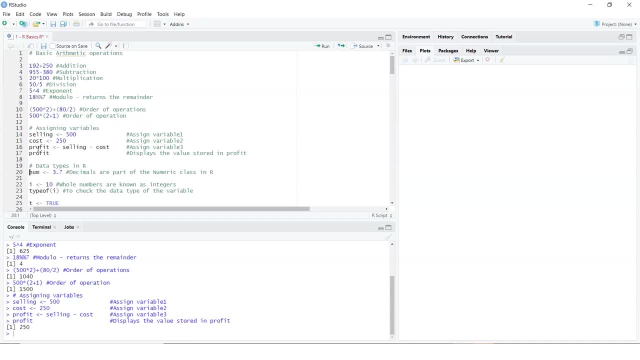 in understanding data types in R So we can have different types of data. So this one shows me an example of assigning a decimal value which is part of a numeric class. So I can do this. and then if I would be interested in seeing the value of num, So I can just look at the value of num. 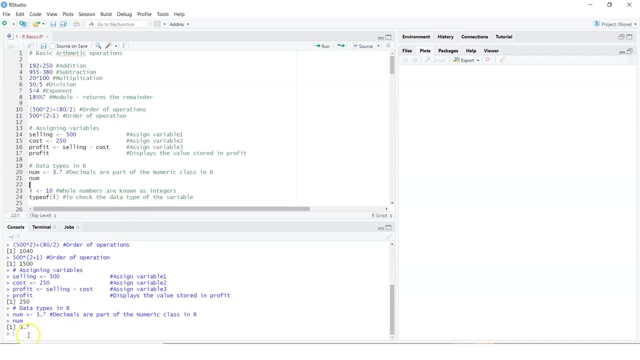 If I would be interested in looking at the type of num. So I can do that here by just typing in type of and then select this one and pass in your num and it shows me the value is double. I can also look at what class it belongs to, and that shows me it is numeric. So in this way you can not only 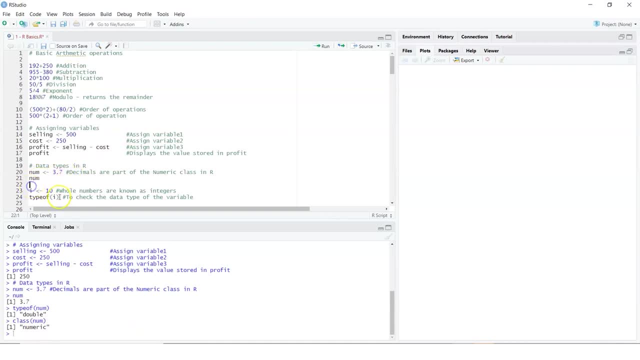 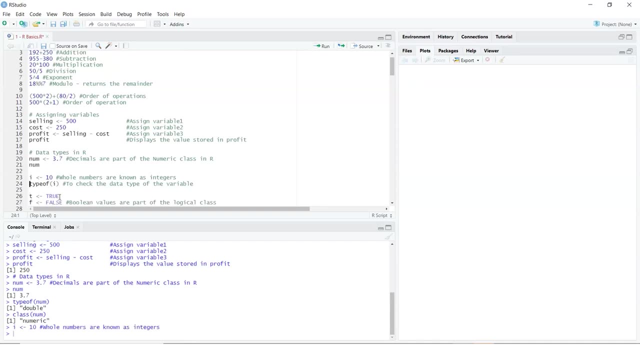 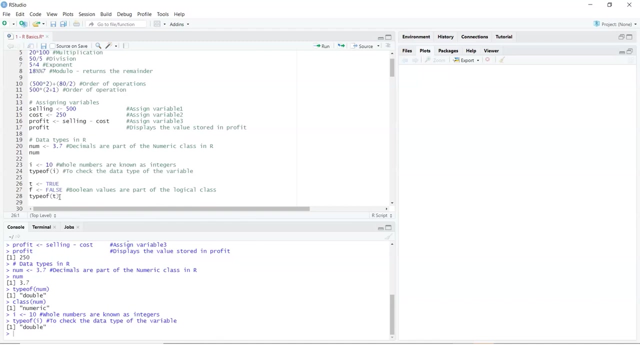 assign values to a variable, but you can look at the class and type of it. Now here we can assign whole numbers, which are also known as integers. Now if I look at the type of this, it shows me double. So if I would want to explicitly assign an integer, I could have done. for example, i: 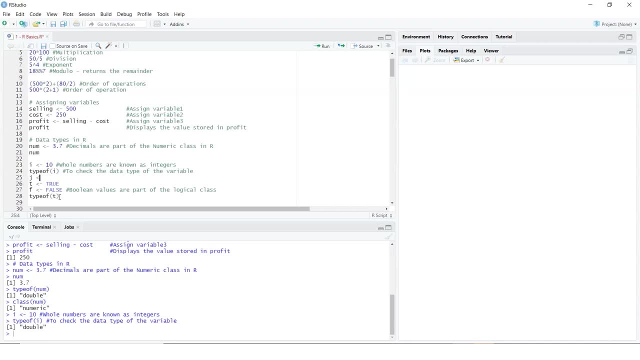 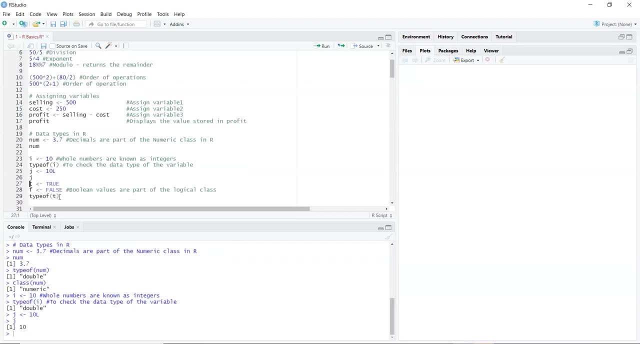 let's say j and I could have used the assignment operator and I could have done this. and then if I look at the value of j, it shows me the value, But what we would be interested in looking at the class of j, So we can do this, and it shows me it is an integer, So explicitly, either I can assign this. 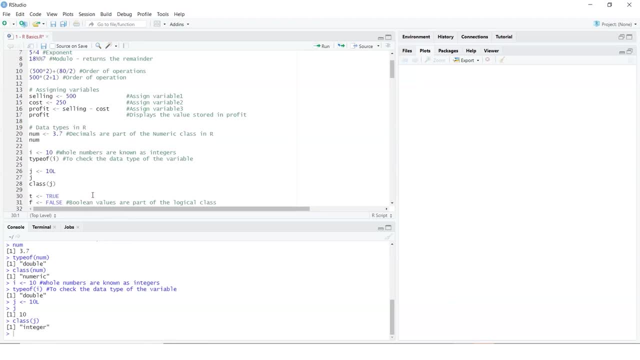 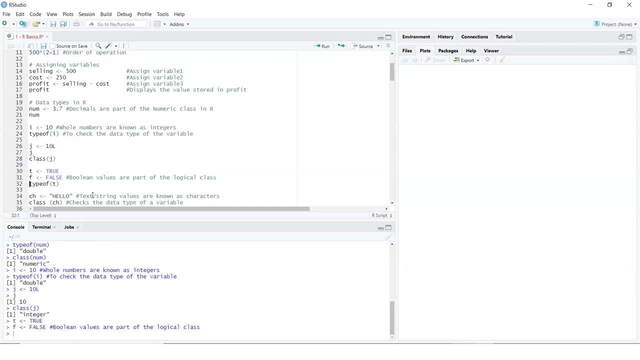 by using a capital L, or I could use a function called as dot integer. So we'll see that later. Now we can also assign boolean values, or basically your logicals. So here we assign true and then we do a false and we can look at the type of t and that tells me it is a logical class. Now, similarly, 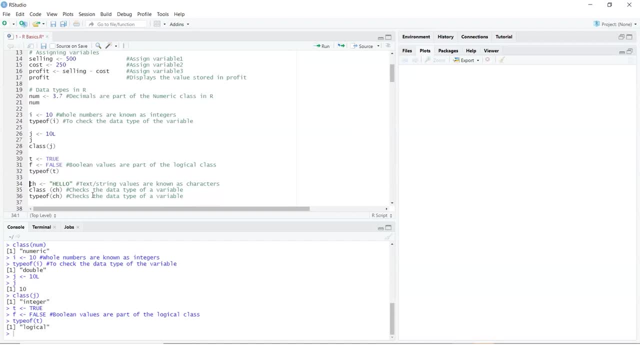 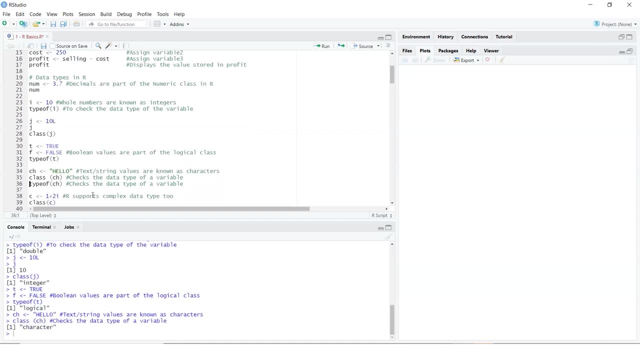 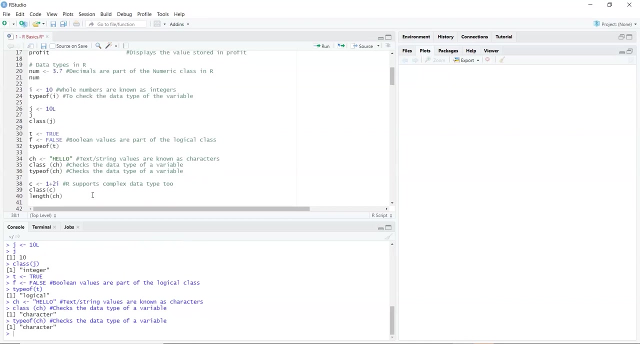 you might be interested in working on text or string values, and here we can do this by saying ch and then passing in a value. Look at the class of this: it tells me it is. the data type is character. and if you look at the type of it, it says me character. Similarly, R also supports. 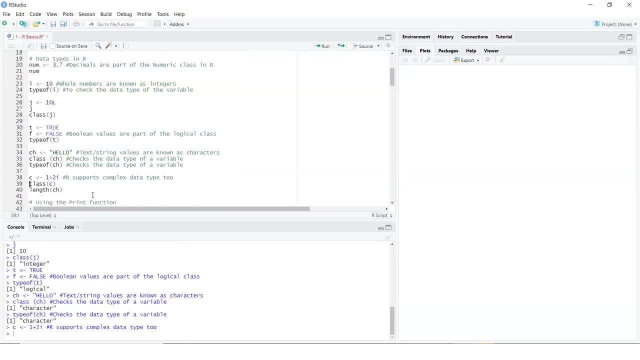 complex data types. so we can do that too, by just doing this and look at the class of it. It tells me it is complex, and you can also pull out different types of data. Now we can also assign the size of the data: not just the size of the data, but also the size of all the types of data. 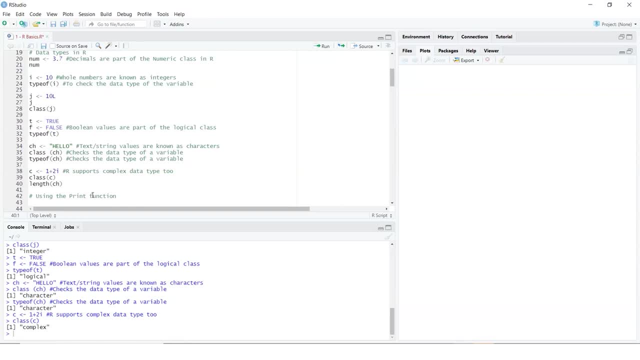 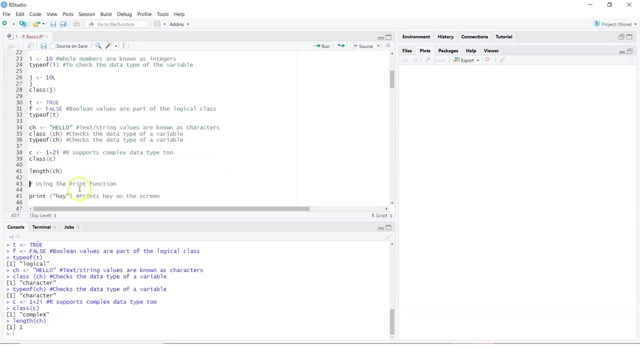 So you can see here the size of the data. Now, if I look at the class of the data now, I can see the the length of this by now. here we are doing a length on the character, So let's look at this one and it shows me what is the length of this. Now, one of the useful functions which we usually 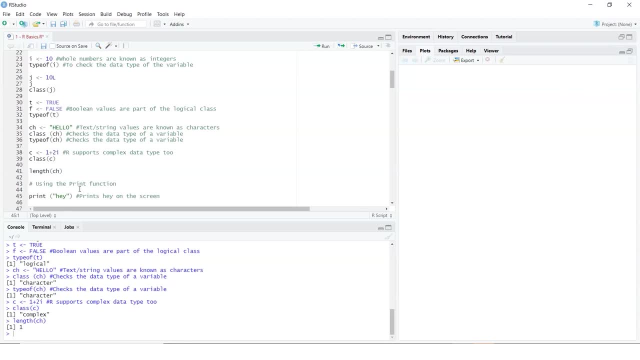 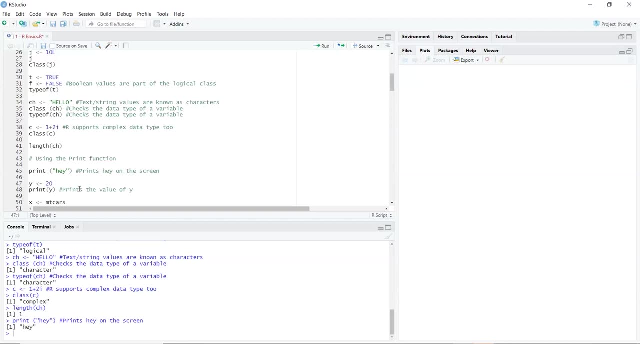 use in R is print. Now I can simply do a print, hey, and that prints whatever value is passed to print. I can assign a value to a variable and then print it, So that is also fine. You could have also without using function, just typed y and that also shows the value. However, sometimes 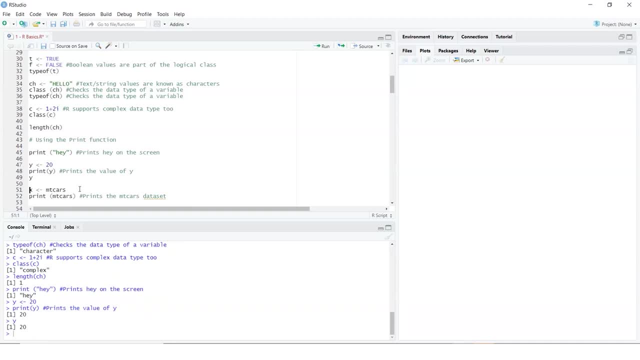 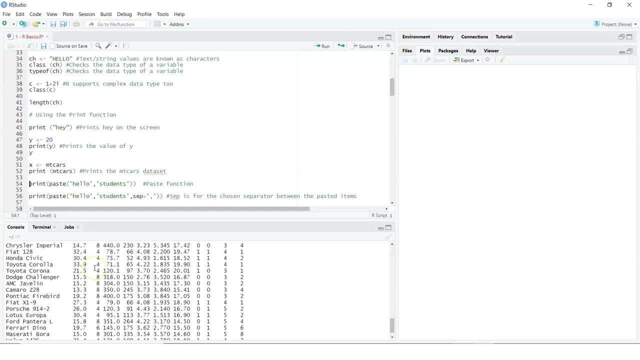 using print as an explicit function can be useful. It makes your code more readable. Now, here we would use an inbuilt data set that is empty cars, and then, if you would want to print the data set that shows me the values, which shows me the car models and different other features, such as mileage, cylinder, horsepower, 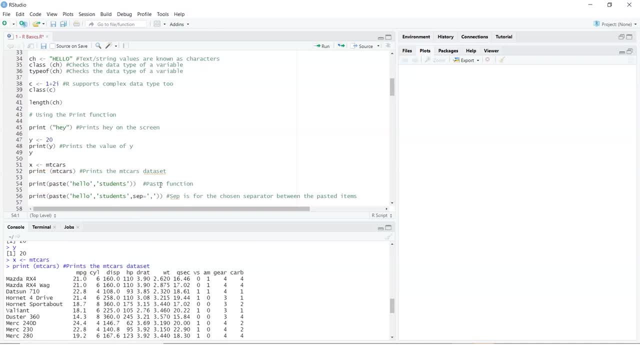 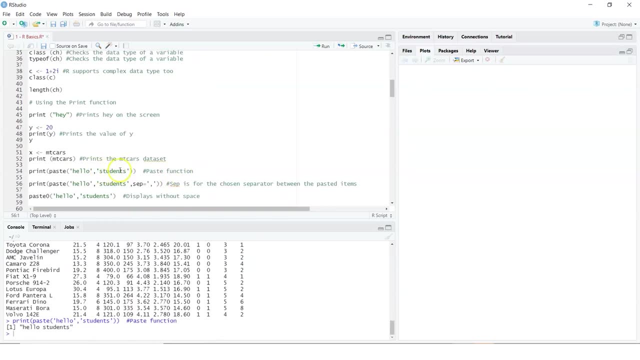 and so on. Now, one of the use case of print with a paste function can also be seen here. So I'm doing a print paste and that basically prints whatever was passed in a concatenated way. I could also do a print paste with a separator if I would want to format my data in a particular way. So 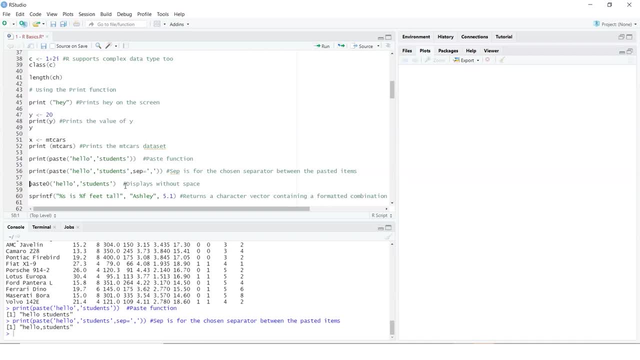 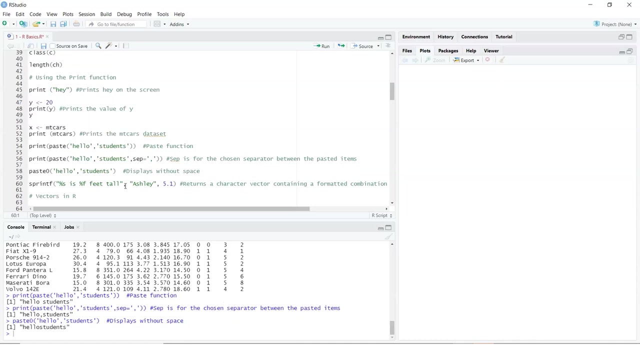 here I've used separator as comma. There is one more function, paste zero, which can be used. So I'm doing here paste zero and that tells me: just concatenate these values without any space. So paste zero shows no space between these two elements which were passed. Now we can explicitly do some printing, and for that I'm using a sprint. 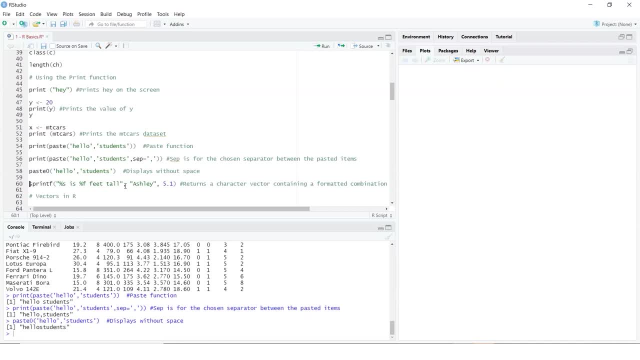 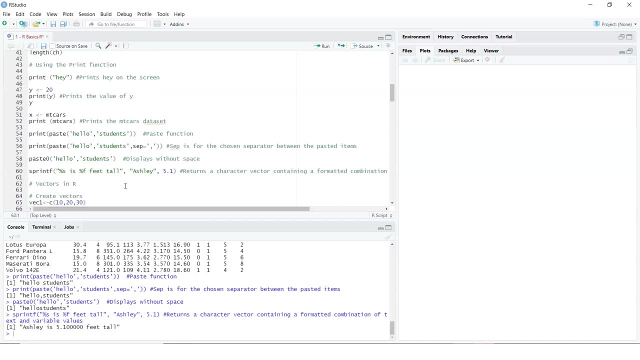 f option. I am going to pass in percentage s, which is for string, and percentage f for float, And we can print the values of this. So these are some basic operations or usage of your functions to basically do some computations or look at your results. 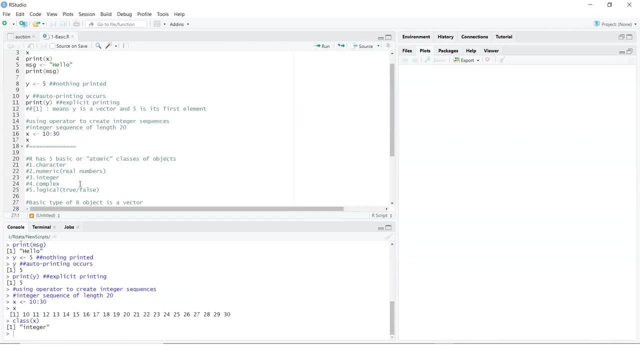 So when you talk about basic type of any R object, it is a vector And when we talk about vectors, empty vectors can be created with vector function. A vector can contain objects of certain size. A vector can contain objects of certain size. A vector can contain objects of certain size. 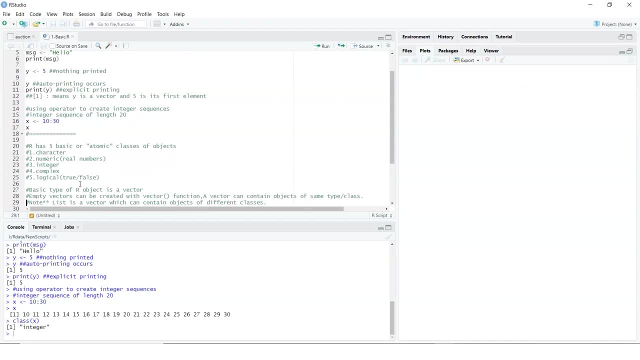 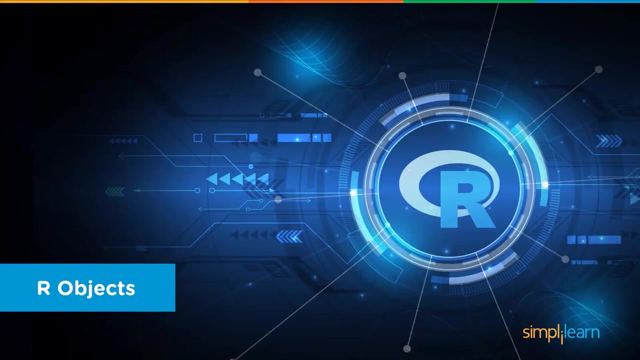 same type or a class. now, when we talk about list, list is a vector which contains objects of different classes. so these are some basic examples. so, apart from your print formatting, we can be looking at what we call as our objects, such as vectors or lists and so on. so when we 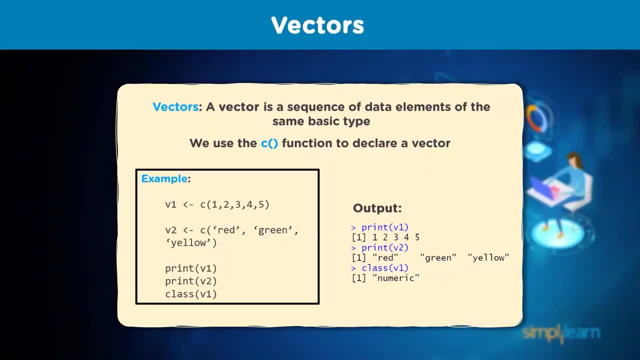 talk about vectors. it is a sequence of data elements of same basic type. we use the function to declare a vector, so we can always do a c function to declare a vector. for example, here we are creating a variable v1 and we are assigning it a vector by using c and then giving some basic 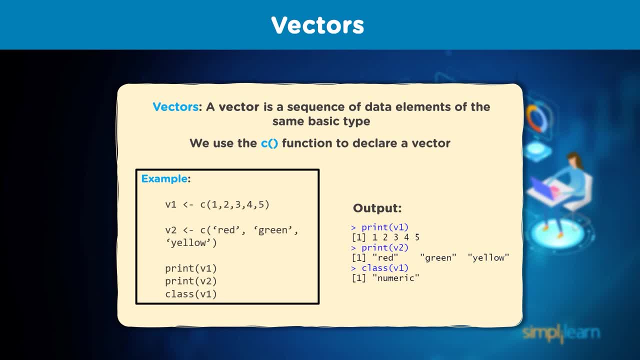 types, so numbers one to five or, for example, words. you can always do a print or a list so you can also use a class to find out what is the class of the elements or the values which have been passed to the particular object. so we can look at some examples like this. for example, we 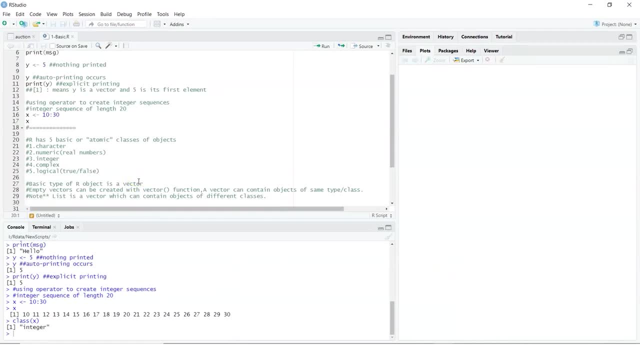 can see here. so list is a vector which contains objects of different classes, so you can have numeric objects, so that is, your numbers, such as one, two, three, four, five, six, seven, eight, nine, ten and so on, which are your numeric values? for example, here what we are doing is we are assigning a 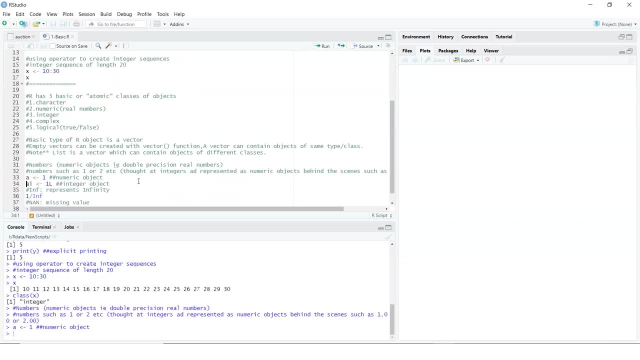 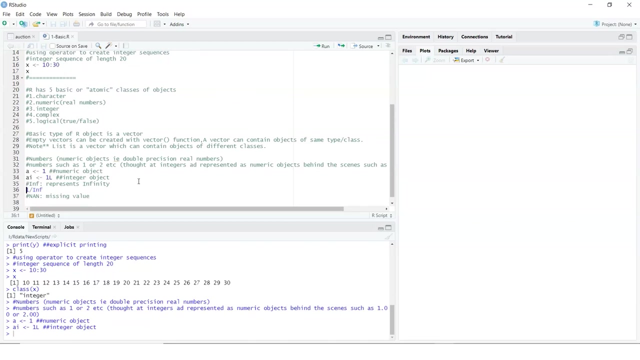 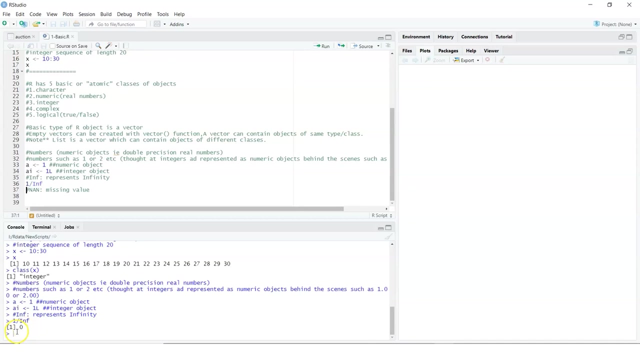 value one to a and that can then be used. i can either do a print or i can just use auto printing. i can also do here a value for a. i or i could be doing something like this- which shows me zero, which can be for missing value. so if i would want to use auto printing, i can just call a and it shows me the. 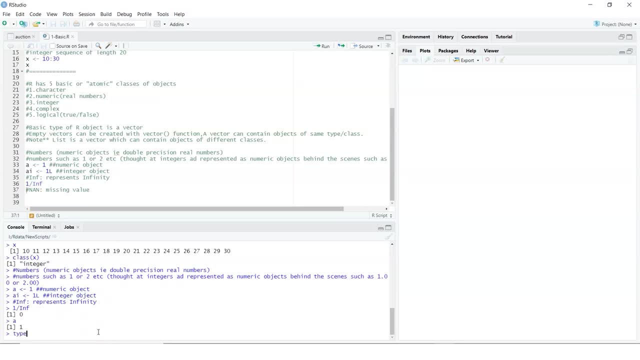 value, what has been assigned to it. you can always use a type of to look at the value of a, which is double by default, and if i look at type of a, i, that is basically an integer, because we used l here. so in this way we can continue working with, say, our different classes. 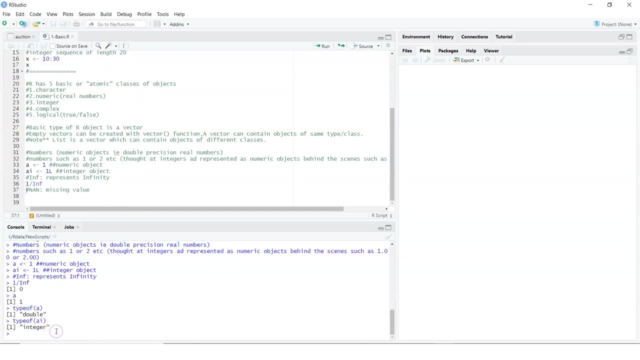 of objects. so, for example, let's create a vector here so i can say v1 and then basically assign it by using a c function and then pass in the values to this one and that basically gives me a variable and you can look at what are the values assigned to it. now, if i look at the class of v1, that shows: 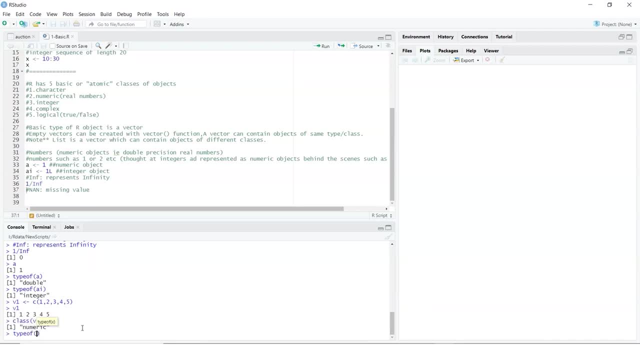 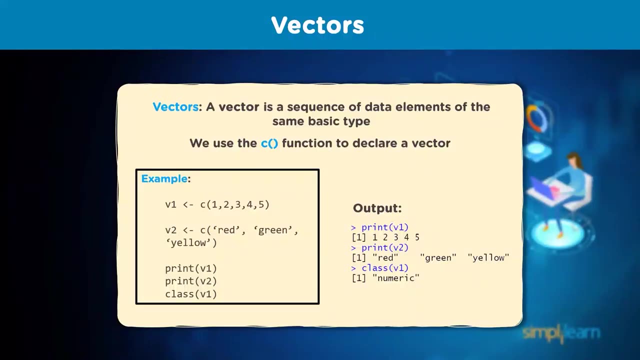 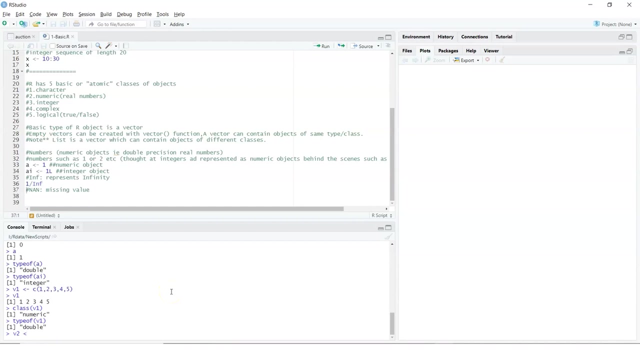 me it is numeric. if you use type of and then you would want to see the values of v1. that shows me the values are double. now, as we were seeing here, we can be looking at the class. so, for example, if i create one more variable and then assign values to it using c, so passing in some words here- 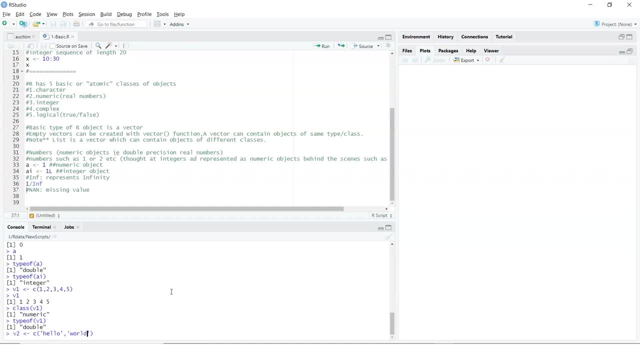 for example, let's go and say hello world, and then i can basically do this and look at the values of this one. i could also explicitly print, as we discussed earlier, by doing a print v2. we could also be having a paste function if we would want to use that. 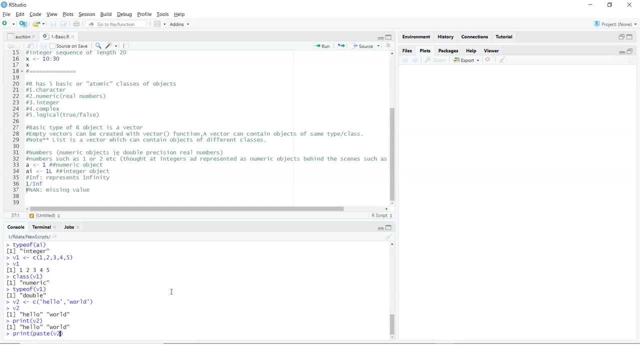 so, for example, if i would do a paste function, i could be using- and this is missing a bracket, so let's complete this- and that shows me the values of this one- and you. i could have also used, for example, paste 0 function, and that also works fine. 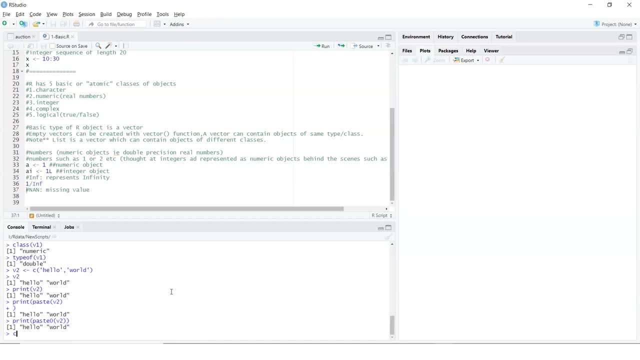 so it depends on what we are looking at here. so if i look at class of v1 which we had, it is numeric and v2 is basically having elements which are of the class character. so this is just a simple example of having your print functions having vectors created, printing out the values of those 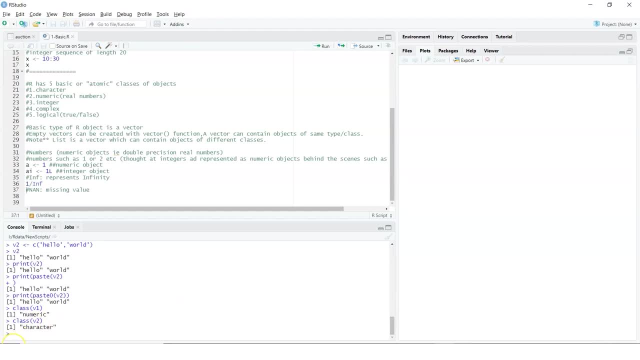 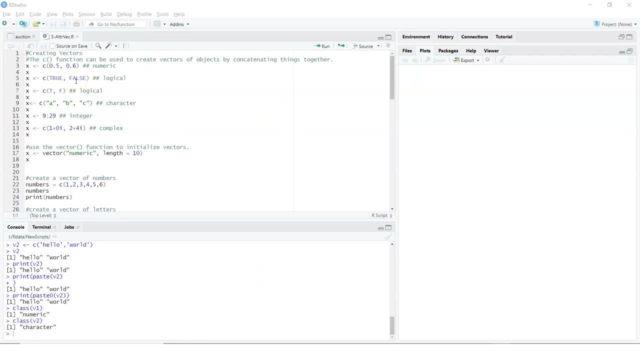 printing out class and type of these. to continue our learning on vectors, as i mentioned earlier, we can use the c function, which can be used to create vectors of objects by concatenating things together. so, for example, if we look at this one which says x, and then i use c function and i say 0.5 and 0.6, so we can have a vector of. 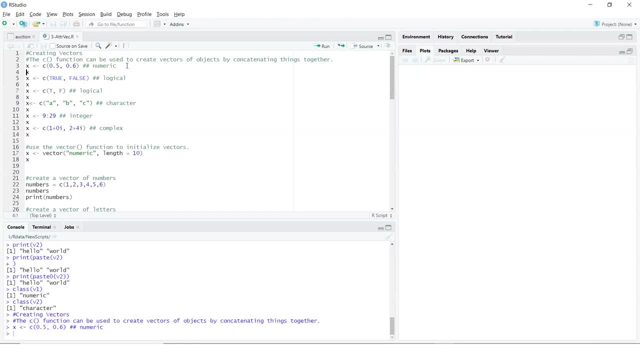 numeric types. so let's do this, and then we can look at the value of x, so it shows me my vector, which has 0.5 and 0.06. i can also have my vector of logical values, and now let's look at the value. 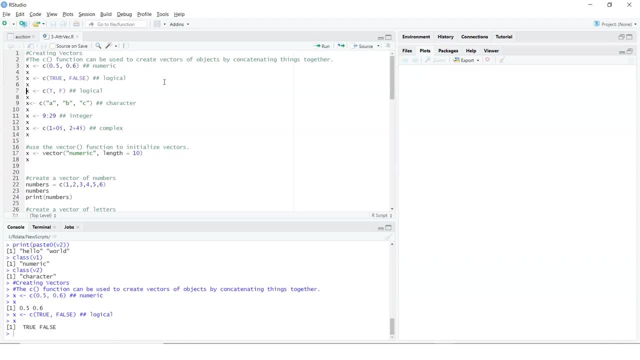 of x, so it has true and false. or we could have done it in this way where we can then look at the values. so we can use the short form: by using capital t and f, I can create a vector with character types and then look at the values of those. I can also be creating a sequence of 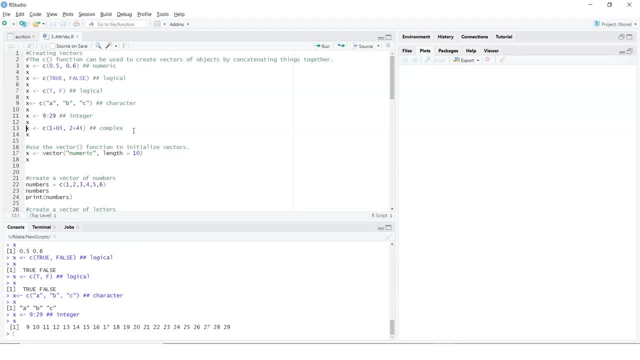 integers, as we saw in previous example, and then look at the values, which start at 9 and end at 29.. Now you can also create with complex types and look at the values. so these are some simple examples of creating vectors. Now we can also use vector function to initialize vectors. so for 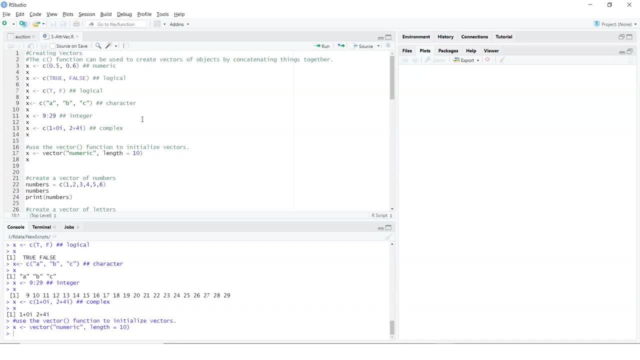 example, if I would do this, where I am saying my vector will be of type numeric length is 10, and then look at the values. so it just shows me a vector which has all zeros and the length is 10 and the length is 10.. Now you can create a vector of numbers by doing this, as we saw in previous. 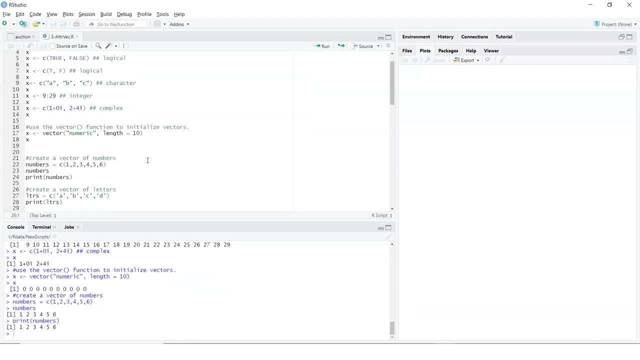 example, and use explicit printing to look at the values- or might be a letters- and then use a print statement to print function to basically look at the values of the vector. Now we can also try concatenating the above two so that creates a mixed vector which has two different kind of. 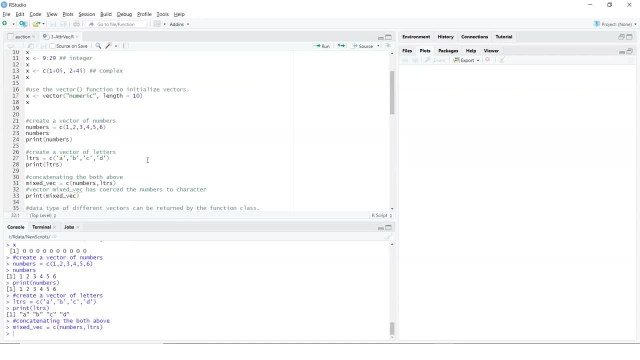 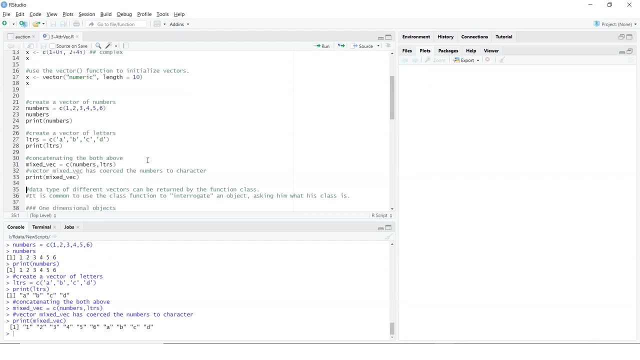 types here. So I can do a mixed vector by using the c function and then passing in my numbers, which has numeric types, and letters, which has character types, and then we can basically do a printing of this which shows me the value. but here what we see is coercion. 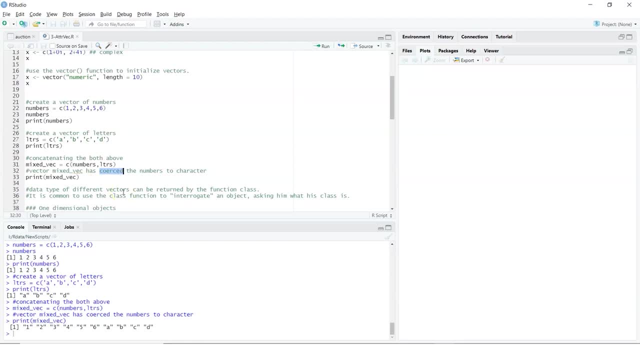 That is basically casting, if you would know, as the word in different programming languages. So it basically coerces the numbers to character, as characters cannot be coerced into numbers, And then you can print the values of this mixed vector, where everything is of character types. 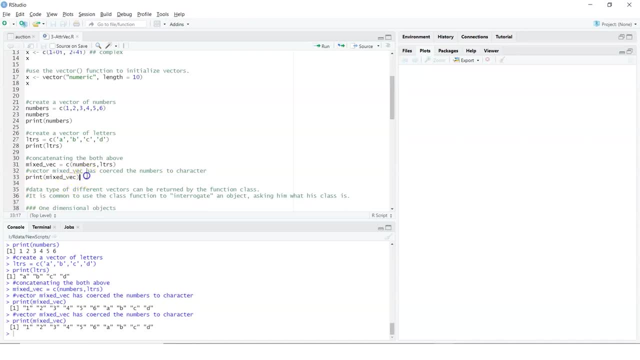 So, for example, at this point of time, if I would have done something like class of mixed vector and if I would want to look into the values of this one, it shows me everything is of character types here. Now, data type of different vectors can be returned by the function class as. 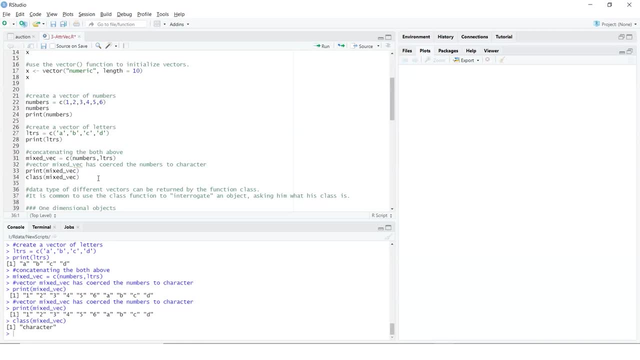 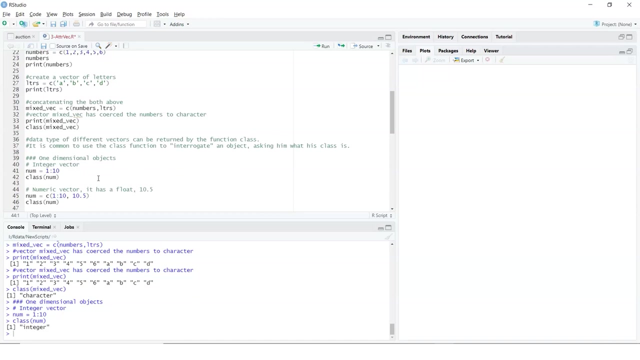 we saw just now. So it is common to use the class function to integrate an object. asking what is a class? Now create one-dimensional objects, such as an integer vector, which we have done earlier, and then look at the class of it which tells me it is an integer. I can. 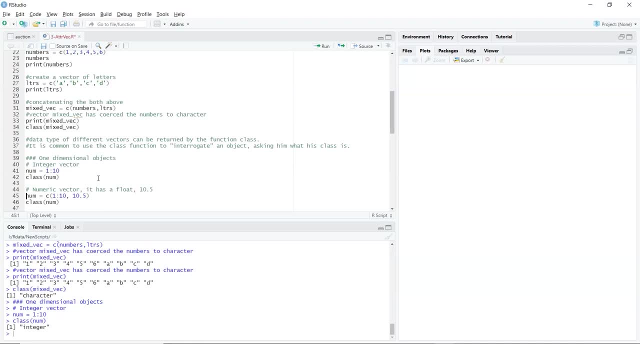 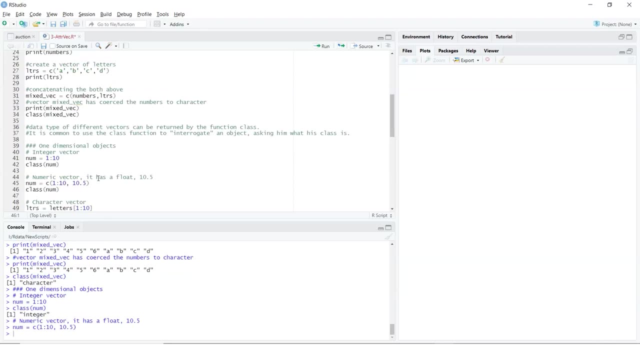 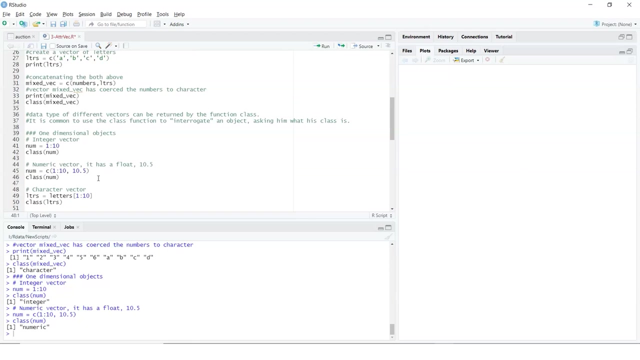 also create a numeric vector by giving in some values here. so when we do this- so I have given the vector, function C and then giving in the value and look at the class it shows me, it would have numeric values. now you can create a character vector and then basically look at the values of it. now at any 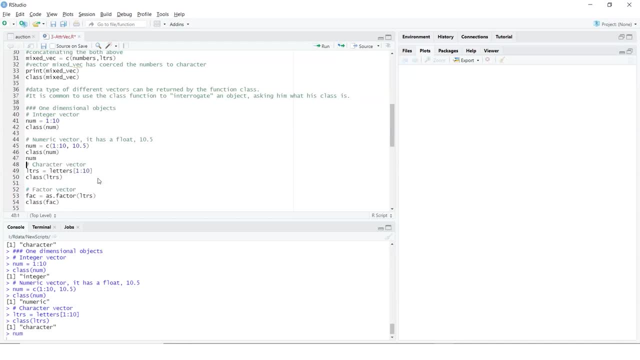 point of time in all of these. for example, if I would do num, I can see what are the values assigned to it. I can do letters and I can see the values of this. so let me just create some space here. now I can create a factor vector. 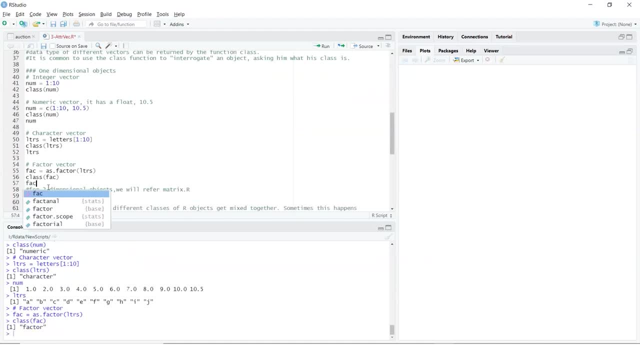 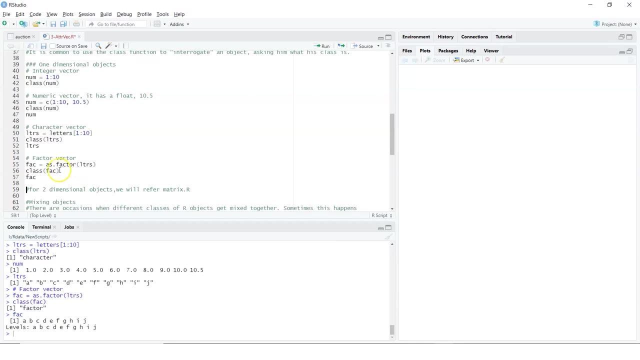 and then look at the values of it. or also you can see what is the value in this factor vector. so here we said: as dot factor, so factor function is being used here and we are creating a vector of letters. and then we look at the class. we also look at the values. what are assigned to this or what are in this? 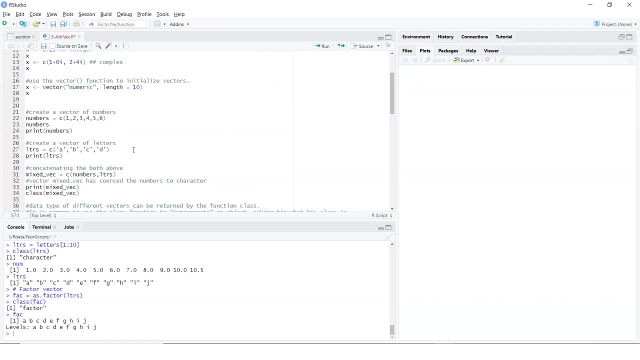 particular vector. so if you look into all of these vector examples, initially we were assignment operator, where we were using the C function, and when we started creating vectors by, say, concatenating or vectors of particular types, we are using equals here and that also is fine. Now, looking further, when we look at concatenating two different kind of vectors, 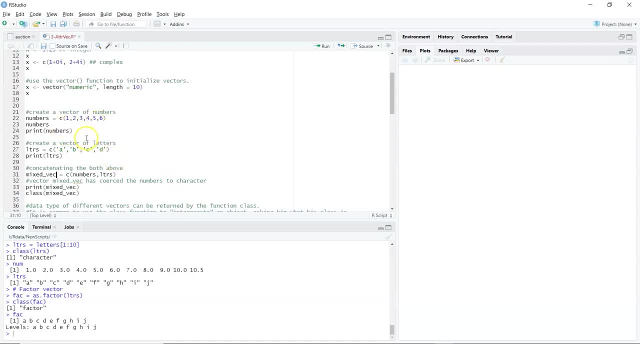 so, for example, here we have say numbers and letters, as we discussed earlier, it will do coercion, that is, change one type into other. Now when we talk about one-dimensional objects, we can have integer vectors or say float, which we saw just now ending at 10.5. so when we say C, 1 is to 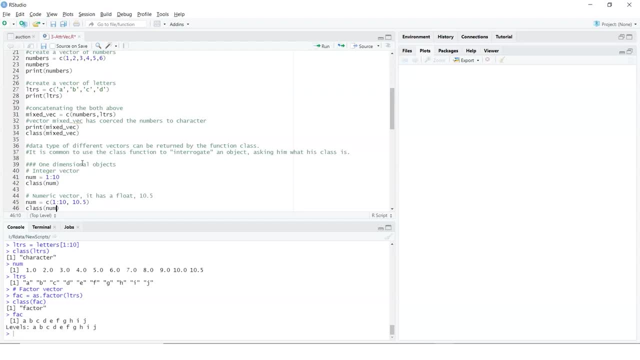 10.. It basically starts with 1, but then there is also, you can say, a coercion happening here and then you have the values ending at 10.5. that is float and I can look at the class of it. and when we did a class of, did we do a class? yeah, so let's come here and let's do a class. 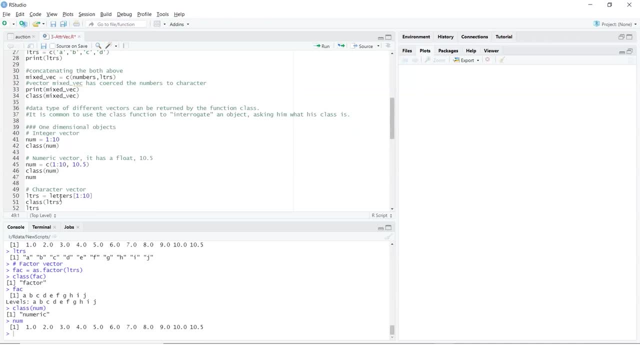 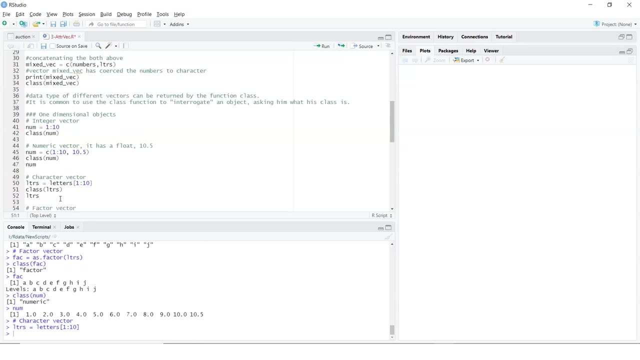 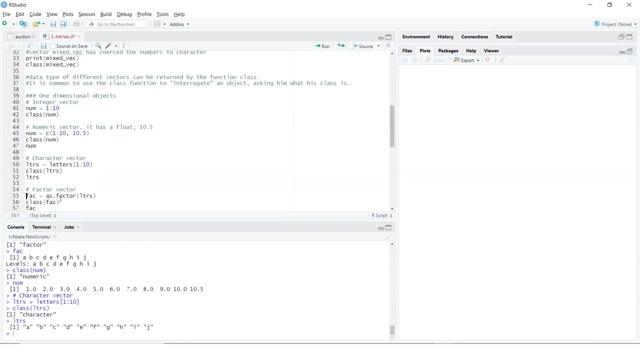 of this one. it says me it is numeric. you can look at the values of it. similarly, you can create a character vector which is 1 to 10 and then basically look at the class of it, or basically the value of this vector, or, as we did, the factor vector. Now for two-dimensionals, we will explore. 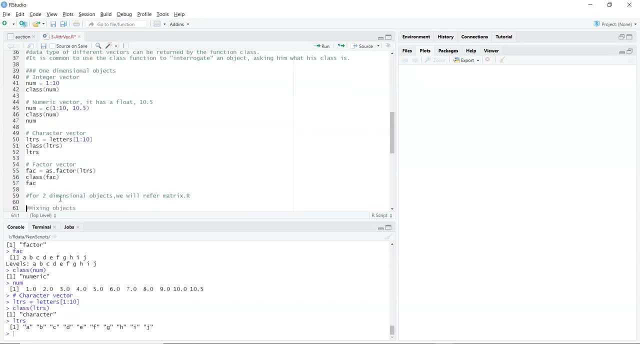 that when we are learning about matrix. so, as of now, let's forget that. Now, when you talk about mixing objects, there are occasions when classes of our objects get mixed together, so that could be accidentally, or that could be by accident, or that could be by accident, or that could be by. 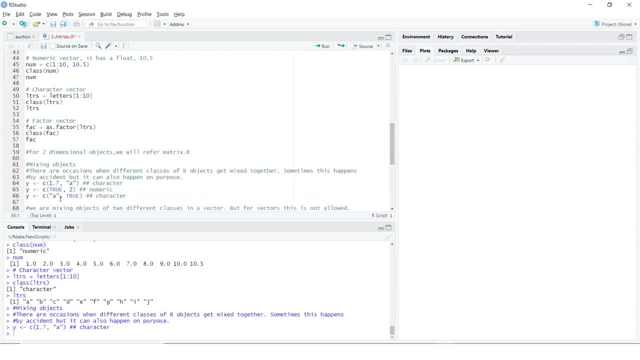 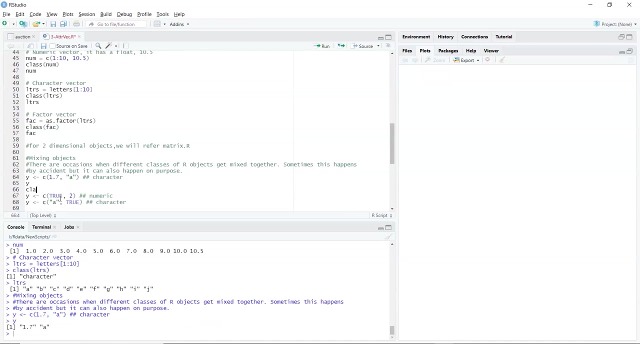 intentional. So if you look at this example, here we have Y, which has been given values, which is 1.7 and A, and at this stage, if I would look at the value of Y, that's my vector. if you look at the class of Y, that shows me it is as character Now when you look at some other examples. so let's. 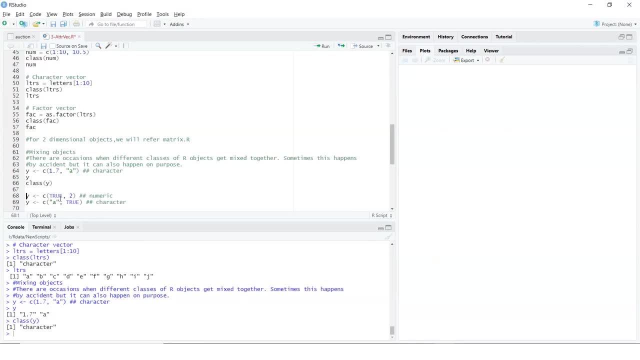 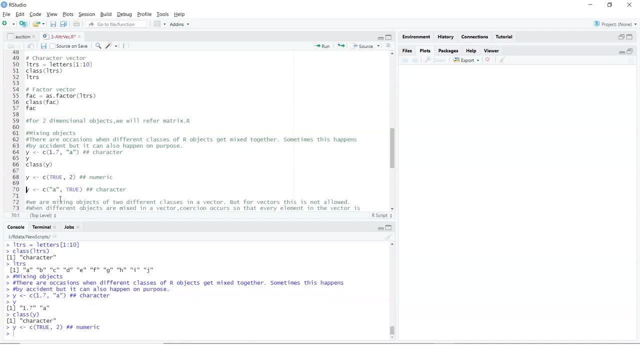 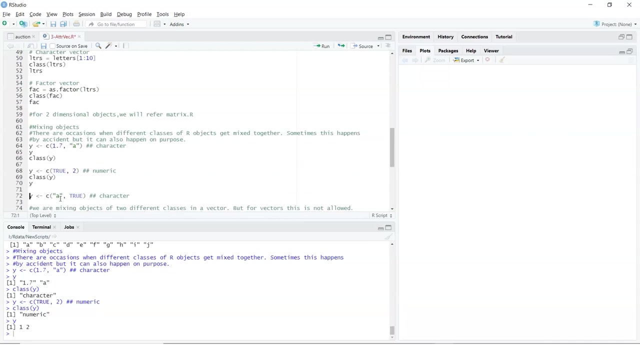 pass in logical And numeric values. What would happen in this case? so we can again use class of Y and that basically has numeric, and if you would want to look at the value of Y, that shows me 1 and 2. here Let's go. 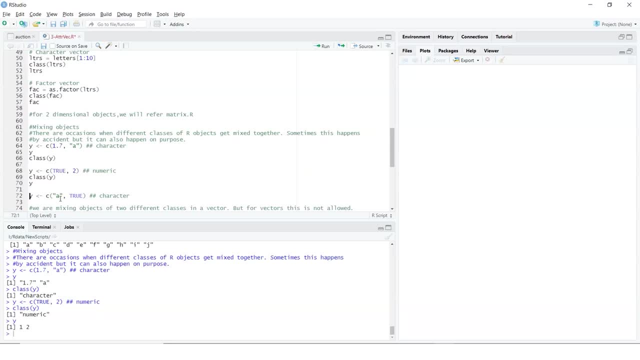 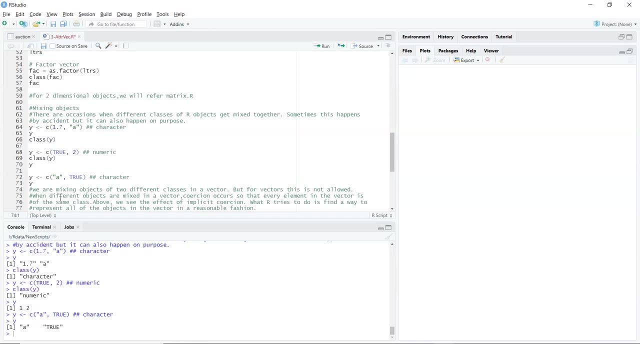 further. so let's look at the value of this one, so Y, and then basically see what is the value of Y. so it is A true, and you can also look at the class of it. Now we are mixing objects of two different classes in a vector. Remember, when we talk about vector, we always talk 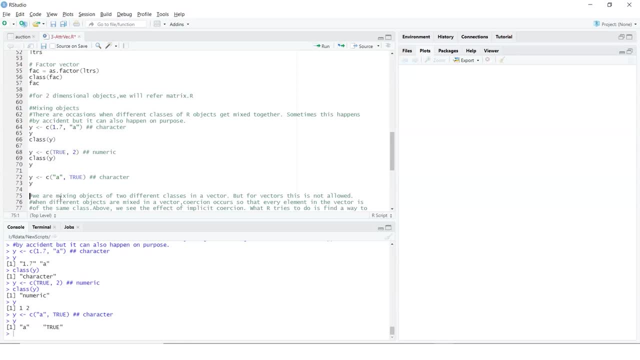 about vector having elements of same type. But when we talk about lists, which we will learn later, that would have, basically, or that can have each element of different type. So for vectors it is not allowed. So when different objects are mixed in a vector, coercion occurs so that every element in the vector is of the same class. Now we have seen earlier. 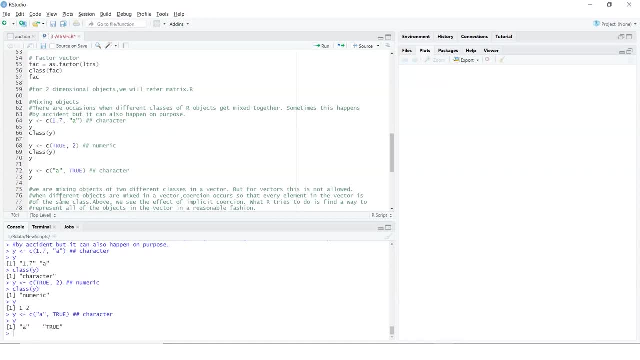 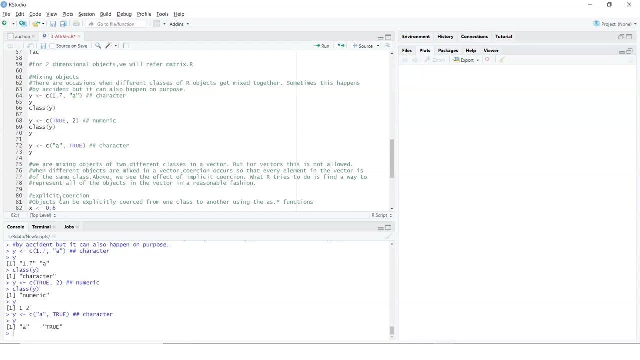 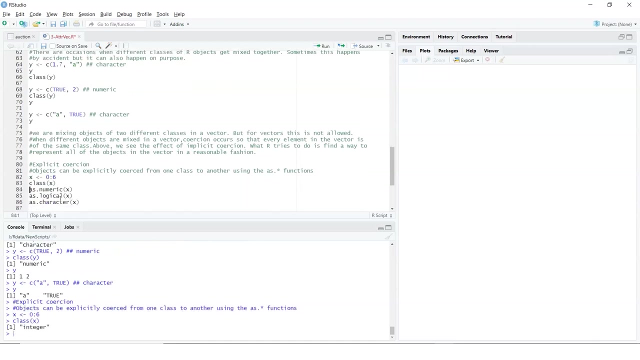 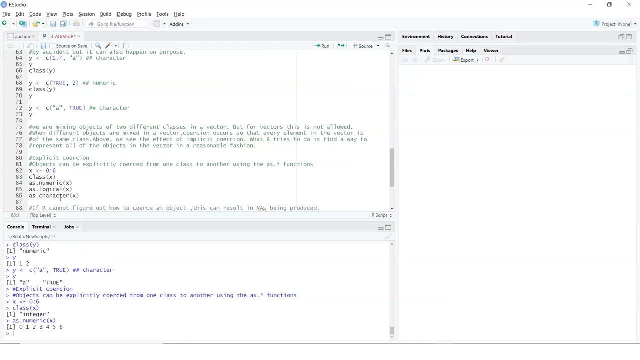 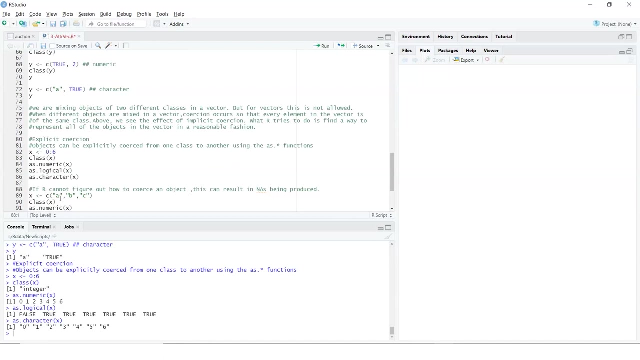 the implicit coercion where R tries to find a way to represent all the objects or elements, as I say, So all the objects in the vector in a reasonable order. So we can also be doing explicit coercion, so that is, from one class to another, by using a as dot and then using a relevant function. so if I have X here now, if I look at the class of X it tells me it is an integer. but I can convert that to numeric by doing a as dot numeric or as dot logical or as dot character, to basically do a coercion and change the class of the object. 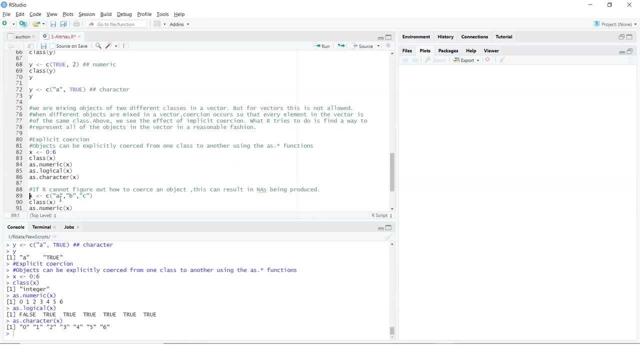 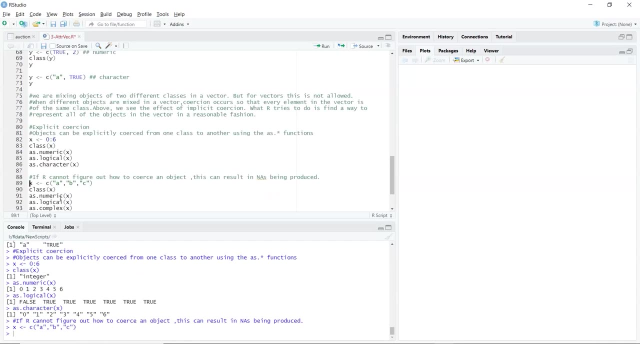 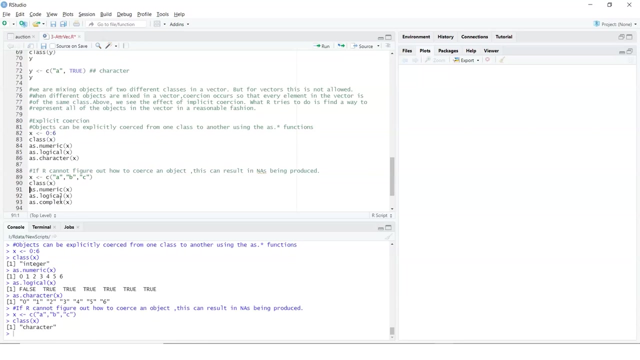 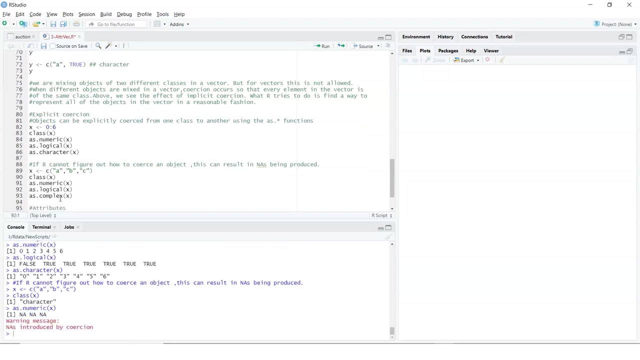 Now, if R cannot figure out how to coerce an object, this will result in NAs being produced, which we can also relate to missing values or not applicable values. So, for example, if we create X and look at the class of X, it tells me it is character. Let's try changing character to numeric, which will not work, and it says NAs are introduced. 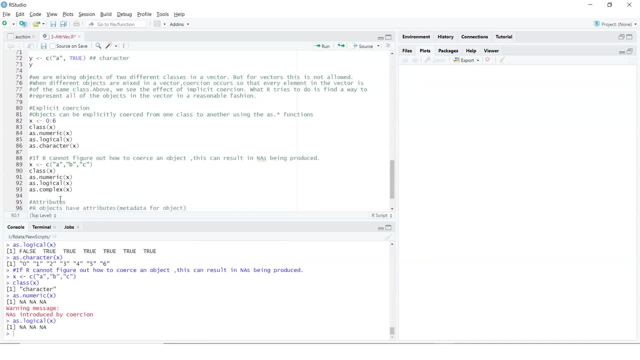 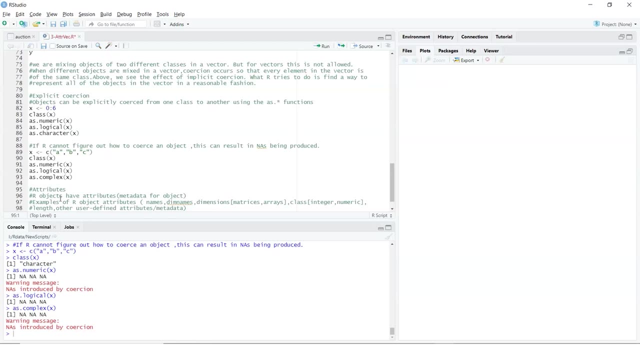 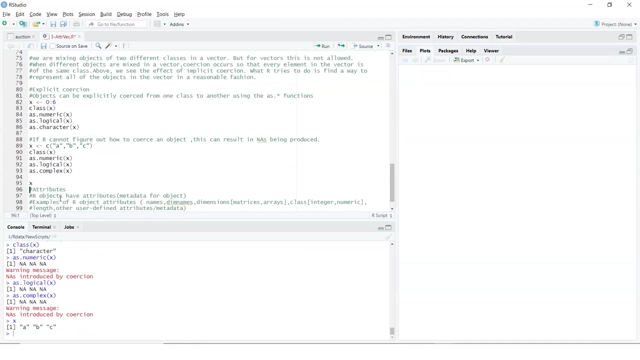 If you do it- even in logical that would not work- It shows me any values. or if you do a complex, it says values have been introduced. So at this point of time, if I look at the value of X, it tells me it was assigned ABC and we try to convert that into a different class. 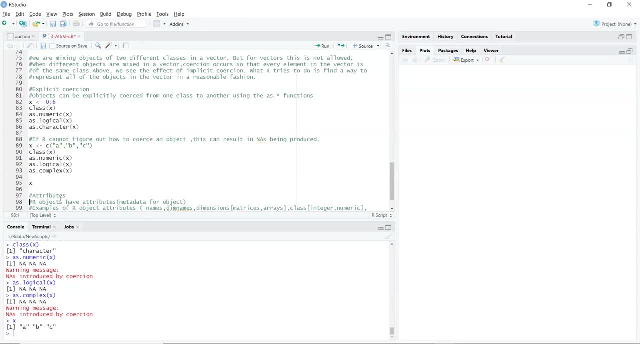 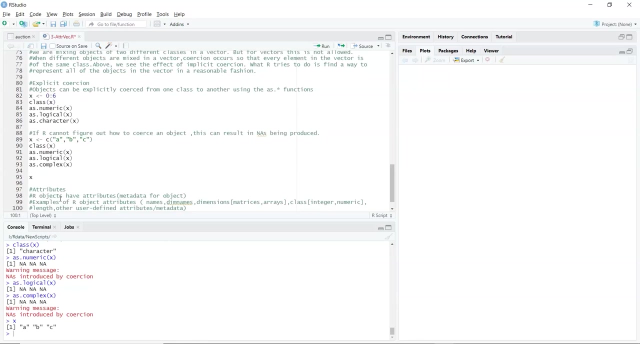 Now, when we talk about vectors, it is also good to know about attributes. in brief, So all your R objects have attributes. that is metadata for object. So when you talk about R object attributes, you could have names. you can have dimension names. you can have the dimensions, that is, matrices and arrays. 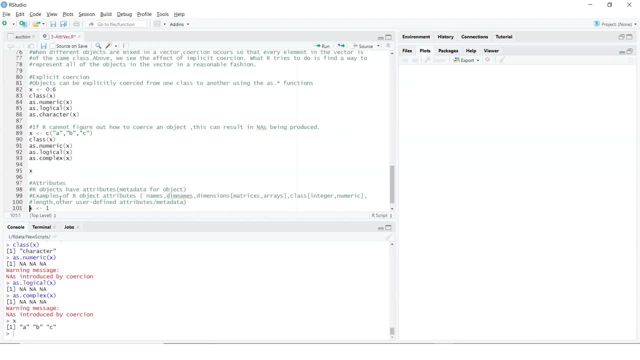 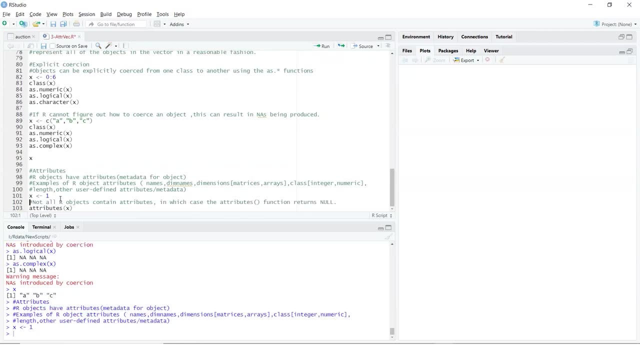 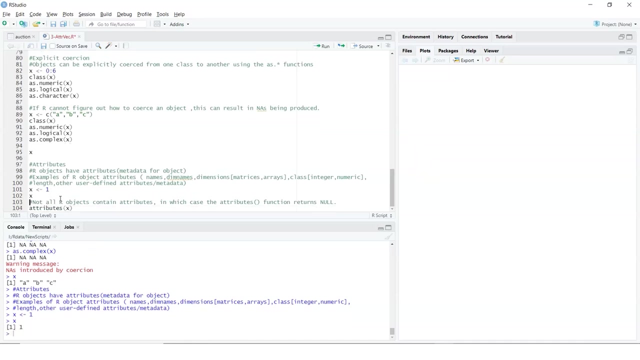 You can look at the classes such as integer, numeric and so on, and you can also look at length, which is user defined attributes. So if I say X, we are assigning a value to X. Now, at this point of time, if I see, my value to X is one, but then all objects need not be assigned. 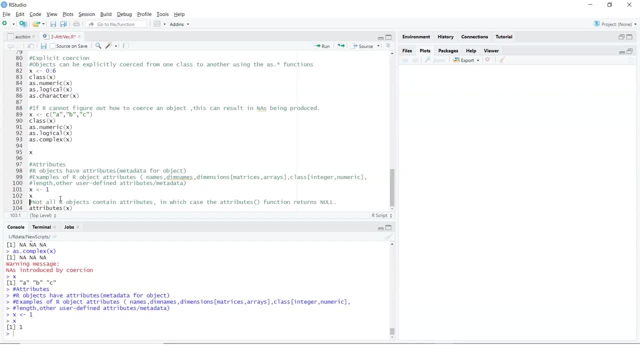 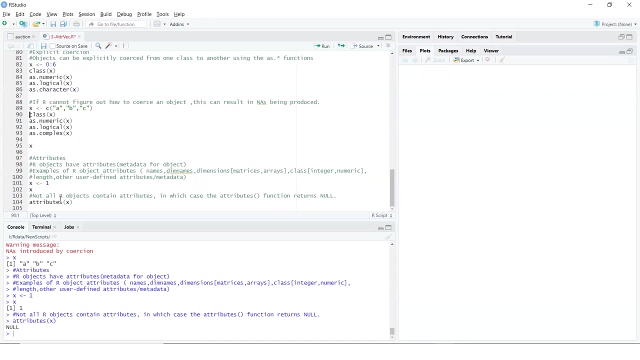 necessarily have attributes. So in that case, whenever you try to use an attributes function, that would return null. So at this point of time, if I look at the attributes of x, it shows me null value. So these are some of the basics which help us in working with R and using your vector. 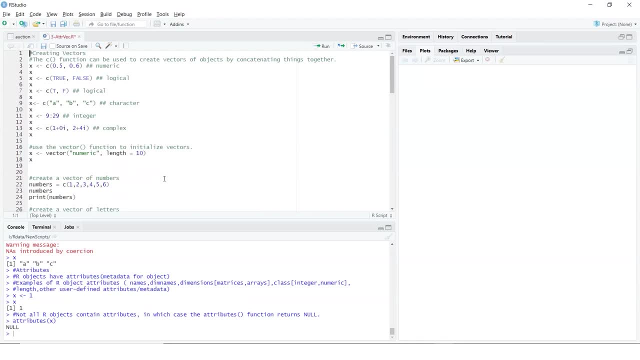 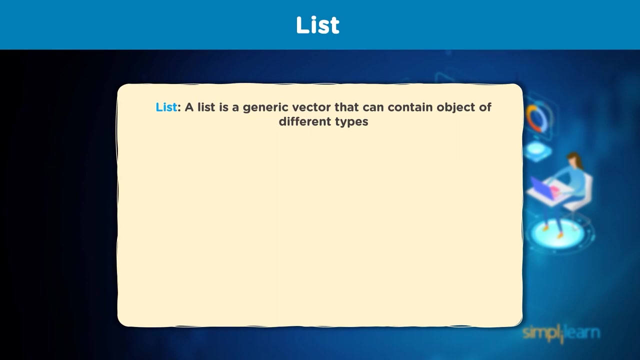 function or looking at the coercion which is implicitly happening or explicitly, can be done by us by using a as dot sum function. Now let's learn about lists and how we can work using R on list. When we talk about vector, which we saw in previous examples, vector is a one-dimensional 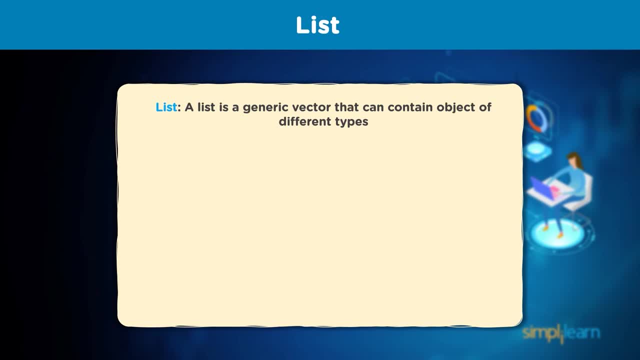 array right and it can hold elements only of same type. So we would say vector is more of one-dimensional. But when you talk about list, list is a generic vector that can contain objects of different types. So when you talk about, say, for example, matrices, matrices can also hold elements of. 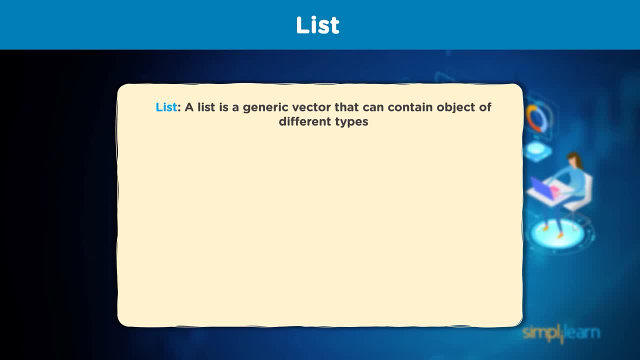 same type, but in matrices it is a two-dimensional array. We will talk about matrices also, we will learn. So when you talk about lists, they can contain all kind of R objects. So you can have dates, you can have data frames, you can have vectors. 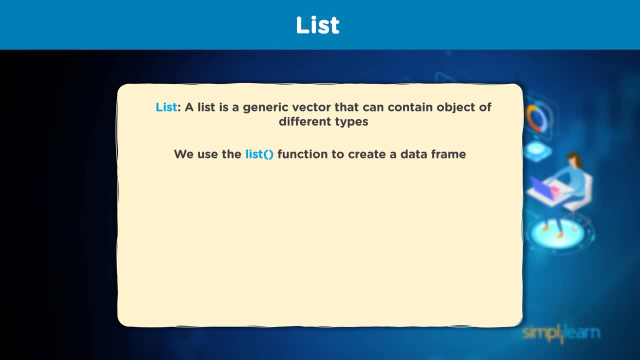 And many more. So. in list there is no coercion, which is required, that is, changing of data type. There is no loss of functionality and lists do not follow any predefined structure. Now we can create lists using this list function as it is shown here, So you can create a variable and then 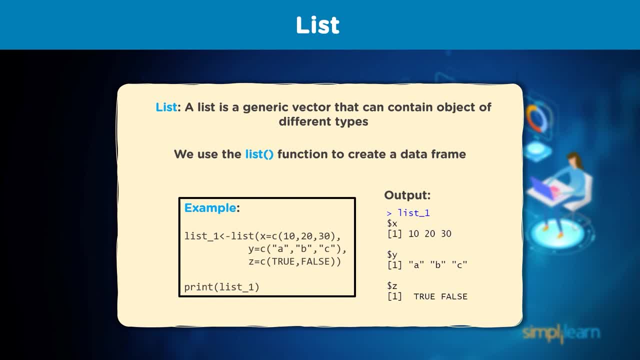 assign a list to it where you can be using either passing in a vector, or what you can do is you can simply create a list by using this list function. So let's see some examples here. Now for that, what we can do is I can bring up my R studio where we can see an example on list and how it works. 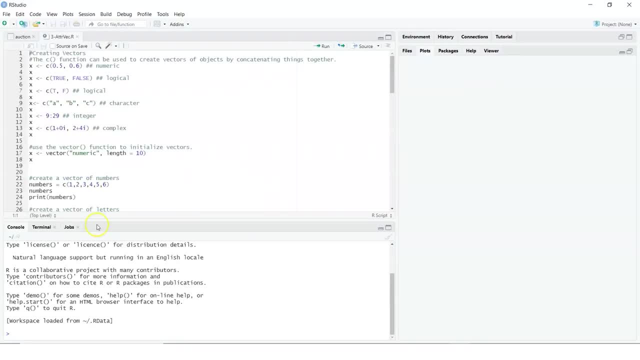 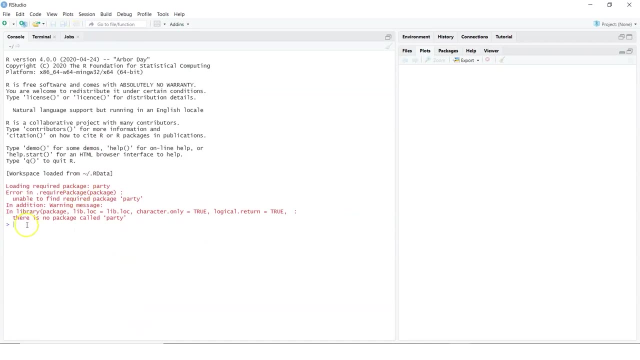 So when you talk about list, what you can do here is: let me close this one and this one. So what we can do is we can basically say, for example, test, and I can see it can basically give something here. so for example, I can say music tracks and then 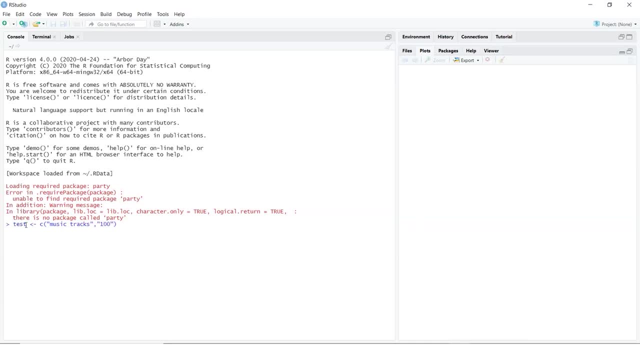 I can say how many hundred of them, and I can say: let's give hundred as number, and then we can say how many of them got five stars, and I can do this, so I can check this and this shows me all the objects or elements of this list. right now, when we do this, 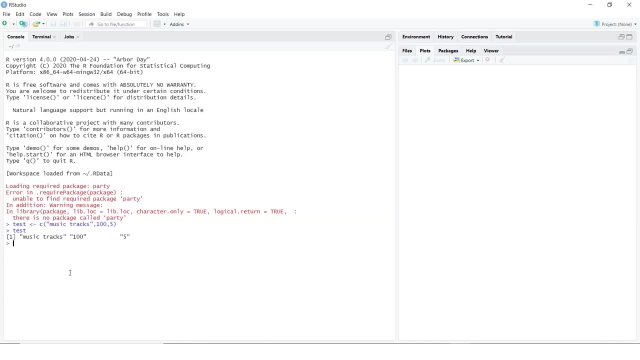 what we are doing is we are creating a vector, right and vector basically can have coercion depending on what are the elements which are passed, because whenever you use the c and you create a vector, it will only accept elements of the same type. so, for example, if I do a class on test, it shows me here all the objects are of type character right. 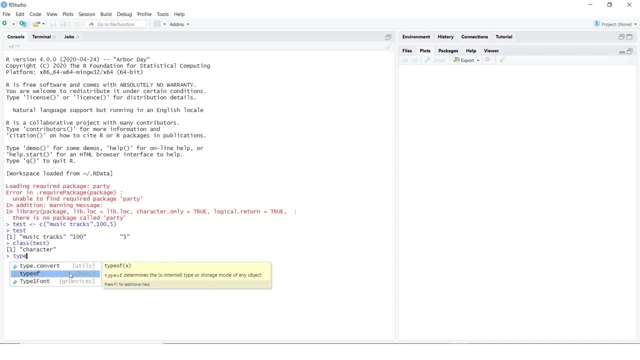 and you can also use type off to check for our test variable, and it is basically having all the objects as character. now, how would you create a list? so what we can do is we can use a list function. so, for example, let's again do a test here, but this time. 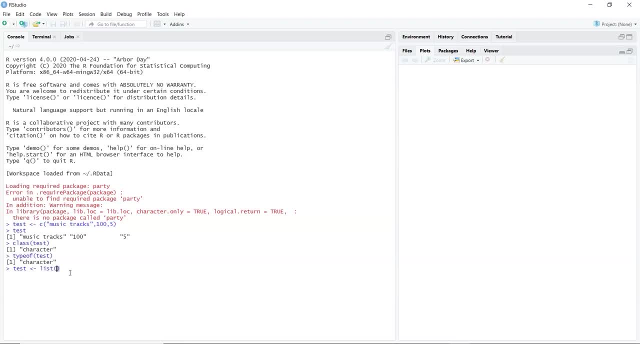 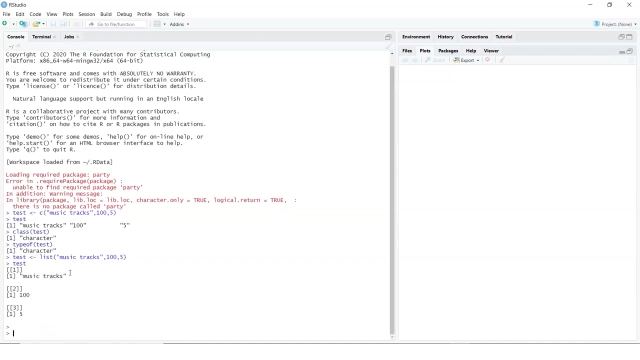 I am going to create a test variable, so I am going to create a list, so I am going to- I'm interested in creating a list, and list can have objects of different types. So let's say music tracks, and then I can just give 100 and I can say with rating 5. and now, if I look at my test, 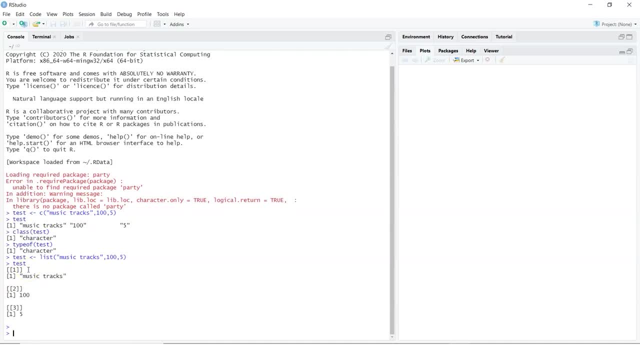 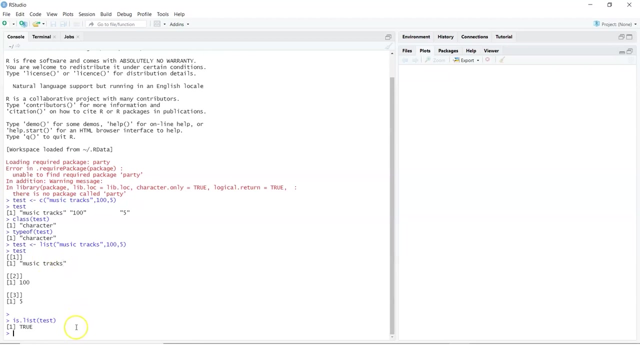 it shows me all the elements of your particular list. Here we see each element or each object with a double bracket, and we can see each element. Now what we can also do is we can use is list function and then we can pass and test here to check what is it. and it is a list right. 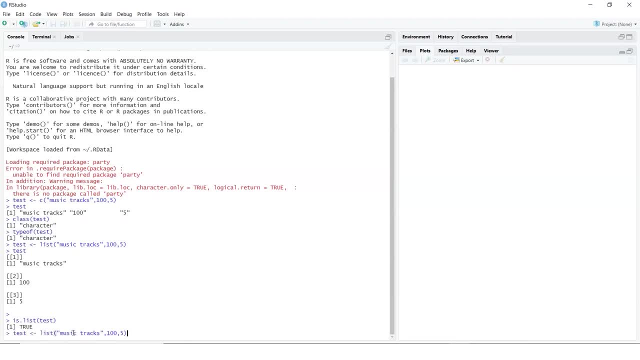 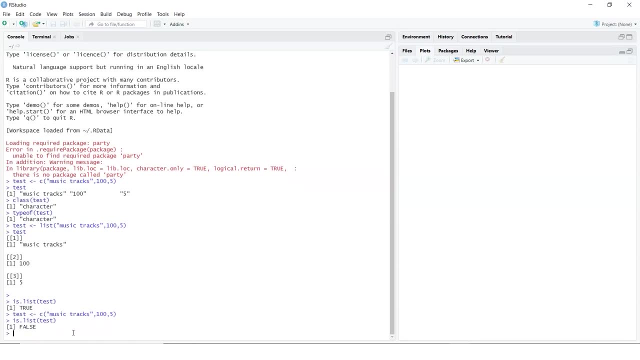 So here we have created a list, but if, for example, we take the previous example where we were creating a vector and if I would do a is list, it would show me false. So we just created a simple list and we can also arrange labels or we can use a name function. 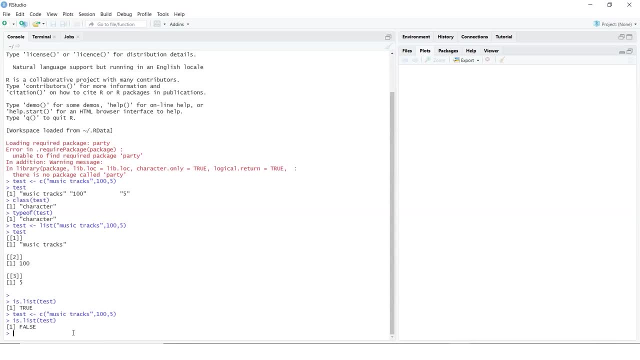 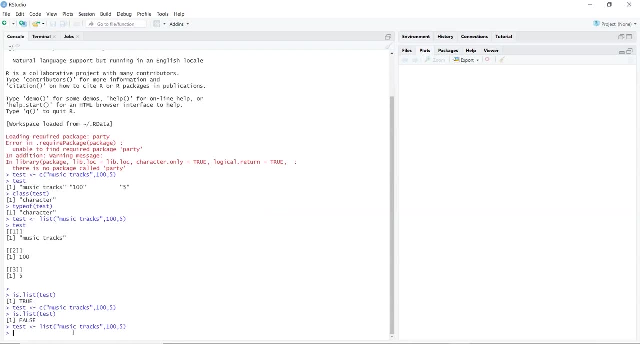 to basically give names. So what I can do here is: let me create a list first, so I can do that like this. and now what I can do is I can do a name and I can use a name function to this test, and then basically what I can do is I can pass labels. 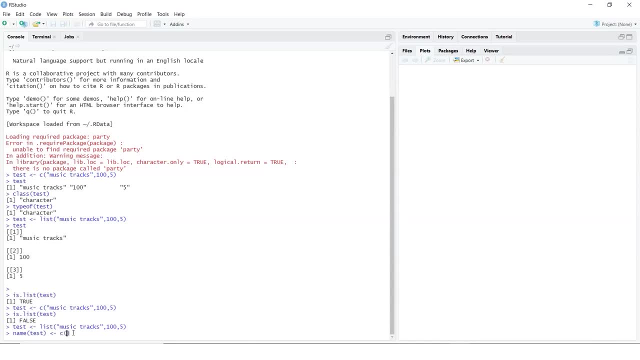 So here I can just give in some names here. So for example, I can say: let's give it a name product. So say we are talking about product of a company. and then we can say: here I can give count and here I can give rating, and this is basically to give in names. 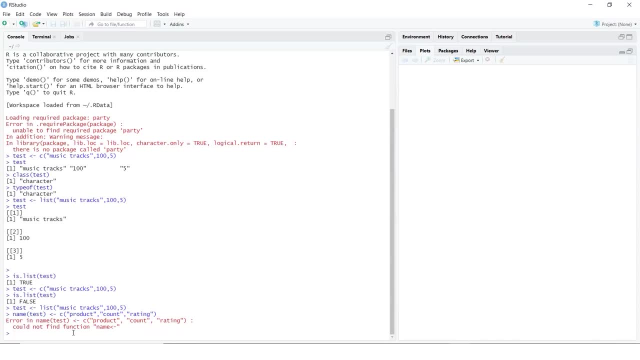 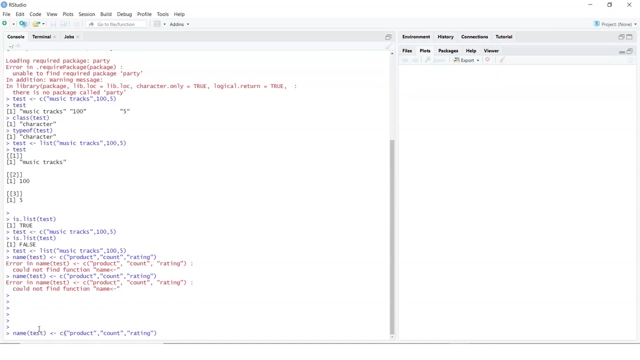 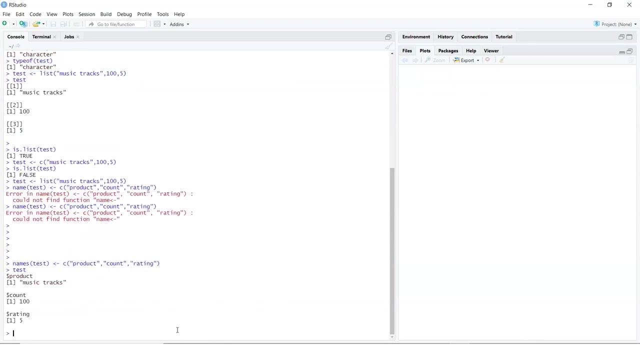 So let's just give there's some error here. let me just check this. So let's use this name function here, and what I'll do is I will basically use names and now let's do a test So that shows me the names, what we have assigned to our list objects. 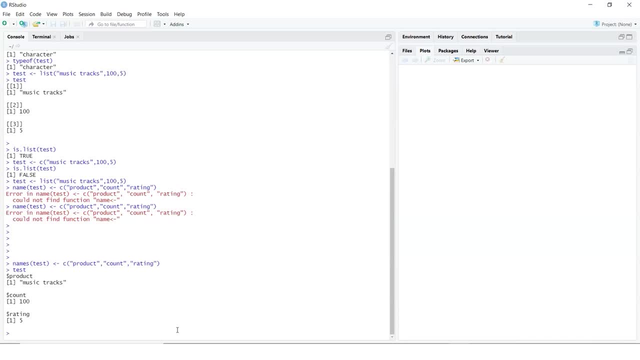 Now we can always access the elements of our objects from a list, using indices or even using double square. So, for example, I have test here and basically I can give something like this which gives me, based on the indices, the position. So let's do a test here and basically I can give something like this which gives me, based on the indices, the position. 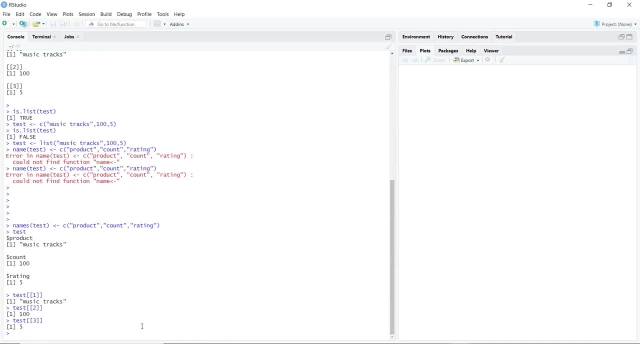 So I Spring, we can do this. What I can also do is we can specify names when creating a particular list. So, for example, what I can also do is I can say product dot, category, And now I can just give list function. So I would want to assign it. 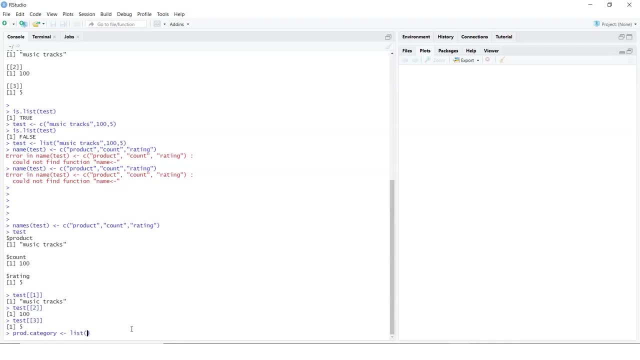 assign names while creating a list, So I can say, for example, product, and this would be, say, music tracks, Then I can give, say for example, count, and count would be 100, and then ratings, and I can say five, and now we can basically access this list which we have created. So what we have done here 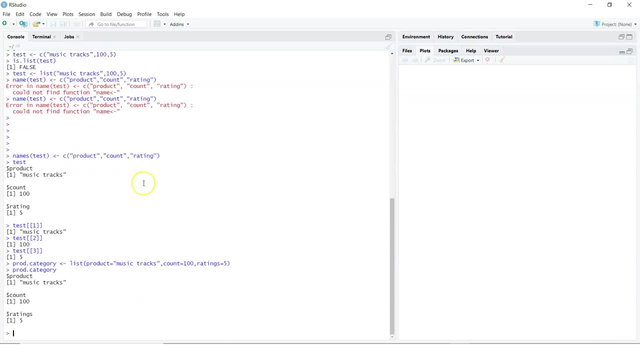 unlike earlier, when we created a list and then basically use names function to assign a name to it or each object. here, while creating a list itself, we passed in the names, So we can also do that Now. if you would want to basically display the list or a compactly display structure of a list, we can always use the string. 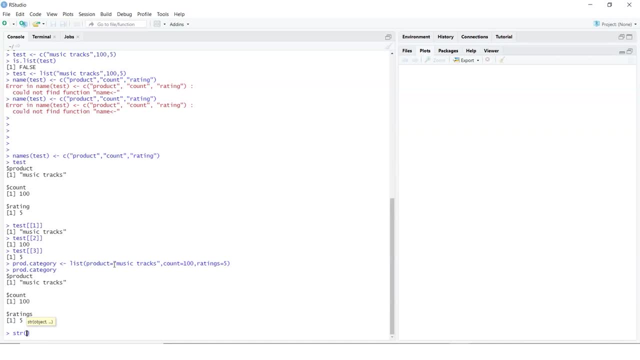 function and here I can pass in the name. So let's choose this one. and this is in a more compact way, listing down the elements of your list. So list can be containing other lists also and we can also do that. So for example, I create one more list, for example I can say similar product and here I can give a list. 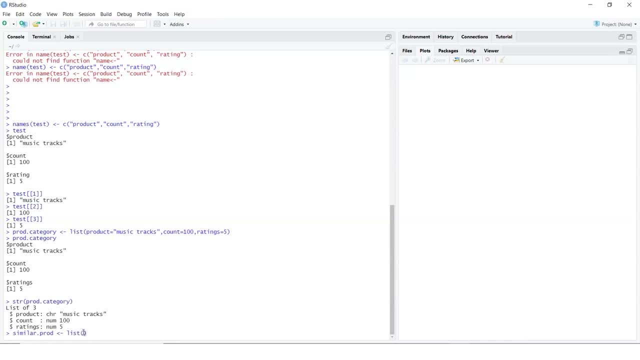 again, and what I would want to do is I would want to say product equals, and I can say film, and then I can basically give a count, And then I can give ratings, say four, and here what I've done is I have just created one more list. 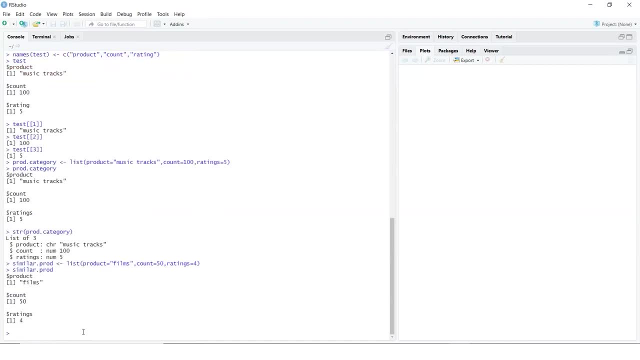 But my intention is not just to create a list, but I would want to add this to our existing list. So what we can do here is we can take our previous list, that is, product dot category, like what we did earlier. And now I intend to say list, and here I would want to say, for example, let's copy this, or we can just 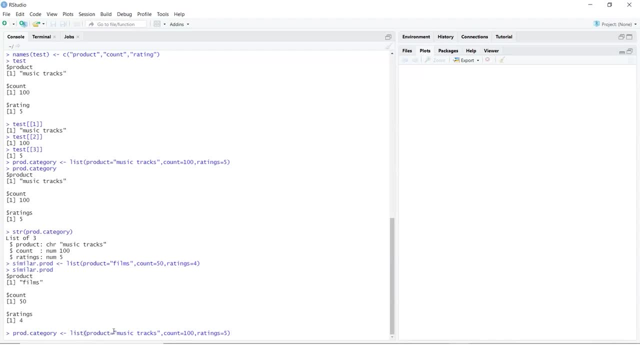 So this is what we were doing when we were creating a list, using product, giving the names while creating a list, And what I also want to do is here I will just say similar and then pass in similarprod. So now, if you look at our list, we have just added new elements. 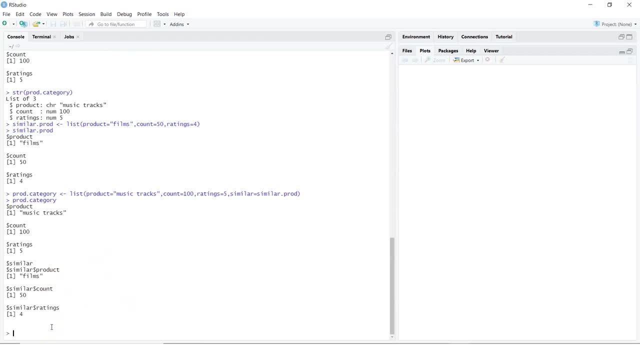 So this is one more way where we can create a list and we can basically add or our list can have Other list. So when we talk about subsetting or extending list, So one of the main ways, as I said, to access a specific element or a subset, we use double brackets and we can always do that. 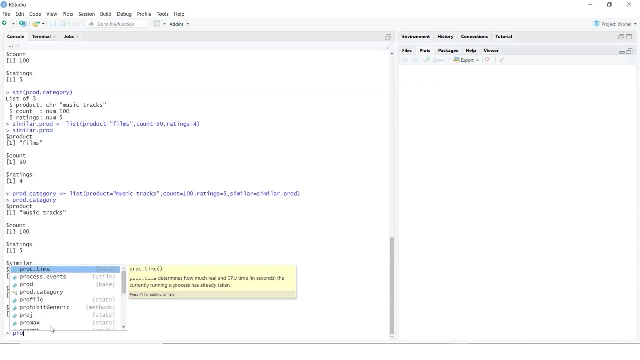 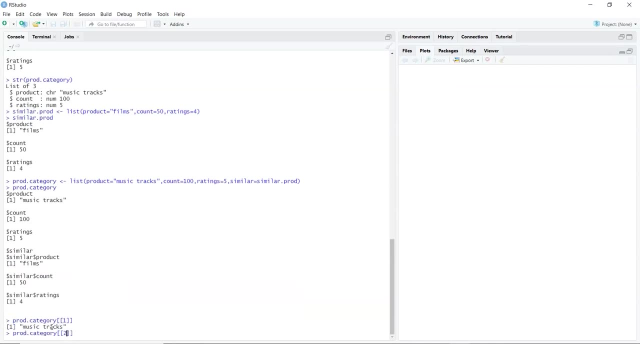 So, for example, we take Our prod dot category and then I would want to access a particular element. so I can always do this by giving the index positions and I can access the elements Or Of my list. So this is one single way. 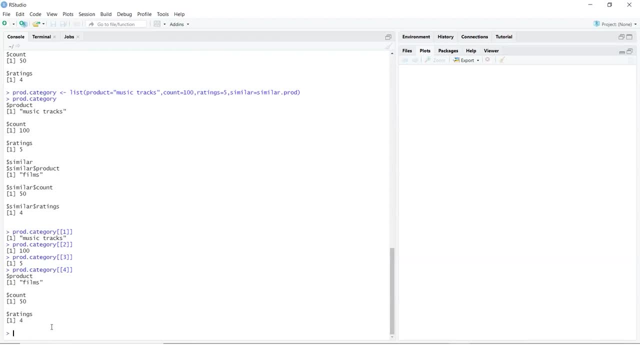 Now here, if we use a single bracket instead of double bracket, then in that case we will. the output would be a list. So if I look at this one, then this would be a list, But if you use double brackets, then you're accessing a particular object. 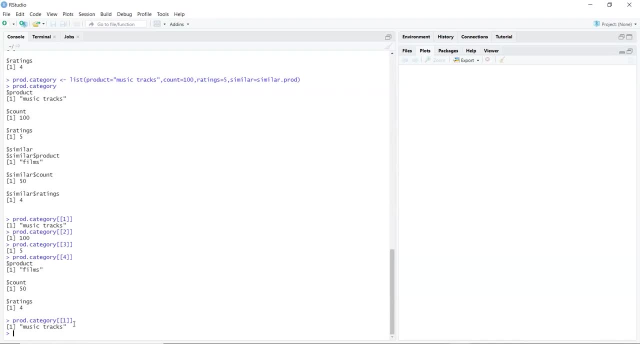 If we were creating a vector, we could just be using a subset by using the C function. Now what we can also do is we can subset by names or even logical. So what we can do here is we can take this product category and if we have defined names, then in that case what I can do is I can say I would be interested in music tracks. 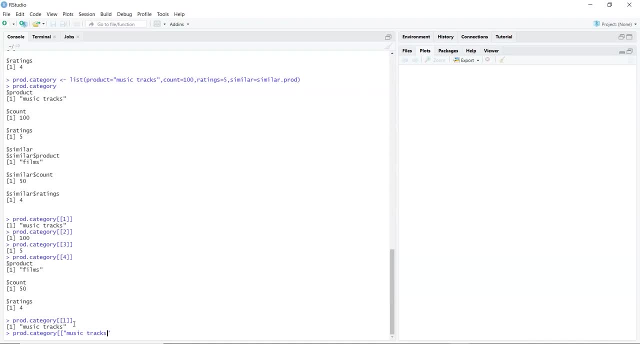 And this is the name we had given. So we can close this one and we can try accessing the elements here. So So we what's the name we had given? so No, it's not music tracks. That's the value. The name is product. 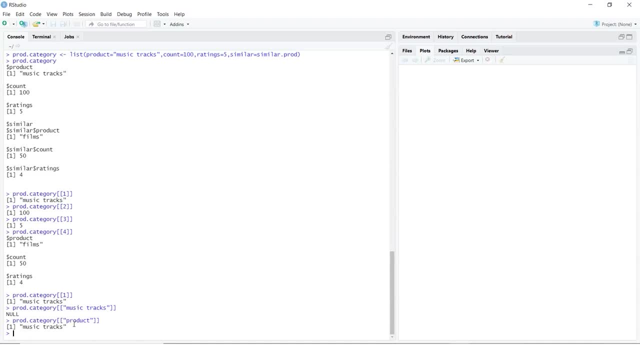 So we do this and then we can access the elements. What we can also do is we can be subsetting based on logicals. So what we can do is we can basically just give something like this, and here we can pass in values, Something like this: 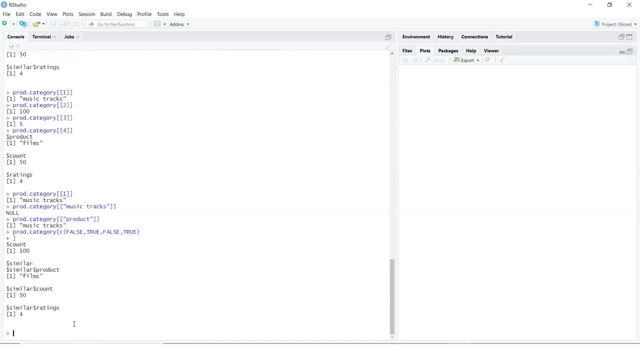 And we missed a bracket. So that's also a way of pulling out the value. So you can be doing a subsetting using the names which you have assigned to objects within your list, or you can say names which you have assigned to the. 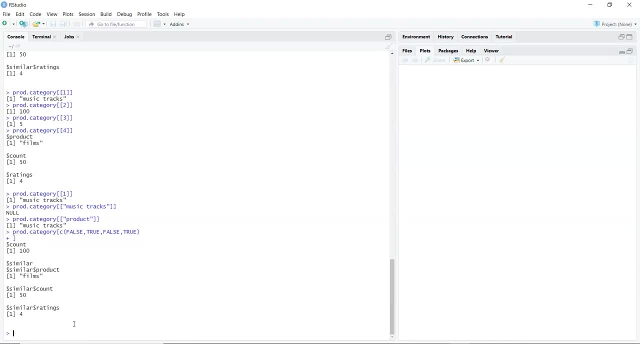 Elements or by using logicals. Now, what we can also do is we can use the dollar function. Now, if you see, here we are looking at the name and that is preceded by dollar. So we can always pull out the values from our list by giving the list name and then give it dollar symbol and then choose the name. 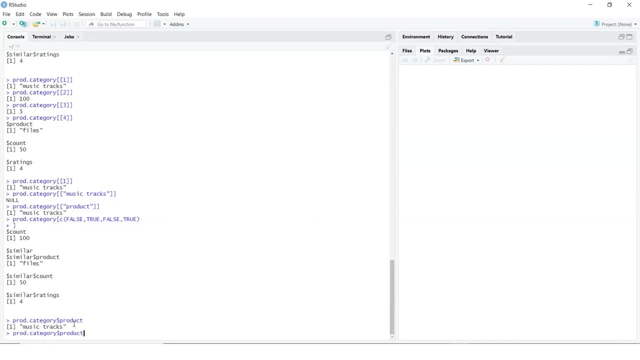 For example, if I choose product, I can list the values here I can be looking at, say, dollar, and then choose a count, And this is also one way of accessing your elements from the list, using your dollar symbol. Now, to add elements to a list, as I said, you can add a vector of names and that can be passed to your list. 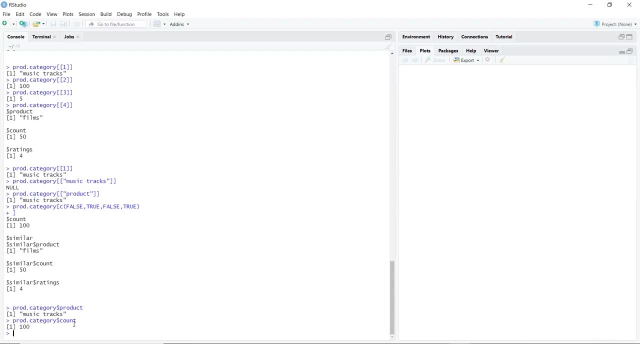 So these are different ways in which you can work with list. and then you can access the elements, Either using indices or using names, or even using dollar symbol and pointing the right names. So this is one simple example of working with your list. Now one more. 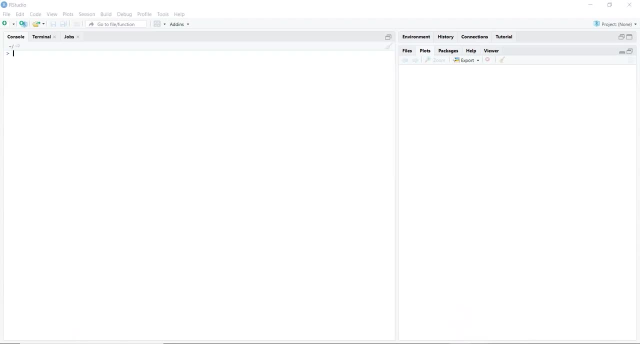 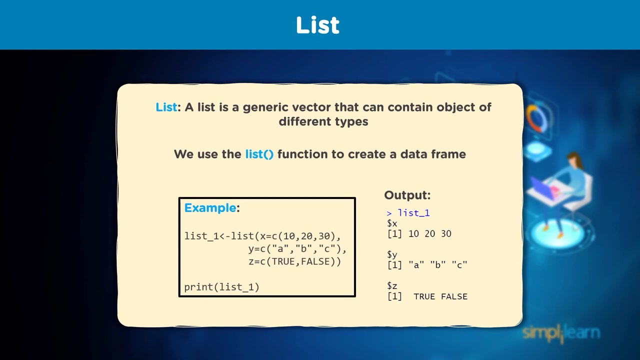 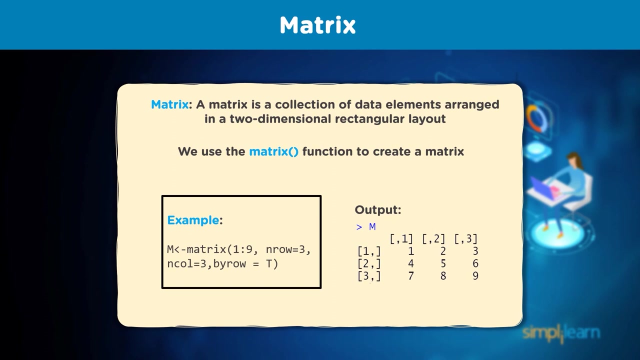 And now I can just do a control L and I can clear that off. So your list always remember, is a generic vector that can contain objects of different types. Now, when we talk about matrices, now, matrix is a collection Of data elements arranged in two dimensional rectangular layout. so we can use matrix function to create a matrix, as shown here. 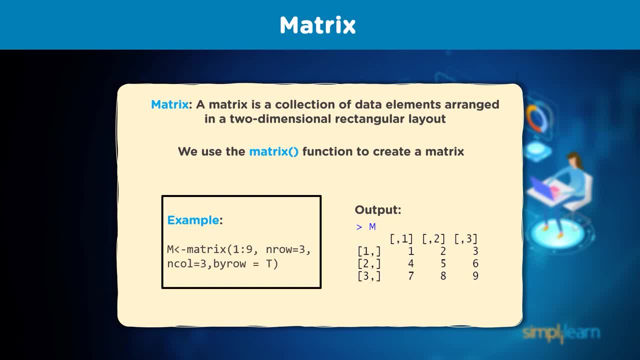 So matrix is two dimensional. Now we already know that vector is one dimensional array of data elements or a sequence of data elements, But when we talk about matrix, it's a collection of data elements that is two dimensional, arranged in fixed number of rows and columns. 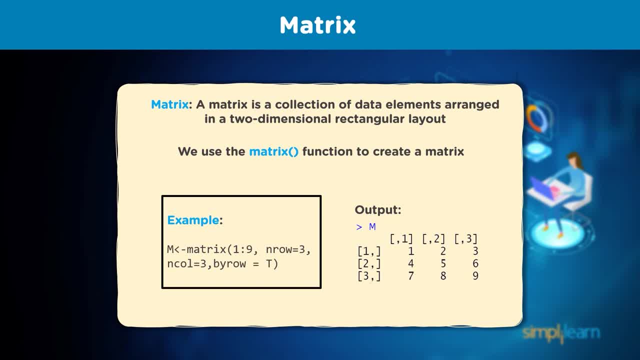 So here You see that we are creating a matrix and we have specified: the number of rows is three, number of columns is three and we want it to be arranged by row where we have given the value is true. So always remember: matrix is two dimensional and matrix can have only one atomic vector type. 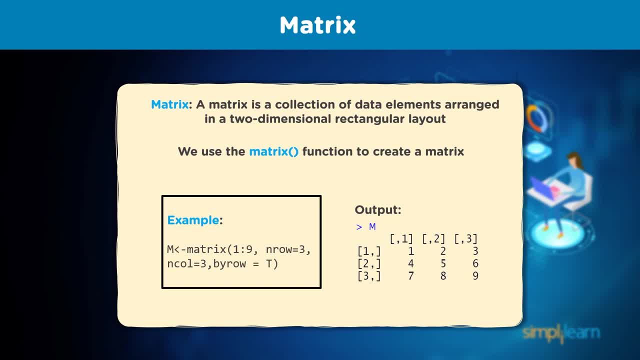 Unlike your list, it's a natural extension of vector going from one dimension to two dimensions. So matrix actually needs a vector Which contains values that you place in a matrix and at least one matrix dimension So we can choose to specify the number of rows or number of columns when we are creating matrix. 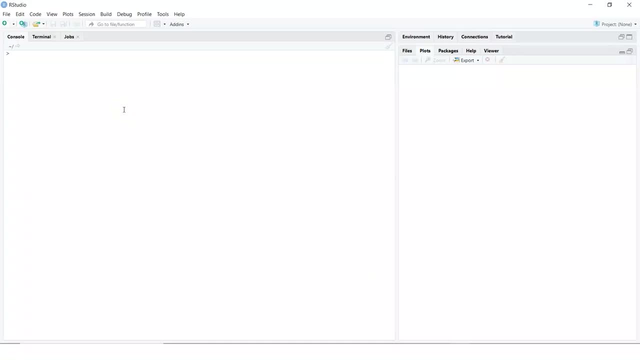 So let's see a quick example of working with matrix. So, for example, I could just say matrix, which will have values one to six, and then I can basically give n row And you can give A value to this one and that's my matrix. 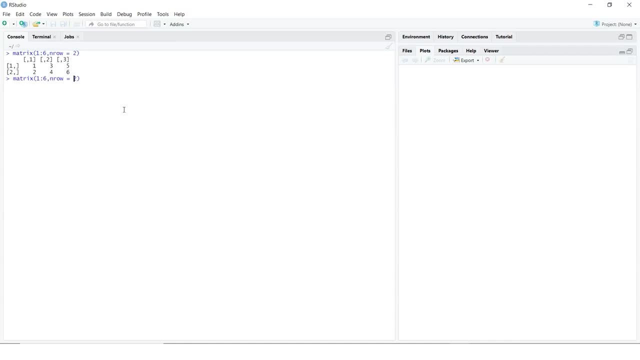 Similarly, you could also be giving N columns, So I can just say and call and I can choose this one and then pass in the value. So that's a matrix where our fills values column by column. Now if you intend to fill up matrix in a row wise fashion, so that your values one, two and three are in first row, then 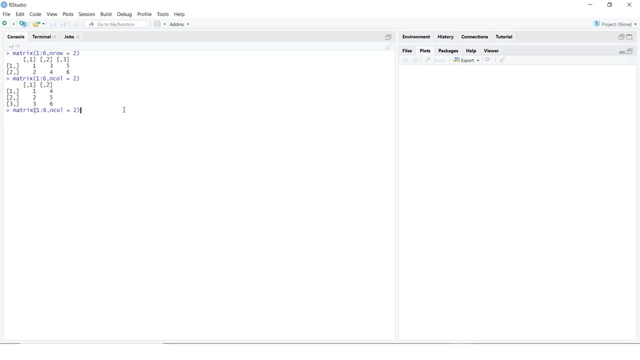 We have to just modify this in a little bit different way. So we have to say: matrix one, colon six and row is two, and then I can give by row. So you always have these helper functions which allow you to put out the values. 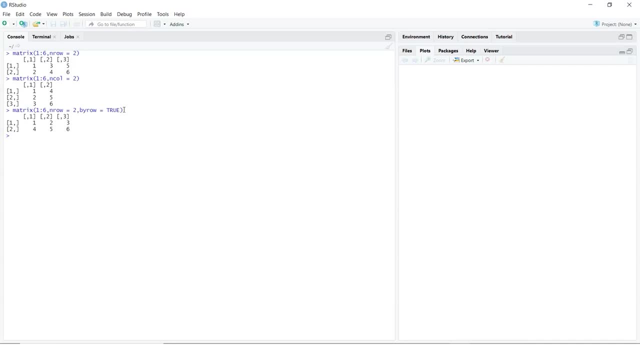 So, for example, I do this and then I can do a control enter. So now, if you see, you have the values one, two and three in your first row. So when we pass a matrix function to a vector that is too short to fill up an entire matrix, then something different happens. 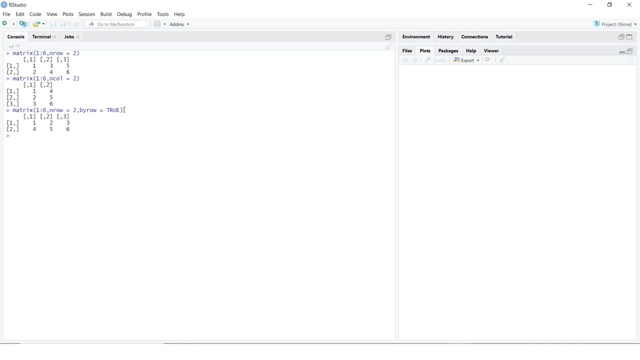 We can have a look at this. So say you pass a vector containing value one, two, three to the matrix function and say explicitly: you want a matrix with two rows and three columns. How do we do that? So, for example, I can say matrix. 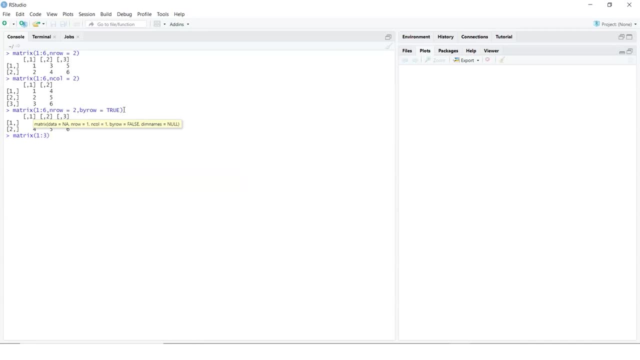 And here I can say one, Here's two, three. Now I can give n row And then I can give the number of rows which we want is two, And then I say n column And this one, I'll say three. So I can do this. 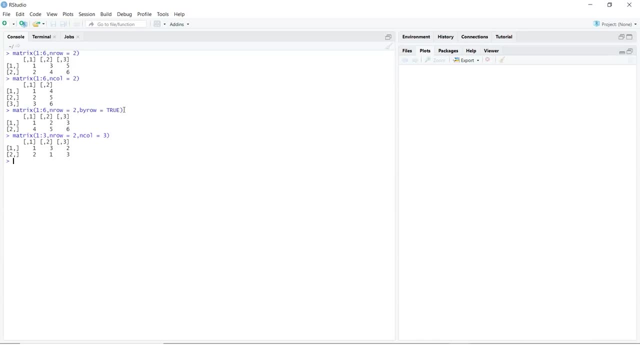 And here what I have done is I have given the values one, two, three. I have said number of rows is two And your number of columns is three. So here R fills the matrix column by column. So I can do this. 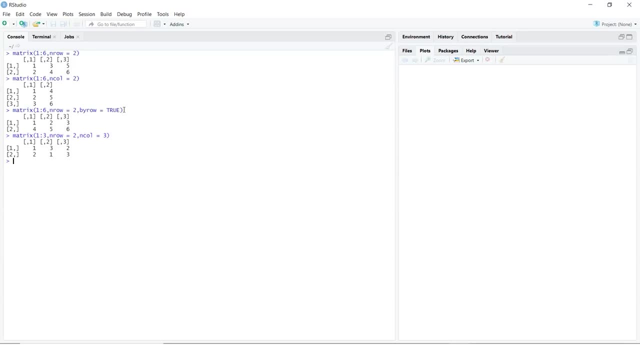 Column by column and simply repeats the vector. Now, if you want to fill using a four element vector in a six element matrix, in that case obviously R will generate a warning message. Now, apart from the simple matrix function which we are seeing, you also have some functions such as R bind and C bind, which R offers when you are working with matrices. 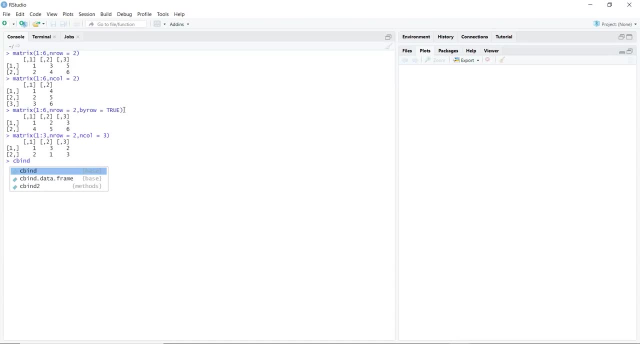 So we can use those. So, for example, I could say C bind, I could say one colon three, And then I can say one colon three, And that's my C bind. that is column bind, where I'm passing the values one, two, three and which are stacked in columns. 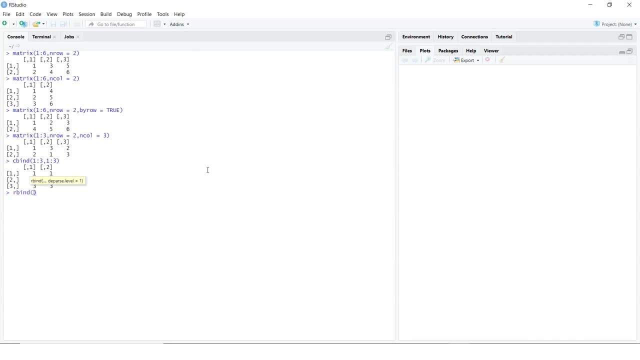 I can also do R bind And similarly we can be passing in the values. So I can say R bind And that basically arranges the values row-wise. So be creating a variable. For example, let's say N And let me create a matrix here. 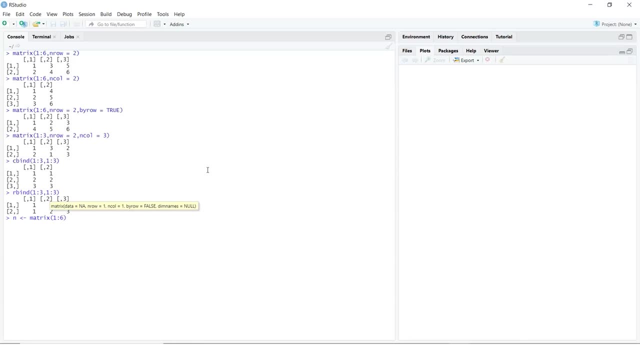 So I'll say matrix, Now that will contain one, two, six, And I can say by row, And then you can give value, which is true, And then I can basically say: the number of rows is going to be two, And this is also fine. 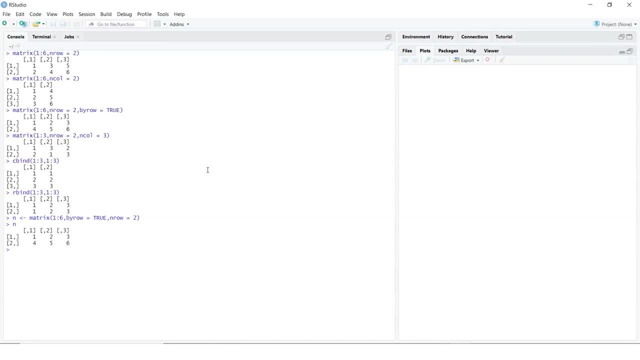 So let's look at the value of N here. So you basically created a matrix with one, two, six. You arrange them row-wise And the number of rows, what you have chosen, is two. So what we can also do is we can use R bind and we can add values to it. 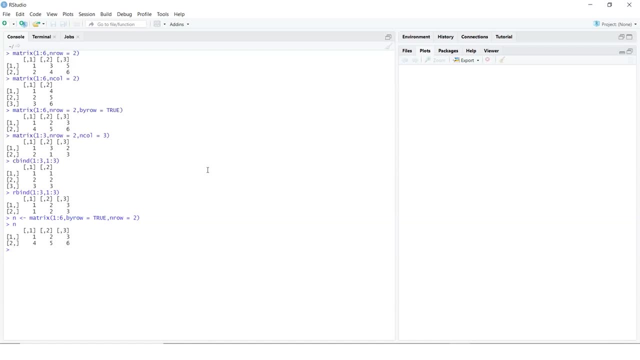 So, for example, if I want to add values seven to nine, what I can simply do is I can do a R bind. I can say I would want to edit my N and then pass in the values. So I can just do this. 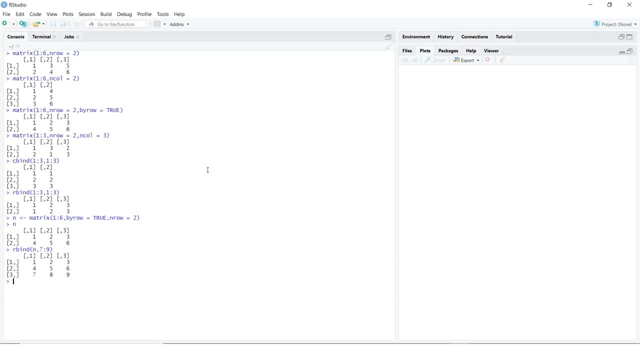 And this has basically appended or added values to existing matrix. So, similarly, you could have done a column bind and you could have added values to your existing matrix. So, for example, if I take this one and look at my N And what I could do is I could do a C bind. 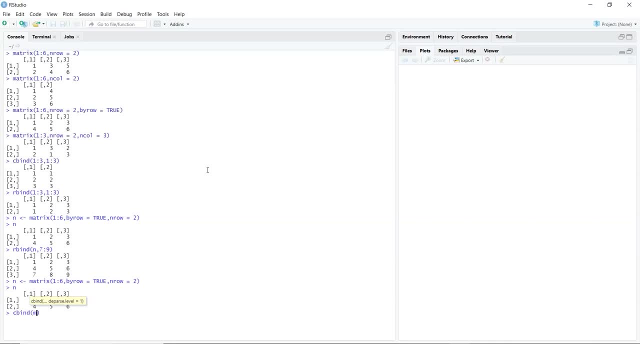 And then I can basically take my N And then pass in values to this one. So let's say 10 and 11.. And basically I've added 10 and 11 as a column to my existing matrix. So this is one simple way where you work with a matrix and you are appending the values either at a row level or at a column level. 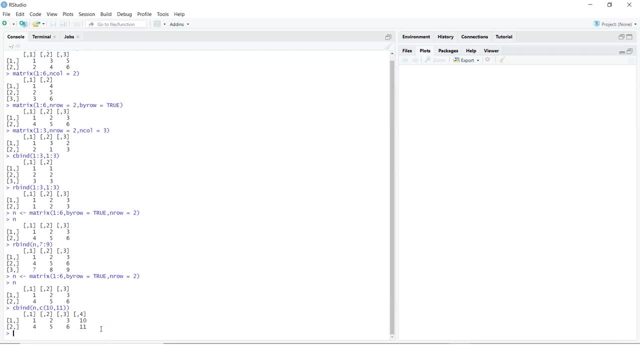 So let's also look at some other examples. So, basically, if you would want to work with matrix, one of the useful things would be naming the matrix. That is, in case of matrices, we can assign names to either the columns or the rows. 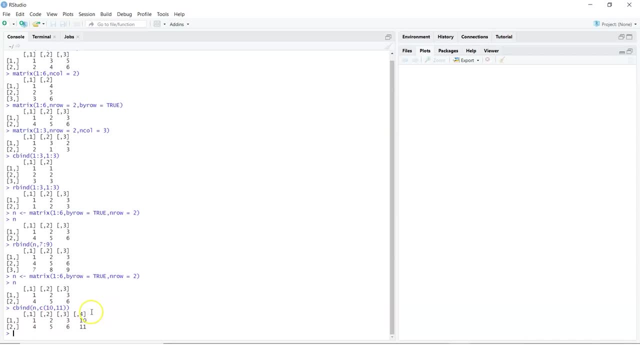 If you don't do it, we see the default values here, which follows a numbering. But what we can also do is we can use two functions here. One is row names, Or you can use column names. So these are the two functions which can be used. 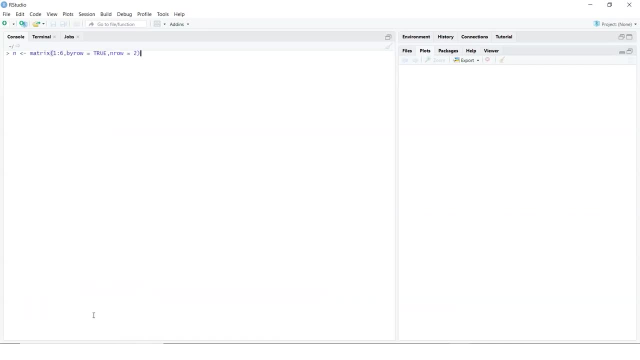 So, for example, let's do a control L, Let's try to get our N, And this is what we are doing here. But what we would want to do is we would want to give them some names. So, for example, I'll say row names. 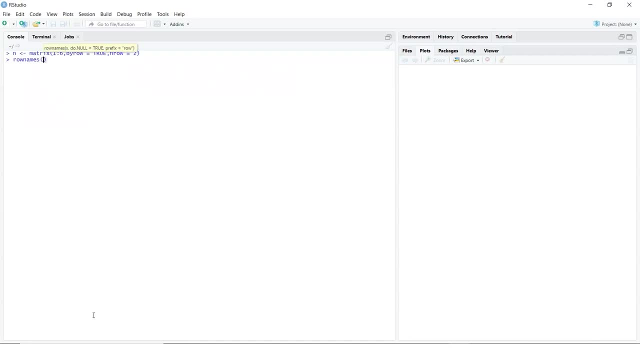 And then I will basically pass in a vector which has row names or vector which has column names. So what I can do here is I can say I would want to give row names to N And then I basically give some value. So for example, let's say row 1.. 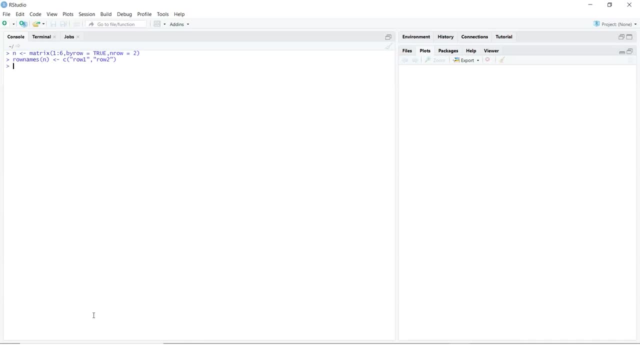 And then let's say row 2. And now I can look at my N, which has the row names assigned to my rows. Similarly, I could have also given column names. So all I need to do here is I need to say column 1.. 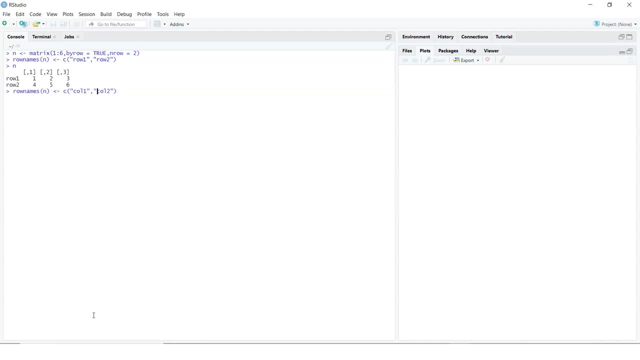 And then I will say column 2.. And then I can be using column names. And let's look at this one. So what went wrong here? So we have three columns here. We forgot that, So we have to add one more column name. 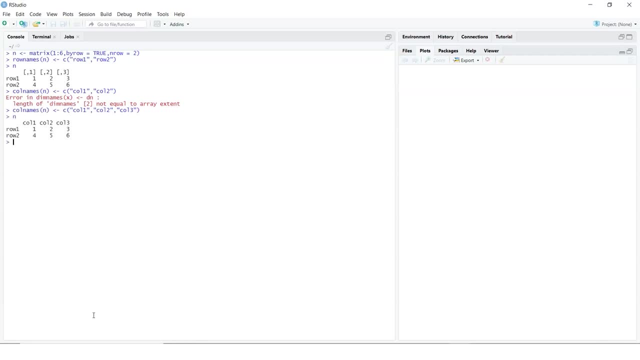 And then it should be fine. So now, if you look at this one, we have just given row names and column names, So naming the columns or rows in your matrices can be very useful. Now, as the previous error says, there is also a function called dim names. 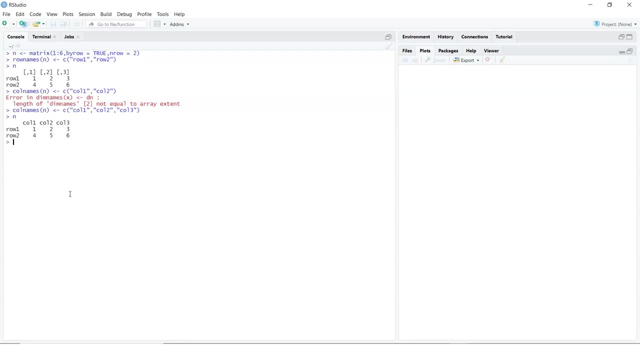 And that's basically an argument of matrix function which can be used. So we could also do something like this. So, for example, I have dim names, So let's have our N, And then what you can do is you can do a dim names. 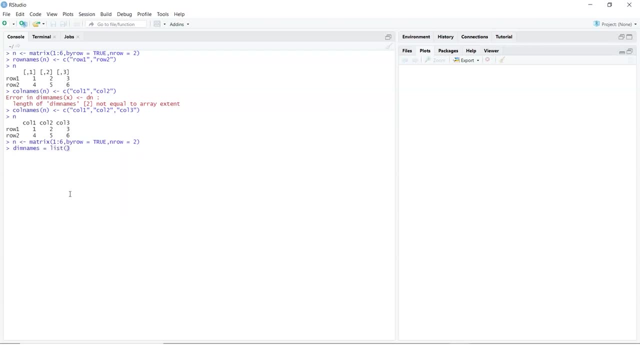 Which you can then just create a list, And in this one you can pass in a vector For row 1.. And then vector for row 2.. And what we can do here is: once we have given this, Let's give a comma here. 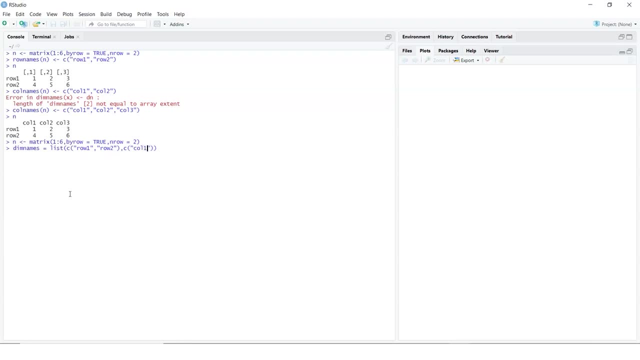 And then give C And then give your column names, Which is column 1., Column 2. And then basically column 3.. And now, if you just look at dim names, So you can just see that you have given some row names and column names. 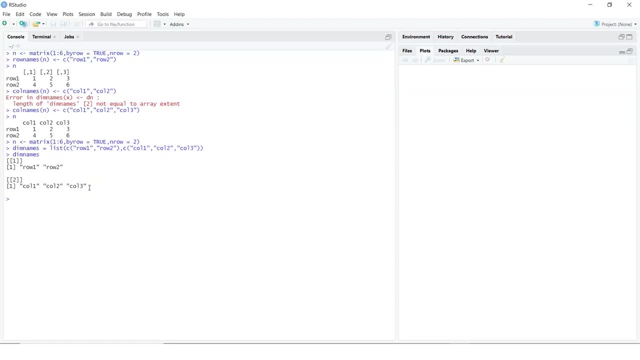 And this can be used basically to assign to your list. So if you try to store different objects in a matrix, What would happen? Coercion would take place Right. So, for example, if I have X And let's basically try to create a matrix, 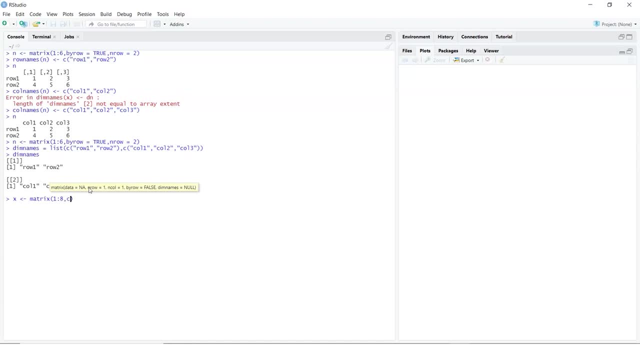 Which will have 1 to 8. And let's say the number of columns Is going to be 2.. So let's look at our X And this has the values. Now, what if I create, say, L, And then basically I will create a matrix? 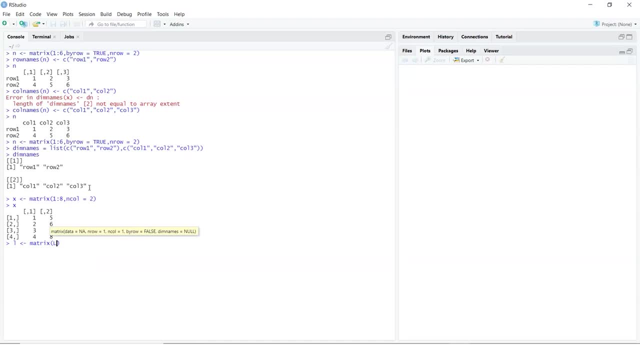 Which will be a matrix of letters. So let's say letters, And then here with letters, I'll say 1, colon, 6.. Now I would want to give the number of rows And let's give it, say 4.. And let's say number of columns. 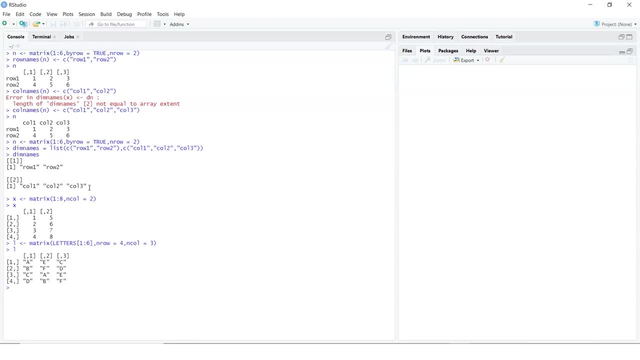 And let's give it 3.. And now let's look at the value of L. So it has letters And X is having numbers. And what if we bind them together using C bind, Which is for column wise binding? So for example, if I do a C bind, 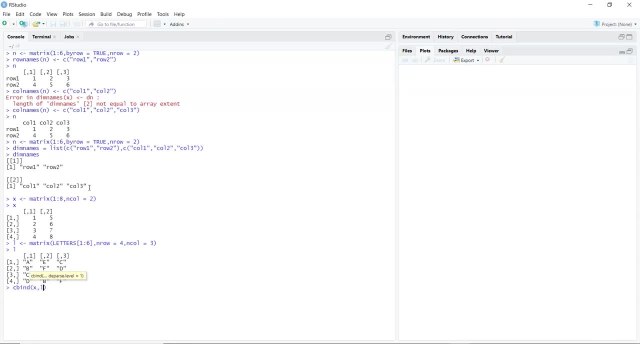 And then pass in my X, comma L. So if you see, here There is a coercion which has happened Where everything is converted into characters, So you can always do a class And you can check. So this is a simple example of working with matrices. 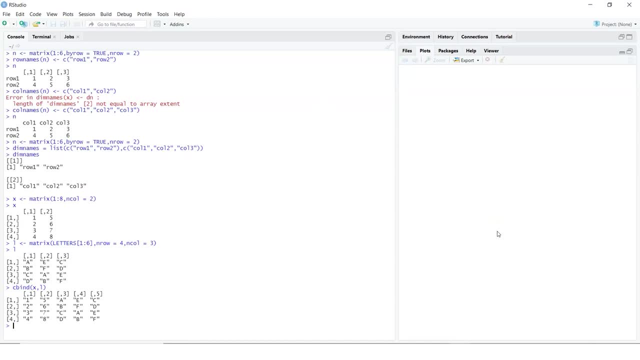 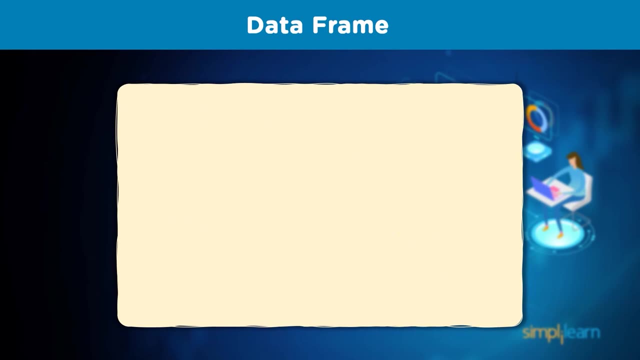 There are much more You can do subsetting, like what we saw in list, But that we can learn later. Now let's learn about data frames And what is a data frame And how do you use R to work with data frame. 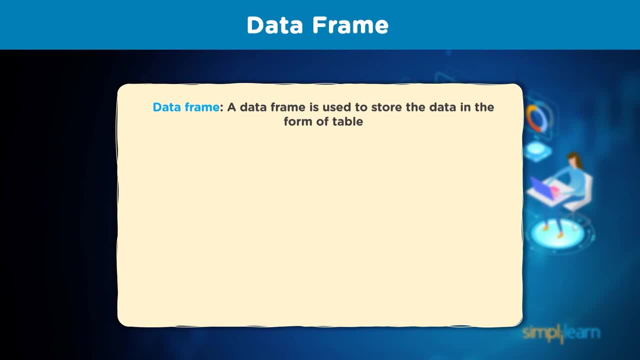 Now, data frame is used to store the data in the form of a table, And for this we have a function, data dot frame, To create a data frame. So what we know already is That data sets are comprised of observations, Or what we call as instances or variables. 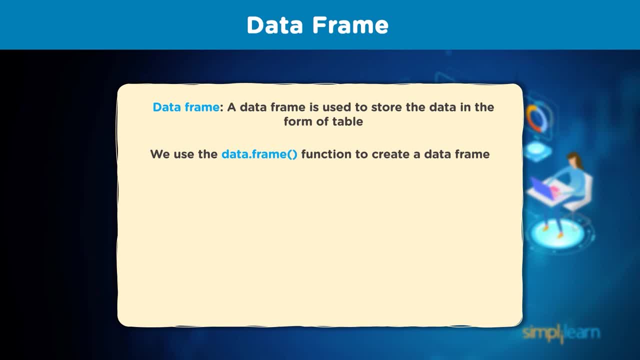 And we always have observations To which some variables are associated. For example, we can talk about data sets, Data sets of, say, five people. Now let's look at the information here. Here we look at the body mass index, BMI, Where we are using a data dot frame function. 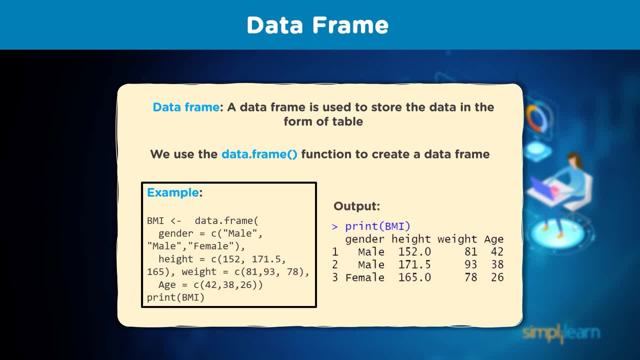 And then we are passing in, say, gender, So we use the C function to pass in the values, And then you have height, And then you have weight And age, And these things then become the columns of your data frame. So, for example: 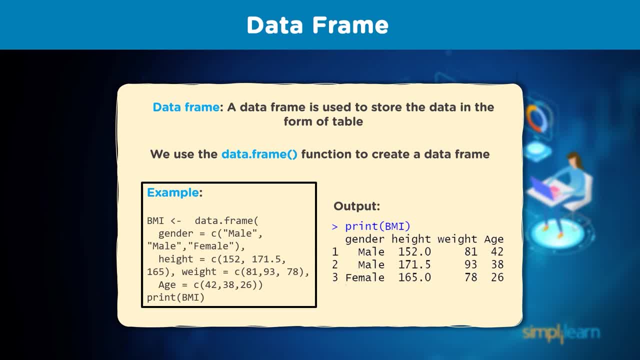 If we would want to work on creating a data frame for people Where, let's say, each person is an instance, And properties about each person, Such as name, Age, Child Or if the person has a child, Would become the variables. 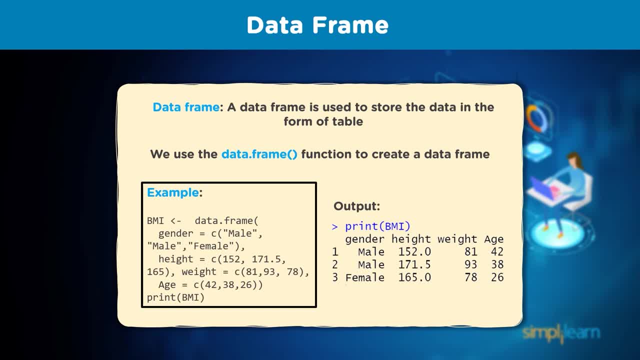 So if we have such kind of information, We cannot easily store that in matrix or list. Now data frames can be used for such cases. Now it's a fundamental data structure to store data sets- Pretty similar to matrix As it has rows and columns. 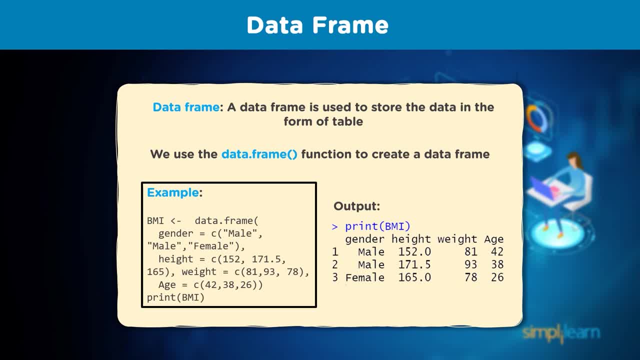 And here rows correspond to observations. Now, here we can talk about in every individual or every person, Columns correspond to variables, That is, properties for each person. Now, difference Between your data frame and matrix Is that data frames can contain elements of different data types. 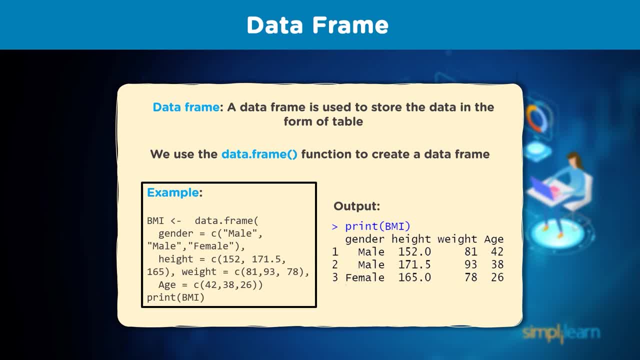 So, for example, We can have one column being character, Other being numeric And yet another being logical or numeric. So restriction is that elements in one column should be of the same data type. Now how do we work with data frames? Let's see some examples. 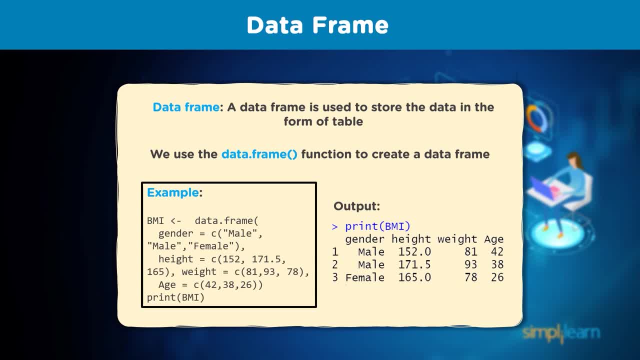 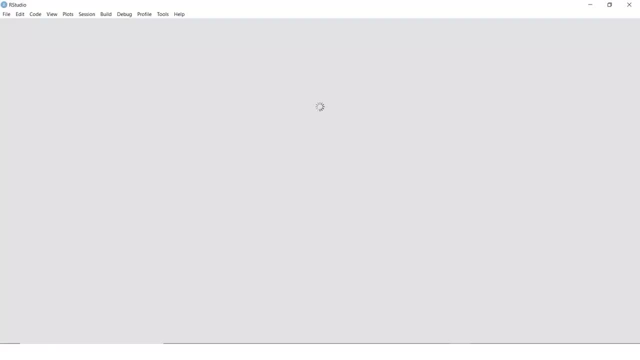 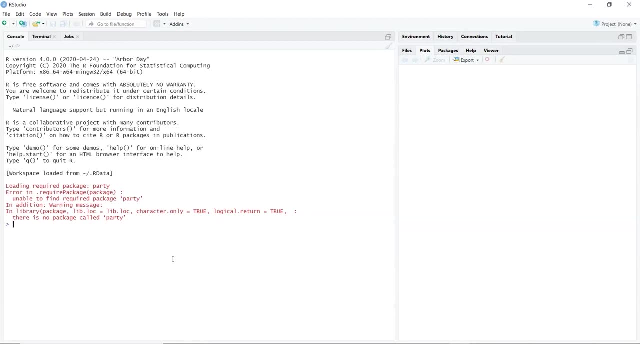 So what we can do is We can bring up our R. So when we talk about data frames, Usually we don't create data frames by our self. We import data from data sources Such as CSV file Or RDBMS, Or even your Excel or SPSS. 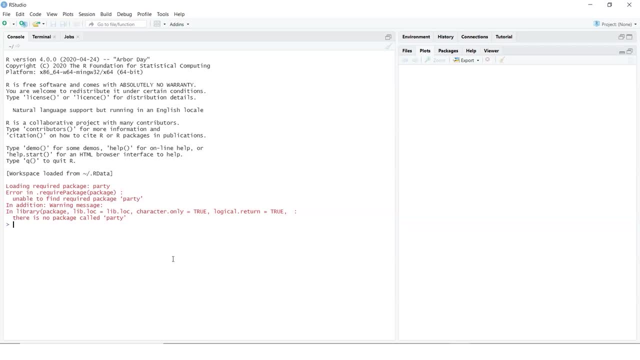 And then we create data frames. Of course, R has ways to manually create data frames Using data dot frame function, So we can create three vectors first, And then we can pass in those vectors To create our data frame. So let's do that. 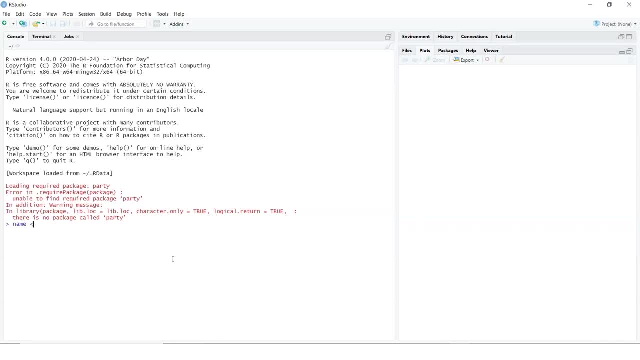 So let's say name, And here I will use the assignment operator Which we have learned earlier, And then I'll use C, And then I can give some names here. So let's say John, And let's say Peter, Let's say Patrick. 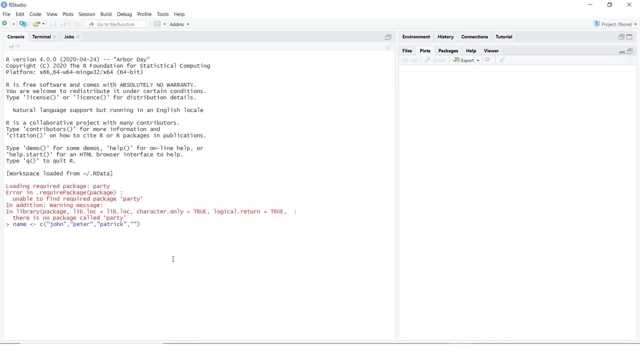 And let's say Julie, And let's also give one more name, So let's say Bob. So this is the vector which we are creating And we can check. This is the vector which we have created. Now, obviously, you can do a class. 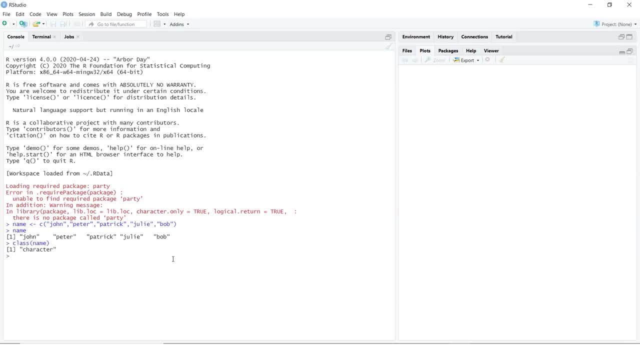 And you can check what is this And that says it is a vector of character. Now, similarly, we can create one more vector, Which is age, And let's give some numbers here. So, for example, let's say 28. And 32.. 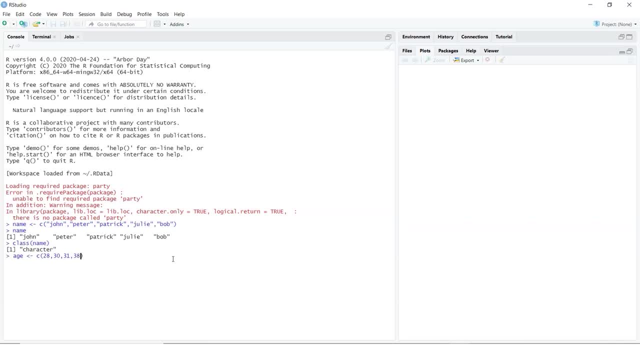 31.. 38., 35. And these are the values for the age, So age is also created. Similarly we can say if each person has children, So we can say children. And then I'll create one more vector And here I'll give values which are logicals. 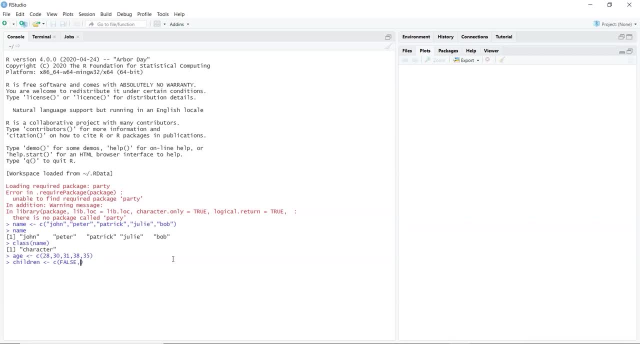 I'm not going to give any numerics Or character, But I'm using logicals here. So if a particular person Has children Or no, So let's have this vector created. And now we have three vectors. That is name. 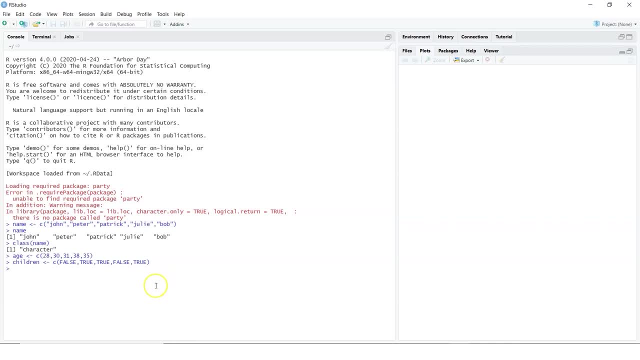 Age And children, And we can use this to create our data frame. So we can just call our data frame as df And what we can do is we can use dataframe function And then what we can do is we can pass our vectors within this. 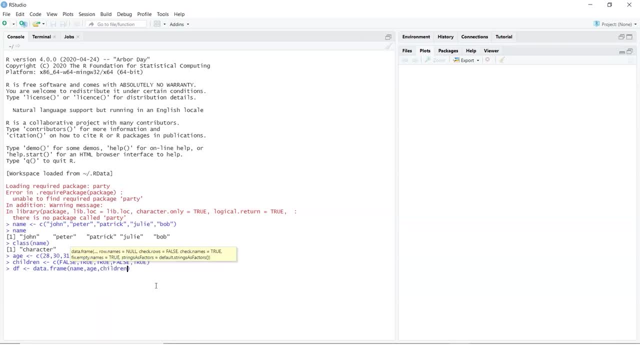 Such as name, Age, Children, And that should create my data frame. Let's have a look at this And this shows me that the data frame is created Now. column names are inferred from variables Which are passed to dataframe function. 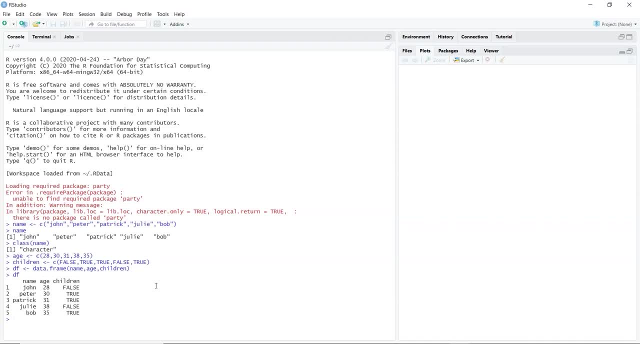 So the variables which we have passed to our dataframe function Is name, Age And children, And those become the column headings for my data frame. Now, what we could have also done Is we could have created it In a different way. 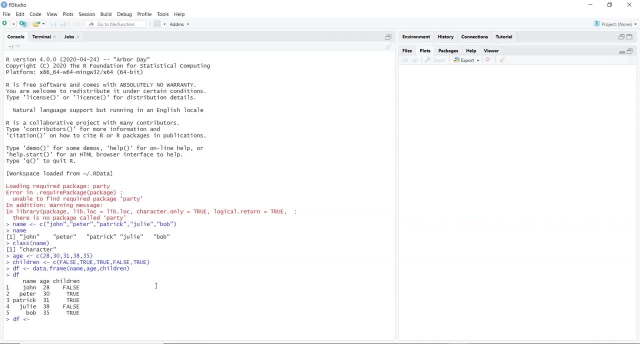 So I could have said df And then I could have used my dataframe function And in dataframe function I could have said: name Is going to be name, Age would be age, And then I could say children Could be children. 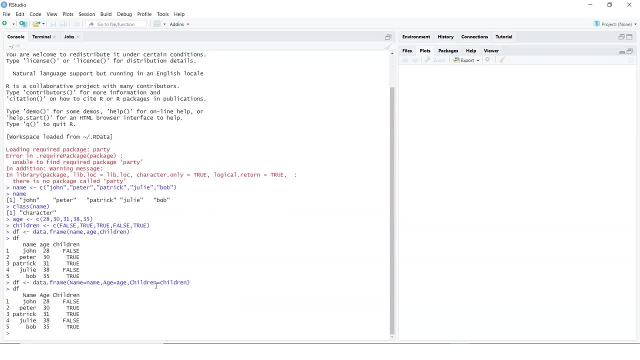 And I could do this, And this is also one more way Where I am creating a data frame, And in this way We can now have rows of data frames, Like in matrix. So this is also one way of creating a data frame. 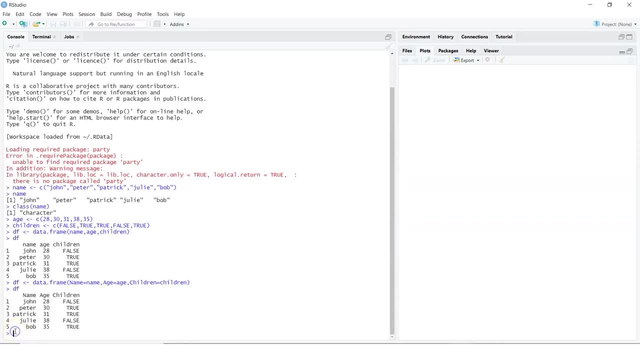 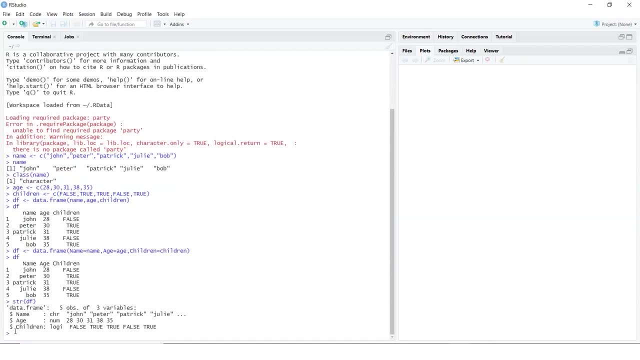 To look into the data frame structure. We can always use str And then we can pass our data frame And this basically prints out Similar to that of list. So We also need to know That under the hood, Data frame is a list. 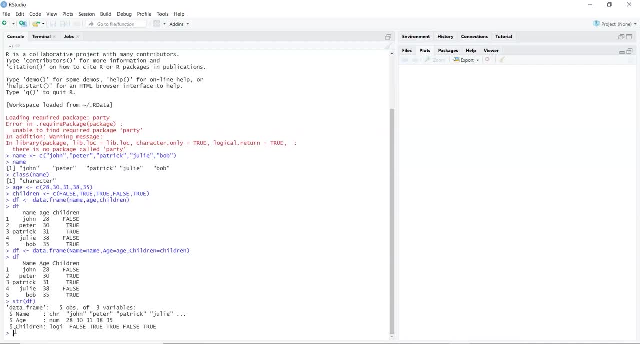 And in this case This is a list with three elements, So each list element Is a vector of length, phi, Corresponding to the number of observations. If we create data frame with vectors Not of same length, We would get an error. 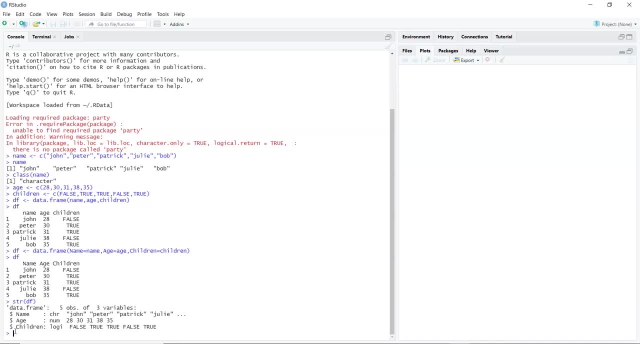 Now here, When we look at our data frame, We know that name is a column. So name column, Which is character, Is actually a factor Instead of character. To suppress this behavior, We can always use a property That is strings as factors. equals false. 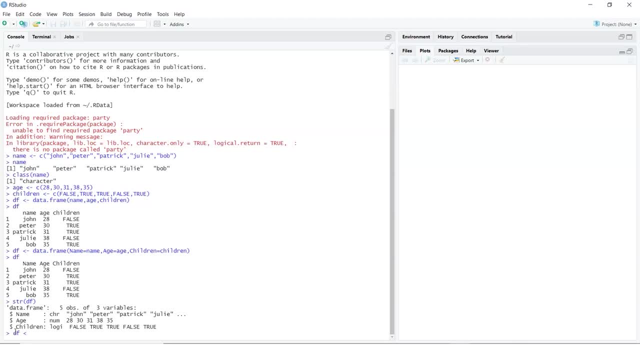 So what I can do is I can do a data frame Like this, Use my data dot frame function And then basically We can pass in our vectors, That is, name, Age And children, And then what I can do is: 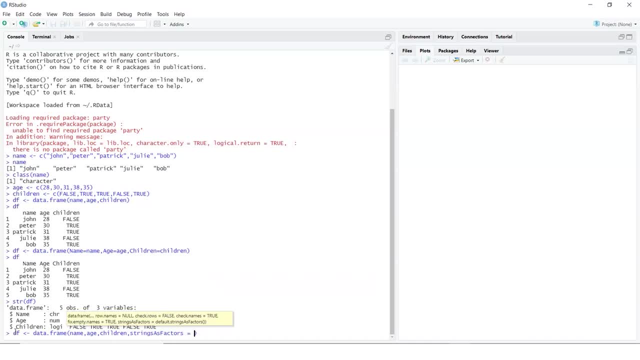 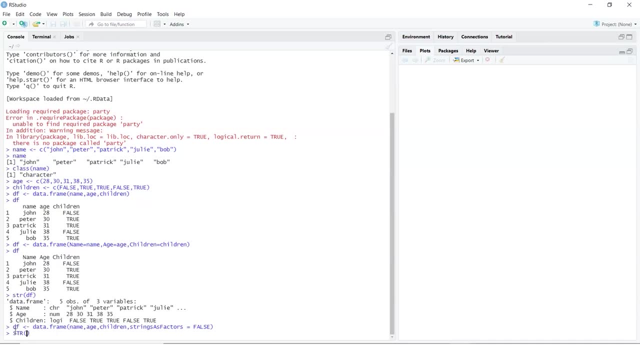 I can say strings As factors And set this value to false. So if I do this, And now, If I look at my data frame structure, Sorry Yeah, Now let's look at this one. And this one shows me. 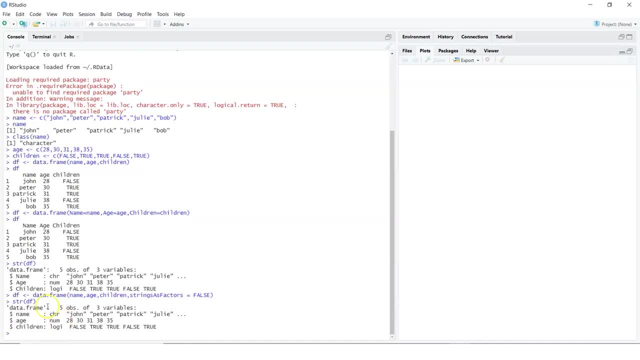 That, Unlike your earlier one. Now we are creating a data frame Where our name Would be Containing Characters. Earlier, also by default, It was showing us character Usually, if you, Because this value by default Is set to false. 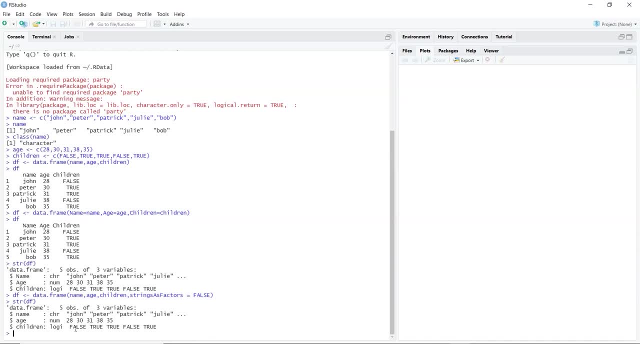 Or It would have created Characters Or factors, As we say. Now, how do we do A subset And extend And sort Data frames In R? So As we have learned So far In brief About your 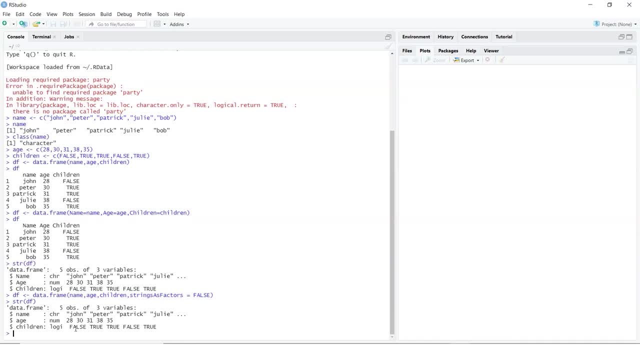 Data frames. So Data frame Is somewhere Like an intersection Between matrices And lists. So If you would want To subset A data frame, We can always use The square Brackets And in that We can use. 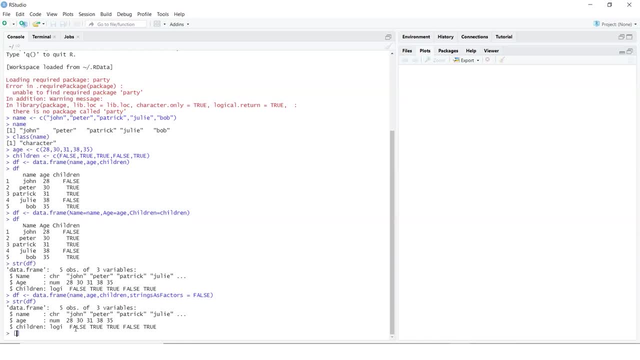 The single Square Brackets Which are From matrices, Or We can use Double Square Brackets From list, Or We can also use The Dollar Symbol. So Let's use Our data frame. 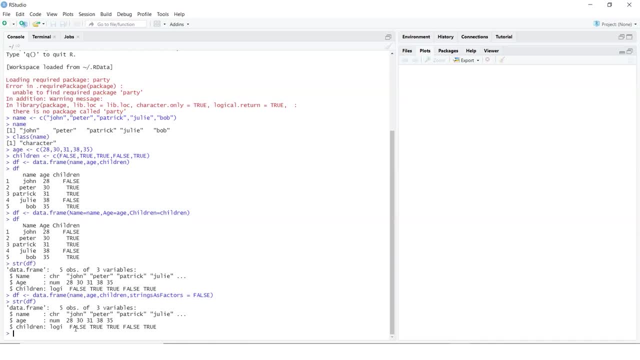 Which contains Information About people, So We can Select Single element From our data frame. So Here What we can do Is We can just say D, F, And then I can use A single. 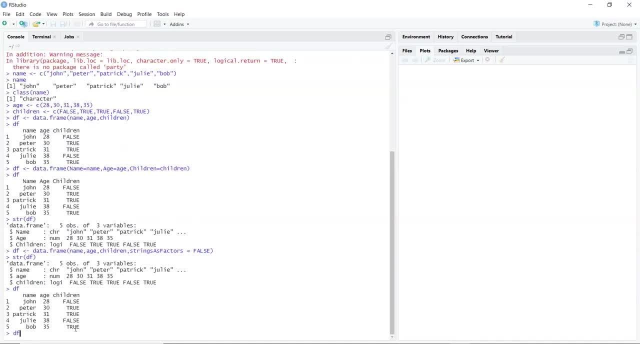 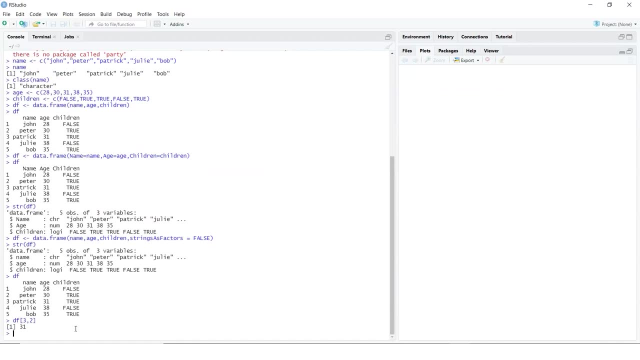 Bracket And I can just Do a Three Comma Two, So It would be Good That We Are Using The Row Index First, Which is Number Three, Which Shows: 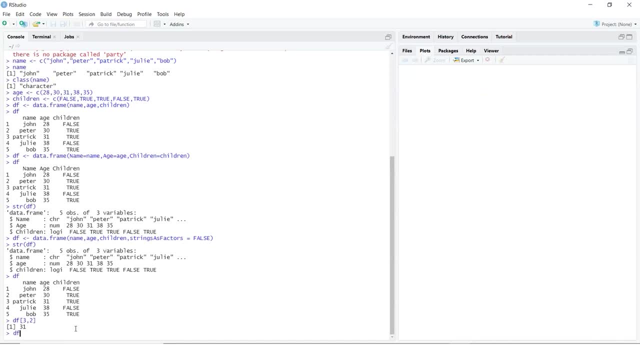 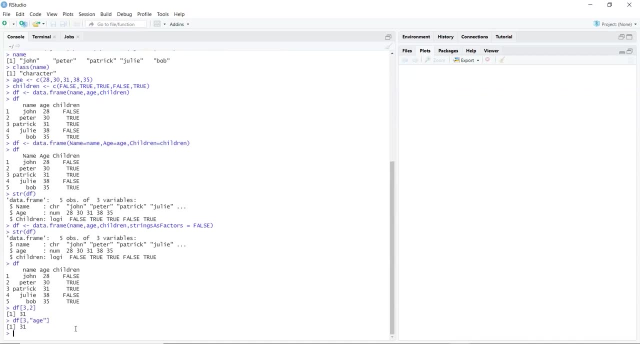 Me That We Would Be Going To The Row Number Three And Then We Point Or One Of Two Indices To End Up With Entire Row. 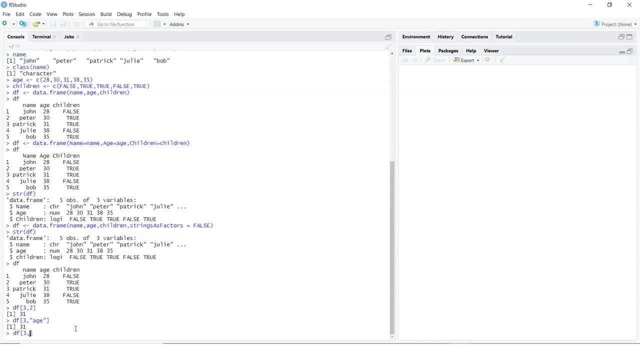 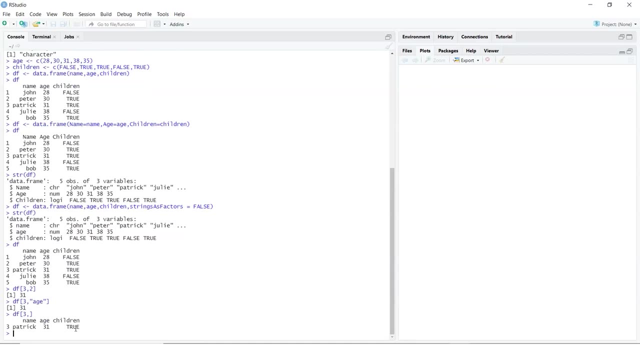 Or Entire Column And, For Example, If We Would Be Interested In Looking For Information For Patrick. What I Do Is To Be A Way To 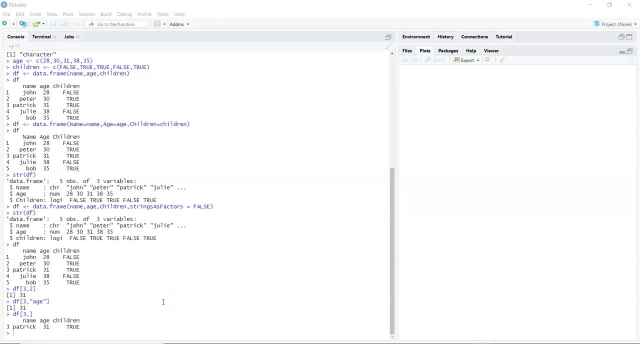 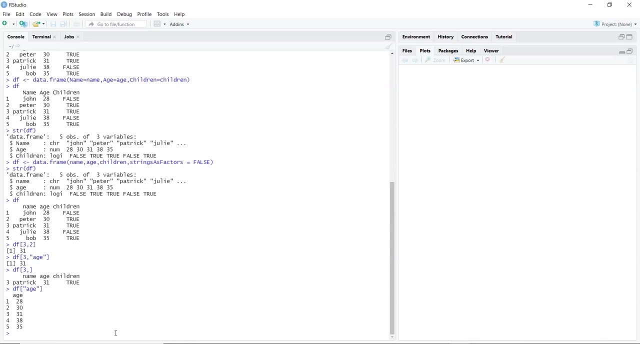 Store Different Data Types, And That's Why The Result Is Also A Data Frame. What We Can Also Do Is To Get The Results From: 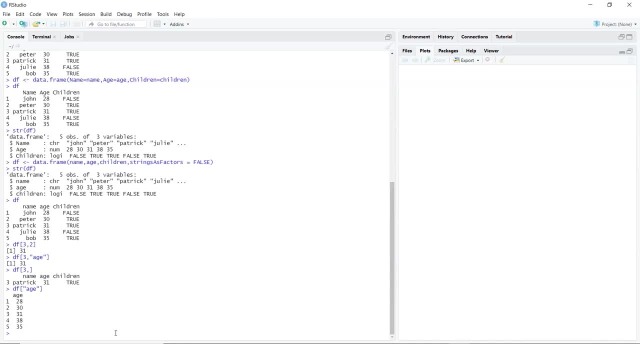 The Data Frame. Now We Have A Data Frame That Is A Data Frame That Results In A Data Frame And Contains Multiple Observations. Can 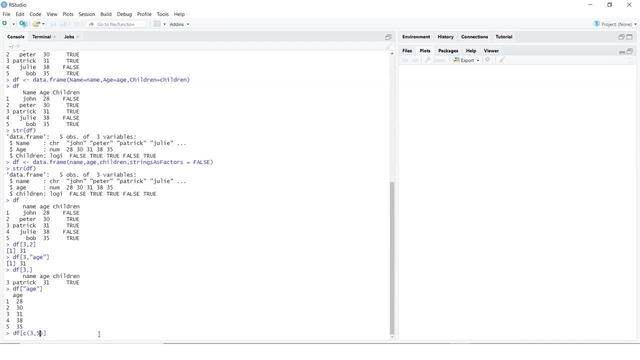 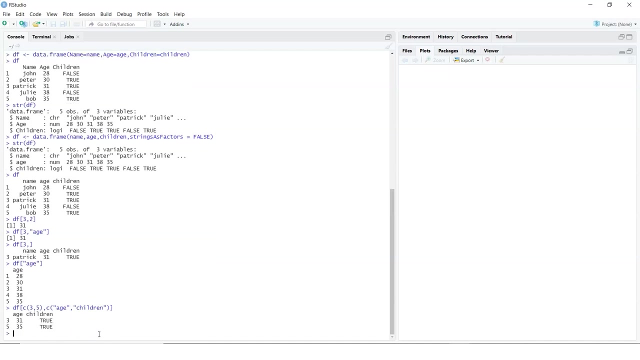 Also Be Three, Five, And Then I Can Just Say Age And Children, For Example. So Let's Say Age And Children And I Can Be. 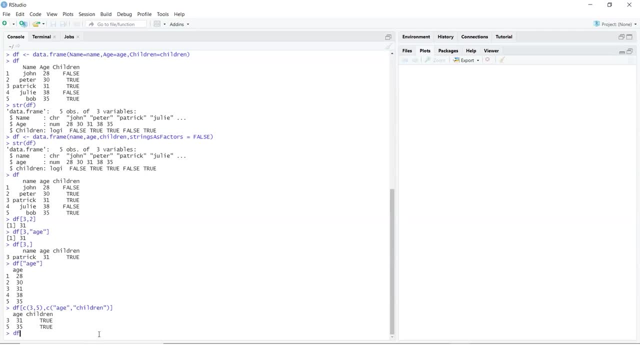 Pulling Out The Values In This Way In The Column Number And That Also Gives Me The Age Column. Now We Know Data Frame Is. 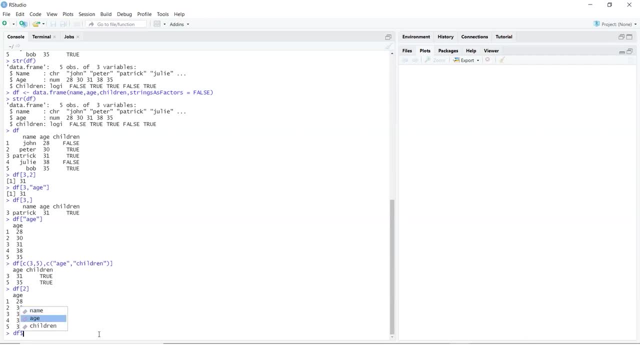 A List Containing Vectors Of Same Length. This Means We Can, As I Mention Earlier, And Pass In The Column Name. So That's Also. 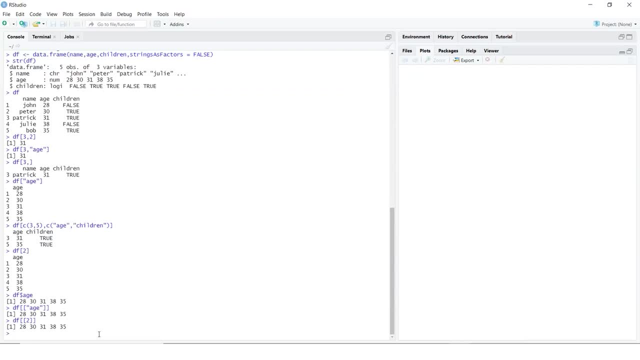 Fine, Or You Can Give A Column Number, And That Also Would Work. And In All Seeing, Here Is A List Which Contains Only Age Column. 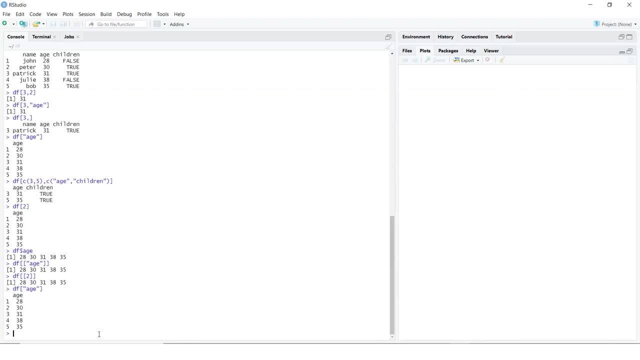 Having The Data Elements. So These Are Different Ways In Which You Can Do A Sub Setting Of A List, That Is, We Can Add Variables. 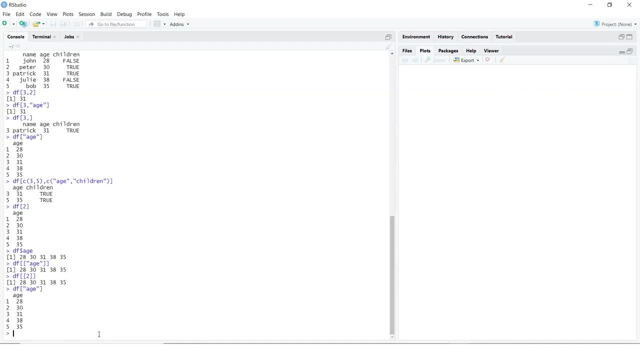 We Can Add Columns, That Is Adding Variables, Or We Can Add Rows, Which Are Nothing But Observations. So Adding Columns Is Create A Vector. 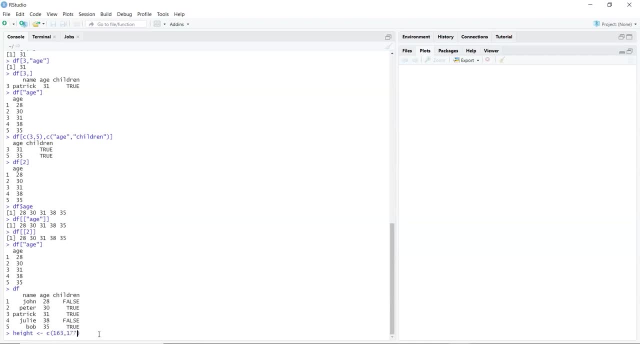 Here, And This One Is What I Would Want To Add For Each Person. So Let Me Do This And Let Me Pass In Some Values. 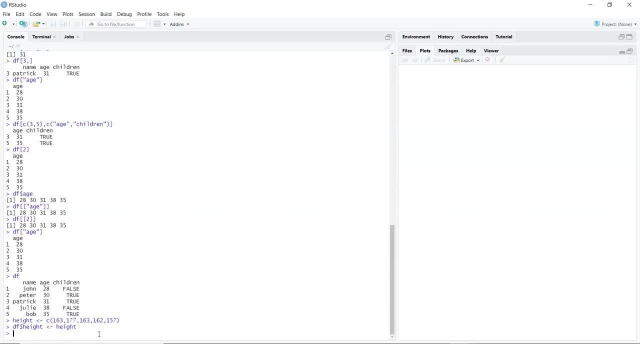 And Then I Will Pass In This Vector Here And Now. If I Look At My Data Frame, You See The Fourth Column Has Been Added. 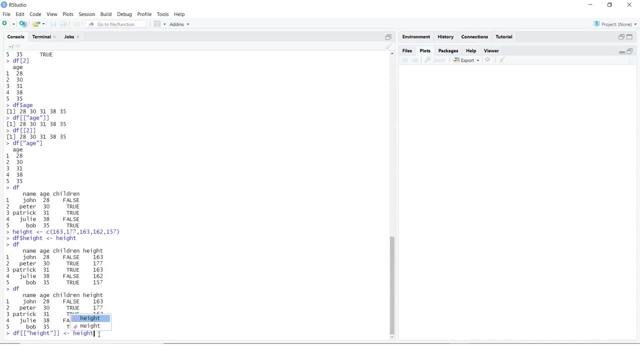 And That's My In This Way, However, So This Is Also One Way Of Doing It. We Have Already Added The Column, So We Don't. 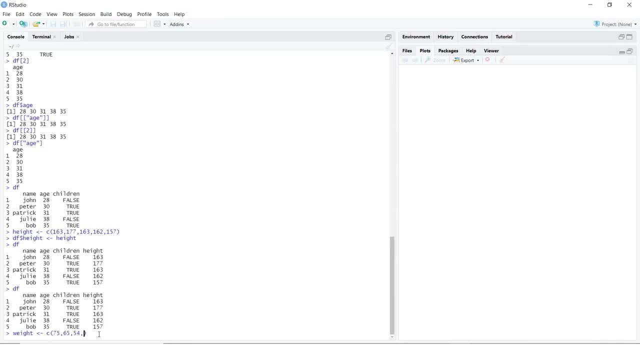 Need To Repeat The Step. Now What? These Are My Values Of Weight. Now, What I Can Do Is I Can Just Do A C Bind. 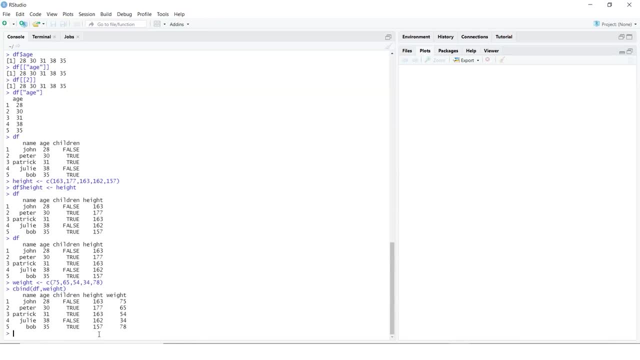 And Then Pass In My Data Frame And Then Pass. We Need To Create A New Data Frame With One Single Observation. Remember Row Will Have. 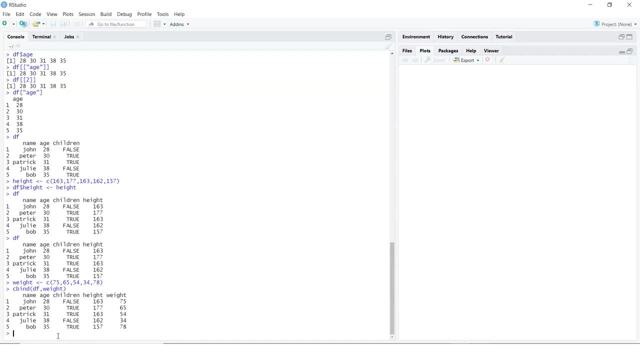 Values Of Different Data Types. So We Cannot Create A Vector, We Have Function, And Then Let's Give Name. What We Can Do Is We: 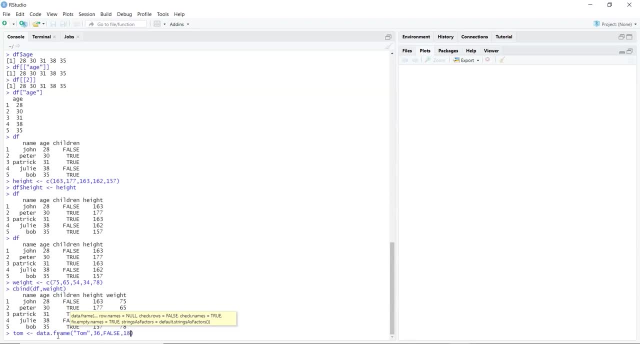 Can Give Age, Then We Can Give The Logical Value, Then We Can Give, Say, Height, And Then I Can Pass In My Data Frame And 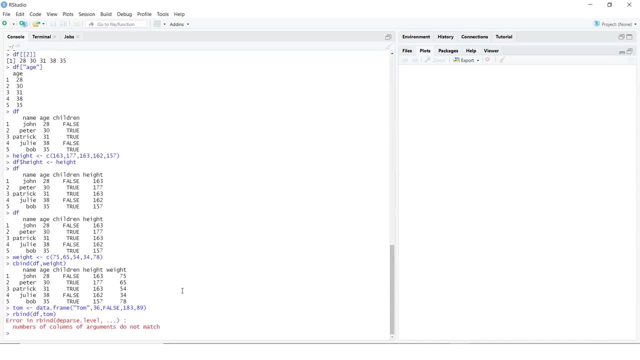 This Tells Me That The Number Of Columns Of Arguments Do Not Match, So We Will Have To Check This. Let's Do A R Bind. 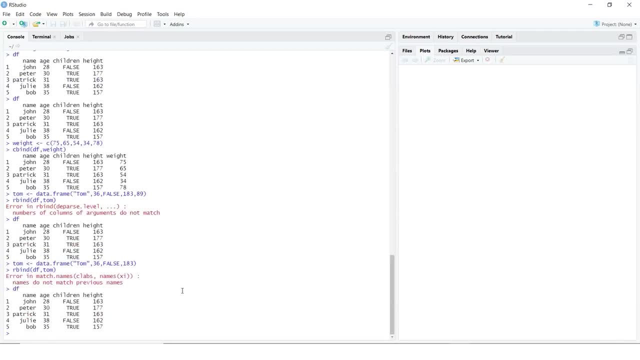 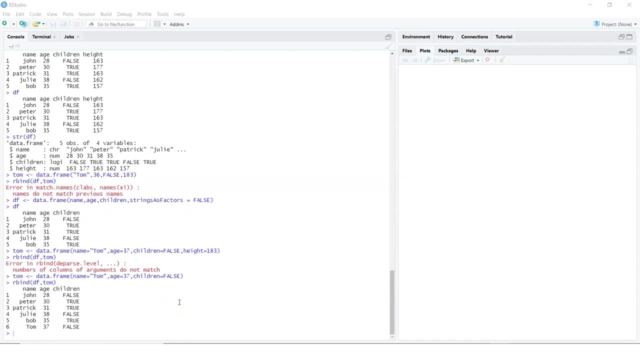 And Let's Again Check What Is The Reason Here. So This Is Height And Let Me Just Check This. So To Look At This, This 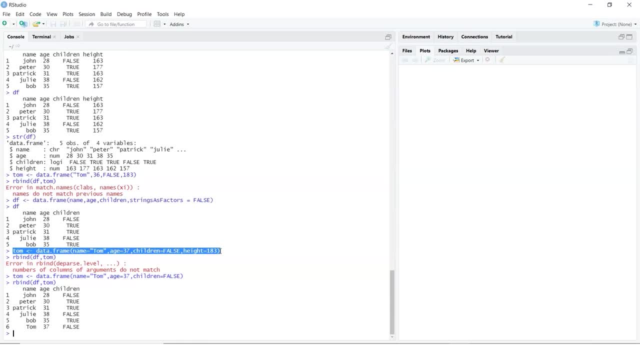 And See, Mind Was Showing Us The Fourth Or Fifth Column, But The Original Data Frame Only Had Three Columns, So What I Did Here Was 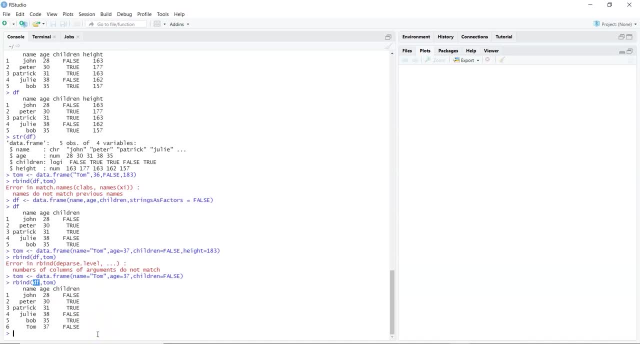 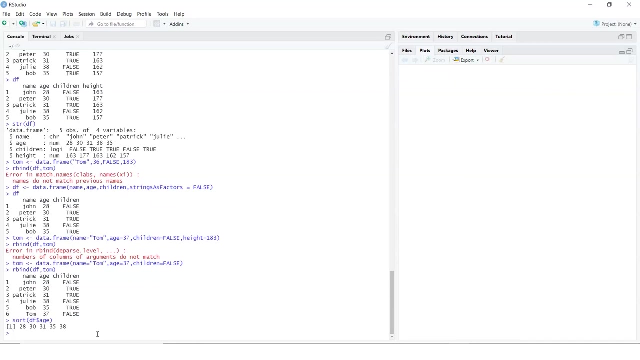 I Did Tom Bind, And Our Bind Was Used To Add A New Row To Our Data Frame. Now, When It Comes To Sorting Or Ordering, 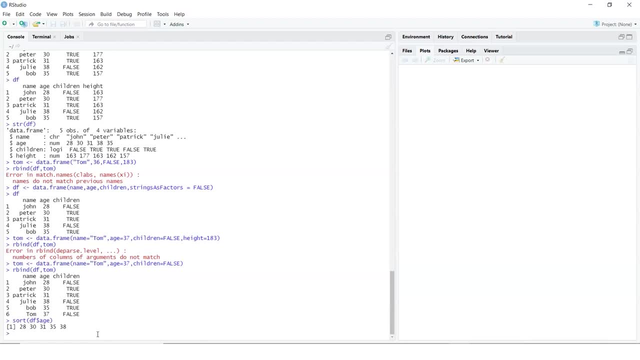 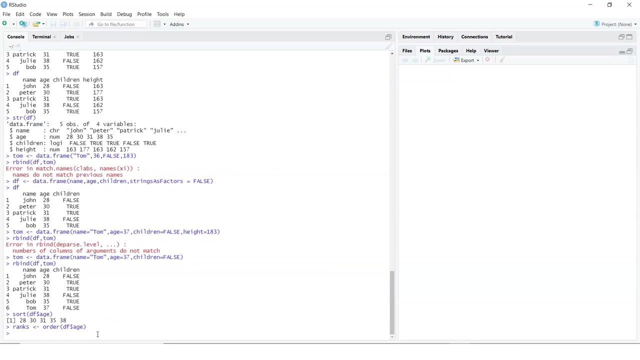 Your Data Frame. Say, For Example, Other Clear Way Of Doing That Would Be Using Ranks. So, For Example, If I Do A Ranks And 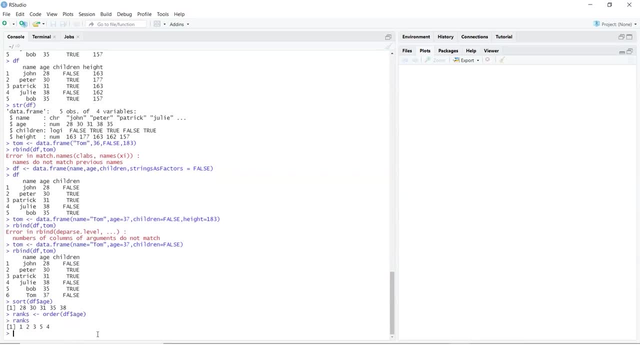 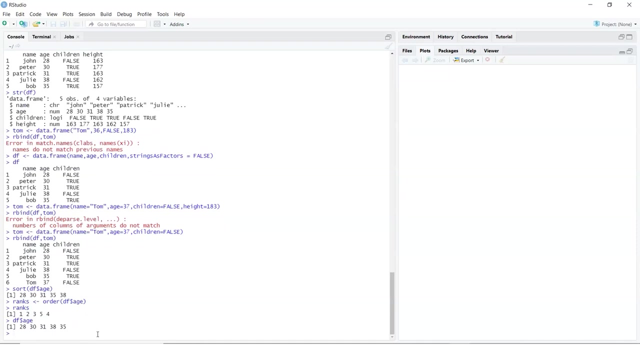 Instead Of Doing A Sort, I Would Use Order, And If I Do A D F Dollar Age, It Shows Me The Values. And If You, 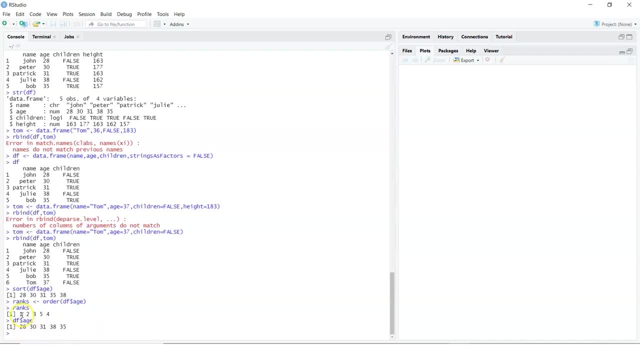 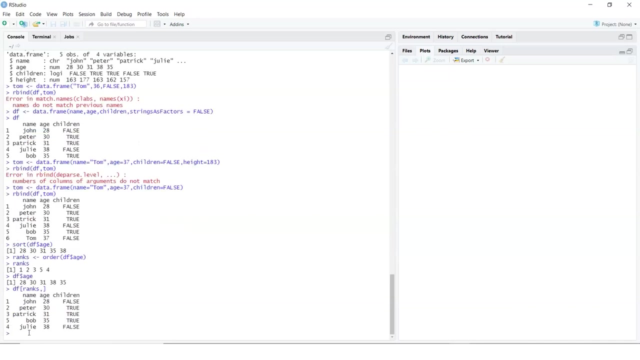 Look At The Ranks, It Will Tell 21.. Or Here The Lowest Value Is Basically Use Ranks And We Can Just Look At The 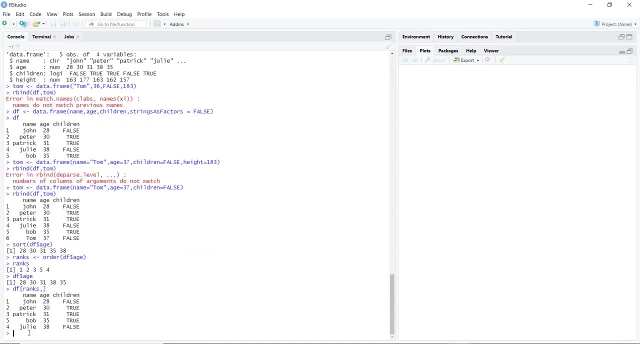 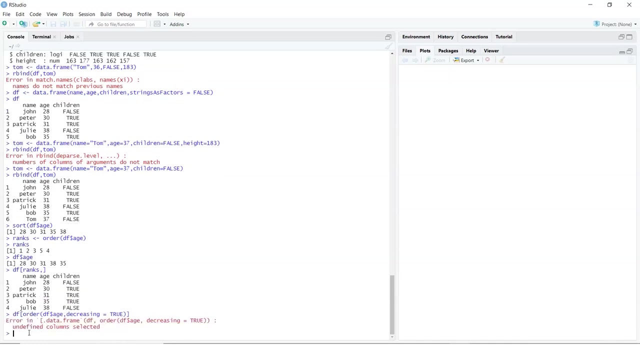 Result. So This Shows Data Frame, Which Is A Order Data Frame, Now Based On Ranks. Now, If You Do This, And Here This Could 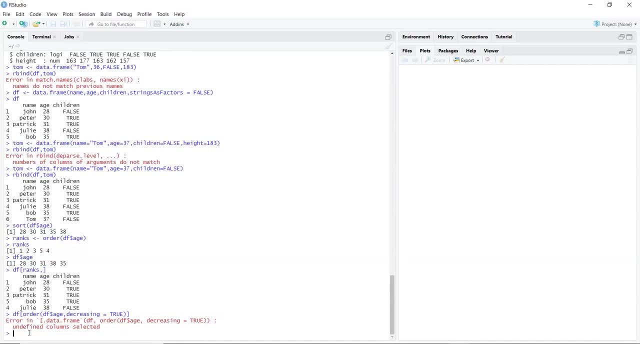 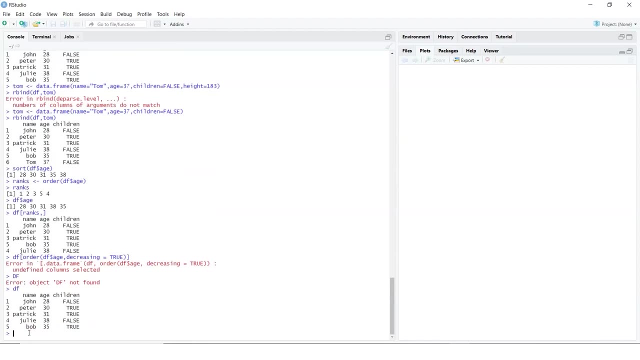 Show Me The Value. So It Says Undefined Column Names. So What I Would Have To Check Is: What Is My Data Frame That Was Showing? 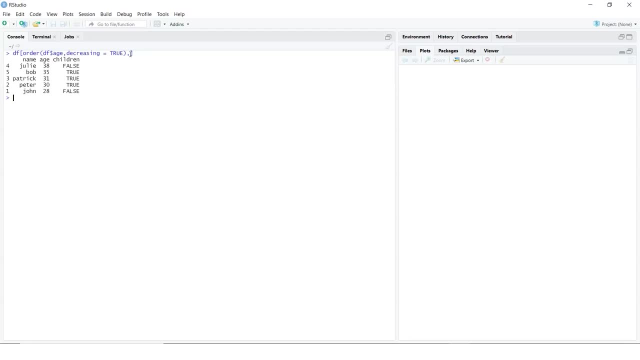 An Error, So Now We Can Have The Data Ordered In A Descending Way. So There Are Dozens Of Packages, Such As Deplier Data. 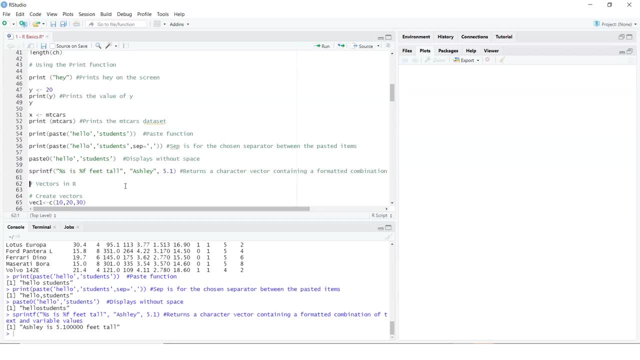 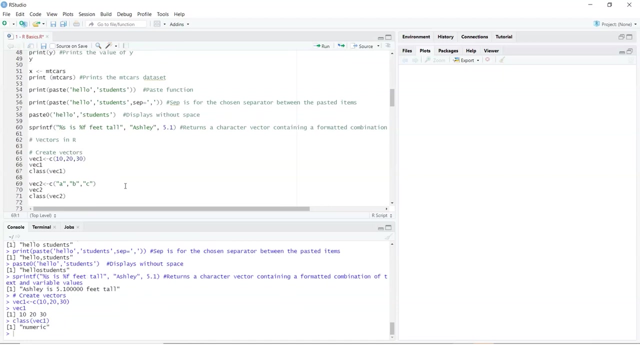 Table Which Object In Your R Is Vector, And That Really Helps Us In Various Ways. So Let's See How We Work On Vectors Here. 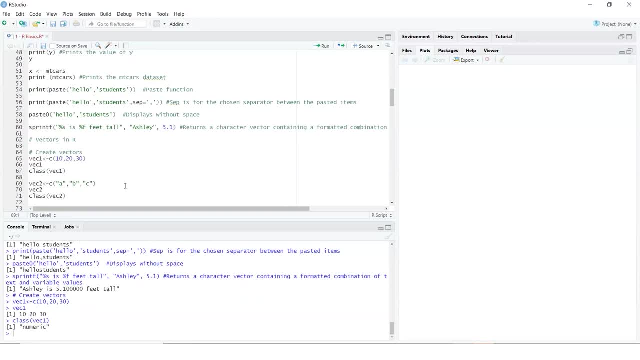 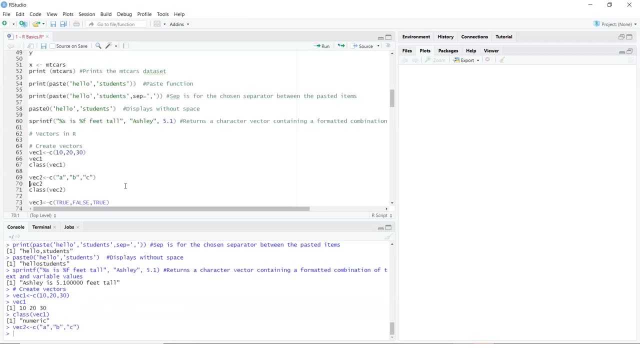 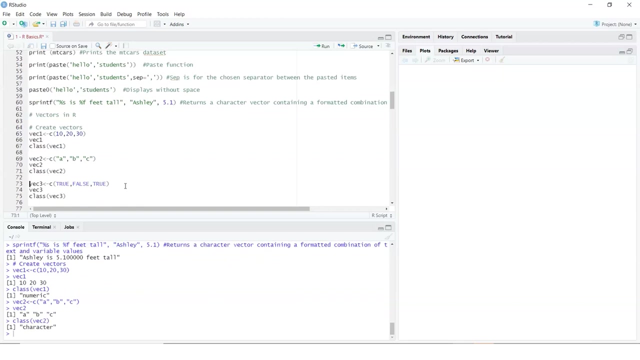 So To Create A Vector, We Can Say: Or Belong To The Same Class, We Can Say. So Here We Are Creating A Vector. Looking. 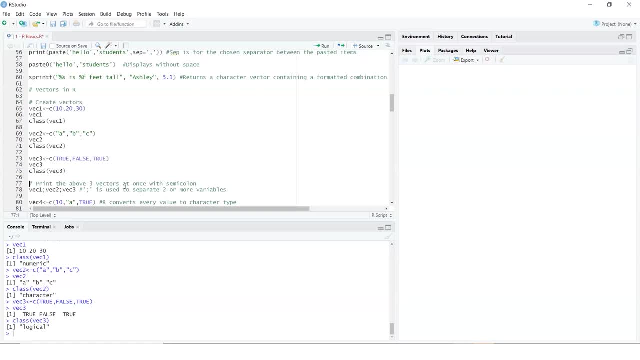 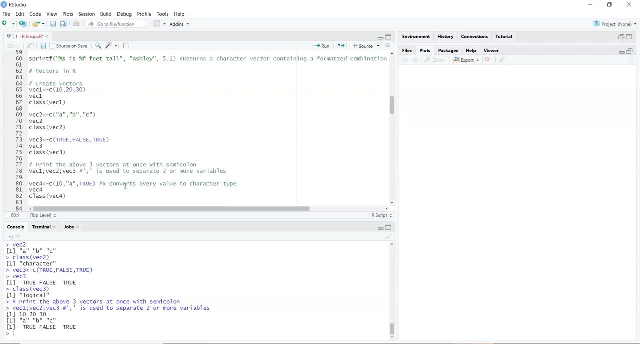 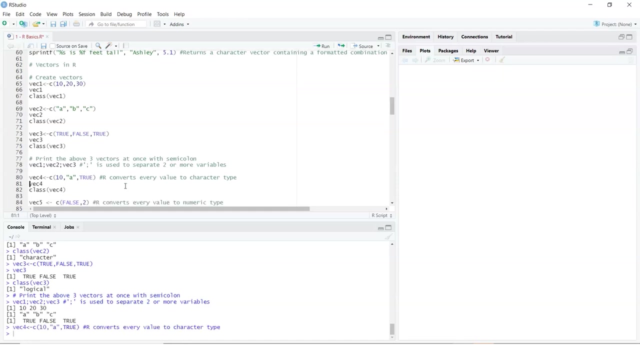 At The Value Of It And Then, Looking At The Vector, We Can Separate Two Or More Variables And We Can Pull Out The Values Of. 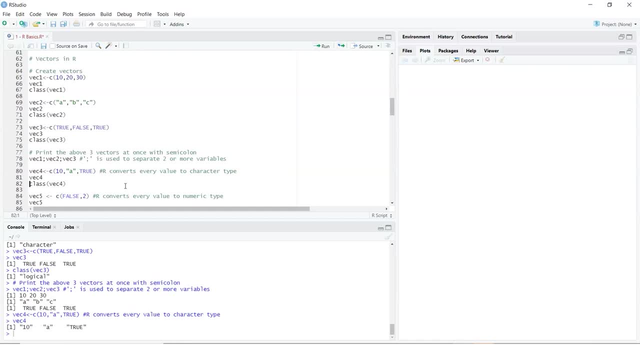 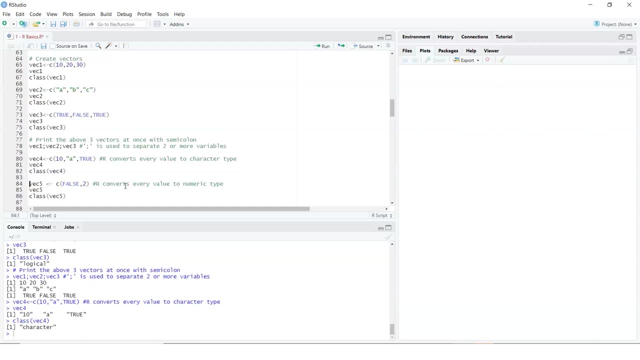 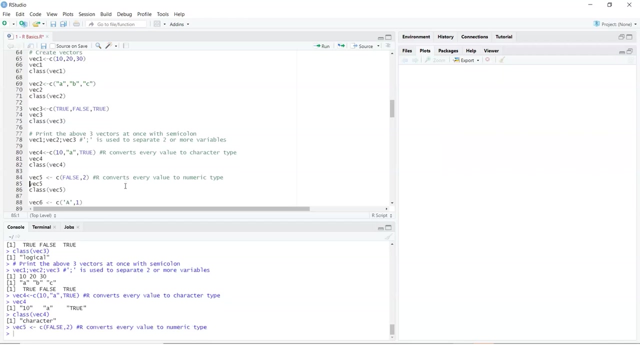 All The Vectors Which We See Here. Now, What Happens If We Pass In Values, Where In We Can Pass Logical And Numeric, And In 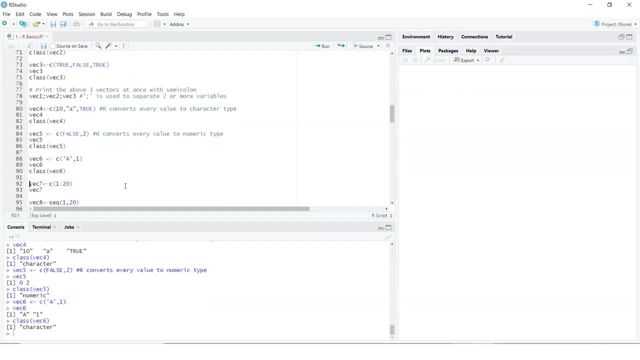 This Case, It's Not Going To Go For Character, It Is Going To Convert Everything Into Numeric. There Is One More Way Of Creating A. 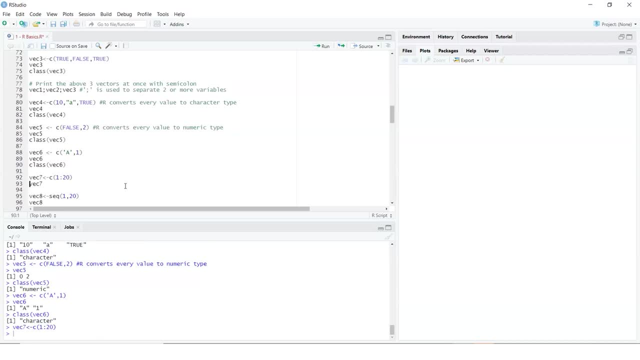 Vector, And That Is By Providing A Range To Your C Function. So We Can Do That Here Where In I See Function And I Can. 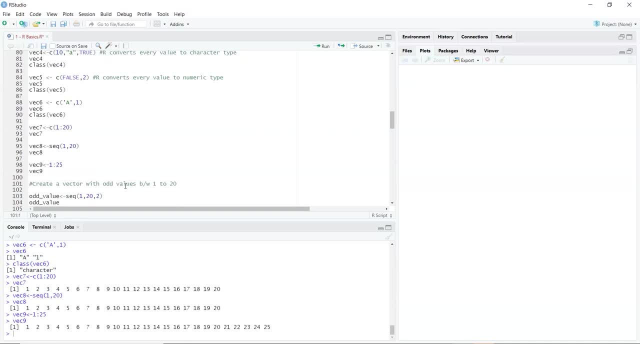 Straight Away, Pass A Range- And That Is Also Fine- To Create Our Vector Starting From One Ending At 25.. So What If I Have? 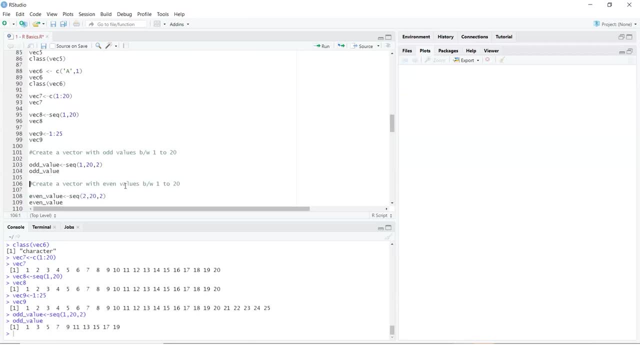 The Ending Number, And Then The Skip Or The Jump. And Now, If You Look At The Values, It Shows Me Only The Odd Values. Well, 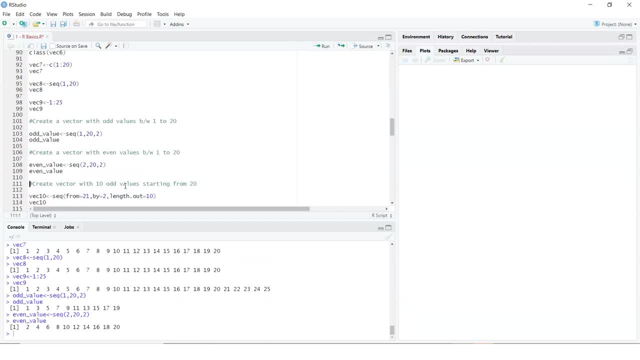 You Could Having Odd Or Even Values. Now What If You Want To Create A Vector With 10. Odd Values Starting From 10. So You 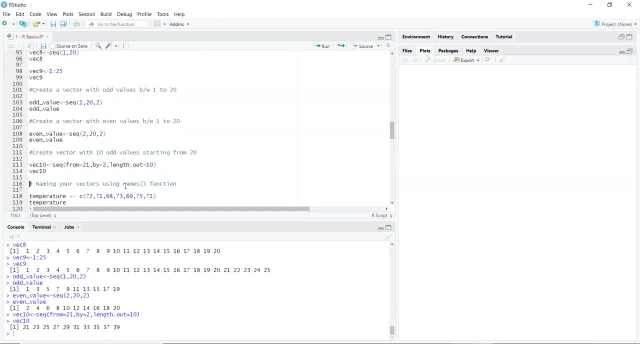 Are Basically Giving A Length. So If You Want To Create A Vector With 10. Odd Values, Now, One Of The Requirements Is Always To 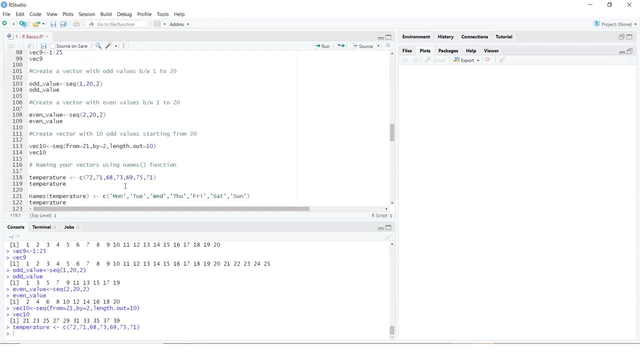 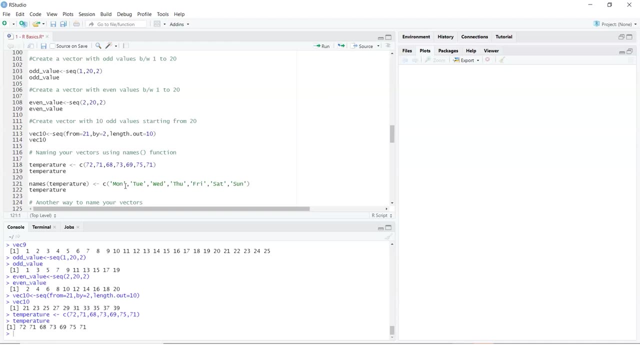 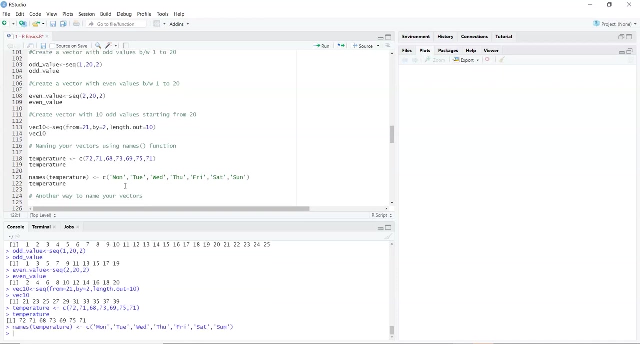 Name The Values So That We Can Access The Values, Which Makes It More Readable, More Accessible, So I Can Use The Names Function Pass. 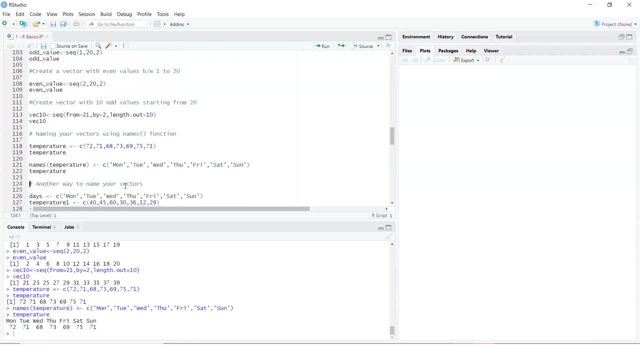 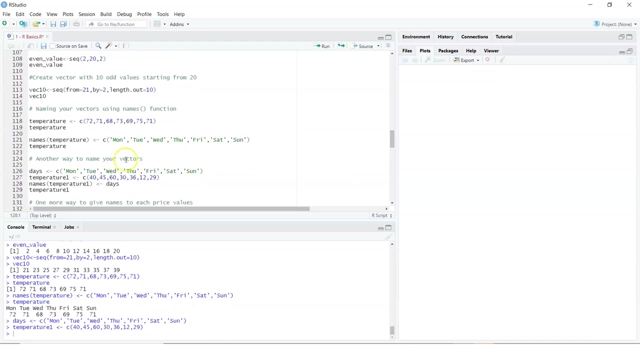 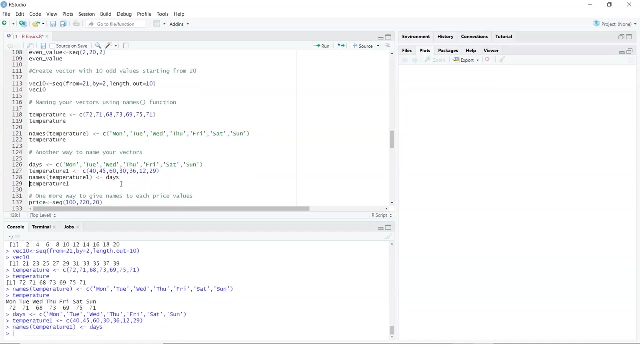 In My Temperature As A Vector To Names Function And Then Assign The Names To Our Existing Vector. So If You Do This, So You Are. 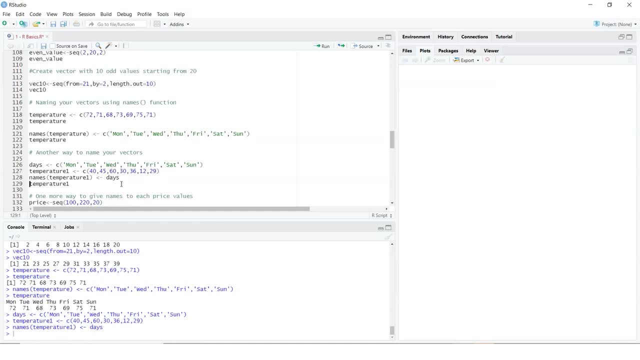 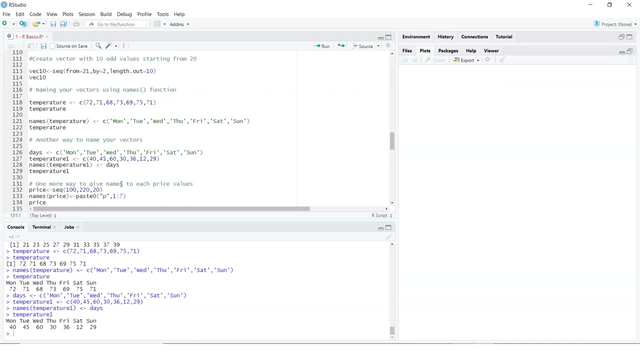 Assigning The Names Vector To The Temperature One, And Now Look At The Values. It Still Does Use Your Sequence, So Here I'm Creating A. 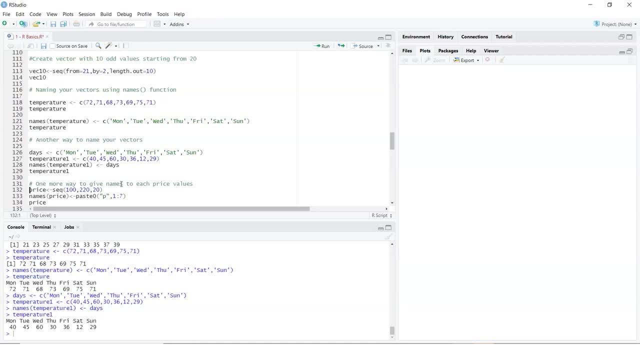 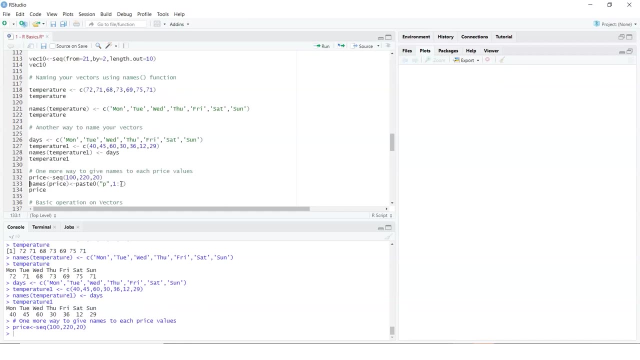 Sequence Which Starts With 100.. And Said To 2020.. With A Skip Of 20. Values, Or Every Jump Would Be 20. Is Zero. 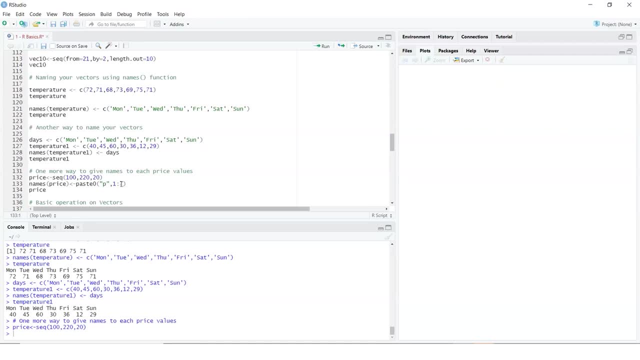 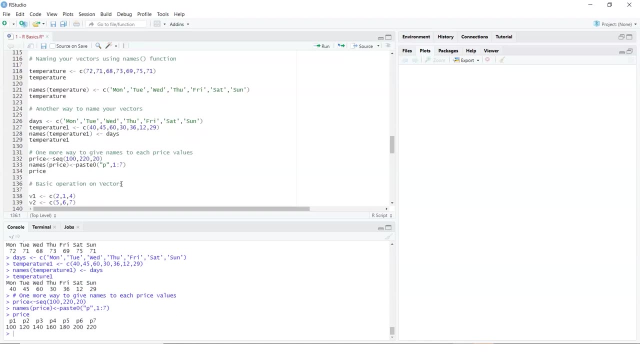 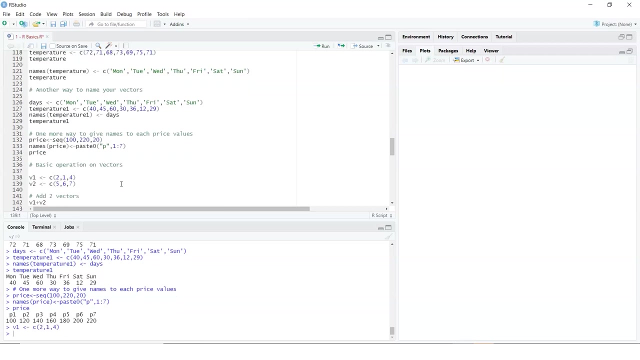 Basically Skips The Space, And We Are Going To Assign Those Values To As Names To Price. And Now Let's Look At Our Price. So 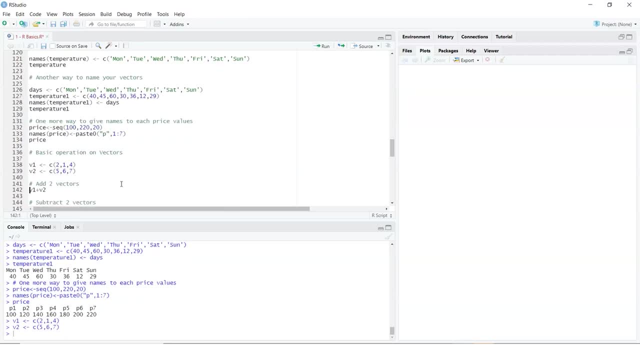 That Basically You Can Simply Do An Edition On Two Vectors Where Each Element Is Getting Added To Other Element Of The Vector. You Can 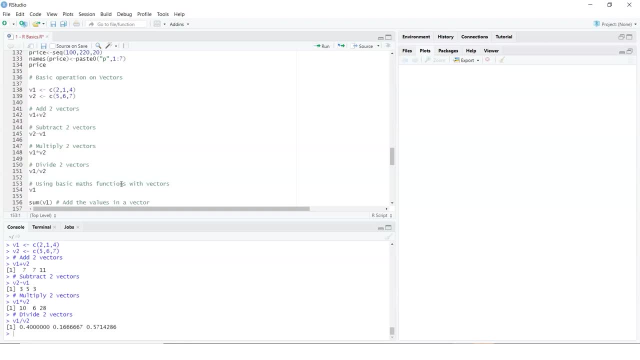 Subtract Two Vectors, That Is Element. Now Let's Do A Sum Which Sums Up All The Elements. Let's Find Out A Standard Deviation. 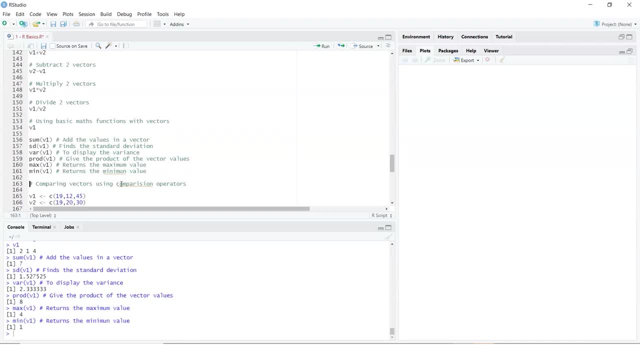 For All The Values. Let's Find Out The Variants For All The Vectors Using Comparison Operators, And This Is Where I Create A Vector. 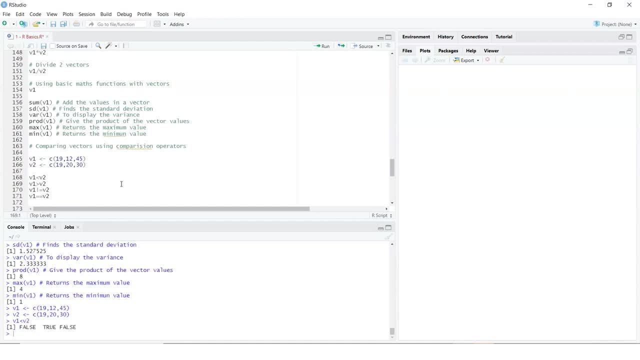 One, Create A Vector Two And Let's Find Out The Values In V1. Which Are Smaller Than V2.. So These Are Some Simple Comparison. 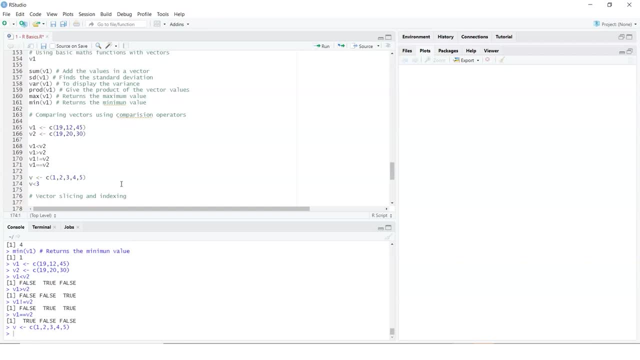 Examples. Now I Can Create A Different Vector And Then I Can Find Out Individually If The Elements In The Vector Are In Vector And 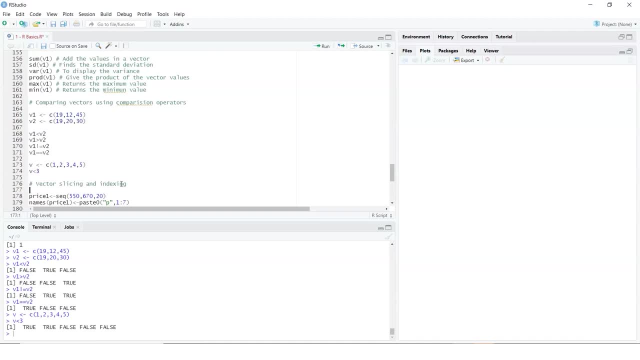 This Is Very Much Important When You Are Storing Your Data In Vectors. How Do You Access Them? So Let's Create A Vector Using 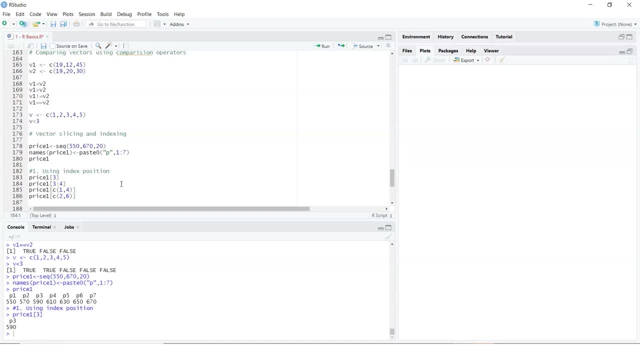 Sequence. Let's Take Other Programming Languages, Like Python, Where Indexing Starts With Zero. Now I Can Also Get The Third And Fourth Value By Doing: 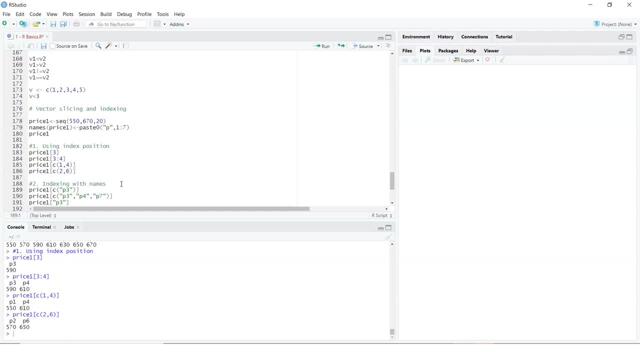 A, Three, Colon Four. I Can Use Names To Every Element, So I Can Use C Function, Pass In The Name And Look At The Value. 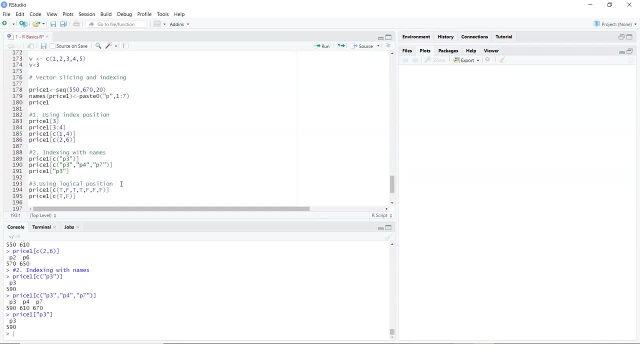 For That Particular Name Or Selectively Select. Different Columns Exists, And We Can Do That Or Using True And False, And Then Look At The 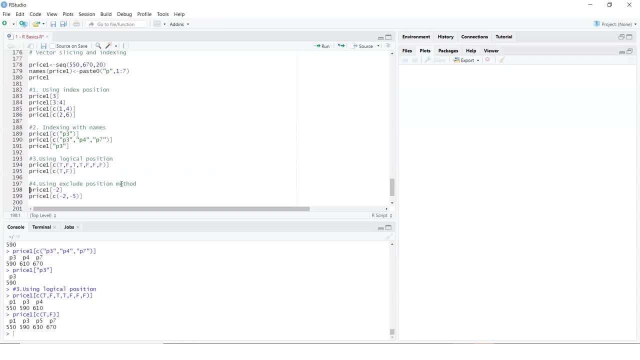 Values. So There Is One Useful Way Where You Can Exclude A Particular And We Can Exclude Particular Values From Our Vector. Now How Do 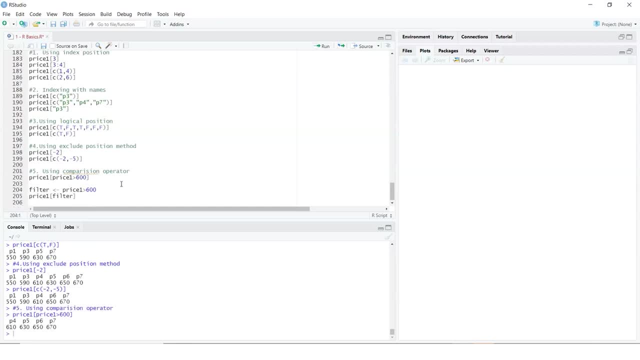 We Do A Comparison Operator On The Values Of Vector So You Can Just Say: Price One Value And You Can Use Your Values To Manipulate. 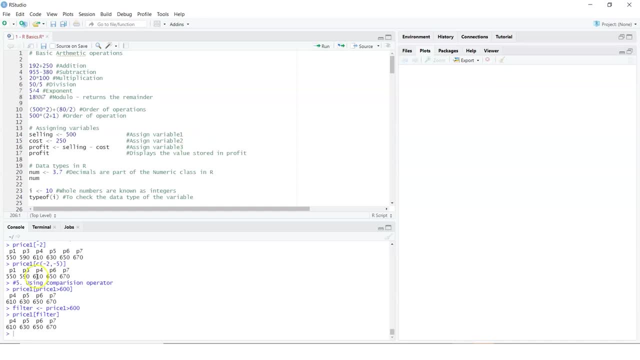 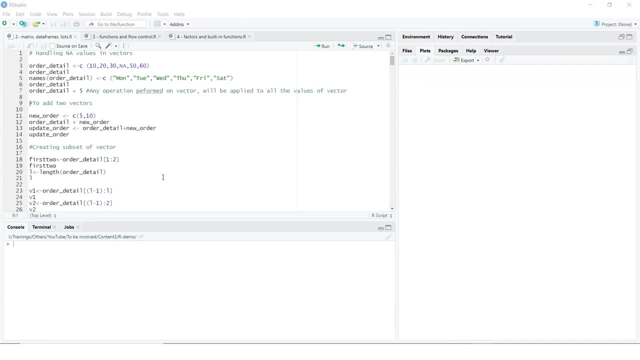 And Extract The Data, Use Your Different Logical Operators Or Other Operators And Perform Your Basic Easy Computations. Now, That Is Assigning A Vector To 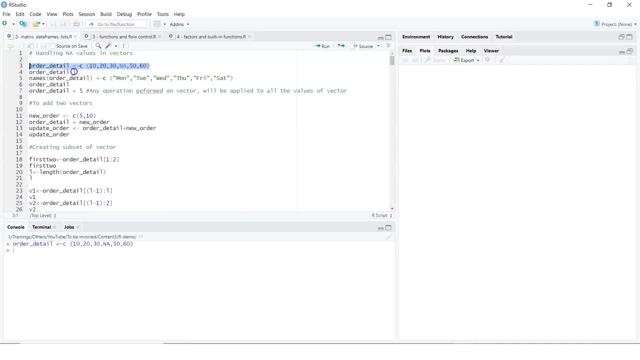 A Variable Order Detail, And This One Has A Missing Value. Now Let's See How This Is Handled And You See All The Values. So 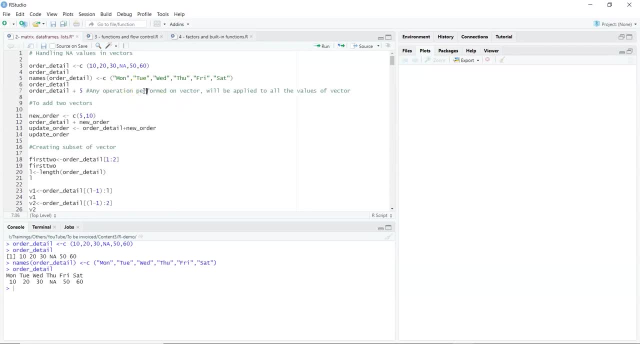 What We Can Also Do Is We Can Perform An Operation On A Particular Vector Which Will Be Applied To All Values Of The Vector. 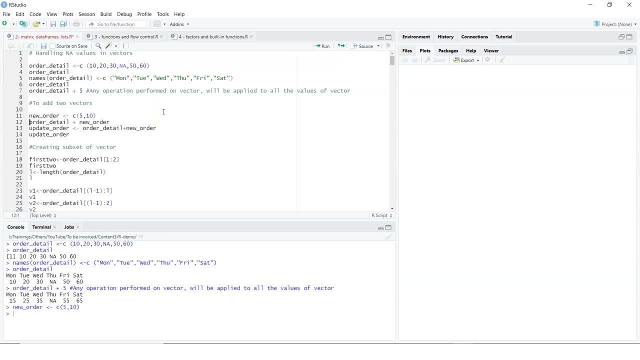 So, For Example, Let's Add It To Order Detail. Now, In This Case, What We Are Doing Is We Have A Vector Which Is From 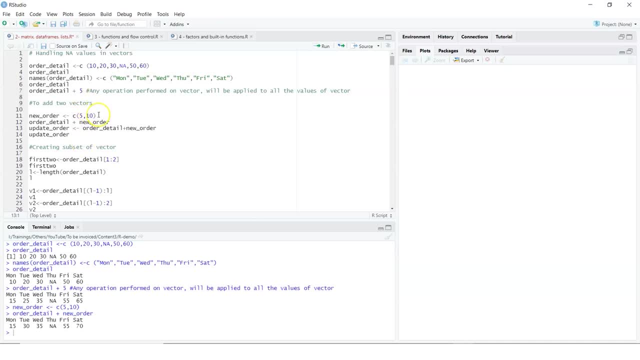 5. To 10. And What We Are Adding To 10.. And Then Your Value 10. Gets Added To 20. And Then You Have 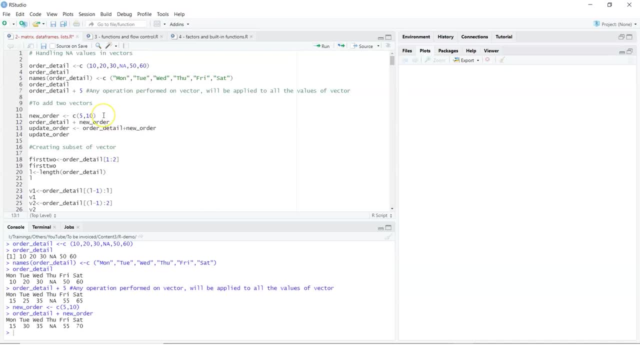 Again 5. Which Is Added To 30. Now You Can Add In Anything By Doing This. So I'm Creating An Update Order And Now 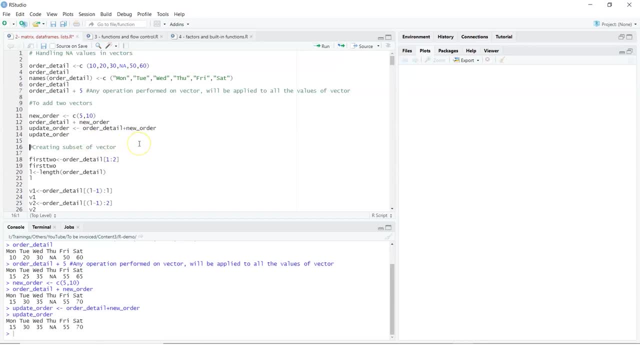 Let's Look At The Value Of Update Order. What Does It Show? So You Are Basically Doing The Look At The Value Which Is Assigned. 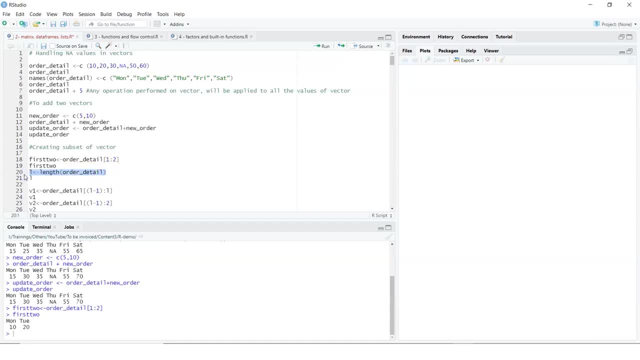 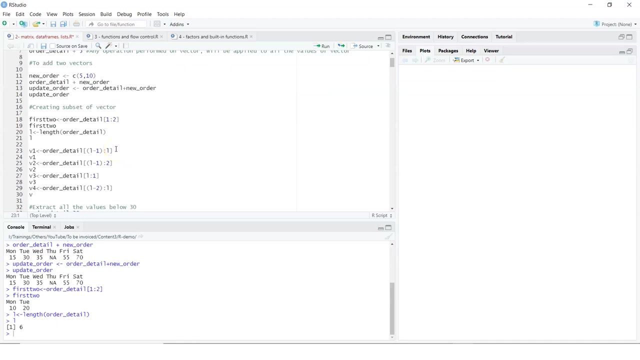 To First To. We Have Just Sliced And Added A Subset Of Vector To This One And If I Would Want To, And Then Up. 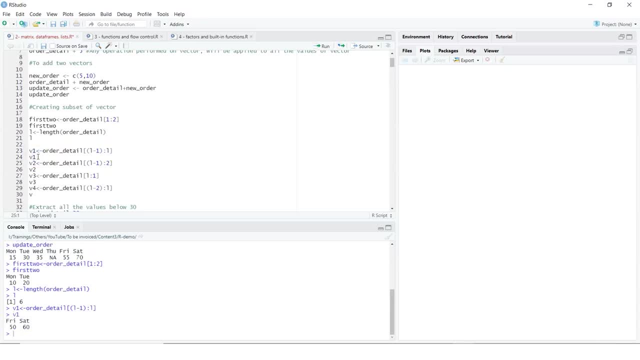 To The Length. So Let's Do This And Let's See The Result Of This. So What We Have Done Is We Had Our Order Detail. 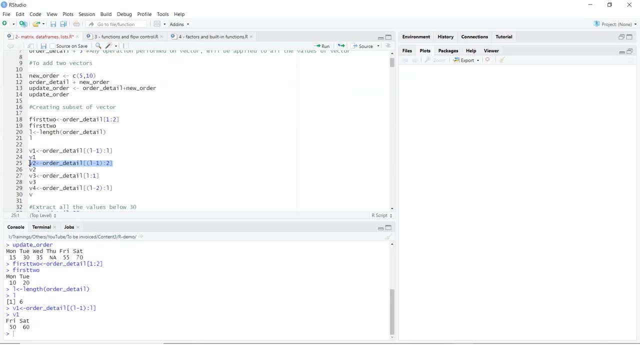 Which Length Minus One And Two Elements. So I Can Do This. And Now Let's Look At The Value Of V2.. So This Shows: 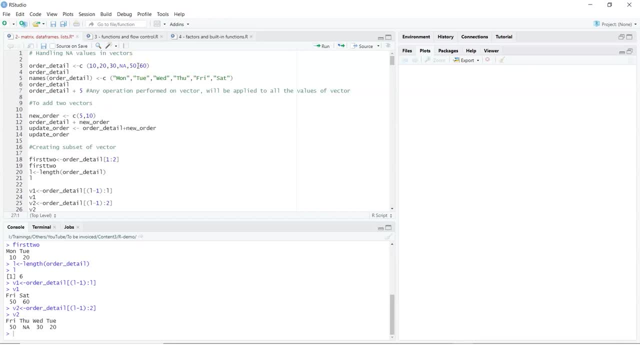 Me The Value Where You Are In Index Position. Similarly, We Can Use The Length And We Can Take It From This Element And Let's 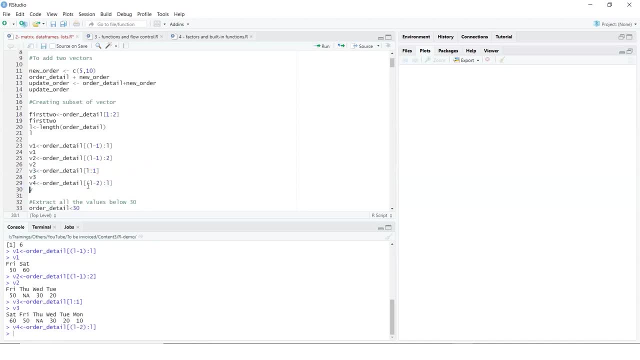 Look At The Value Of V3.. So That Shows Me That Is The Value Of V1.. Now You Can Extract All The Values Below 30.. 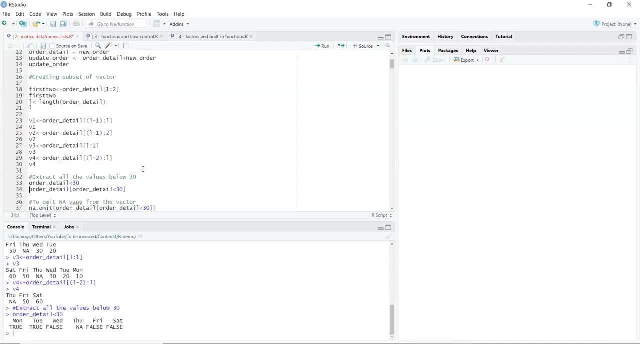 And This Is Where You Are Doing A Comparison. So You Will Take Your Values. This Will Show Me The Actual Values. Here We Were Just 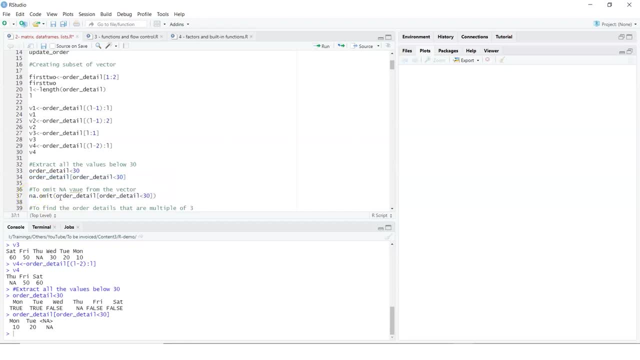 Getting The Logicals, But Here We Are Getting The Values Now To Omit Any Value From The. So You Can Do Something Like This: You. 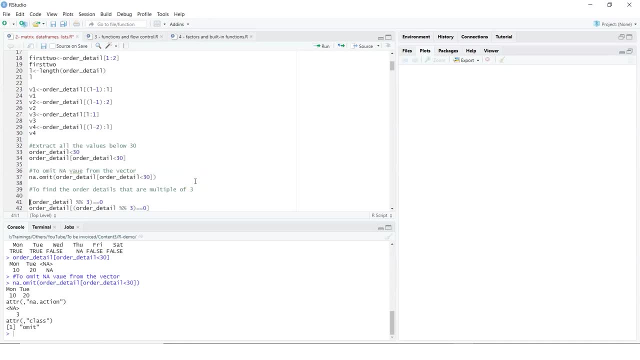 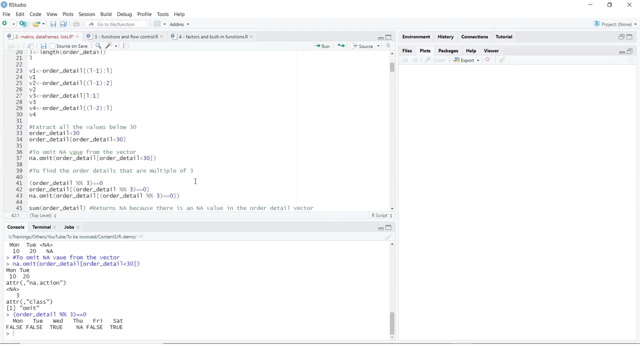 Can Look At The Values. What You Can Also Do Is You Can Find The Order Details That Are Multiples Of Or, If You Would, 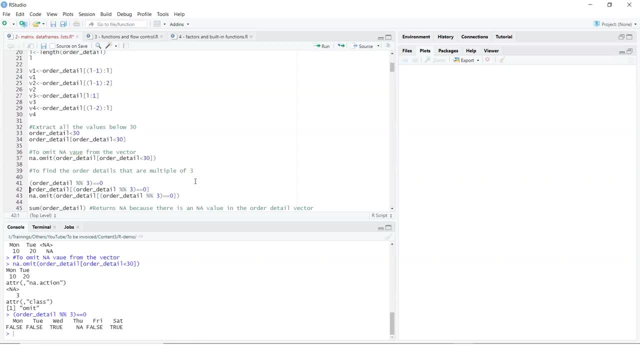 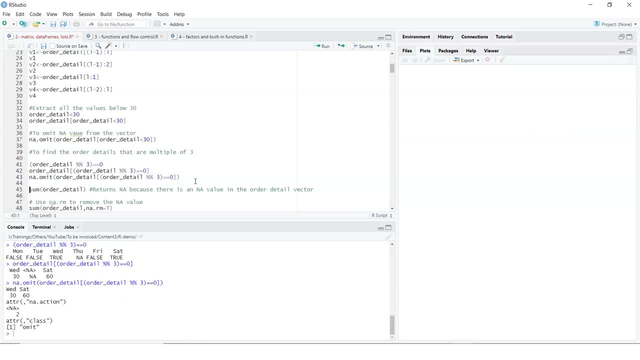 Want To Look At The Values, Then You Can Say Order Detail, Open Up A Square Bracket And Then Pass In Your Condition. Now We Have. 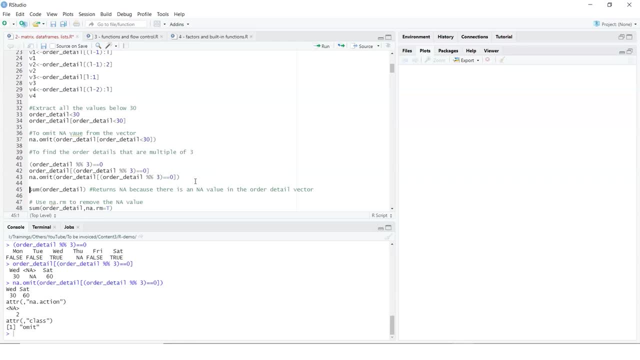 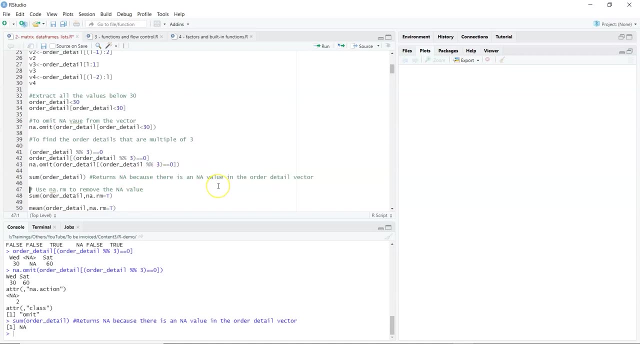 A Data Extraction. Now I Can Also Use A Sum Function. Now, If We Do This, It Returns Any, Because There Is Already A Missing Value. 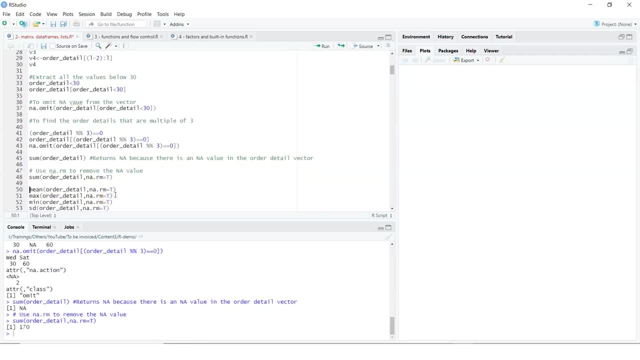 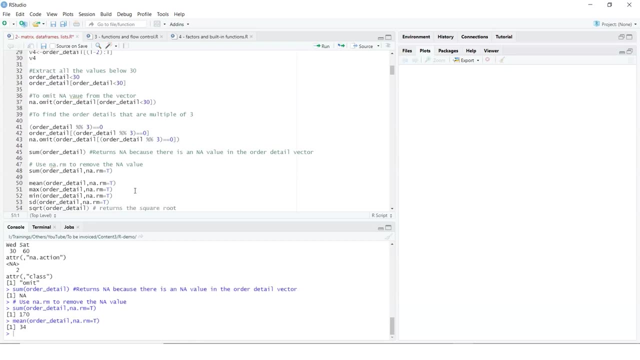 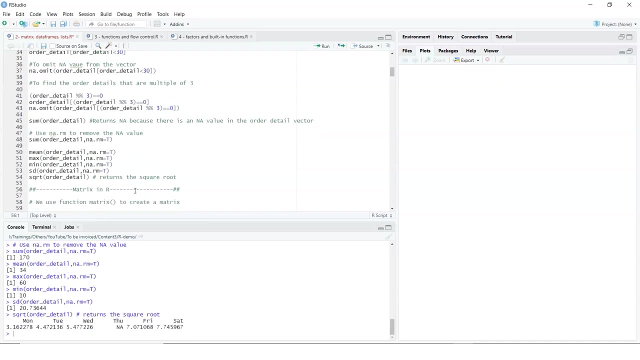 And You Enter Any Value, So I'm Giving It A Value As True, And Then, If I Do, It Gives Me The Sum Of All. 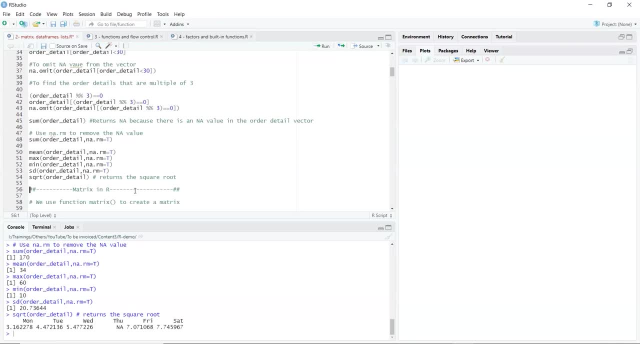 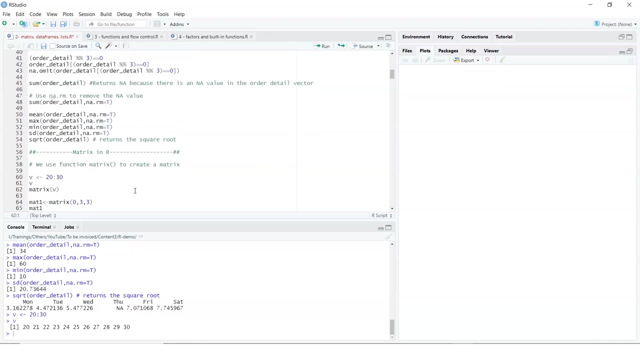 The Values. So Similarly, You Can Also One Way Where You Can Use The Matrix Function To Create A Matrix Which Is Multi-Dimensional, So For. 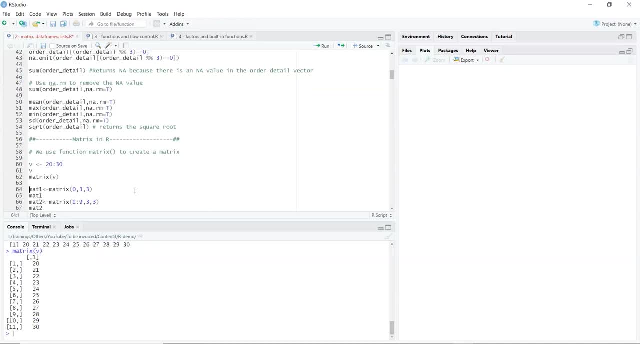 Example: If I Do This And If I Look At, I Am Seeing The Values In That Particular Column. So You Have Already Done That. 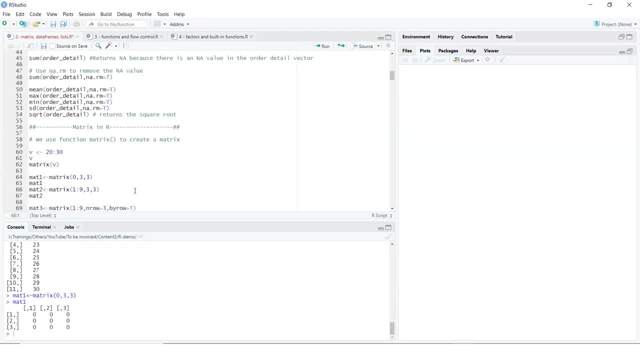 Now Let's Take It To The Next Level. So Let's Create A Matrix Where We Can Also Create A Matrix By Passing In Values. So 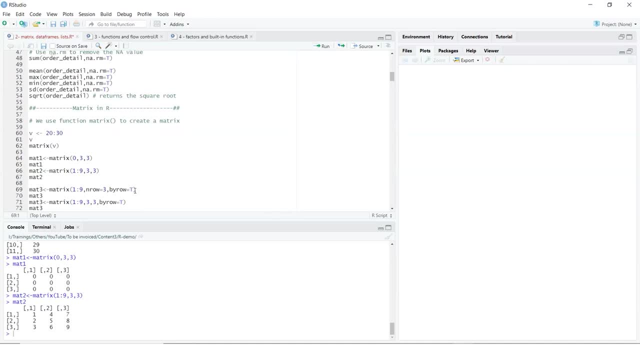 We Can Say One Colon Nine And Then Give The Dimensions, That Is, Number Of Columns Is Three By How Many Number Of Rows You Would 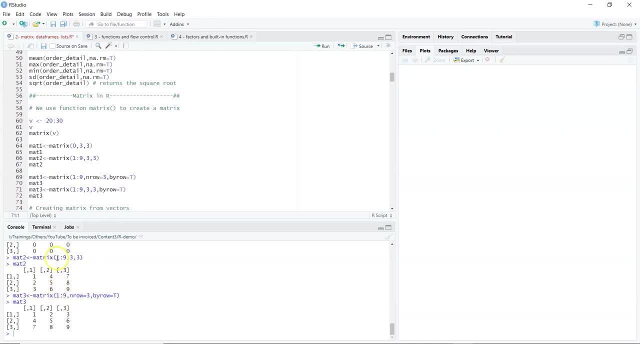 Want And You Would Want To Assign The Data Row Wise. So When We Are Doing This, Now, If You Notice That We Have The Dimension, 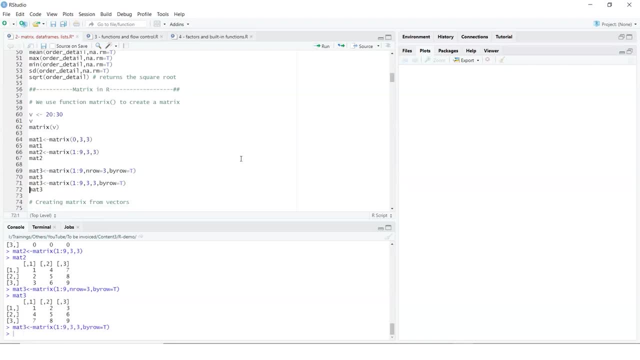 And Selecting By Row, And If I Do This, It Is Still Doing The Same Thing. Now, What We Can Also Do Is We Can 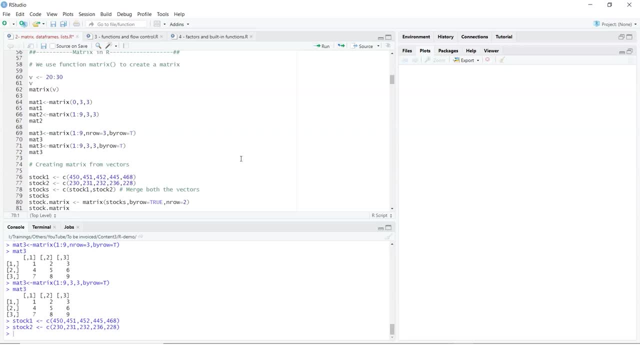 Always Do A C Function And Then Create A New Vector That Is Stocks, Which Is A Merged Result Of Stock One And Stock Two. 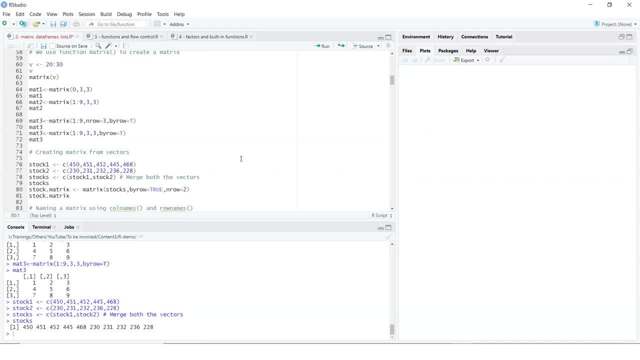 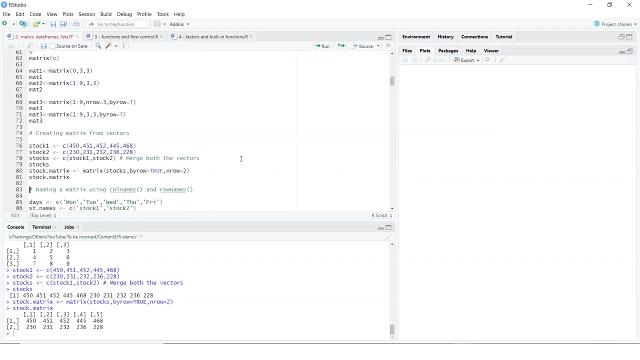 And Let's Look At The Values To Be Arranged Row Wise And I'm Also Selecting The Number Of Rows. So If You Look At 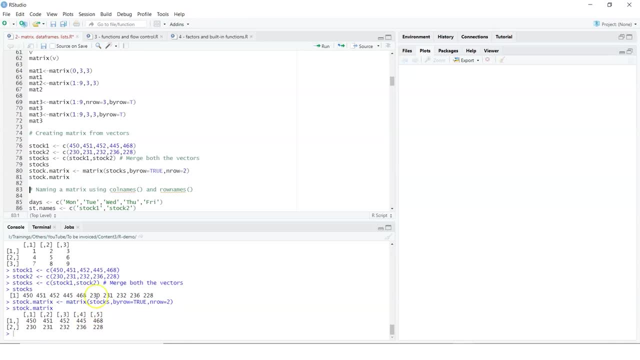 This One. So The Values Which We Had In These Requirements Is, Instead Of Going For Default Column Names And Default Row Names, We Can Give. 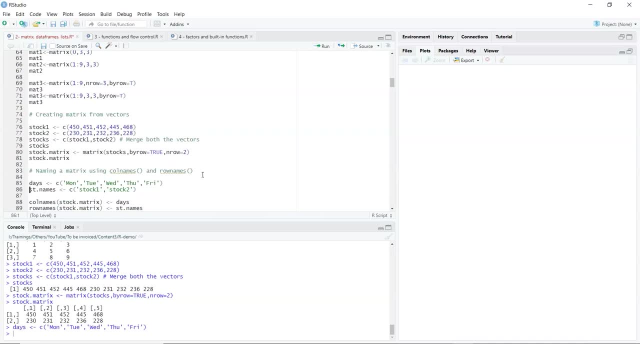 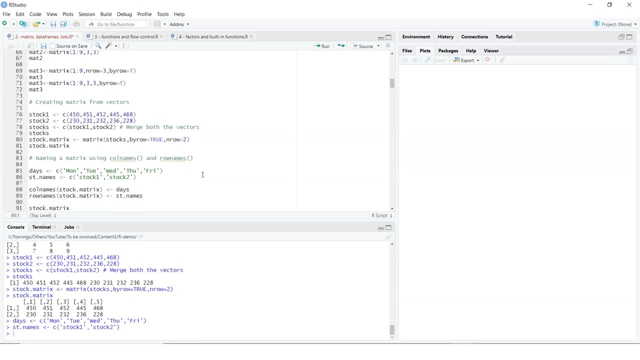 Specific Names To Our Columns And Rows To Make More Sense To Our Columns, And This Will Be For My Rows. Now, How Do We Assign? 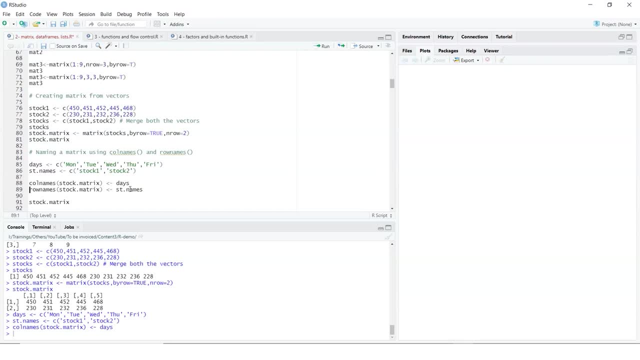 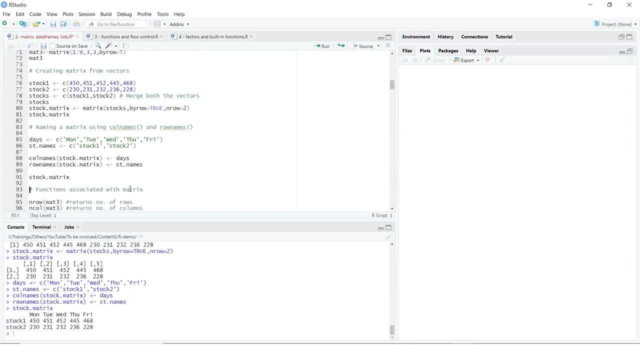 That, So We Can Say Column Names. And This Is Where I Will Say On Our Columns: We Have Passed To Our Matrix. Now There Are 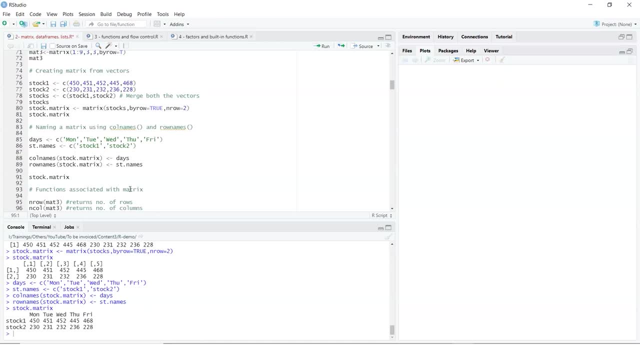 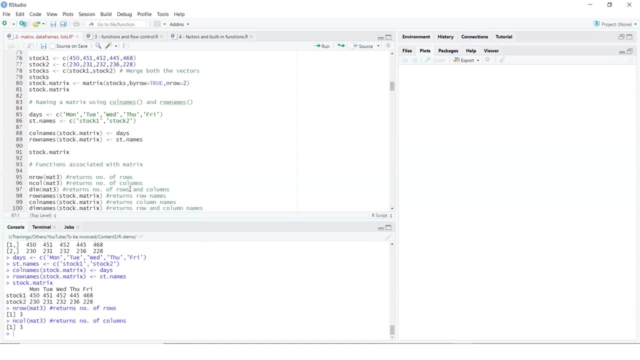 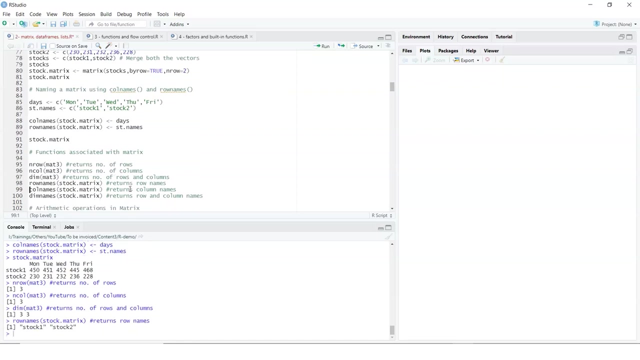 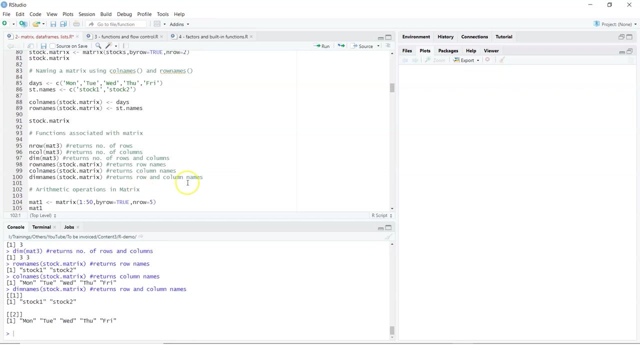 Different Functions Which Are Associated With The Matrix, And Let's Look At Some Examples. So These Are Some Column Names Or Even The Dimension Names. 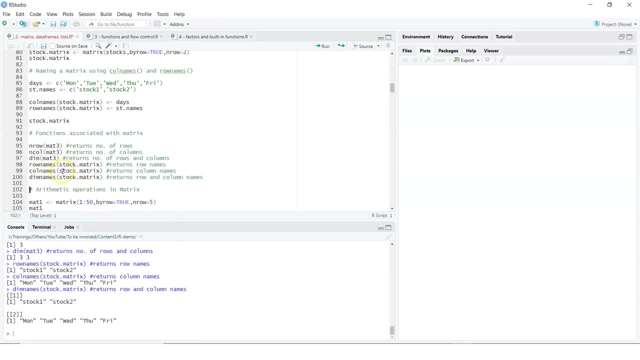 Which Basically Will Give Me Returns The Row And Column Names. So In This Way You Can Use These Simple Functions, Which Are Different Functions Of 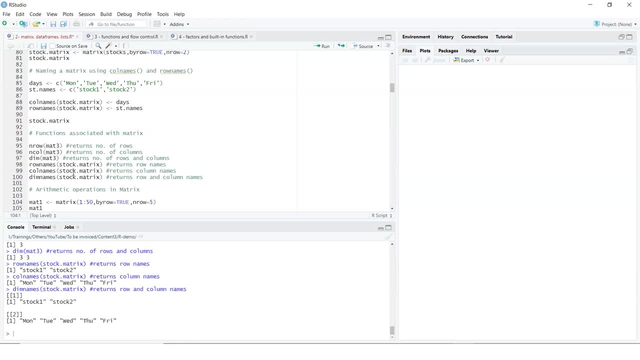 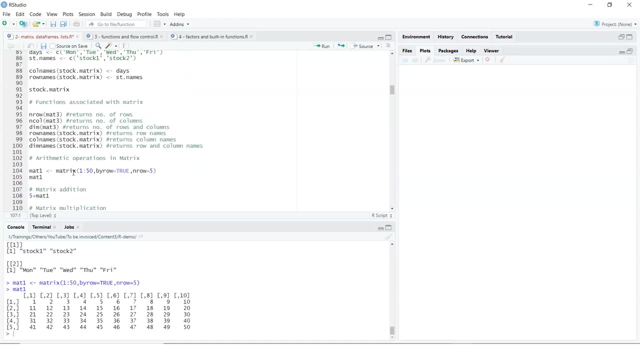 Your Matrix. Now What We Can Do Is We Can Create A Matrix Which Takes Values 1. To 50. We Want To Arrange It By: 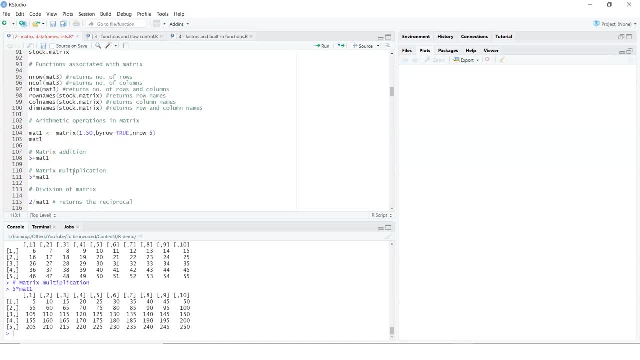 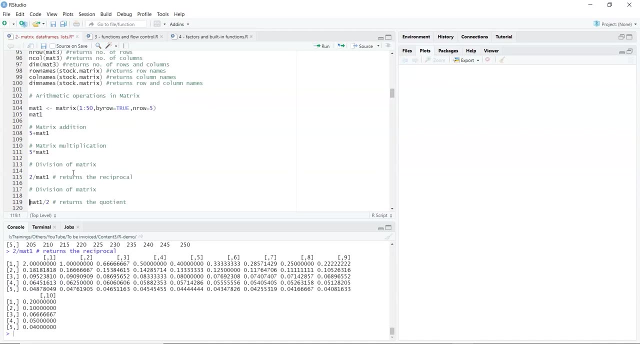 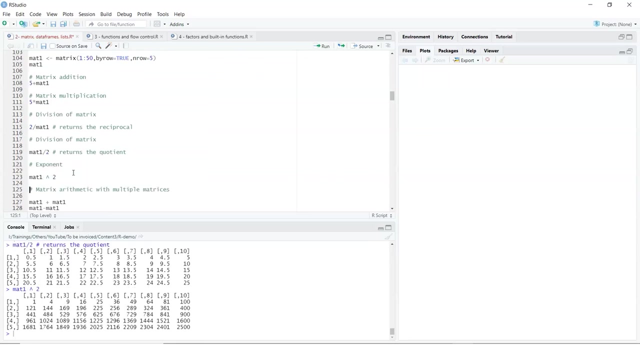 Each Element Of The Matrix. Similarly, You Can Do A Division. You Can Basically Return The Quotient If You Would Want To Do That, Or 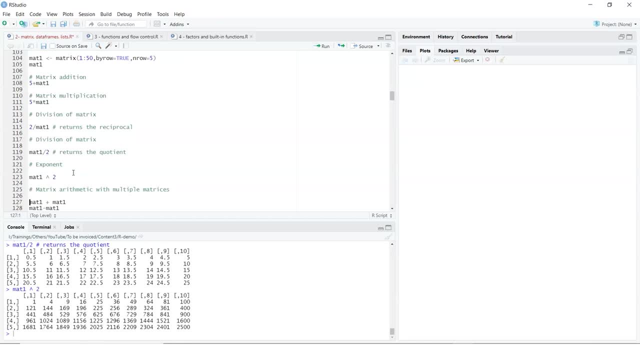 Go For Exponential Values, We Get Mat 1. Plus Mat 1. And We Get A Total Where Every Element Is Added To Every Element. 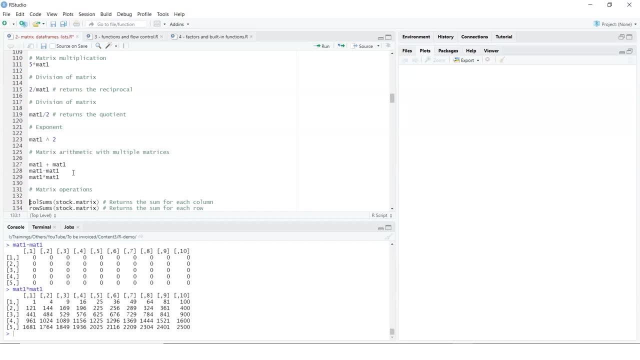 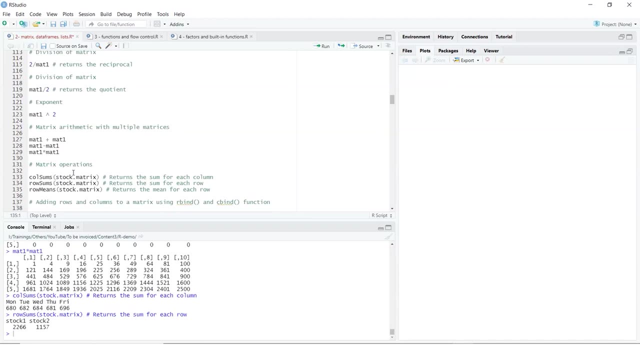 You Can Do A Subtraction, You Can Do A Level, Or You Want To Do A Mean For Every Row. You Can Do That By: 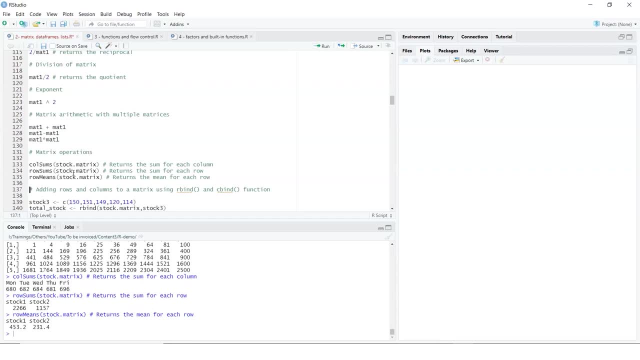 Using These Simple Functions, Now You Can Add Rows And Columns To A Every, Or Added As A Row To My Existing Matrix. Now My Matrix. 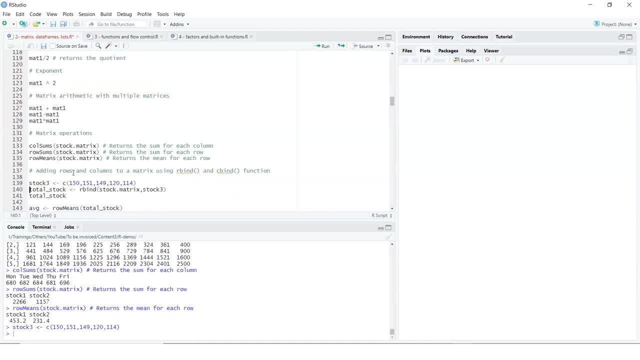 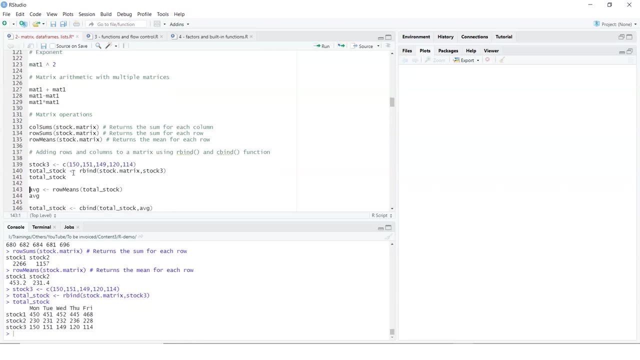 Has Five Columns. So Let's Create A Vector With Five Elements And Then I Can Basically Add A Name. And We Have Added A Row. 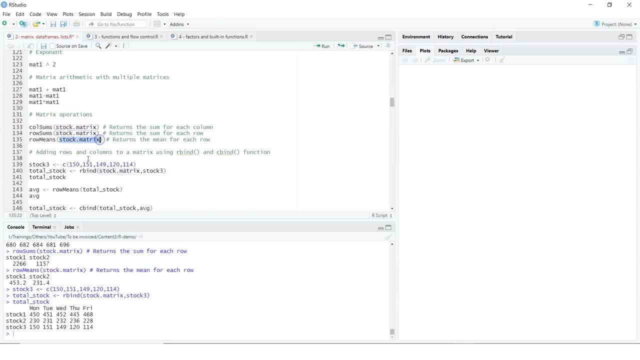 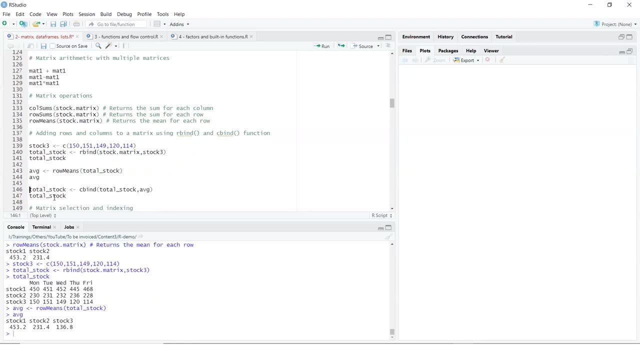 To Our Matrix. Now, Similarly, I Can Find Out Row Means, That Is We Have Seen Earlier- By Calculating The Mean And I Will Say: 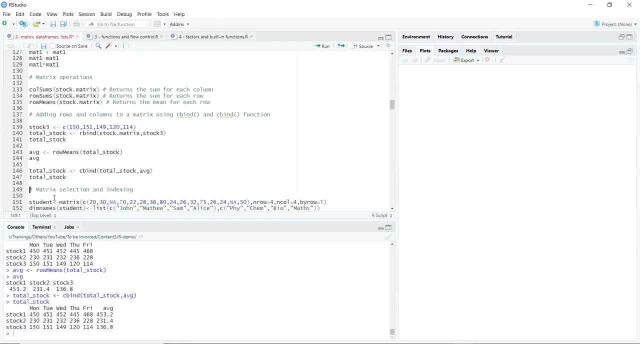 I'm Going To Take The Total Stock, Which Shows Me The Average Value Which Has Been Added To The Matrix. So These Are Some Simple. 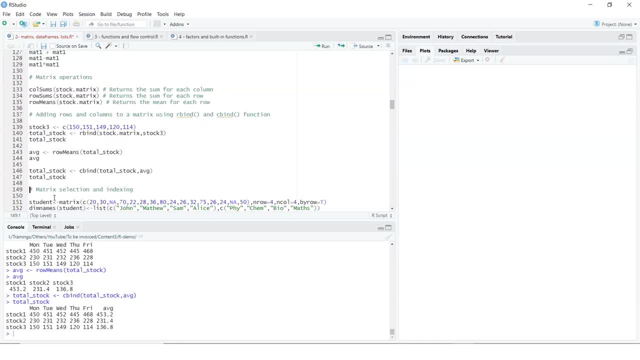 In Matrix, So In Vectors We Were Using Either Names, Or We Were Using Positions, Or We Were Using Indexing. Now, Here Let's Create. 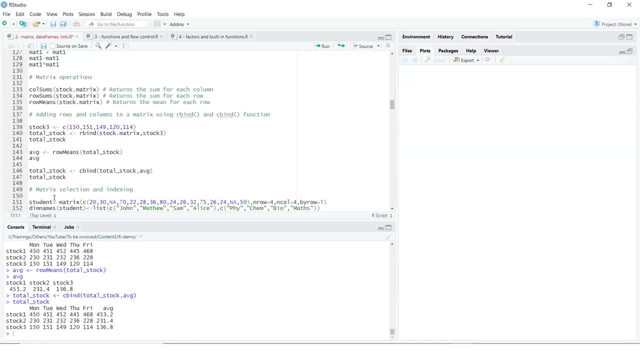 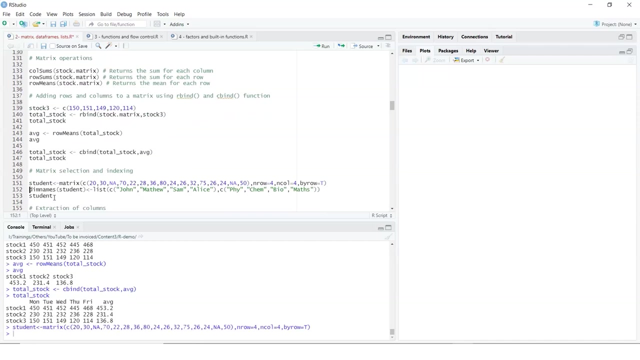 A Matrix Called Student, And So That Means The Values. The Number Of Values In This Vector Should Be A Multiple Of Four. I'm Saying 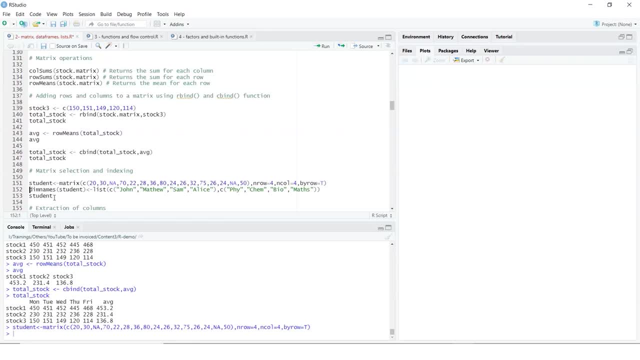 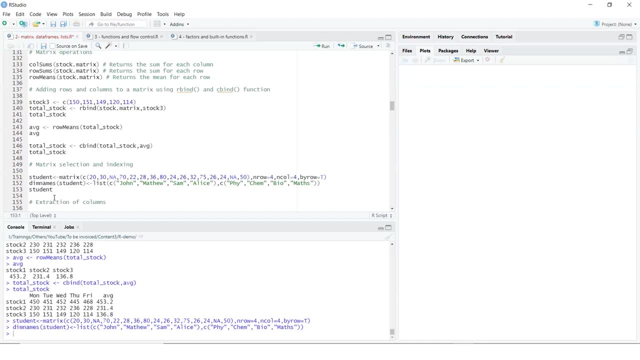 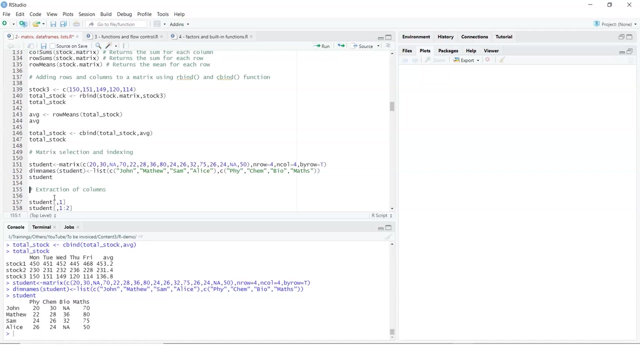 Columns Is Four And I Would Want To Get A Vector. And Now If You Look At Your Student, It Basically Shows Me The Values Which 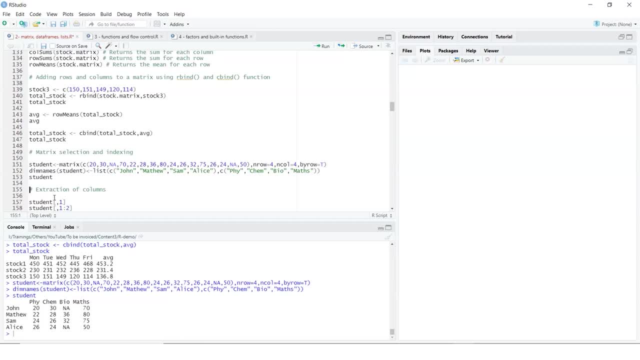 Were First Applied To The Row Names, That Is, John, Matthew, Sam And Alice, And What We Are Looking At: The Vector Of The Vector And 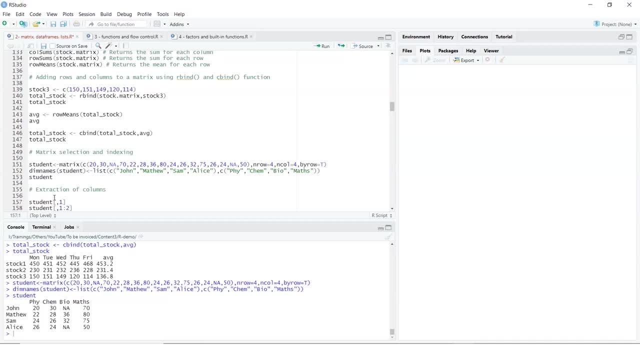 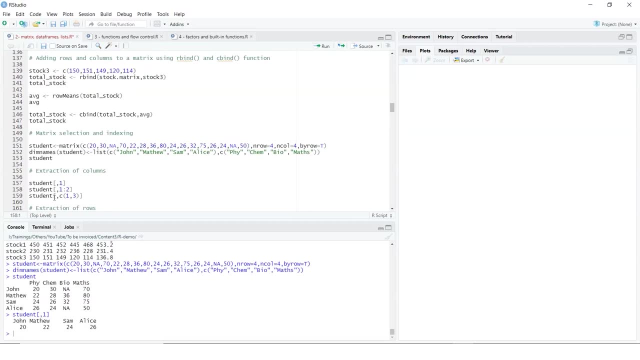 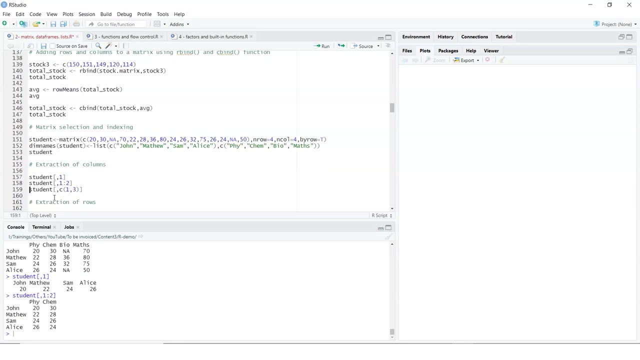 What We Are Looking At: The Vector And The Values Of John, Matthew, Sam And Alice. That Is Just The First Column. Now I Can Also. 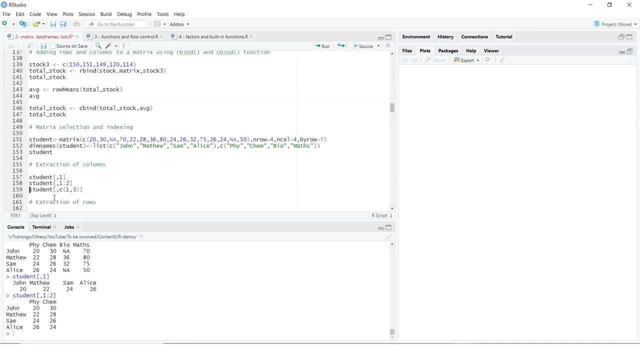 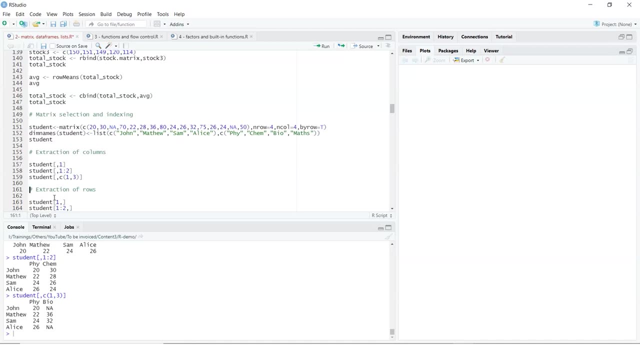 Say From First Column Onwards- I Would Want To Look At How Many Columns So I Can Do This- the row position first. So if I do a student one, that gives me the row values and this is giving. 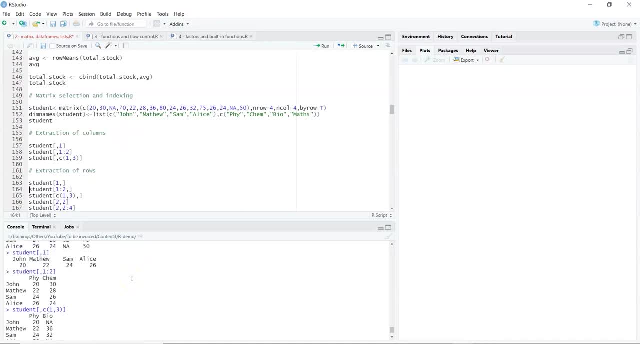 me values for my student, which we are seeing here. So for John, we have 20,, 30,, NA and 70, and that's what we get here. when you do a row wise operation, You can also do a row wise, and how many rows do. 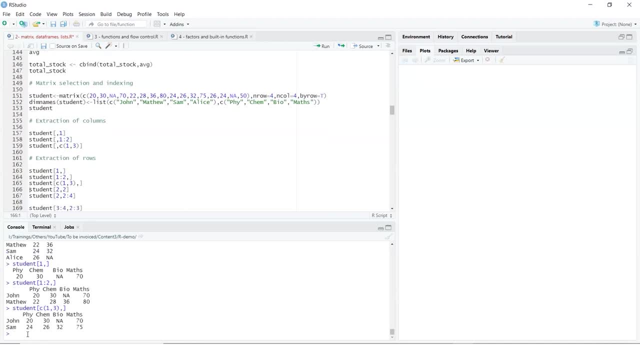 you want, You can use the vector function to do that. You can also select or slice out a value where you are getting an intersection of row 2 and column 2, and then you can also start from a particular position and then onwards get your rows. So these are different ways in which you 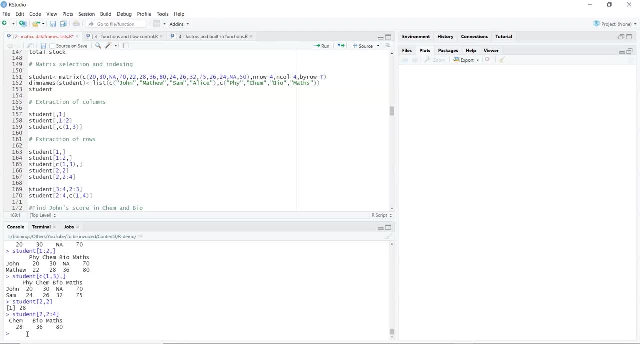 are slicing the values from your matrix by columns or by rows. So at this point of time let me just type in student here and let's look at the value of student. and then here we are interested in 3, colon 4, and then 2, colon 3.. So what does that? 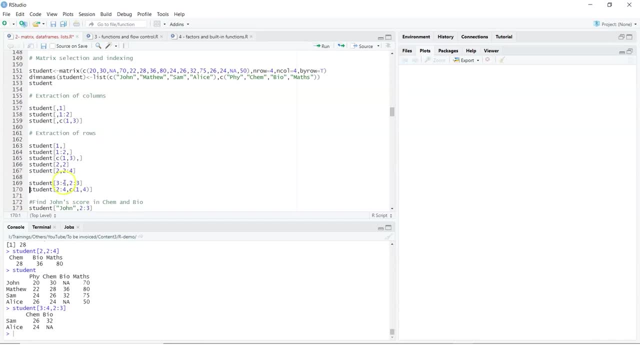 give me. So you are looking at third to fourth row, So you are looking at Sam and Alice, and then you are looking at columns 2 and 3.. So that basically gives you your 26,, 32,, 24 and A. So first is you are giving your row positions, or how many rows you want, and then 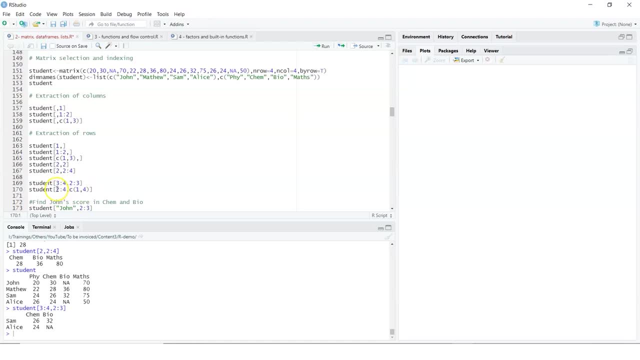 you are giving your column, So similarly you can do this, You can say from row number 2 to 4, and then, column wise, you can say 1 to 3.. So if we do this, so this tells me two columns, which is first: 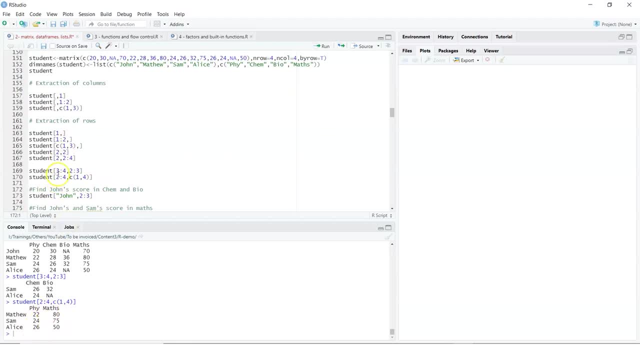 and second, and it shows me rows which is from second to fourth. So in this way we can extract columns. Now, if we would be interested in finding out a specific value. So, for example, if I again bring up student, This is my student and what I would be interested in is getting the value of. 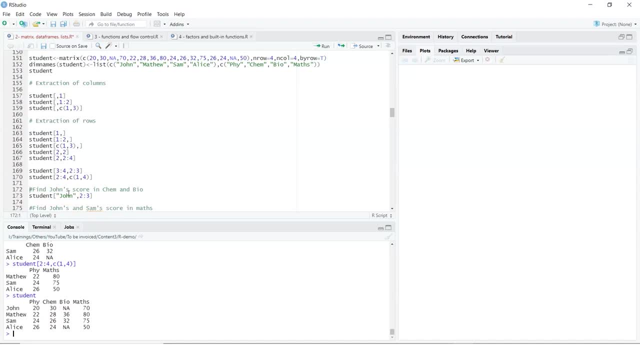 John and for specific subjects. So maybe we are looking for 2 colon 3.. Now, if I do this, it shows me for John and what we are interested in is 2 colon 3.. So that gives me the value for chemistry and biology. So that gives me the value for chemistry and biology. So that gives me the 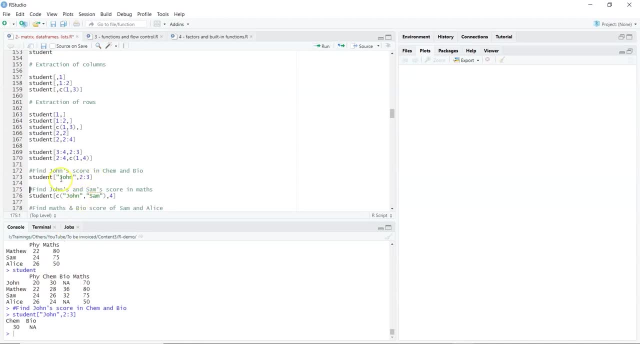 so you are giving the columns, So, row wise, you have already specified the name and that basically selects the particular row. I could have given a number and chosen which row or which rows we would want to pull out the values. Now, if I would want to find out the value for John and Sam, 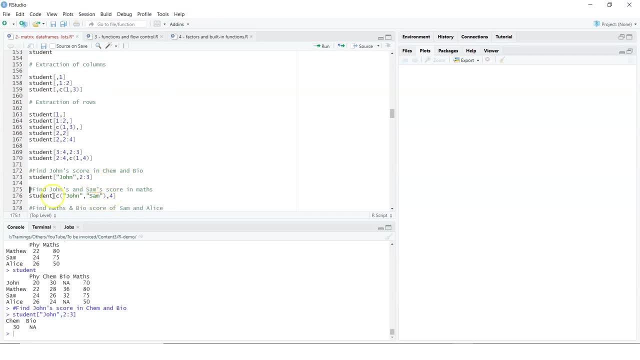 Now, in that case I could use indexing or positioning, but that has to be continuous. But here you are talking about John and Sam, which has met you in between. So we will basically create, We will get the values for John and Sam and then we will look at the value. 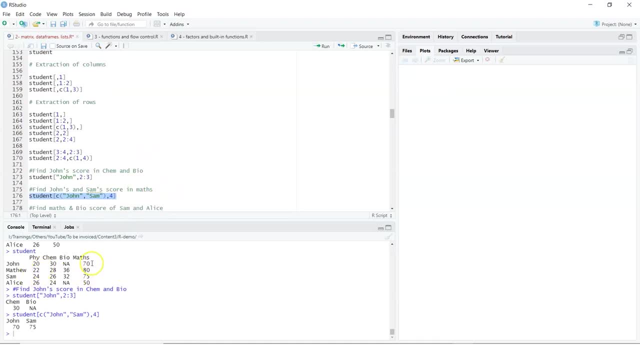 4.. Now that is basically giving me the values in the 4th column, which is 70 and 75.. Similarly, if you go further, you can look at maths and bio score of Sam and Alice. So you will give your row names, that is, Sam and Alice. 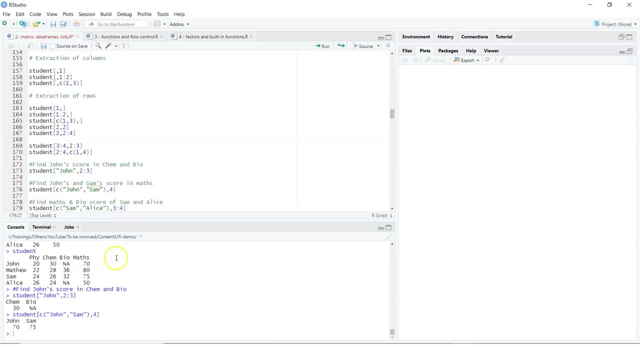 And then you would want the values for maths and bio. So that is basically your 3rd and 4th column, And we can do that by looking at the values. How do you find out an average? Well, that's pretty simple. You can use the mean function on student. 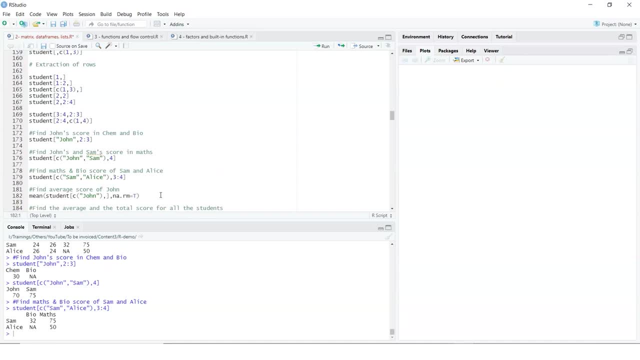 You will select your row name, that is, John. You also want to get rid of any values, Otherwise that will give a poor problem. So you get rid of that by saying any dot Or M equals true, And then you get the average score of John. Now how do I do further computation? 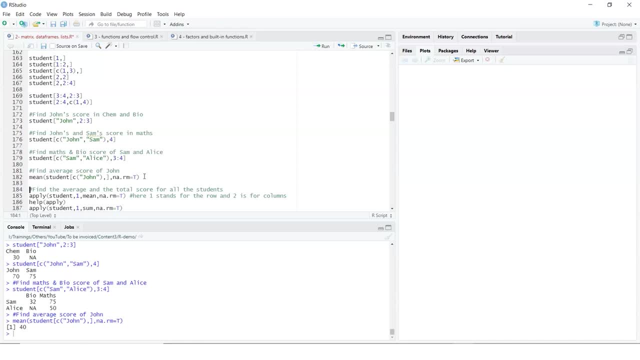 That is, if I want to find out the average and total score of all students. So in this case I can apply or I can use an apply function. Here I'm saying I'm working on student And we would want to give the row number, that is, 1.. And we want to also give the 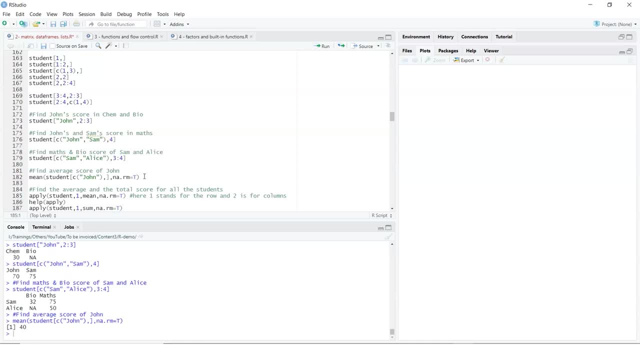 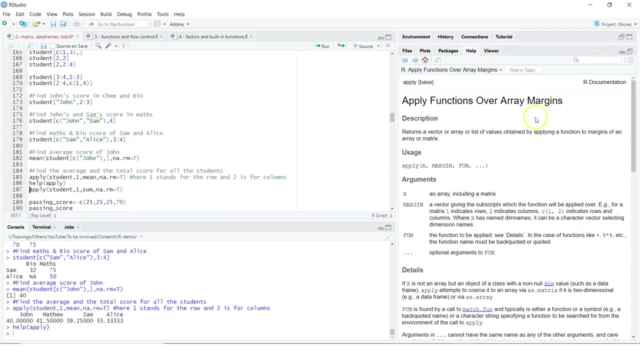 number of columns. So I want to find out, mean I want to remove or get rid of the any values. And now if I look at help apply, it tells me how does the apply function works over the array margins. So I will do an apply function on student where I would want to select the 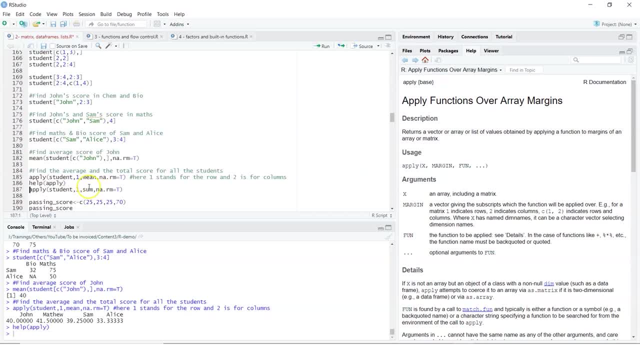 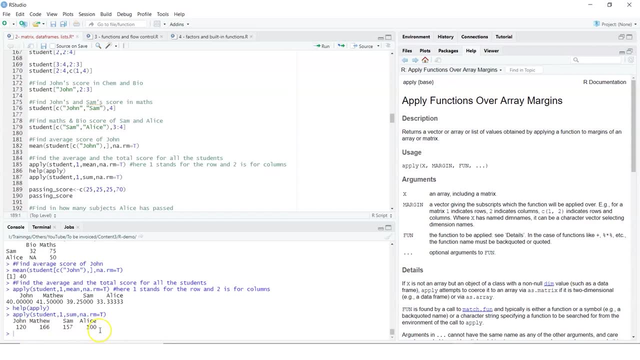 first row, I would say I want the sum And I want to get rid of the any values. So this gives me the sum for each student And here we are getting a mean value, which was for each student. So what we are doing, 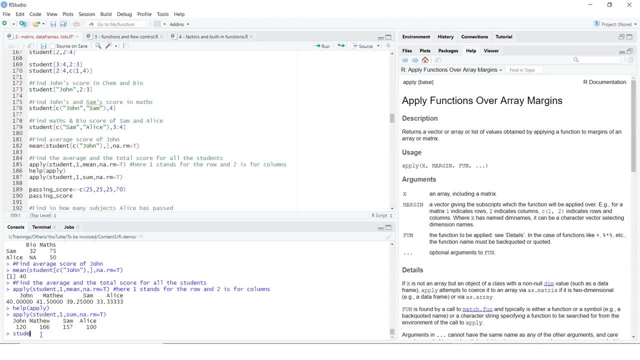 here is, for example: let's look at student again, just so that we avoid confusion. So we have student And then we have physics, chemistry, bio, maths, And I have said row 1. So basically, what we want is for John, We want the total number of columns. 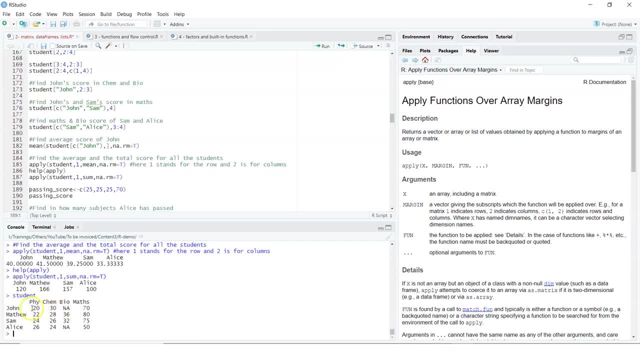 Total. And what we can do here is we can say 20 plus 30, avoiding any, and then 70, that gives me 120.. Then you look at Matthew, So this is again doing a totaling. There is no any value. And you look at the value Right. So when we have chosen apply function, we have 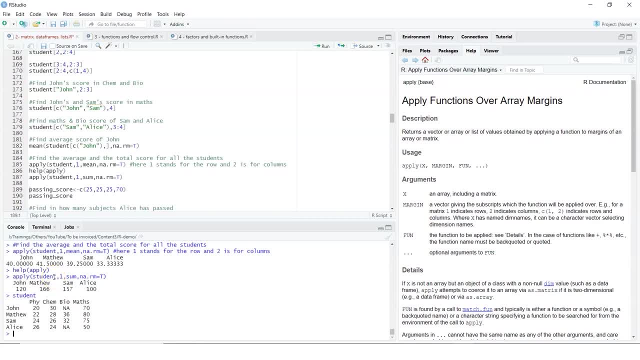 worked on student. Now here we are interested in the values, that is, sum of all the values for this particular row. I am saying: take care of any and then give me a sum. Similarly, you did a mean, and that was giving you a mean for each student. So these are some simple operations. Now what? 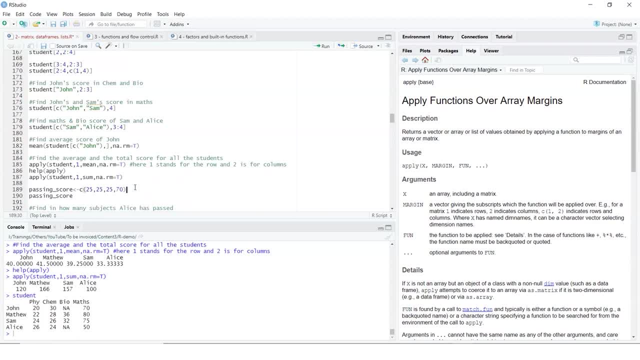 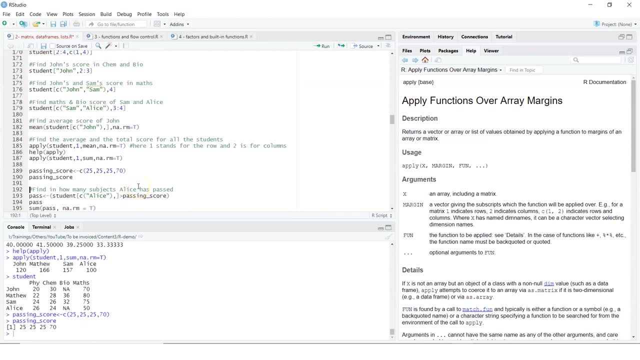 we can also do is we can basically create a vector called passing score, And what we would want to do is we want to get the values or find in how many subjects Alice has passed. How do we do that? We will have to compare. 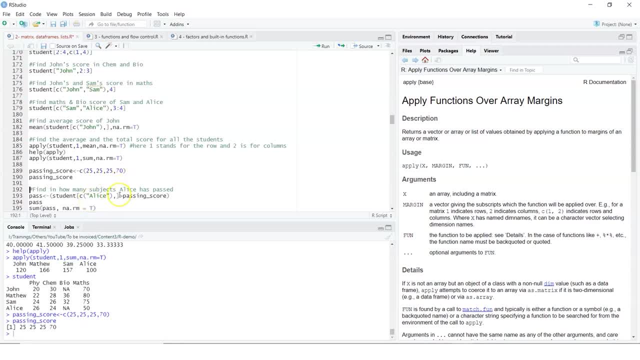 Alice score, which should be greater than or equal to the passing score. So what we can do is we can create a variable here. pass. Now I'm saying student, I would be interested in the values for Alice. So I've mentioned that row name here. I am then comparing it. 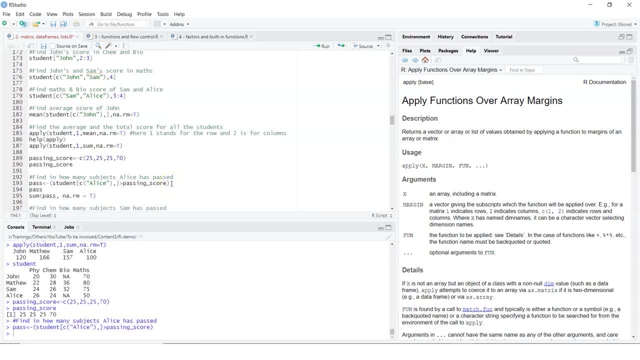 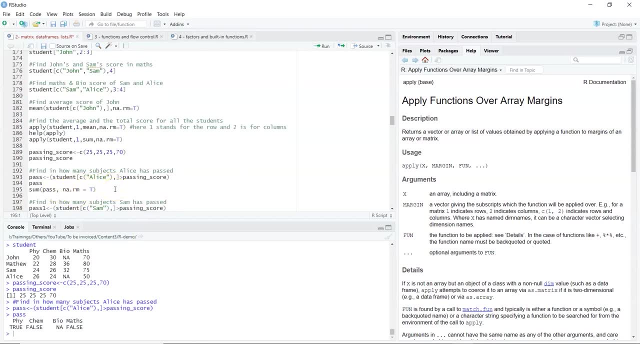 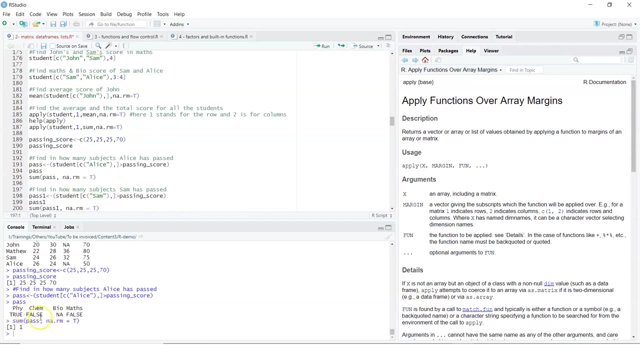 with passing score which we have created here, and that will give me the values wherever Alice has passed in a particular subject. Now I can obviously get rid of the any values And then look at this, which basically tells me there was one subject in which Alice passed. 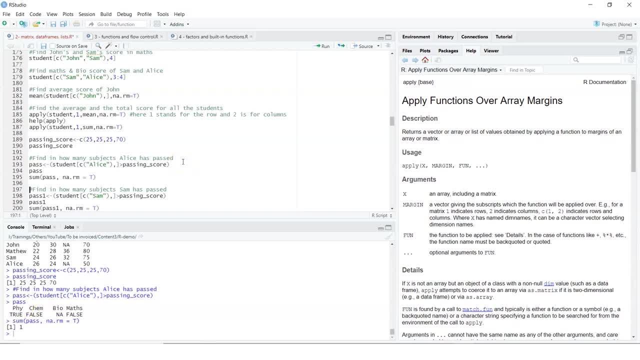 and rest were either false or any. Now, same thing we can do for Sam. So Sam is here And what we want to do is we want to look at the values here. So we will say let's do the same thing for Sam and find out the. 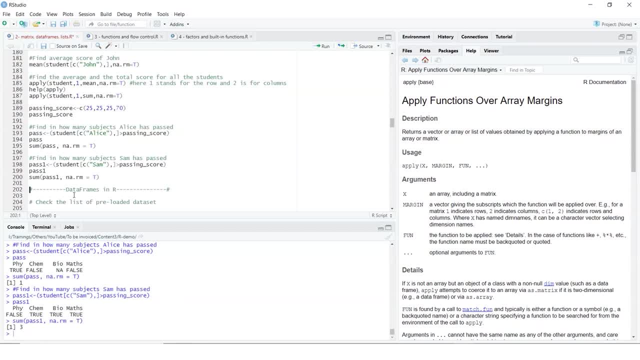 comparison with passing score and get rid of any values. So you are Basically Extracting value. So these are some easier operations and usage of functions on your matrices which are filled in with values at row level and column level, And then you can. 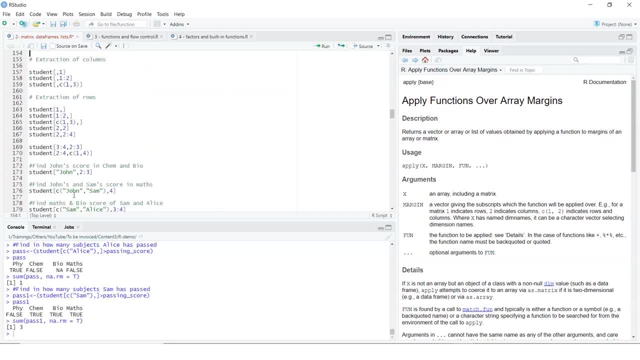 apply one of these functions, or multiple functions, to basically extract value which makes more meaning. So that's with your matrix. Now let's also look at data frames. Now, data frames, as we know, is basically data which has been ordered In rows and columns. 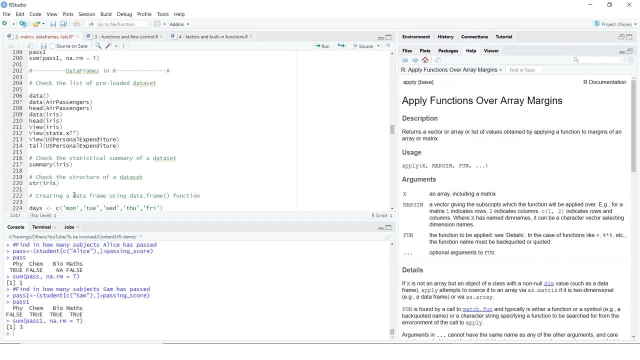 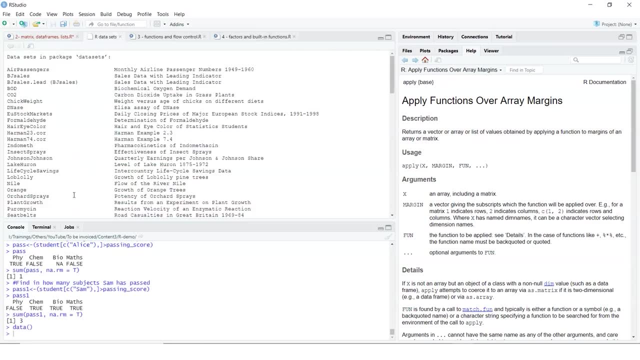 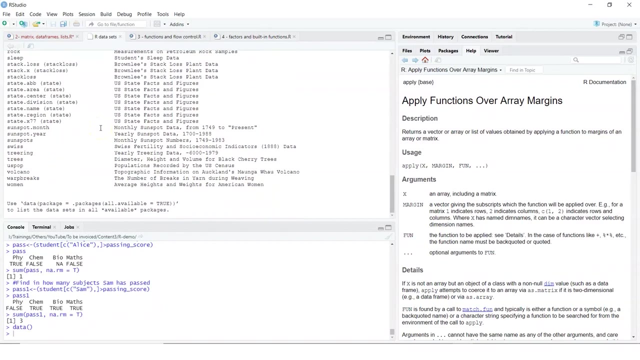 Where in we can assign row names, we can assign column names, we can do some operations on data frames. So let's look at example. So if I do a data here, so that gets me some sample data sets or functions, what we have here. So let's do. 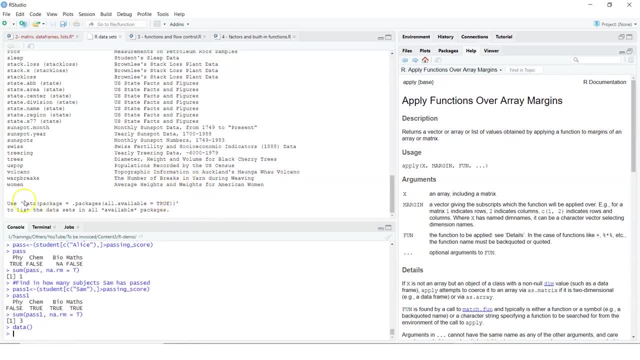 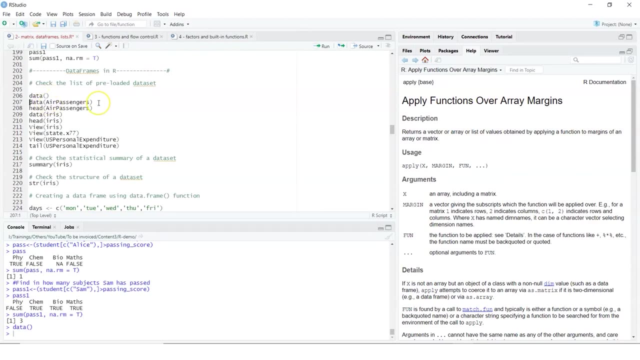 Once we have our data here. So it says use data package And then you can get List all the data sets and available packages and you can basically look at all the R data sets which we are seeing here. it has opened up. So I would be interested in getting the air passengers data. 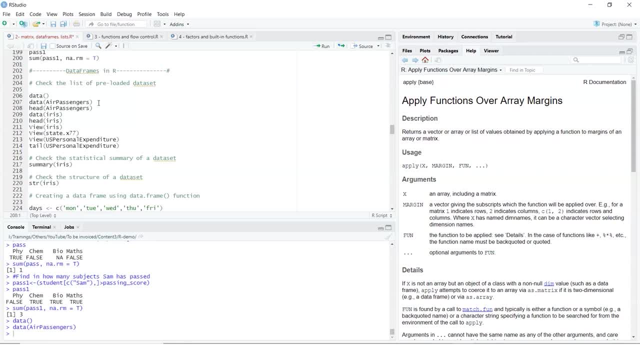 So I'm going to pass that in the data function and then, if I do a head to see the initial data from air passengers, it shows me the values, what we have. Similarly, we can do that on iris data set and look at the head values. 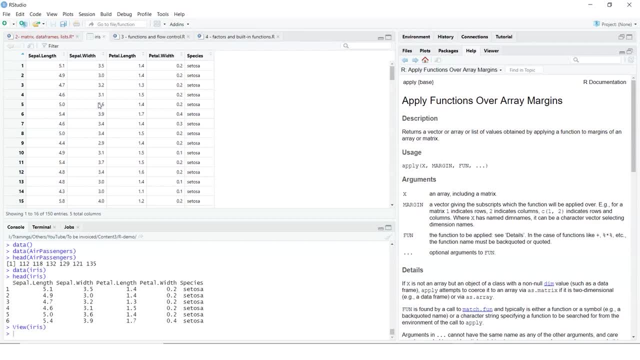 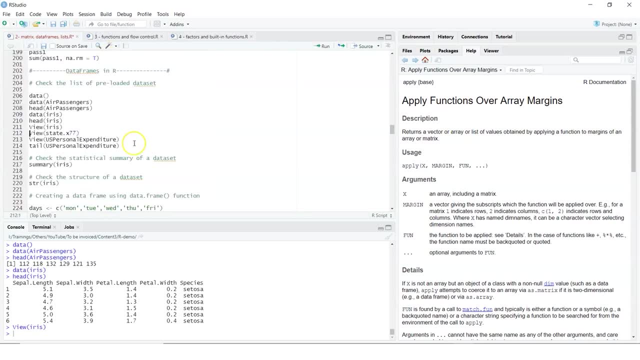 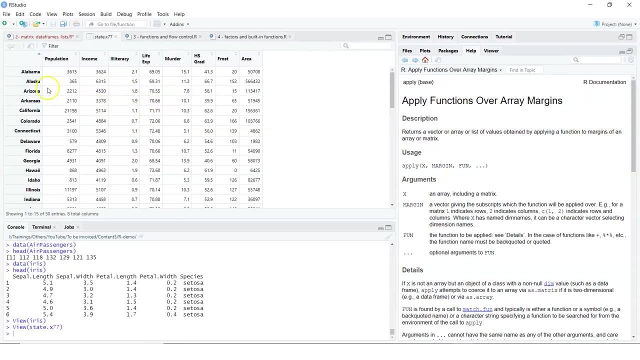 I can Do a view to look at specific values in a tabular format if that makes more meaning and that makes it easy for analysis. Now I can do a view on state Ex 77 and that basically shows me the population income and all this for different US states. 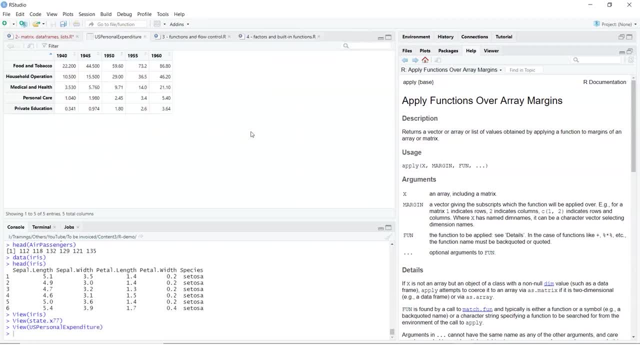 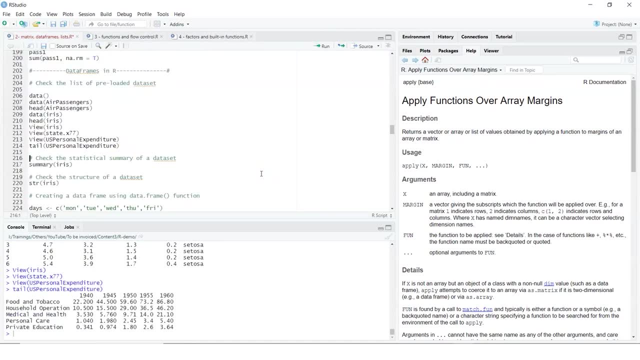 so these are some different data sets, what we have. You can do a view on them to basically understand the data or look in a more readable format. You can just do a tail to get some end data. so head and tail functions just give you the 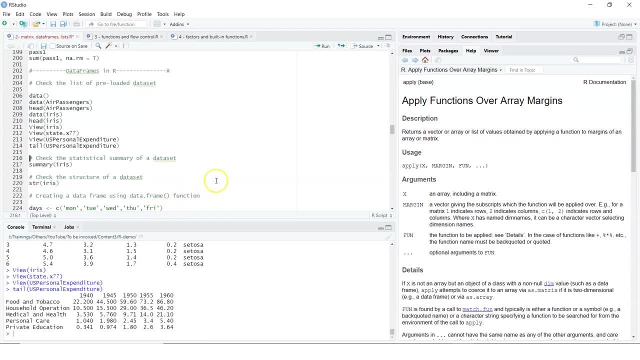 top six entries, or basically your entries, from that particular data set. Now the question is: how do we work on this data so I can get a statistical summary? So I have the iris data set which we had here, So if I do a head it shows me iris data set. this is a popular data set which shows the 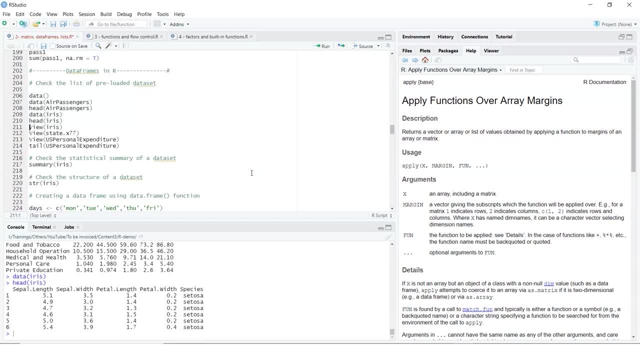 petal lens, The length of particular flowers and the species. what is the length, what is the width and what species does that flower belongs to? Now here we can get a summary, that is, statistical summary, of a data set which gives me mean, first quartile, median mean, third quartile and maximum values. 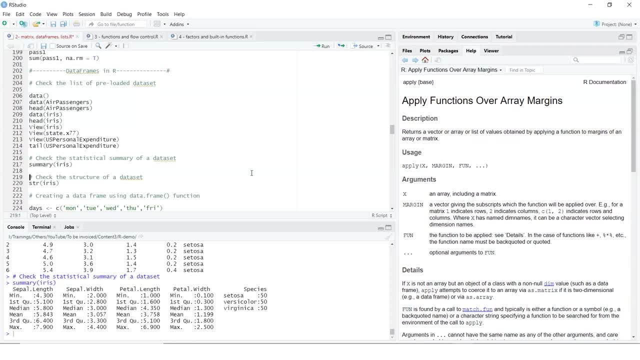 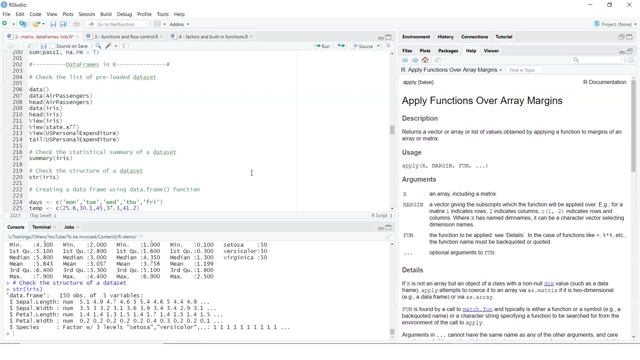 It basically shows you the count of the entries for each species, what we have under the species column. Now, For instance, I can check the structure of this data set using STR. I can create a data frame now of this data using the data dot frame function. 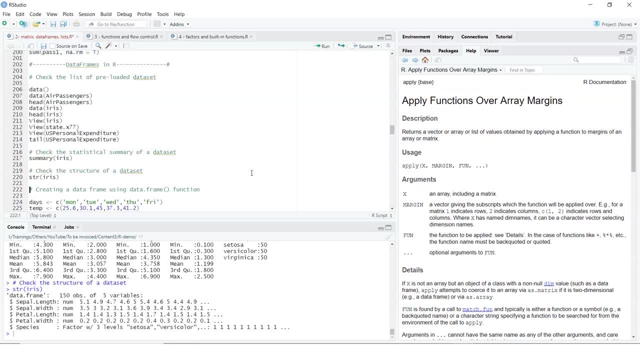 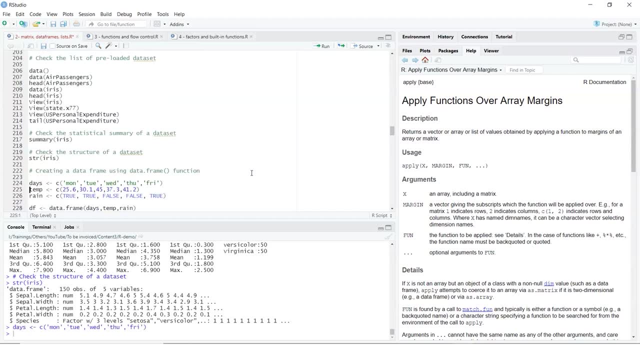 So for that we need to also have, say, for example, if we would want to create a data frame. let's see how do we do that. So first we create a vector of days, we can create a vector of temperatures and rain, and then we want to create a data frame. 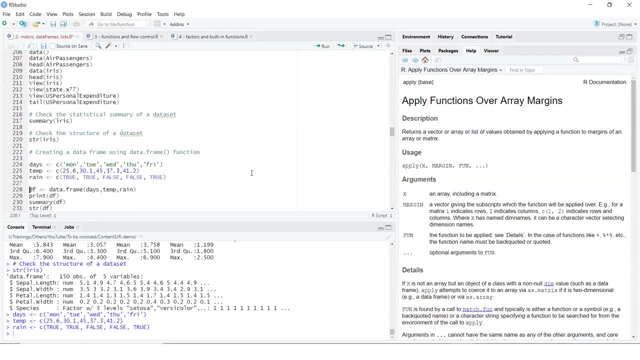 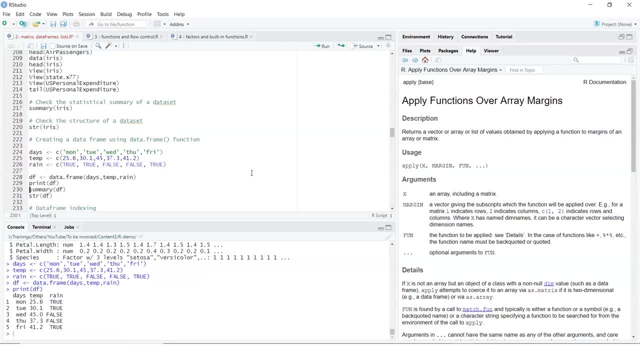 Out of this. so I use the data dot frame option. I pass in my days, temp and rain as the vectors and now if you look at the data frame, you basically see that I have my days, my temp and rain. So those were the variables, those were the vector names and those have become the column. 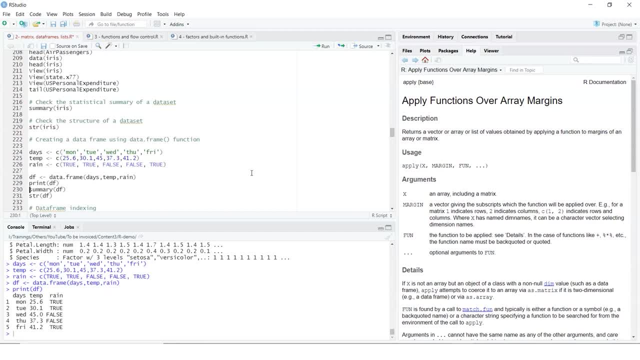 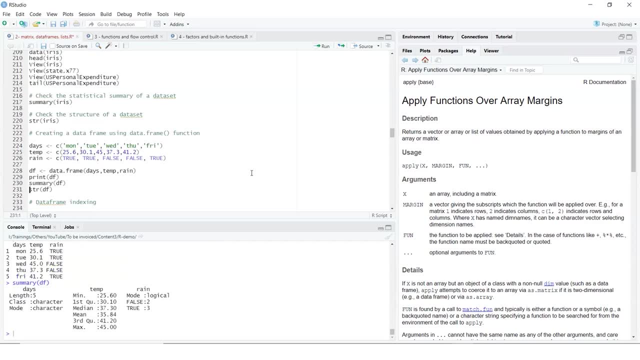 names, row names are auto assigned and basically we are seeing the values which have been passed in my data frame. Now I can do a summary on this to basically look at what is the length or how many values we have in data frame. What is the class of elements. 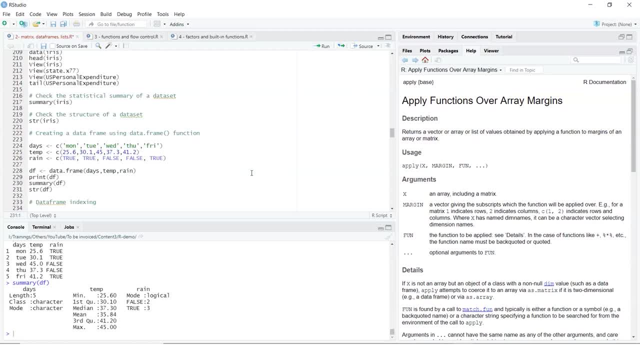 So that is character. You are looking at your values, or summary, which gives you mean, first quartile median mean and so on, And then it also shows you the complete data on rain. What is the mode here? What, how many falls or how many true values we have. 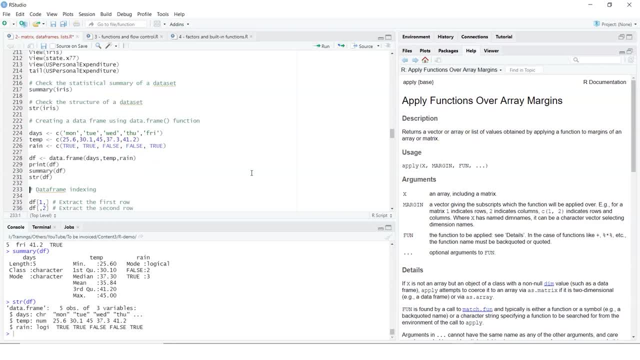 You can also look at the structure Of this data frame by doing a STR, which gives me how many objects we have, how many variables we have, What are the different variables? So that is days, temperature and rain, and the values for those for days. 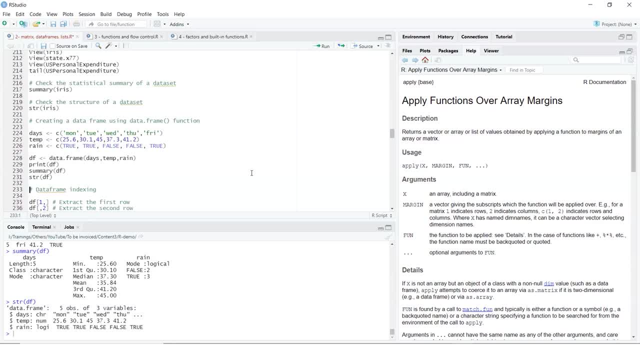 If you notice, it is of the type character: temperature is numeric, rain is logical. Now how do we do data frame indexing? So, like your matrix, which basically has rows and columns, And in multi dimensions, similarly in data frames also you have indexing, so you can. 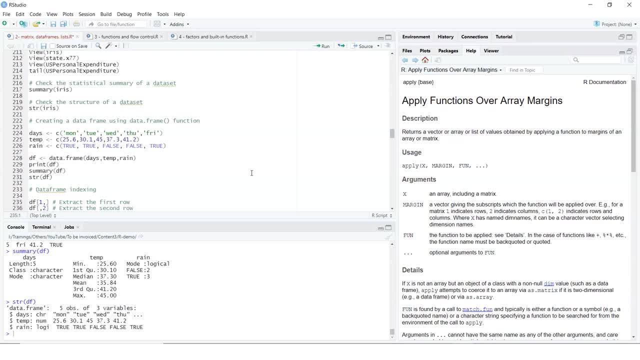 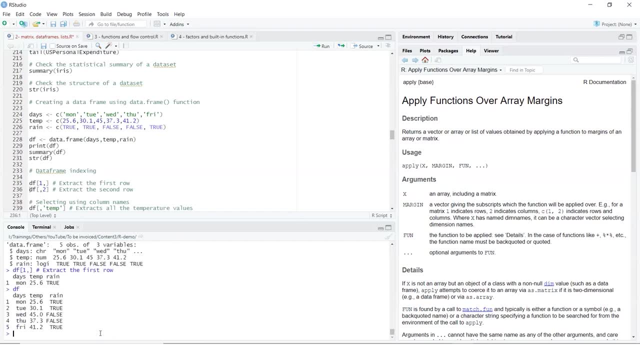 do a data frame. So I could just extract the first row by doing this and that basically gives me the value. So you can always compare it by just typing a DF. So that's my data frame. And now let's look at the values. extract the first row and that shows me Monday twenty. 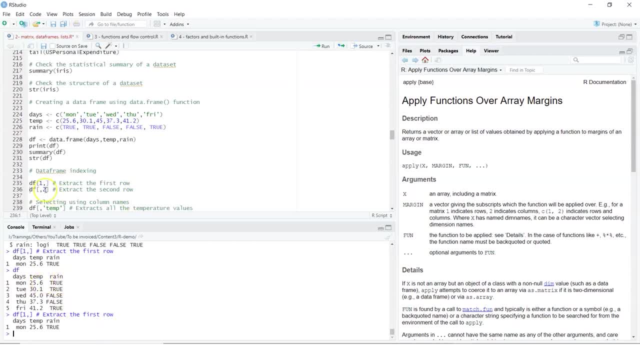 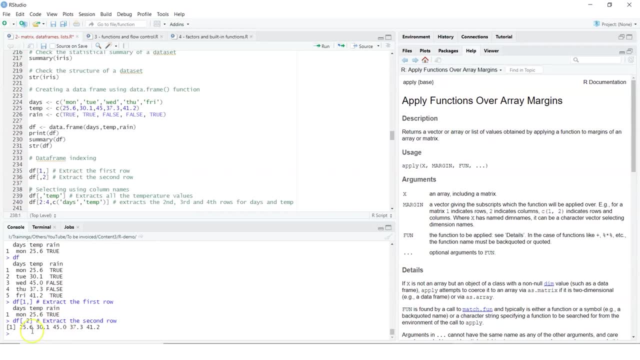 five point six. rain value is true. Now, I can also do it, column wise, For example. I could do it in this way. So here, what I'm doing is I'm doing extracting the second row from this one, So it tells me: twenty five point six, thirty point one, forty point zero, thirty seven point. 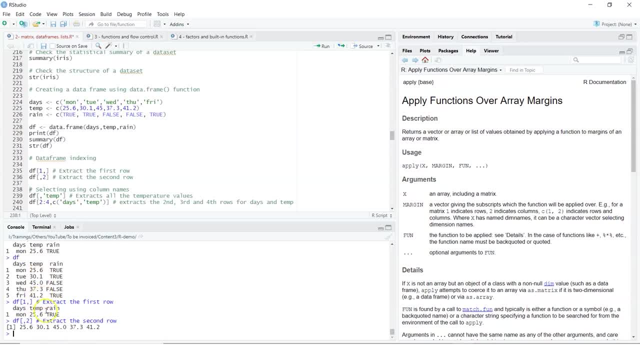 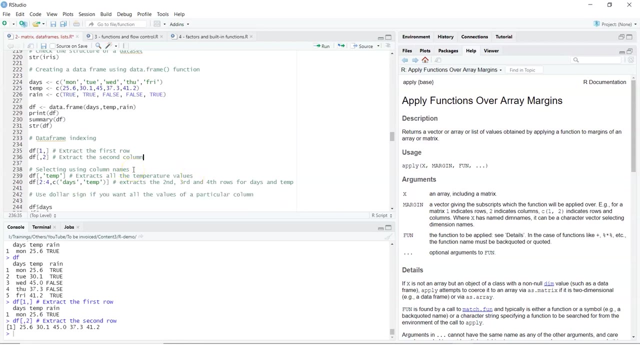 three. So you have extracted the values for the column. So I would not say extract the second row, you would say extract the second column. So this one should be second column. Yeah, Selecting using column names. So that's the easiest way to extract the values for a particular column. 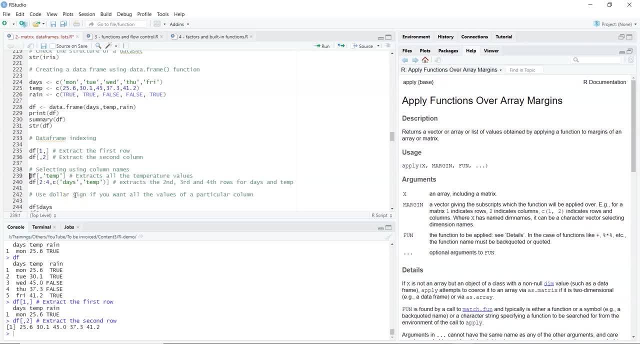 So I can just do this: instead of giving the position of the column or the column number, I'll give the column name and that gives me all the values of temperature. And if I do this, where I'm saying two, colon four, and then I'm giving the columns, so it 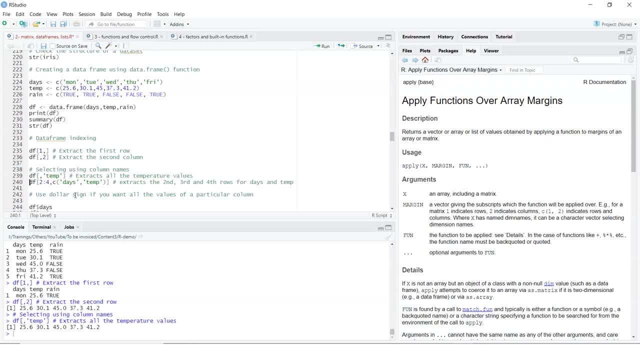 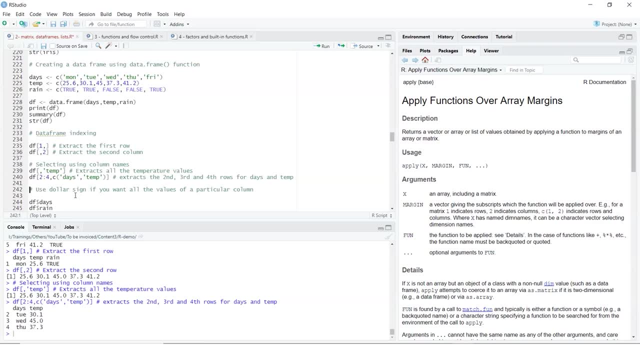 gets me the second, third and fourth rows for day and temperature And we are looking at the value. so you have given your own names and then you have selected your columns. You can also do a dollar sign if you would want all the values of a particular column. 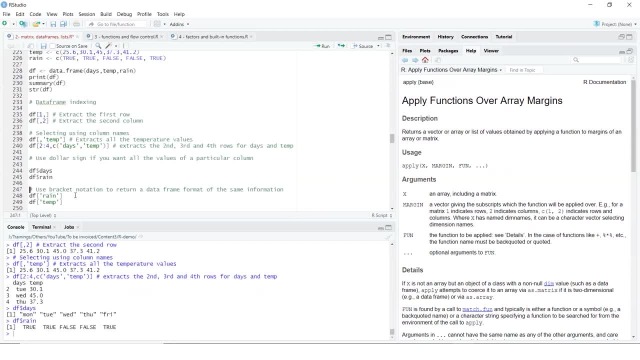 So I can just do a DF dollar days or DF dollar rain, and it shows me the values from my data frame. Now one more way of doing that is using your bracket notation to return a data frame format of same information. So if you want the resultant data in a data frame, 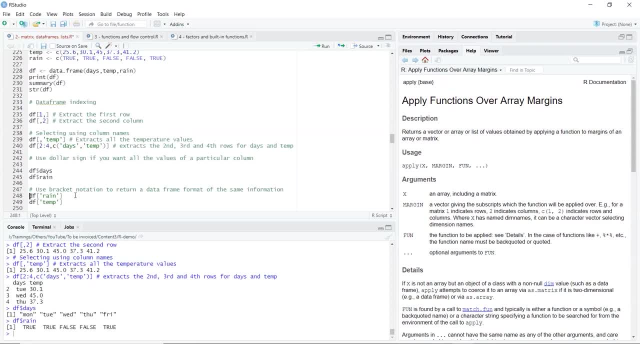 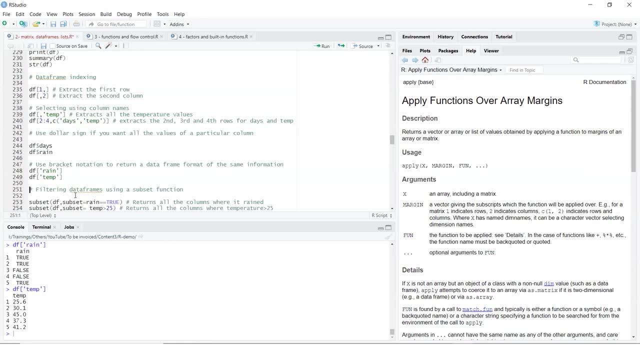 So if you want the resultant data in a data frame, You can just do a DF rain or DF temperature and that is basically giving a data frame. So if I had assigned this to a value and if I had look at the type of this, that would 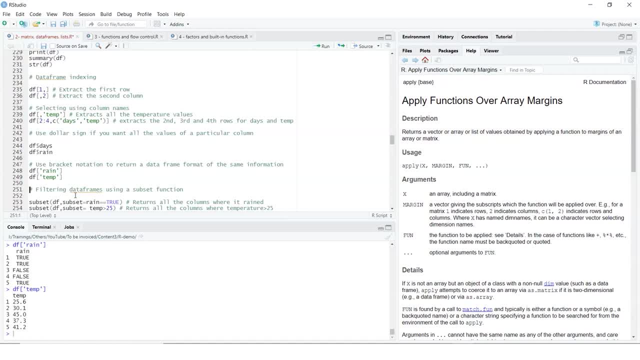 be data frame. Now, one of the things which we also require is filtering data frames using a subset function. So that is subsetting the information from a data frame. So we know we have our data frame. Let's look at our data frame. 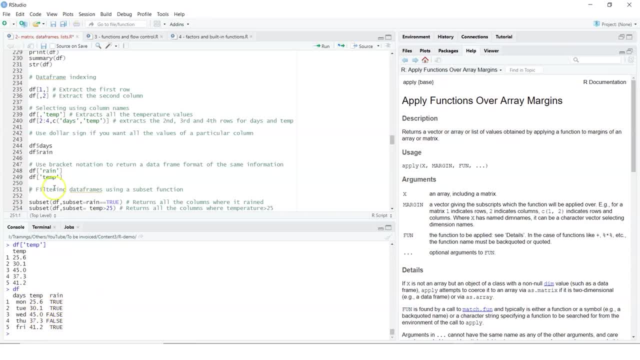 Again. so that just reminds of what data values we have. and here let's get a subset out of it using the subset function. So I'm passing in my data frame, I am saying I would be interested in the rain column, So I'm giving subset rain column and wherever the values are true. 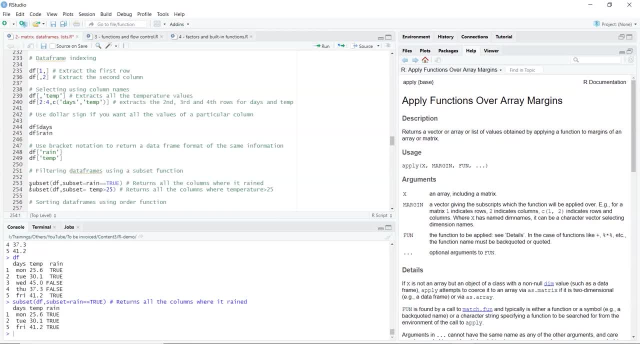 So returns all the columns where it has rained. Similarly, I can do a subsetting by giving a value for temperature Where it has rained. Similarly, I can do a subsetting by giving a value for temperature Wherever the value is greater than 25 and that shows me the value. 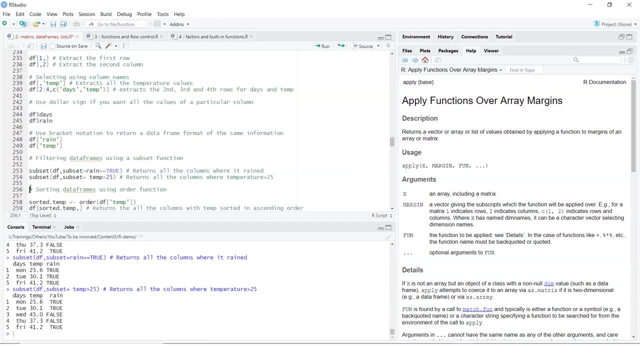 So this is where you are filtering the data in data frames using a subset function, to which you have to provide a column name, and then giving a condition. Now, one more important thing which might be required is sorting your data frame using order function, So I can create a variable by name, sorted dot temp. 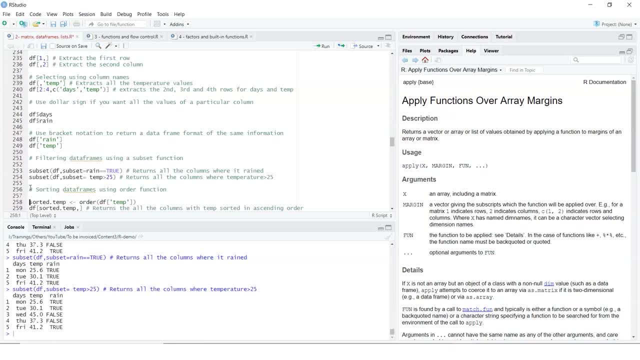 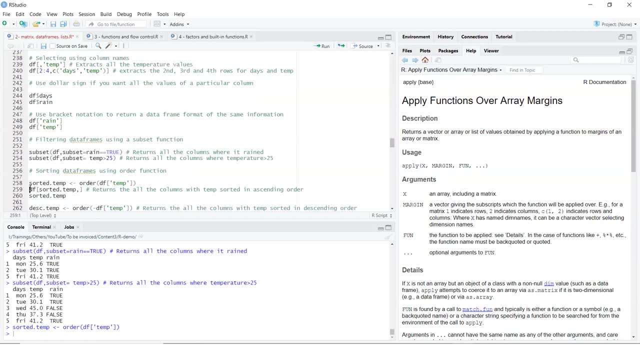 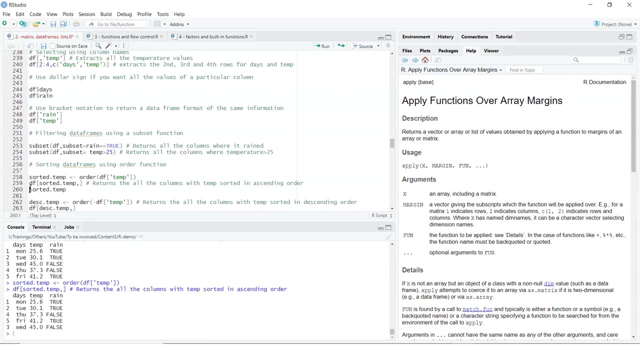 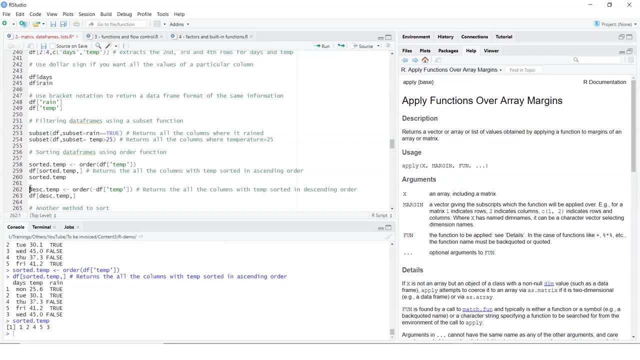 I want to do a ordering of data frame. So here I'm doing ordering based on temp. And now if I look at the value, or I can create this in an ascending order. So let's look at the values. And now, if I look at my data frame, it just gives me the order or the ranking for the 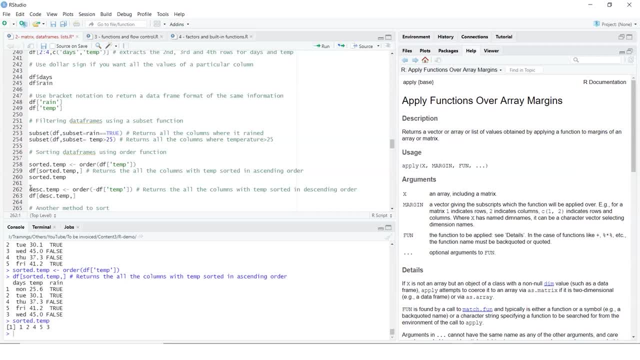 particular values. So we have discussed this in other section also. So what I can do is I can return All the columns with temperature sorted in a descending order. So right now what we were seeing was we were seeing an ascending order, But what we can do is we can do that in a descending order. 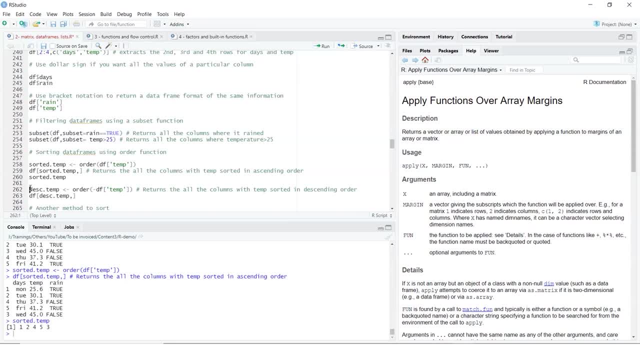 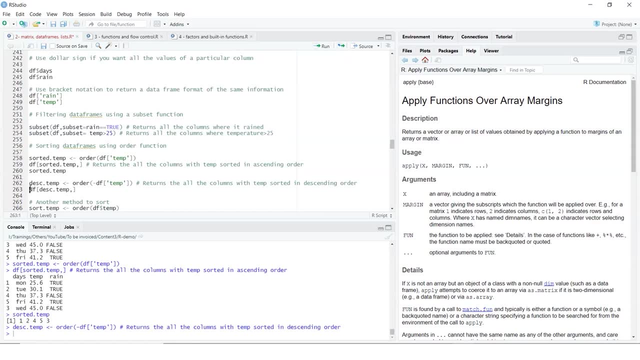 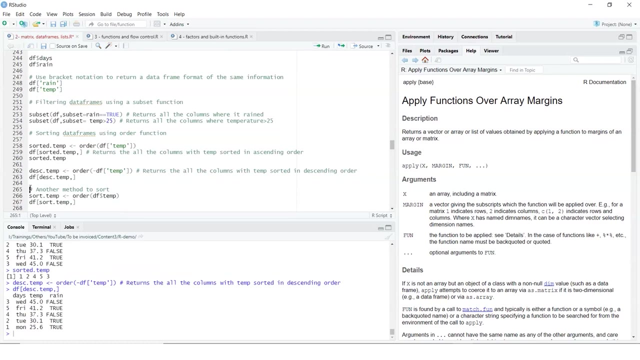 So here I'm creating a variable descending dot temp. I'm doing ordering, But when I'm doing ordering I'm using the minus symbol. And this one, if you would look at in the form of a data frame, it shows me the values which are ordered in a descending order based on the temperature column. 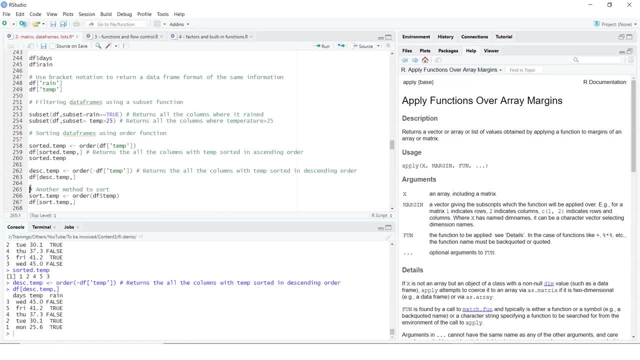 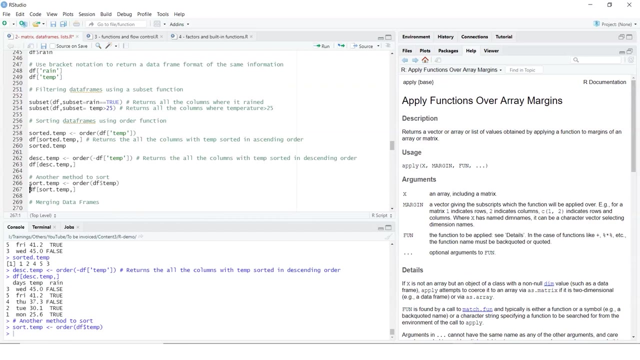 Now, another way of sorting is by using a particular column. So what I can do is I can sort, I can do a order, and then I can choose the column based on which I would want to order it, And then, if you would want to get the values of this, 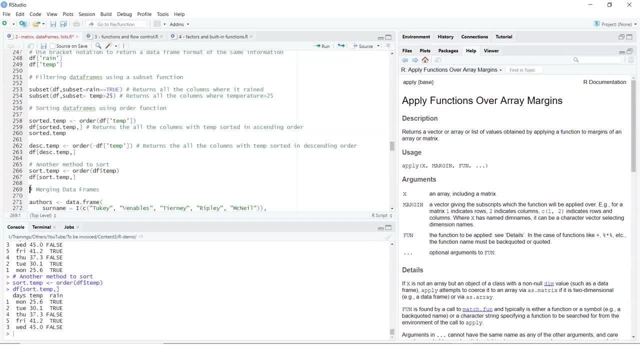 So it tells me the values have been ordered based on temp, So this can be very useful when you would want to sort the data or order it in a particular way To basically understand your data or to make more meaning out of it. Right, 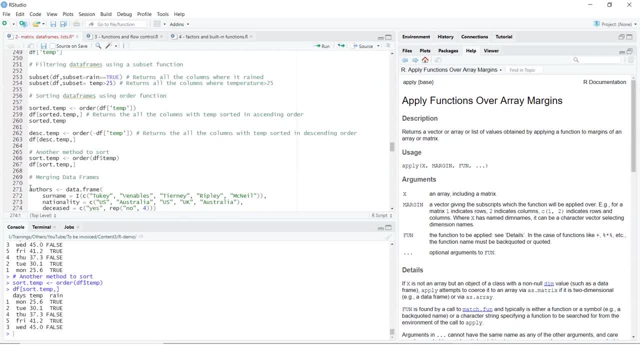 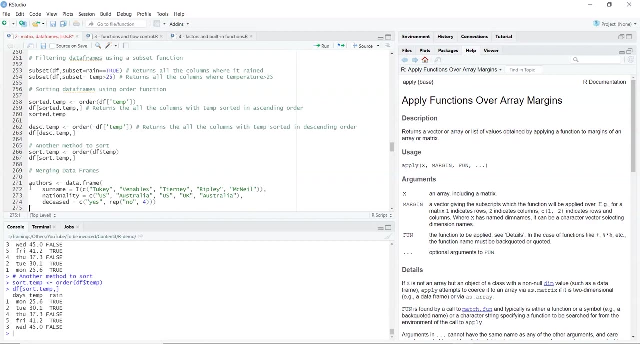 Similarly, one more requirement might be merging your data frames. So here I am creating a data frame, So I'm saying authors and I'm using data dot frame function, And what we are doing is, instead of creating three vectors, I am basically doing that within. 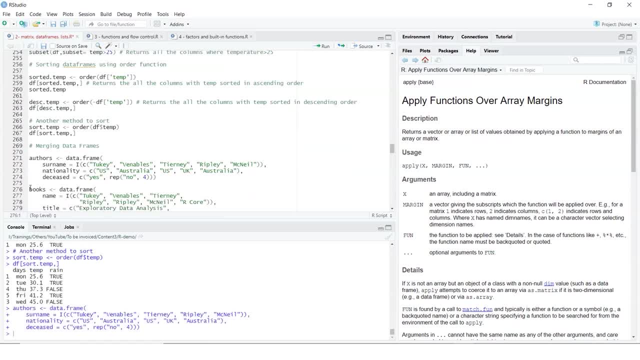 my data frame function. So let's do that. And now what we can do is, at this point of time, I can check my authors look like. so this is my authors now here. if you see, we have the vector turkey- venables, tierney, ripley and mcneil, so that becomes my first column, which is surname. then you have your. 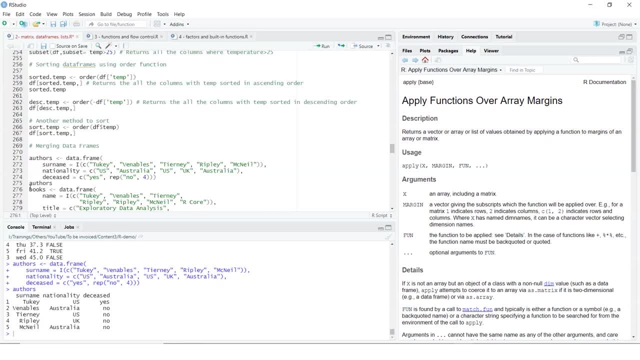 nationality, and then you have deceased, where you have also repeated the values four times. right, so that's something new which you might be seeing. so you are creating a vector where you are passing in a value and for other set of values you are basically using a repetitive function. now, 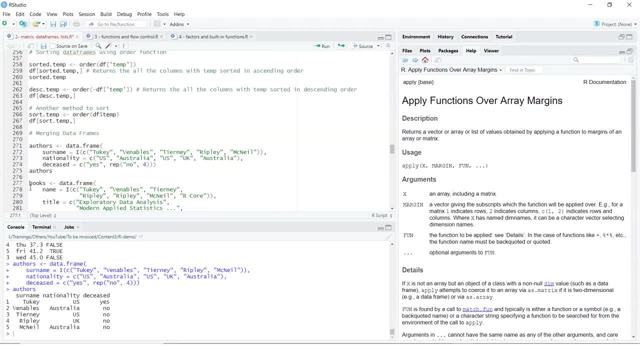 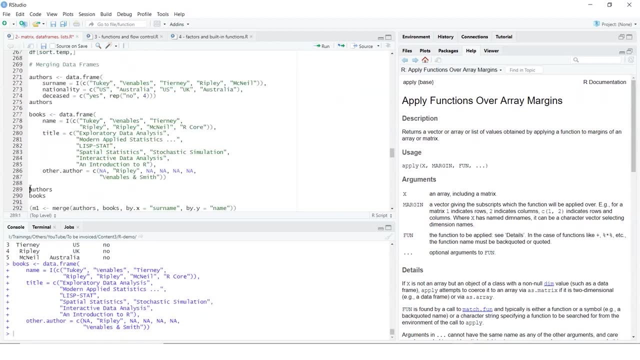 similarly, we can create a data frame called books, and this one is where i am having name, column, title, and then i have other dot, author, and you are passing in the values. so at this point of time, if you would want to look at your books, it would look something like this: so you have given a name. now just closely look at the data. 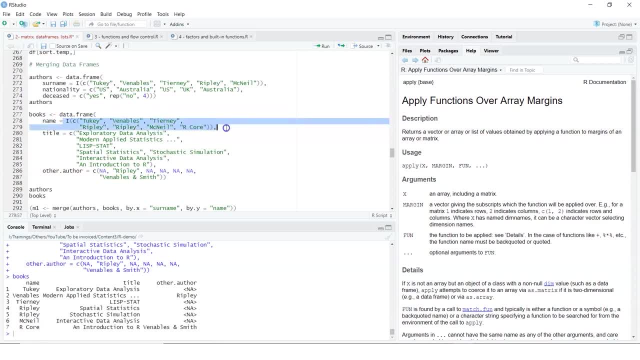 frame function. so here you are using the names, you have the titles, whatever values you are passed in, always remember when you have multiple vectors they are ending with a comma, right, so do not forget that. and then you have other dot author. so that's the name of the column and you are passing. 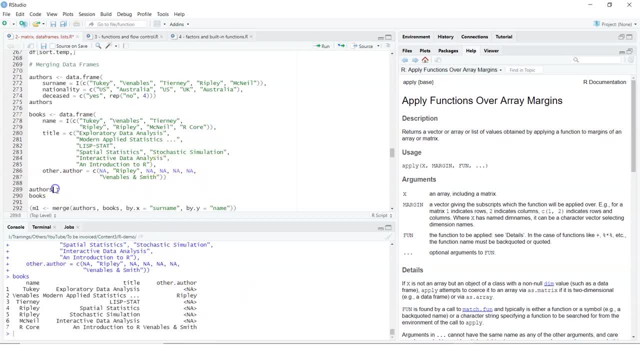 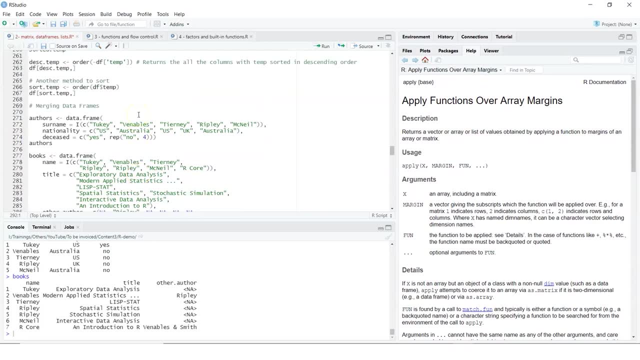 in the values where you have also passed some na values and at this point of time you can look at authors. this is your books and our intention will be to merge these data frames. so that's what we would want to do might be. we are interested in getting the data together. 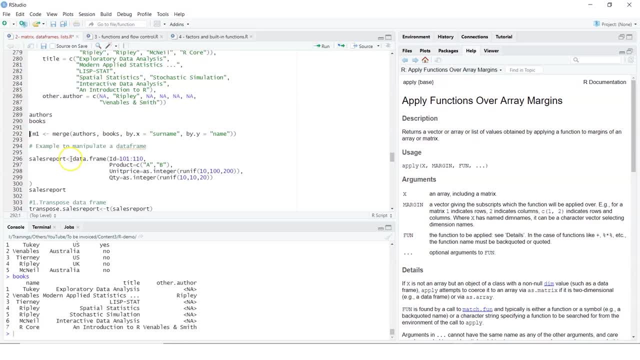 so what i'm doing here is i'm saying m1. now i want to use the merge function. i pass in my data frames, that is, authors and books. so if we closely look at authors, it has three columns and five rows, and here you have three columns and we have seven rows. 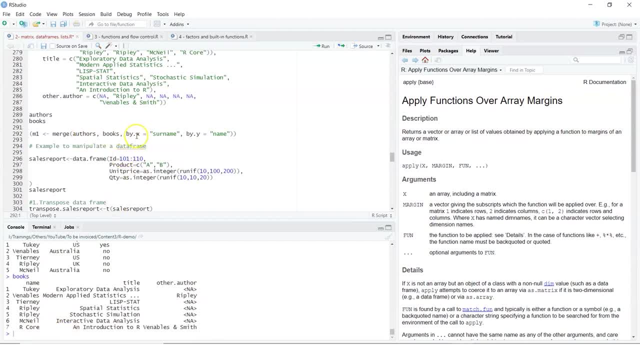 would want to do a merge. so we'll say authors, books, and we will say by dot x. so this is where i'm choosing, which is the column based on which i would want to merge. so i have by dot x, which is surname, and by dot y, which is name. so we would want to merge the data where we are giving a. 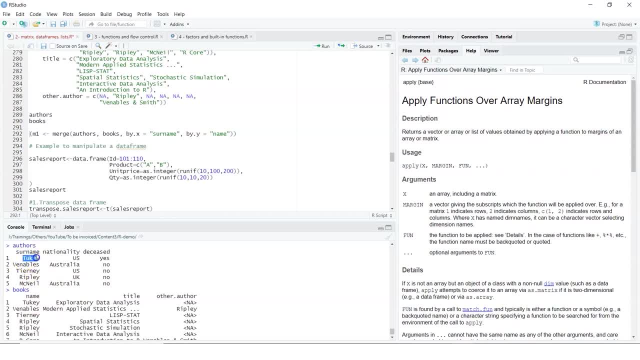 condition based on values and surname and name. so you see, there is turkey here. there is turkey here, we have venables. we have venables, we have tierney, we have this one, we have ripley, which we have here multiple entries, and then you have mcneil. now we don't have r core, which is there in your author. 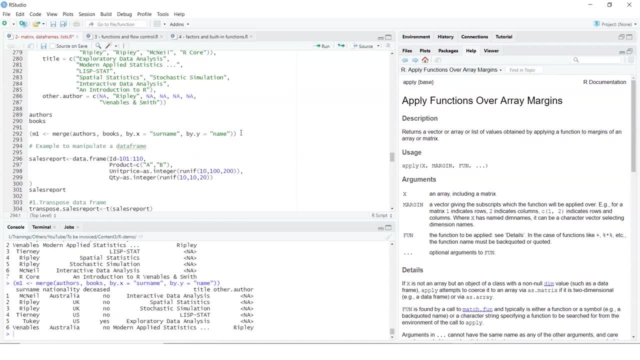 so let's see what happens when we do a merging here. okay, and now we see the result of this merge, where it has taken all the values from both the data frames. so you have surname, nationality, deceased, you get the title, you get the other dot, author, which you 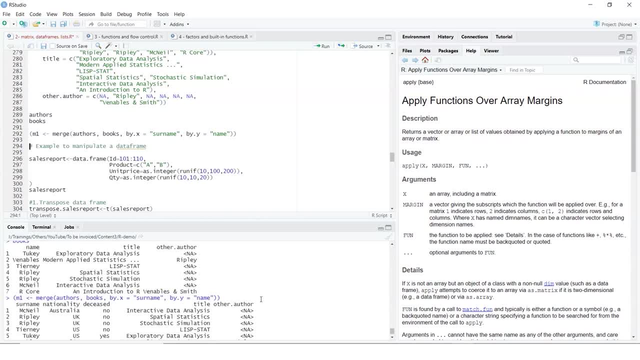 are getting in from your books and the name column is avoided, right, because we are doing the merging based on surname and but y dot name is name, so we don't see the name column. but what we are seeing here is the values which have been merged and then you can compare. so, for example, 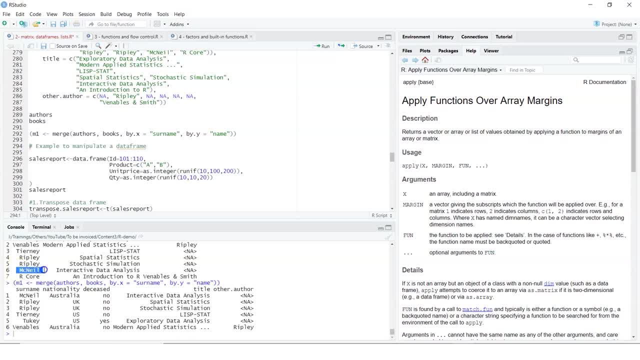 let's do a random check. so if i look at mcneil, that's the surname or here it was named. so you have mcneil, you have a nationality which comes from the first data frame, deceased from the first data frame. then you have your interactive data analysis and then you look at title, dot, author. what you don't look at, 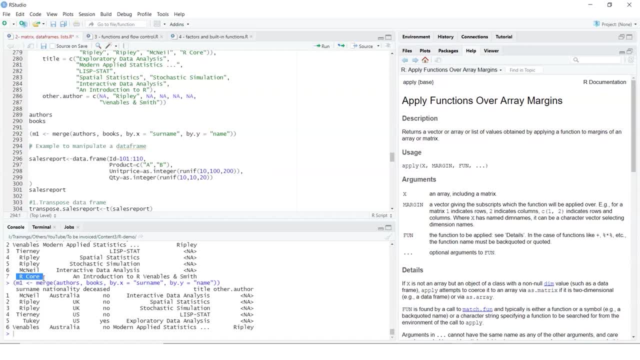 in the merge is this r core, because this does not have any value in your author's data frame. so you can do a merging of your data frames using the merge function. so please try it out and you can create different data frames and try to use this. similarly, you can manipulate a data frame. so, for example, here we are. 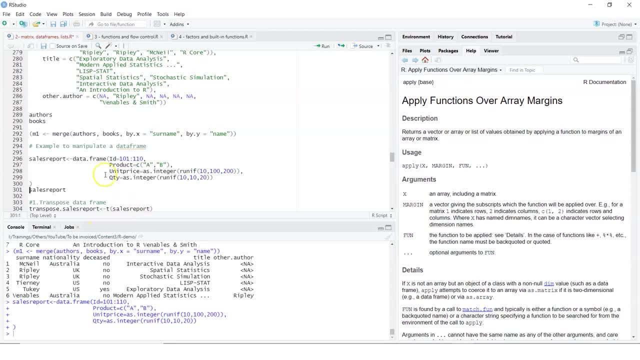 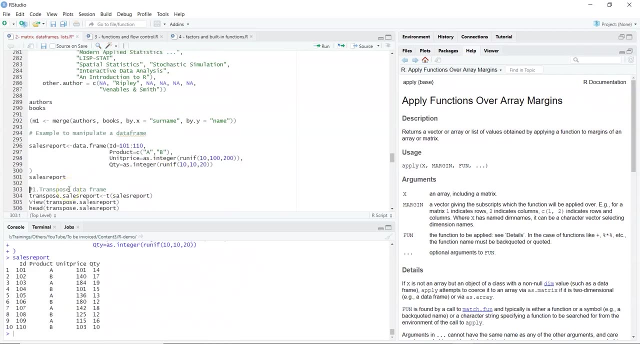 creating one more data frame called sales report, which is dataframe. you are giving an id. product has some values. unit price is where you are getting the values as integer and quantity as integer. so now, if i look at my sales report, this is the values which i have. let's spend a couple of seconds to look at this value. 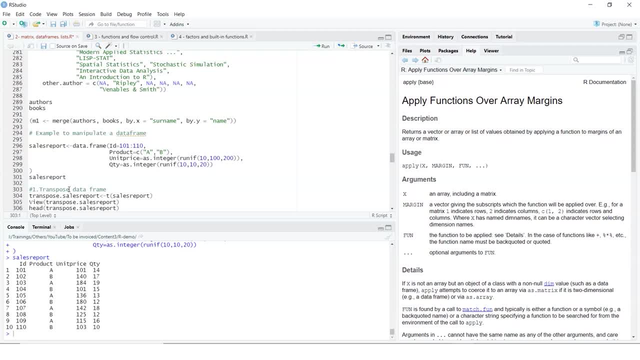 so id value is 101 to 1010, product is a, b, so that is automatically assigned. unit price is starting where you say 101, 140, 184, right, so we are using a as dot integer, we are converting it into integer and basically we are. 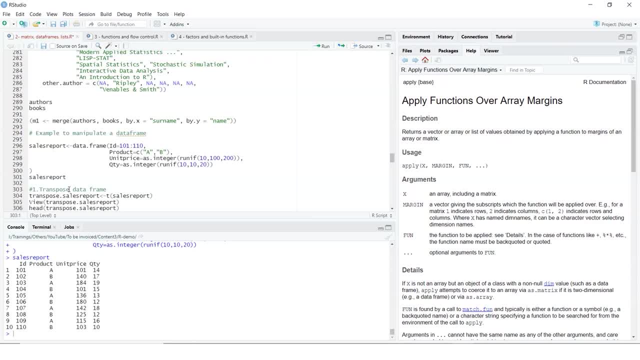 assigning these values here for your unit price and similarly for quantity. we are assigning the values by doing a as dot integer and then just doing a run. if now, once we have done that, we have created a data frame, now how do you transpose? what do you mean by transpose? so transpose is 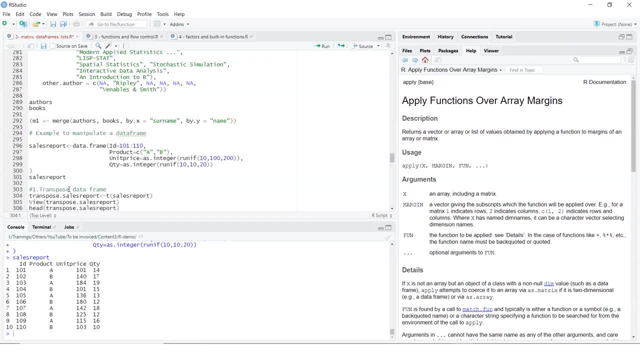 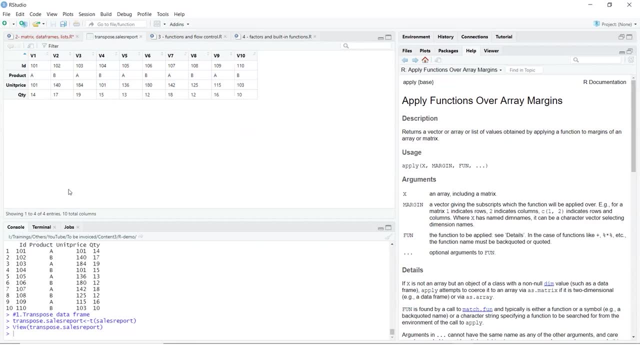 when you are changing your accesses. so if i do a transpose on sales report and if i want to do a view so you will see the positions which have changed, so you have all these values. so my row names or row whatever values, become the column headings and basically your column headings. 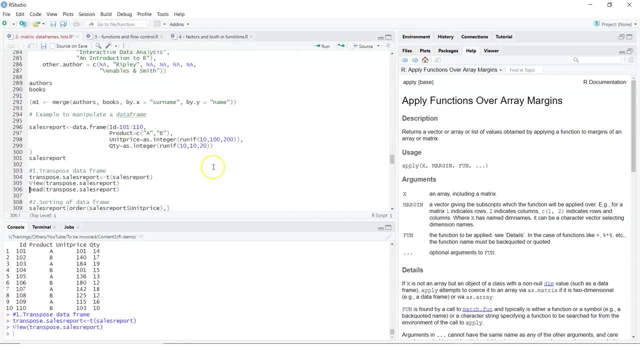 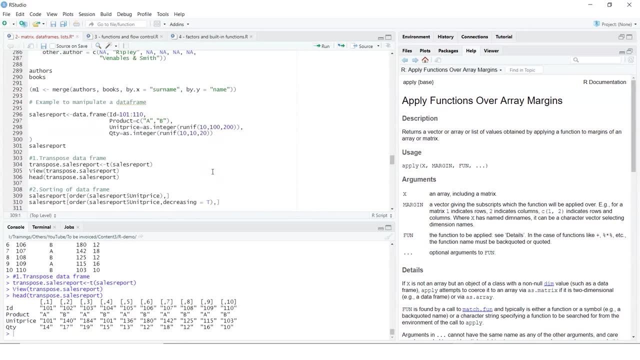 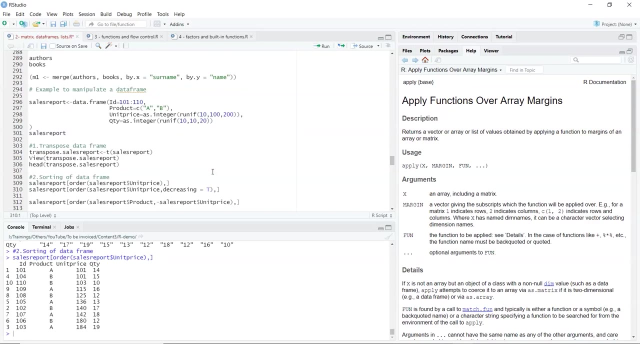 becomes your row names. so that is what you are achieving by doing a transpose. you can do a head to look at some initial values. you can do a sorting of this data frame by using the order function and you can choose the column and also the order if you would want to have it in ascending or descending, or basically increasing or decreasing. 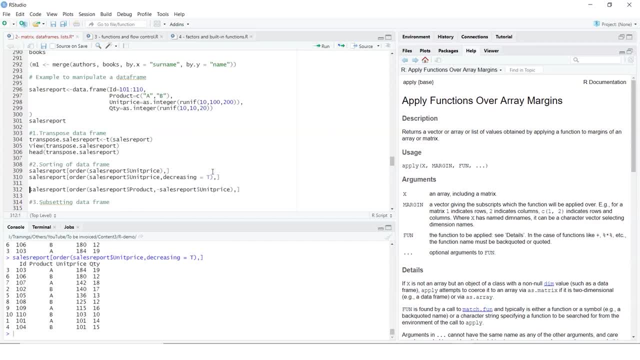 values. you can also choose a particular column, like we are choosing product as a column, and i would want to take the values of sales report in a descending order. that is unit price and we can just do ordering of data frames or sorting the values and data frame. so this is pretty easy. 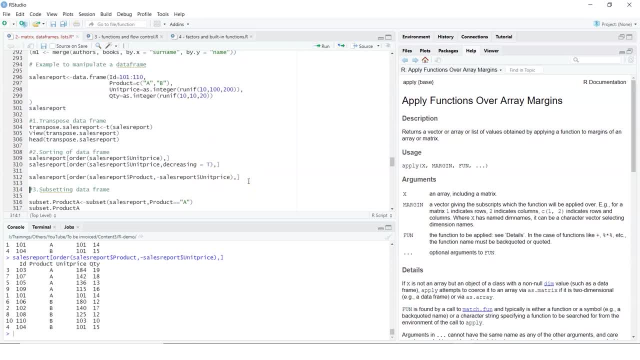 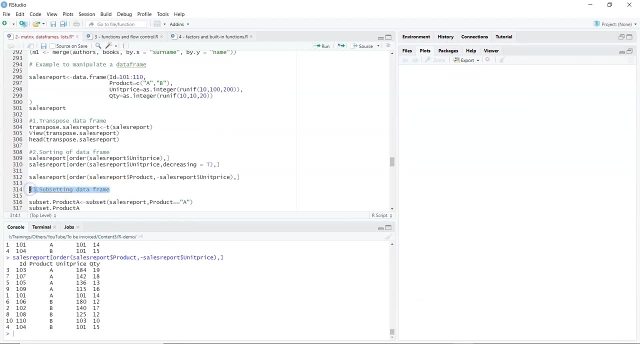 please spend some time in practicing these things, taking these examples, and you will learn more about these functions. you can always try creating an example at your end and you can try to look into these now. what about subsetting the data frame? so when you are saying subsetting the data frame, let's do a subset function like what we used earlier. i will say: 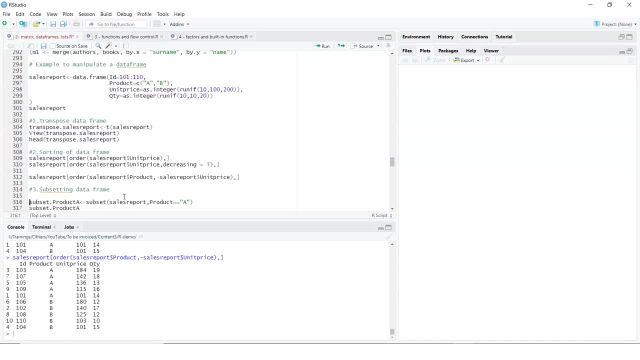 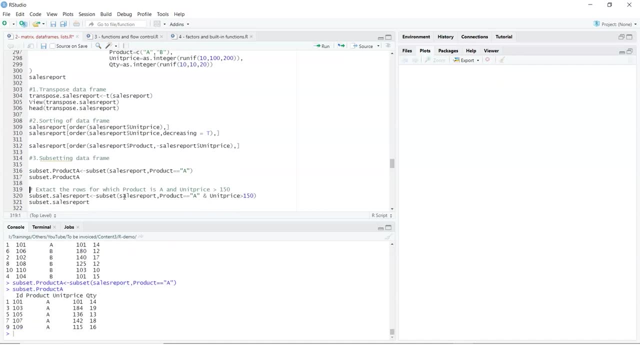 subset dot: product a. i'm using the subset function and here i will get the subset based on the product value being a and i will get the subset function based on the product value being a. let's look at this, and this shows me only the values where product value matches a. 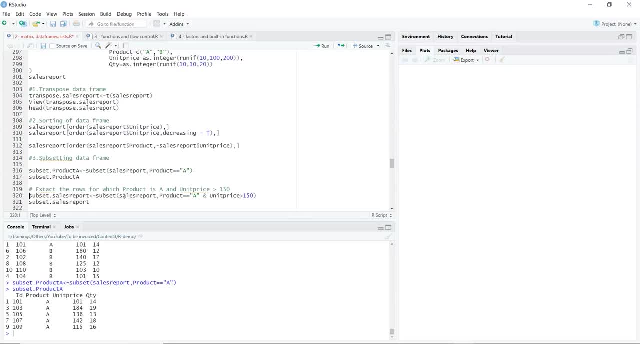 now extract the rows for which product is a and unit price is 150. so you are still doing a subsetting, you are still passing your data frame. here you will give the product is a, which will tell basically the values for product and unit price greater than 50. so you are giving some. 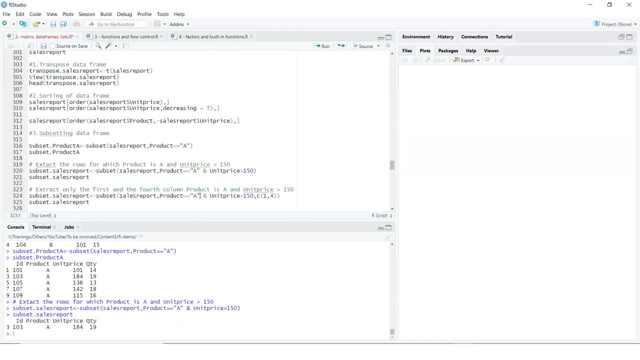 conditions and look at the values now, if you are only interested in particular columns. so if i say only the first and the fourth column, product is a and unit price is 150.. so you have to still use your subset function passing your data frame. product will be given as a and unit price should. 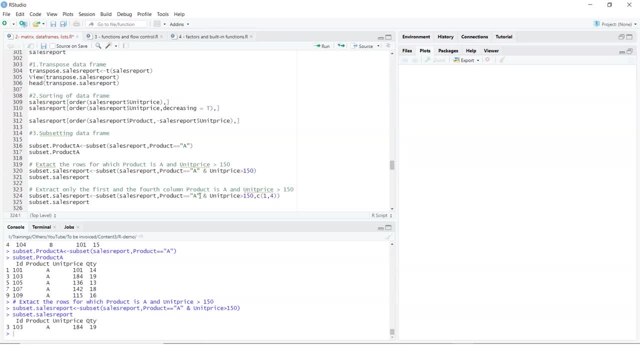 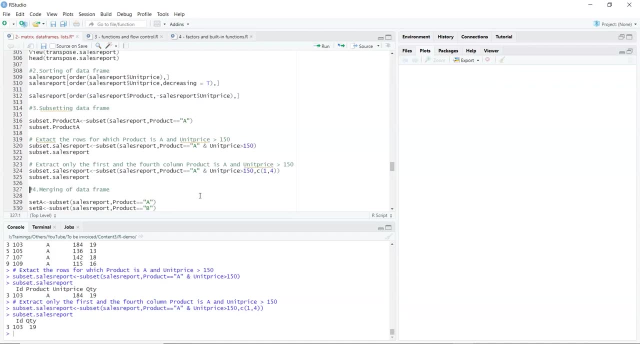 be greater than 150. but what i am interested in is the values from the first and the fourth column, and now, if you see, it shows me the values for my fourth column. what we can also do is we can create two subsets, so set a from the first and the fourth column and then if i go to the second column and i 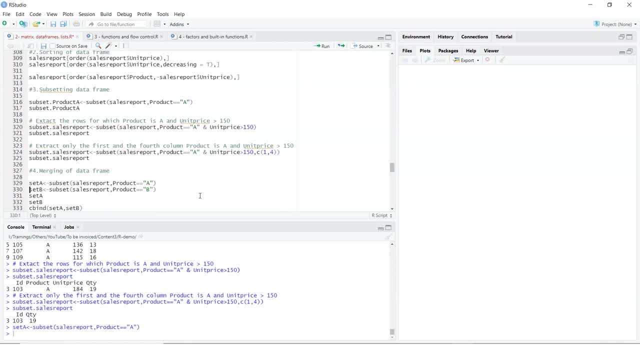 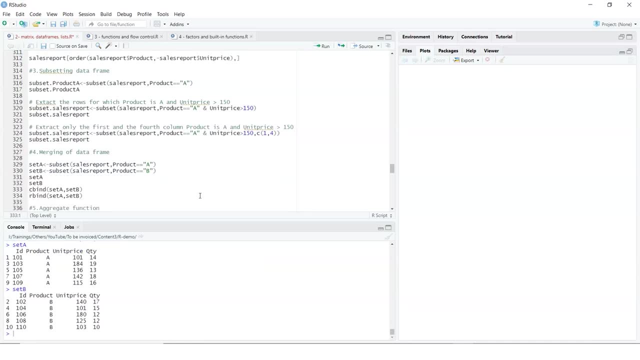 data frame where we take the product as being a other, one is being b, and then we can look at the values. so this is just a, this is just b, and what we can do is we can combine them or we can merge them using column bind. so when i say column bind and i'm saying set a, set b, so it is basically. 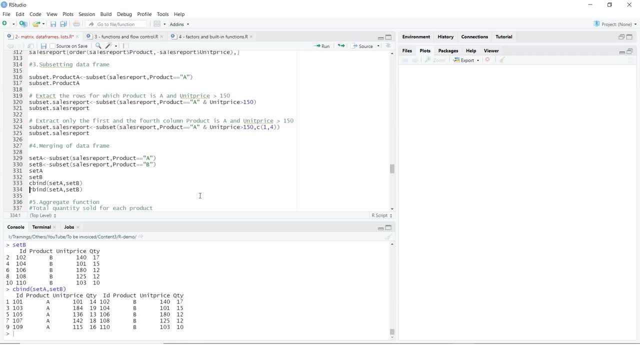 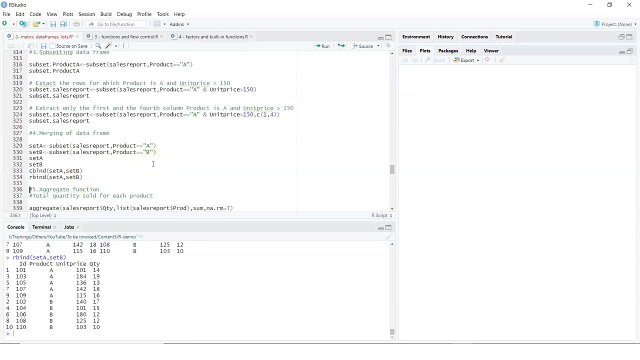 going to stack the data frames column wise and if you do r bind, it is going to stack the data frames row wise. so we can either use column or we can do a row wise. so this is in one way where you can merge. the previous example where we saw merging was based on a particular condition which is met. 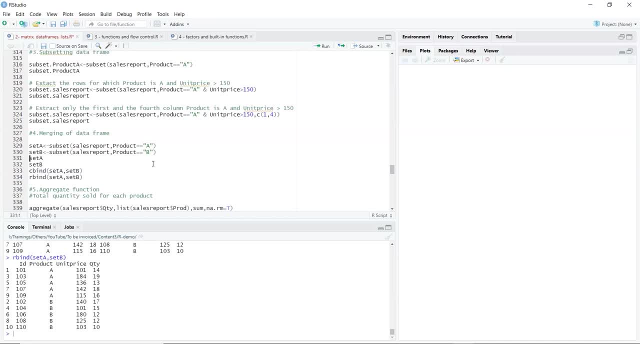 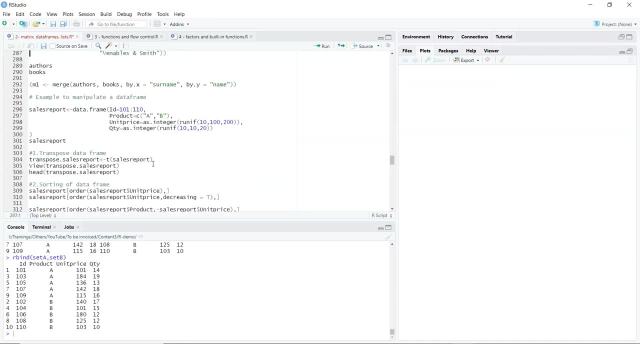 based on some columns which might have similar values. right, and this is where you are straight away merging the data frame using column bind and c bind. so if you compare this with the other merge operation, what we saw here, this was where you are comparing the values of first data frame and second data frame and then merging. but 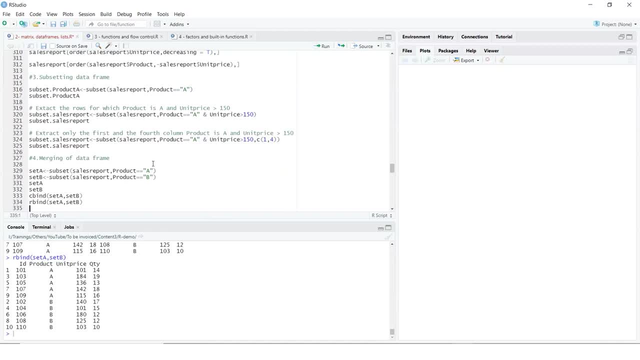 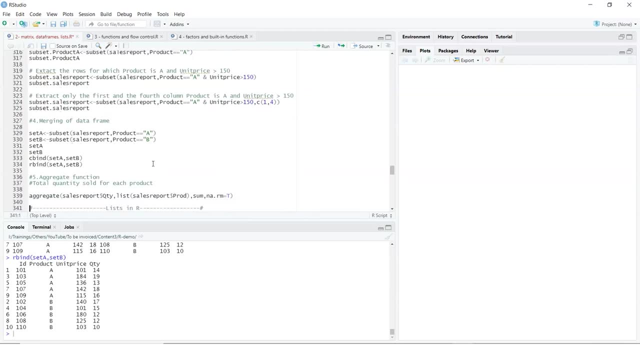 here we have just used column bind and row bind, so we are not merging on a particular condition, we are just stacking them, either column wise or row wise. now what we can also look at is doing some aggregate operations. this is going deeper into data frames. so when you use aggregate function, 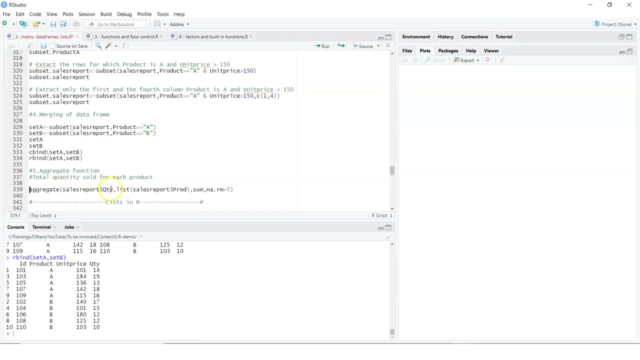 you are passing in your data frame, you are choosing the quantity column and then you are basically using the list function. so list function is going to work on your data frame, on the product column. so product column for your sales report. so at this point of time, let's look at sales report and let's look at the value. 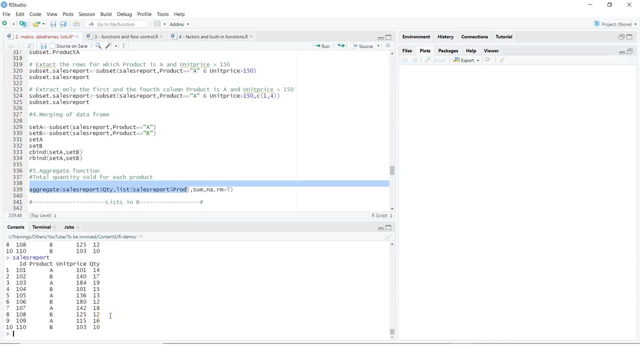 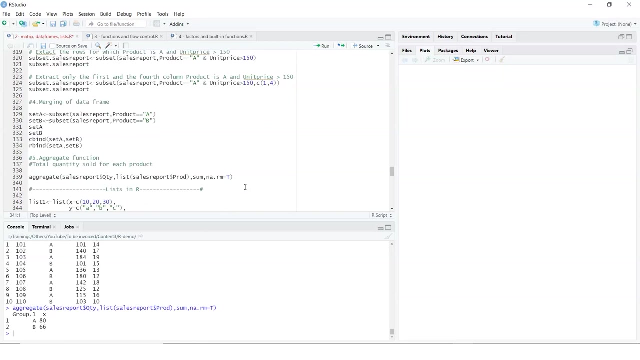 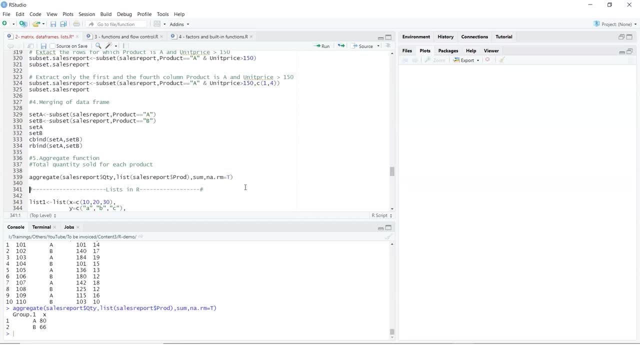 have. so you are kind of grouping by based on product. so we have two products here, a and b. now what we also want to do is we want to take the quantity column, so that's why we have given that first. and what we are doing is we are doing a summing up, so we are summing up all the values. 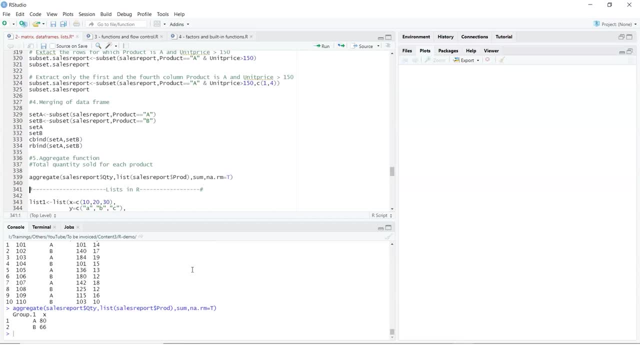 for a and all the values for b, and we are seeing that here. if there are any na values, we are ignoring it. so these are some basic operations on data frames or matrices, subsetting them, extracting useful information, using some inbuilt functions to do transformation or computation, and 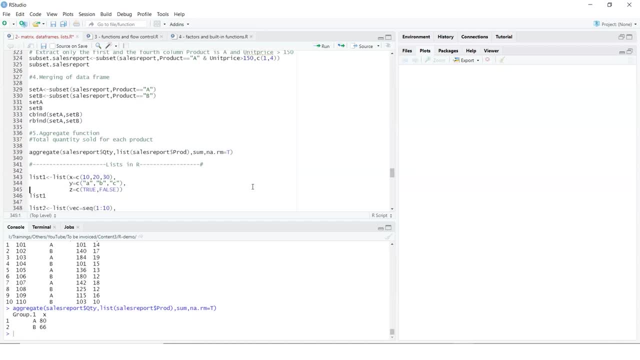 extracting some values now. similarly, we can also work on lists. now that we have looked at data, frames, matrices, vectors, let's also look at one more structure and how we work in r when we have to work on lists. so list is basically a structure here and what we are doing. 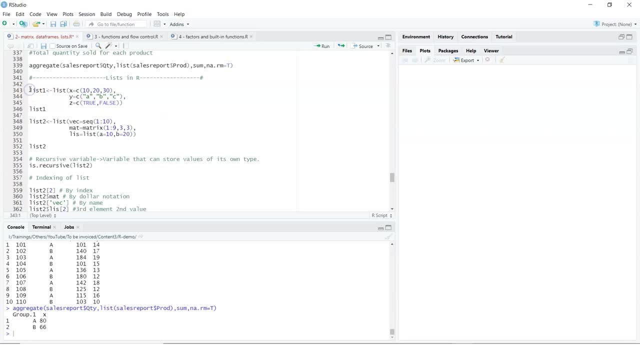 is, we are creating a list by using the list function, and here i am passing in three vectors. you see here now c function is being used now in vector. we know that all the elements are of the same type. now let's create a list wherein we see three vectors which are of three different. 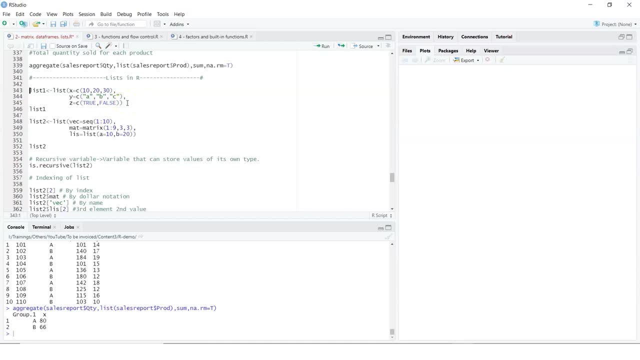 types or, obviously, objects of three different types. so let's create this list. and now let's look at our list. so it basically has elements wherein you have values of different types. we can create a different list which can also have sequence elements, that is, one to ten, a matrix which is of three dimensions. 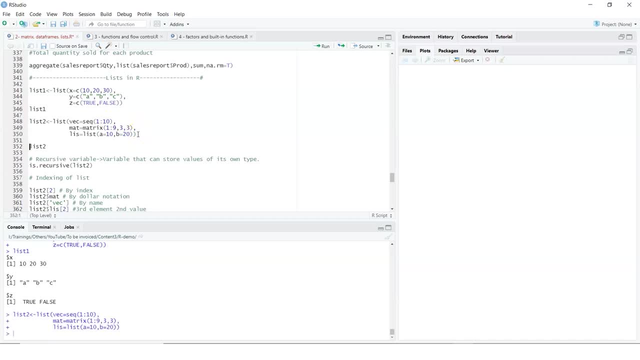 and then also passing a list. so this is also one way of creating a list. let's look at list two and if we look at the values here, we have a list of three different types. so let's create a list here. list two basically has a vector which has values one to ten. it has a matrix of three into 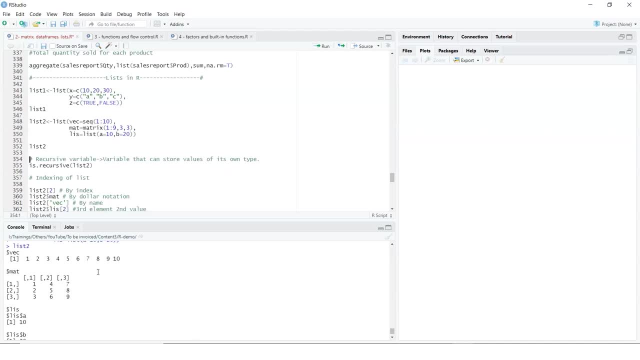 three, it has a list which has values- a having ten and b having twenty. so this is how you can create a list which can have objects of different types. so we can also use recursive variable, a variable that can store value of its own type. so for that you have to use a recursive variable that can store 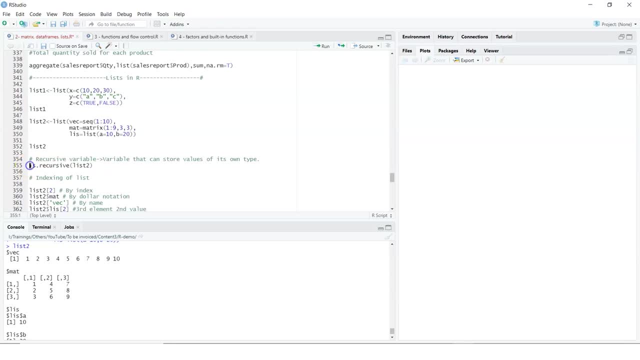 value of its own type. so if I use a recursive function, something like this, so I am saying is recursive, and then do it on your list and we can check if the list basically has a variable that can store values of its own type. now, one of the main requirements when you are working with lists: 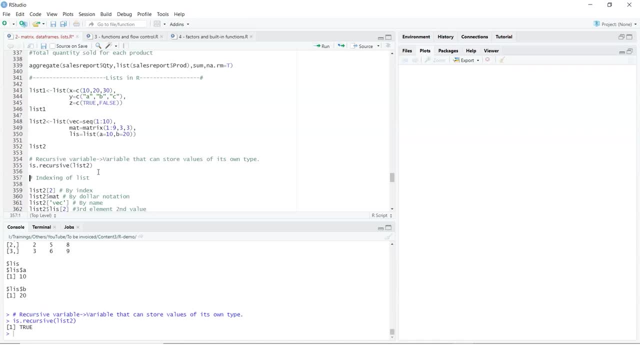 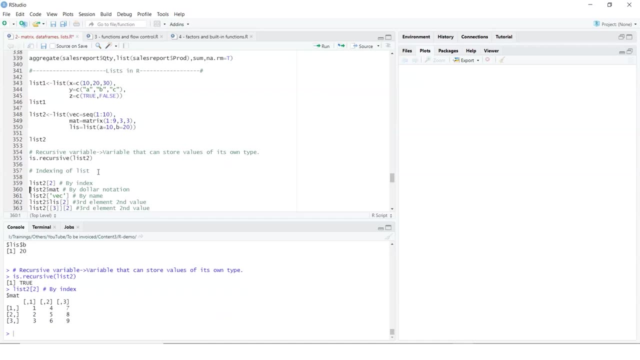 is indexing. so I have created a list and here I can access this elements by using index. so if I do this, this shows me the matrix. what I could have also done is using the dollar symbol and then choosing particular element of the list by doing a mat, which is the name given to our matrix. 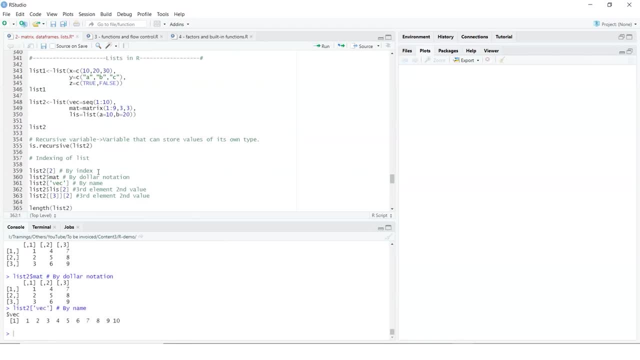 or by choosing a name. that is vector, so you can access the elements using indexing or dollar generation or giving the name of a particular element. now I can also work on list and I can get the third elements, second value, so we can do that and that shows me 20, or you could have done. 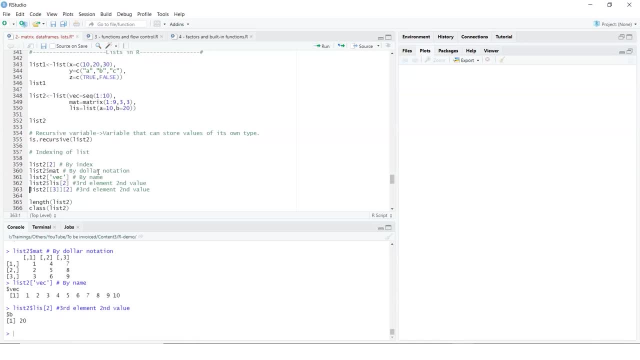 by giving the value 3. that is the third element and within that you are looking for second element. so I can get the length of the list, I can get the class of the list which shows me this type list, and what I can also do is I can convert vectors into list. so here we are creating a variable. 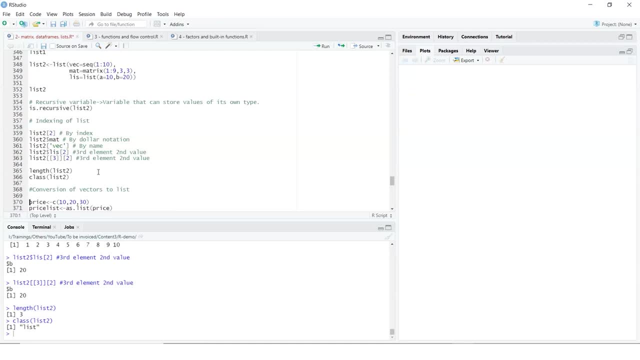 pattern, price, which is being assigned a vector which has 10, 20 and 30. and now what I want to do is I would want to convert this vector into list, and for that I'm using the list function. so I am creating a variable called price list and then I am saying as dot list, so that's going to convert. 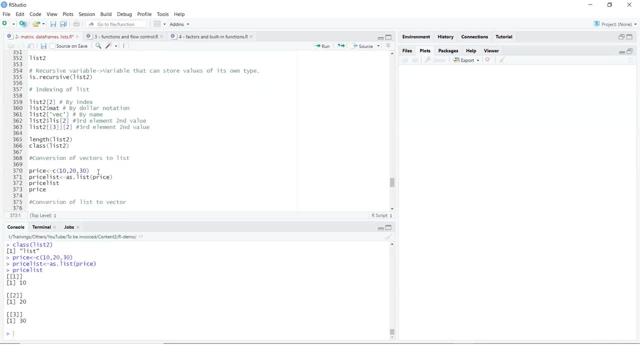 my vector into list. and now let's look at price list, which shows me a list, or you can look at price, which is a vector. so that's when you are converting your vector into list. now how do you convert your list into vector? and that also can be done by doing a unlist function, so I can basically 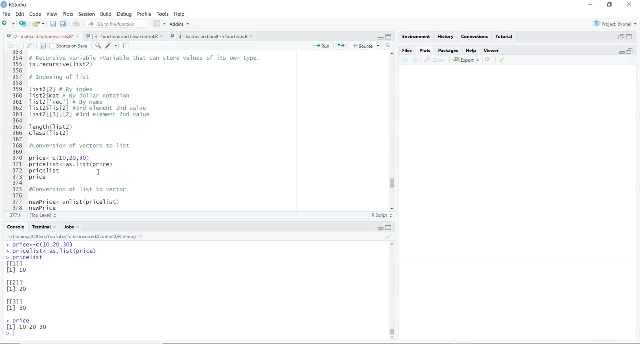 work on price list, wherein we converted vector to list and I can just do a unlist on that, which will convert my list into a vector, looking at the values of the vector. now, sometimes we may want to get the dimensions, so we can use the unlist function to convert the list into a vector and 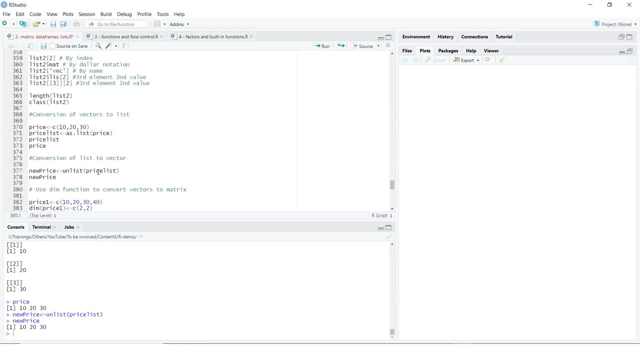 use the dimension function to convert the vectors to a matrix so that it can have multiple dimensions. so here we create a vector which has four values, and then I am going to give a dimension to this, so that it is converted from vector into matrix by giving dimensions 2 comma 2. and now, if you 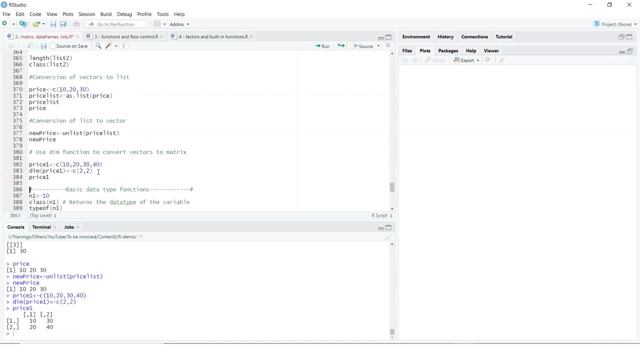 look at price 1. it has basically changed into rows and columns of 2 into 2 dimensions. so these are some simple examples of working with the unlist function. so let's look at price list list. now, when you talk about basic data type functions, we have seen how you use the assignment. 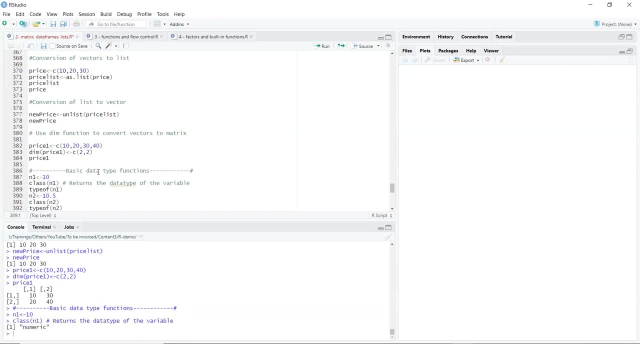 operator how you get the data type of a particular variable or the class to which it belongs. I can assign different values, such as 10.5. so the previous one was showing me the value numeric, and now what we would want to do is we want to assign a value, 10.5. look at the class of it. it 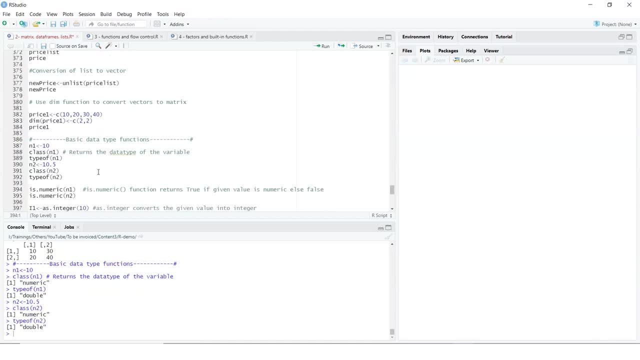 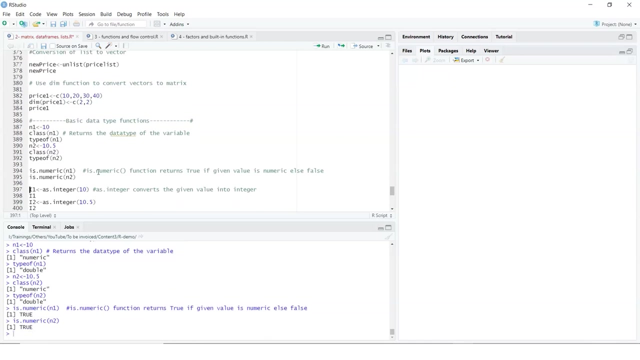 is numeric type of. it shows double, so by default it belongs to the double class. now I can check if the values in n1 are numeric, and that shows me true, and similarly for n2, and that shows me 2. so you are using the numeric function, which returns true if the given value is numeric. 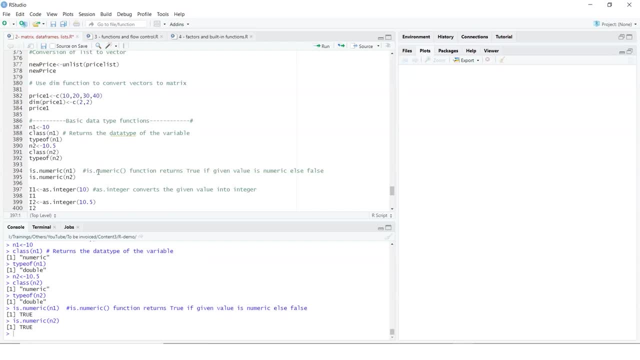 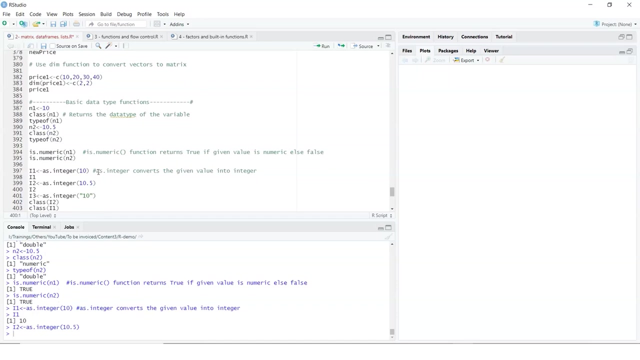 similarly, we can have integer assigned to a particular variable and for that I am going to do an integer and I can do asinteger, or I can assign a value with capital L. so I can do this and look at the value of i1, similarly i2, and look at the values and if I would want to check if that 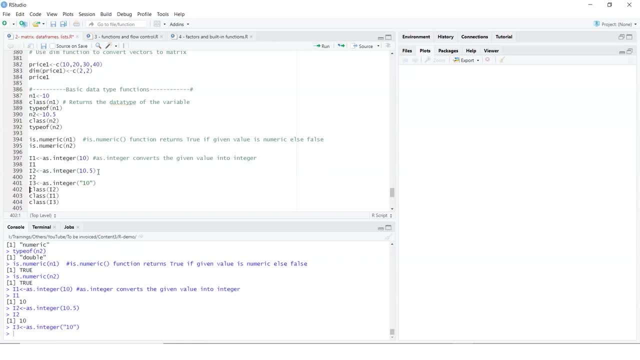 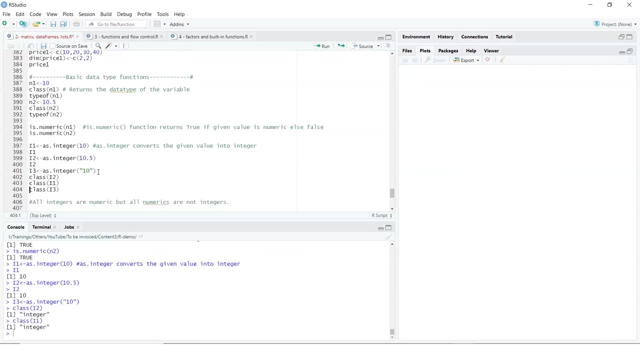 is an integer. let's look at the values of i2, which was an integer, i1, which was an integer, and i3, which is an integer. so here we have assigned integer values to a particular variable. now all integers are numeric, but all numerics are not integers. so 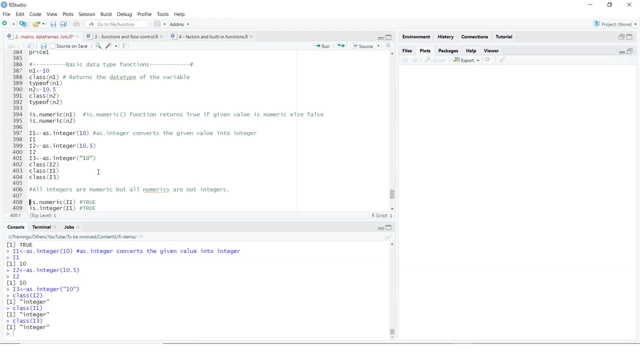 let's check that. so if I do a is numeric on i1, which was assigned asinteger 10, that shows me true. if I say isinteger on i1, so was that an integer. and if I look at the value, it shows me true. now let's look at the character values. so if we say c1, c2, and look at the class, 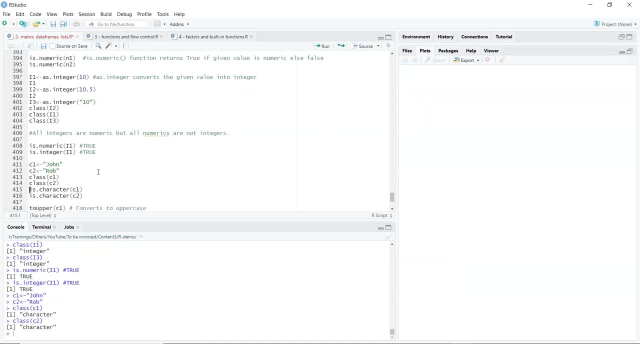 of this. it shows me it is of character type. similarly on c2, and you can always validate that by using the character function. you can also use some inbuilt functions, such as converting to an uppercase or getting a substring. from the starting till the position: what you would want, the elements. 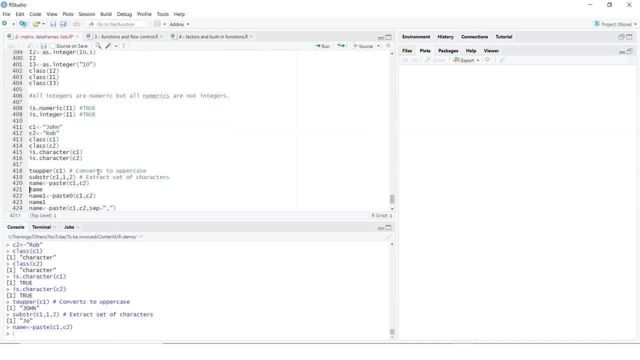 I can do a paste function which basically will give me the data combined, or you can say concatenate. You can also use a PACE 0 which we know will get rid of the space and it just concatenates them without a space. I can also use a specific separator, which we have seen examples, and we can do that and 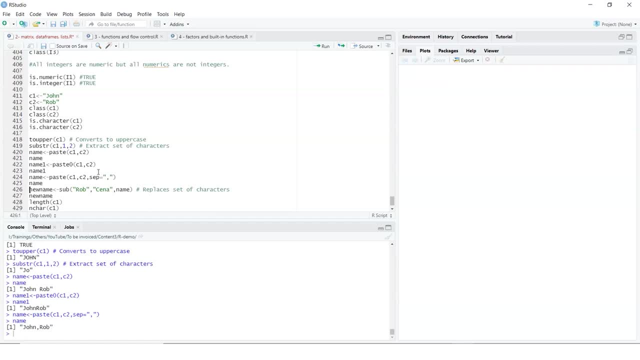 what we can also do is we can replace set of characters. So here I am saying substitute and then if I look at the values, it has basically replaced Rob with Sena, and let's look at the length of it or number of characters in this. 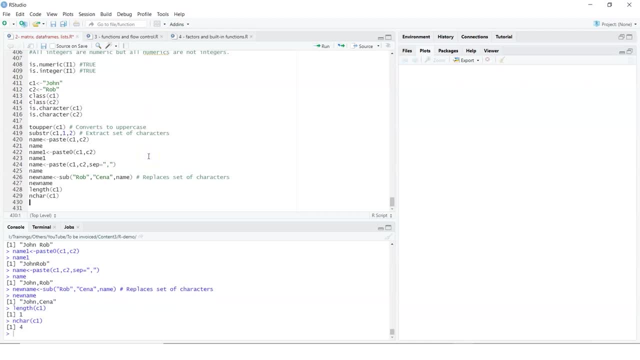 So these are some basic operations, what you are doing on matrices, on your data frames, on your lists and also on your variables, where either you are assigning them values of a particular type or you are changing the data types. You can also go for coercion in case of vectors. we have seen that where, if you are passing, 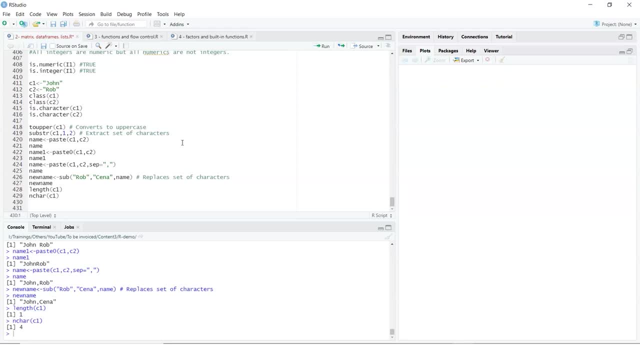 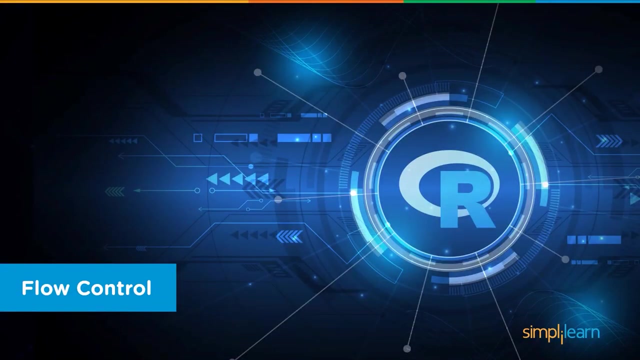 in values of different types, that's coerced into same types. So later we can learn more on functions and flow control and how that is handled in R. Let's learn how R can be used to take care of flow control. that is if I would want to. 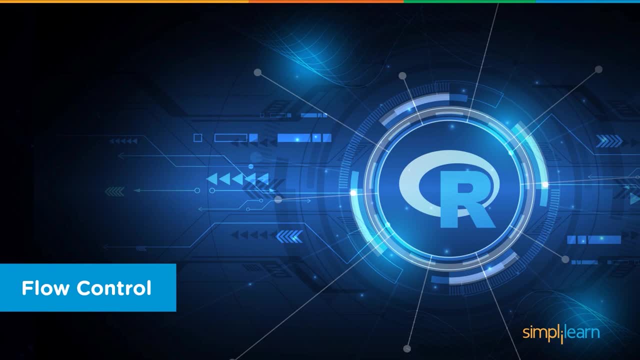 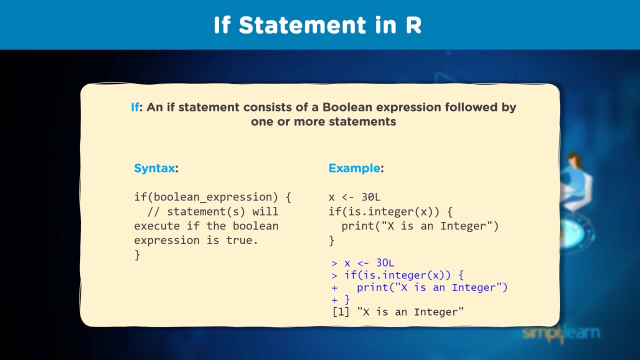 have a if else condition and if what I would want to compute or if I would want to check some values, how R can be used If statement consists of a Boolean expression which is followed by one or more statements. So we can just say if we can pass in a Boolean expression where we would want to compare. 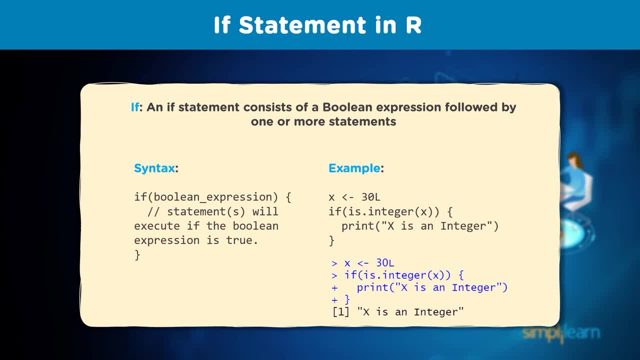 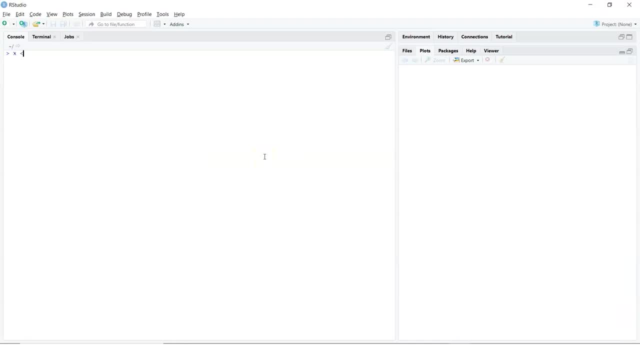 particular value, or we would want to check a particular value, and then whatever is passed in the statement will get executed. So what we can do is here we can use assignment operator. I can pass a value to x. now we can always do a type of 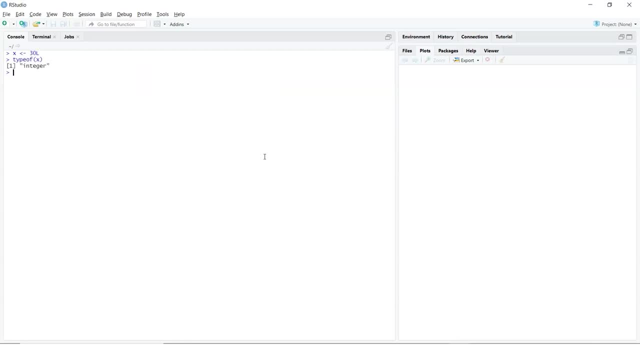 And that can tell me that x is basically an integer. and now I can use my if where I can say is dot, and then I can choose integer and I would want to check the value of x. if that is an integer, then I will just use brackets and I'll pass a statement here. so let me say: 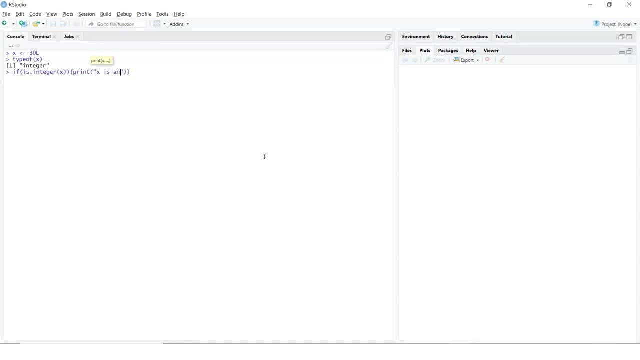 print And let's say, x is Is an integer, and we can execute this and this tells me that the Boolean value is true. Now, if, for example, we would have done something else, or say, for example, instead of integer, if I had used, let's say, character, for that matter, and we can check the value and we can. 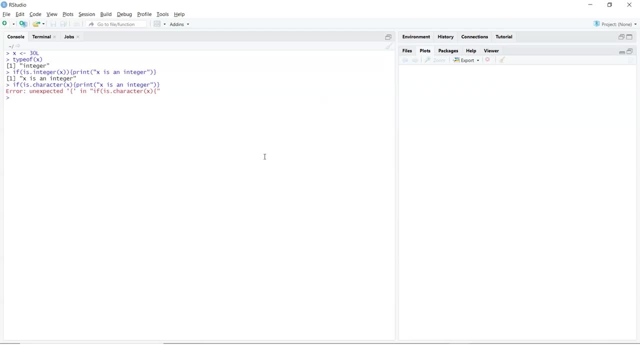 do this. So here we will check the value. So and it says there is an error with the bracket. and let's check this one. so if x, because we missed a bracket here, So let's do that one and then try this, and it doesn't show me any result. 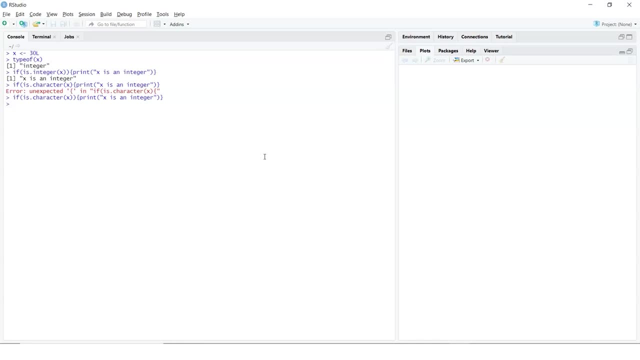 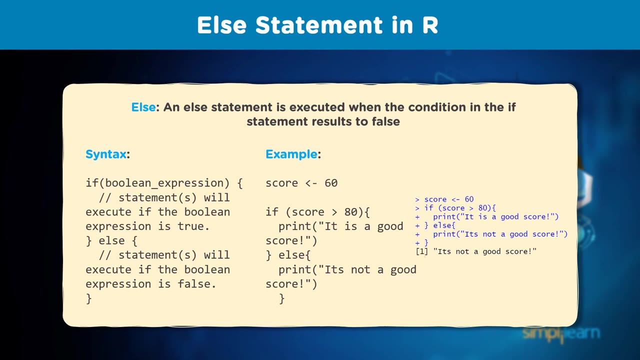 So how could we handle something like this: if the Boolean expression does not match to true, and in that case we can always go for else statement, so we can check for a value. So if the Boolean Expression is true, statement will be executed, and if it is false, then next statement will. 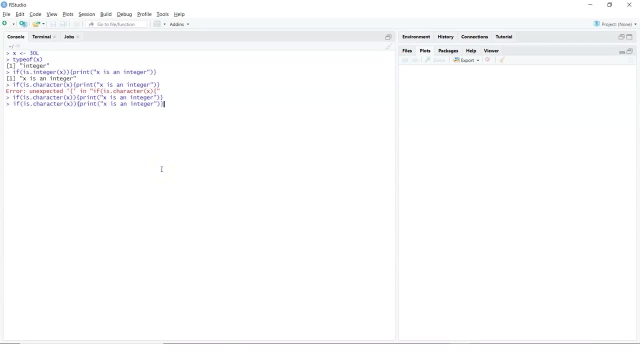 be executed. so we could have done the same thing here, where I said print x is an integer, which we know is not true, and what I could do is I can, here after this one, Say else, and then I can open up one more bracket And then I can say print, and I will say x is not a character. 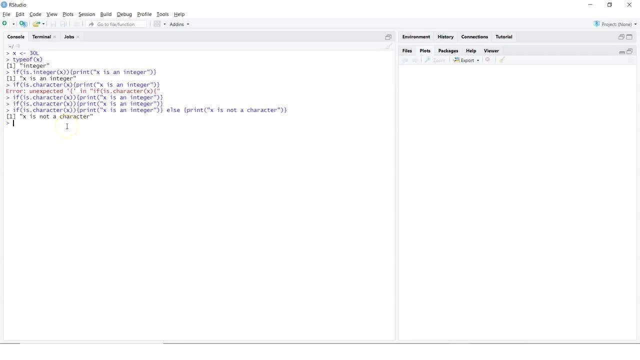 And now we know that x is not a character. So this is a simple way where you can use if else and you can control the flow by passing in the conditions. Now, that's when you are using if else statements. Now, what about while loop? 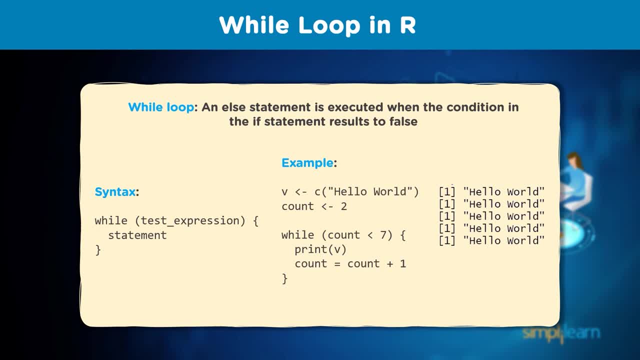 So that also can be useful when you are programming in R. So an else statement is executed when the condition in the if statement results to false. So that basically means what we can do here is let's pass in a word or a set of words. 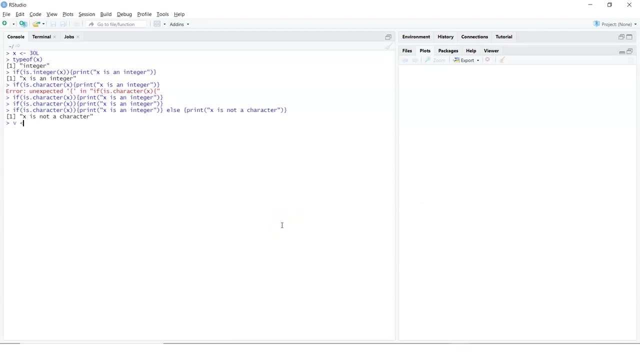 like this, For example: let's say v and then we use C function to create a vector, for example, and then I can just say: hello world. And If you look at v, You can look at the class of v- It's of characters. and if you look at type of v, 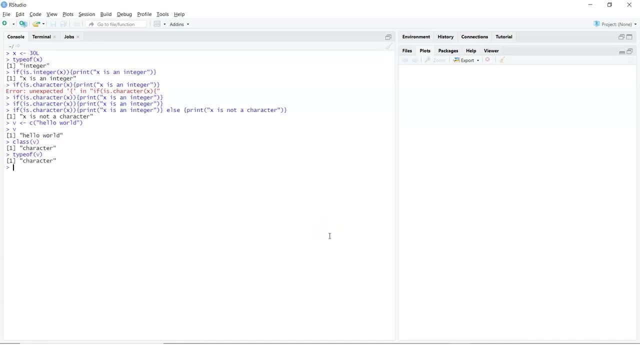 It is having the objects or elements as character. Now what we can do is we can basically then say: count, and let's assign this a value to. Now what we would want to check is: is the count of elements in our v Equals to two? 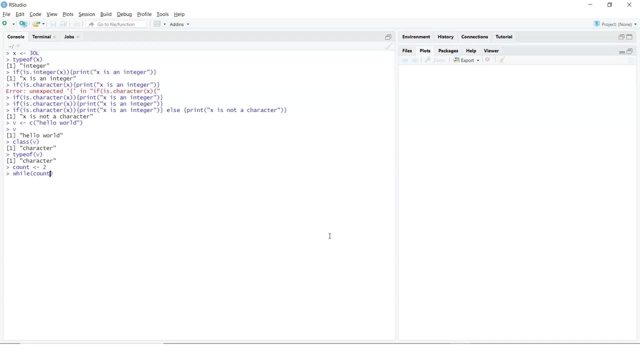 So what I can do is, while My count is less than, Say, five. Now I'm saying I would want to do something while the count is less than five, So we have already given a value to count as two, And now what I can do is here I can open up a bracket, I can say print and then pass the. 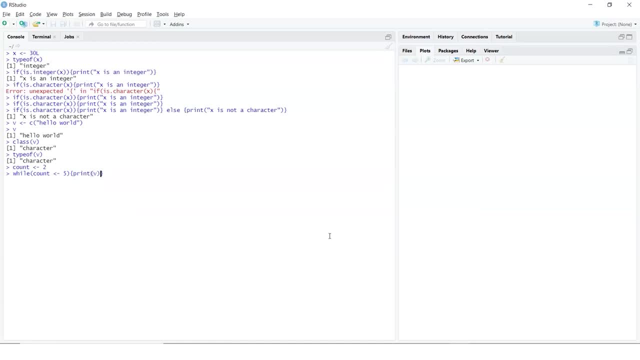 value of v. and then what we do is not only this, we will also increment the value of count and we will say count plus one. And here it gives me error, probably because we have missed a bracket. So let's see what we are missing out here. 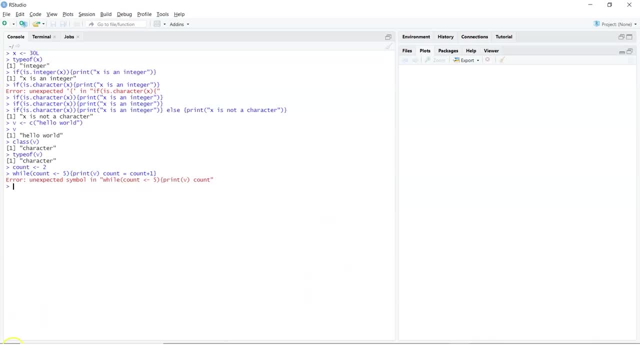 So let's just check this one again. So here it is. We have created v, which has two elements, So Of the type character. and then what we do is we assign count a value of two and we would want to check while the count value is less than five. we would want to print the value. 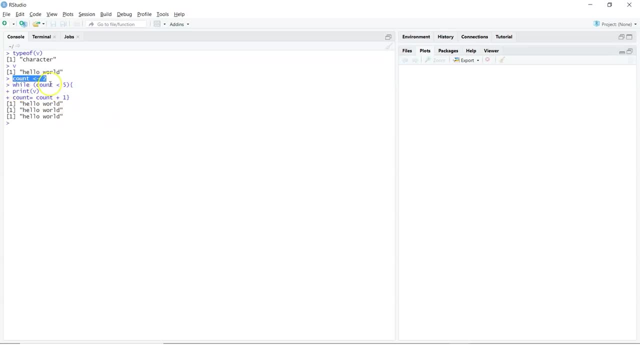 of v. So what we are doing here is we are saying while, then you pass in an expression which will check the value of count, we do a print and then we increment the value of count. Now this is a simple example where you are using while. 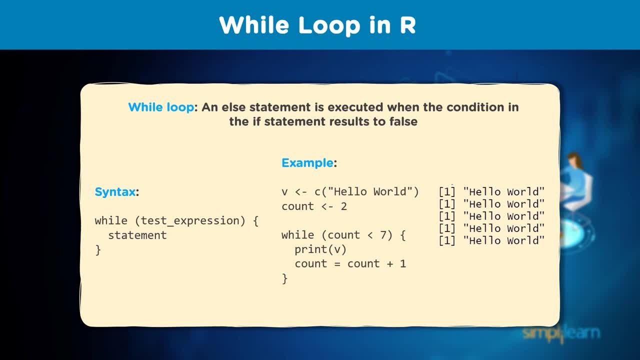 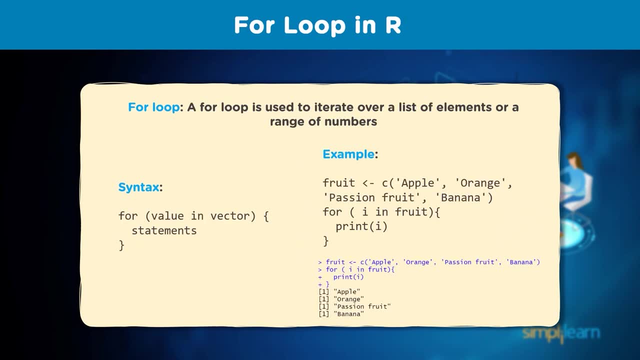 To Test an expression and while that expression is true, you would be doing something, whatever is passed within your brackets. Now we could also be going for for loop. Now, for loop is basically used to iterate over a list of elements or a range of numbers. 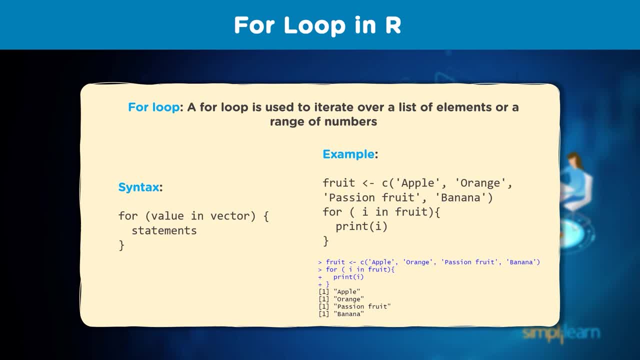 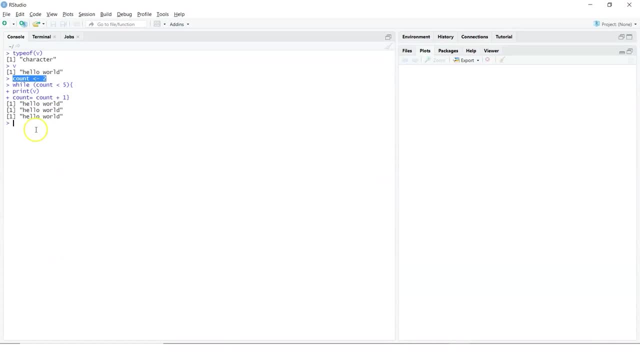 So, for example, if I have a vector like fruit which has some values, I could just say, for I in fruit, I would want to print something. So let's try this also as an example To Test our for loop. Now we can just say names and we can basically then assign values to this. 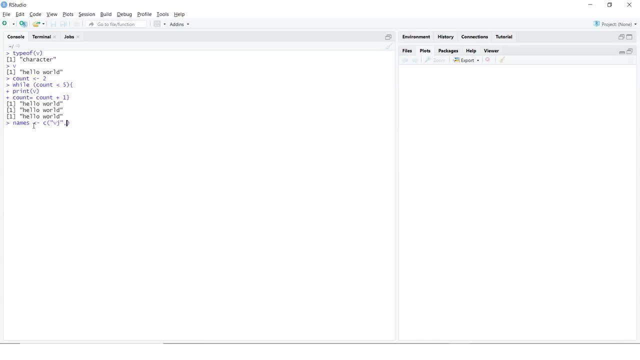 So let's say v? j, a, j, d, j and let's say s? j, and let's create this. Let's look at the value of names. Now, what I can do is I can use a for loop and I can say for I In. 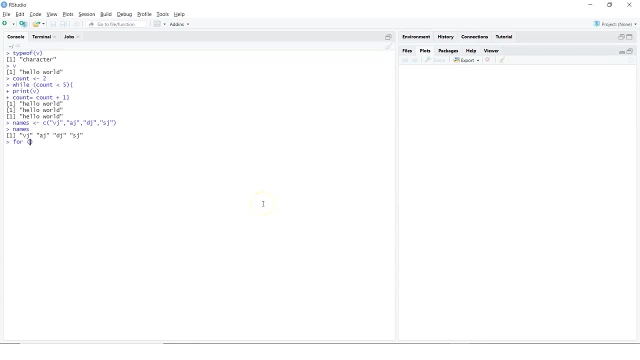 For I In My Names. So I will say: for I In Names. Now, what do you want to do? So open up your brackets here, and then we would want to say: print I and then basically close the bracket. 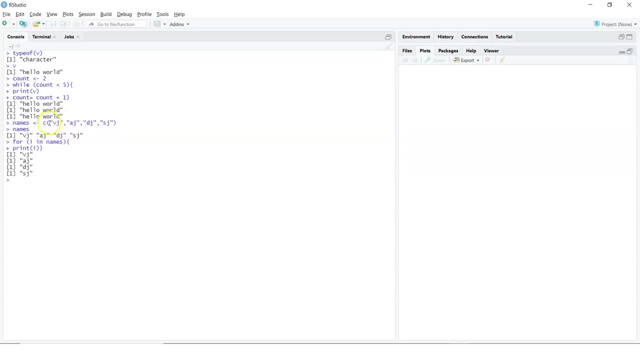 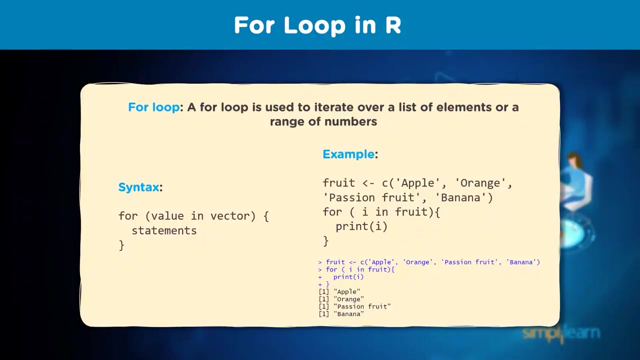 So you see, for every element in this vector, it is basically going to print the name one by one. So you are iterating through a set of objects By using a for loop. Now, this is how we can work on for loop. So, if else, while and for loop can be very useful when you would want to iterate or when. 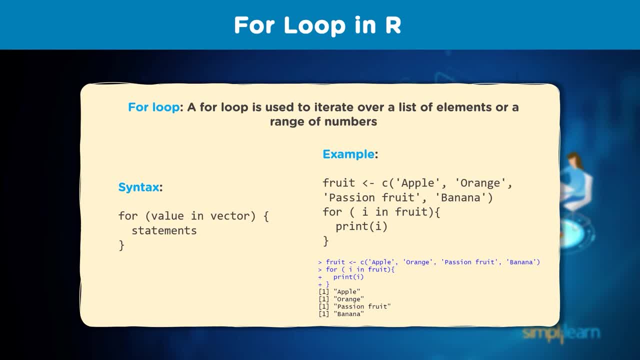 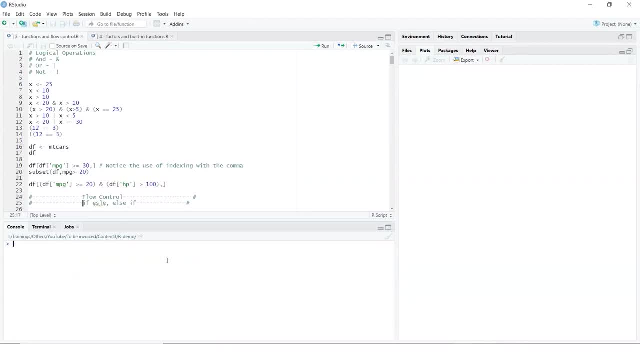 you would want to check the value of an expression or when you would want to loop and do a particular task. It's always good to understand how you manage flow control in R. That is either is either when you're working with your for loops, your while loops, also understanding how you can. 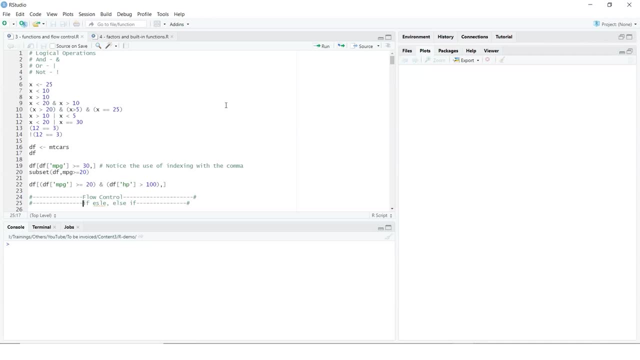 use your logical operators for working with your data in r. so let's look at some examples and understand logical operations. so either you could be having and, or you could be doing a, or where you're evaluating one condition, or you're using not. so these are your logical operations now here. 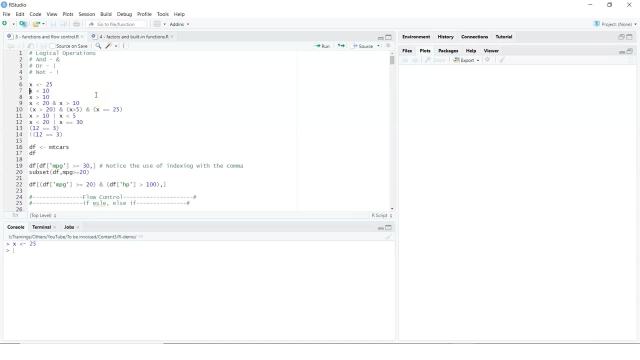 i can assign a value to x and then i can check if my x value is less than 10 and it shows me false. so i have been checking the value of x, so let's see: is it greater than 10? and that's true. now i 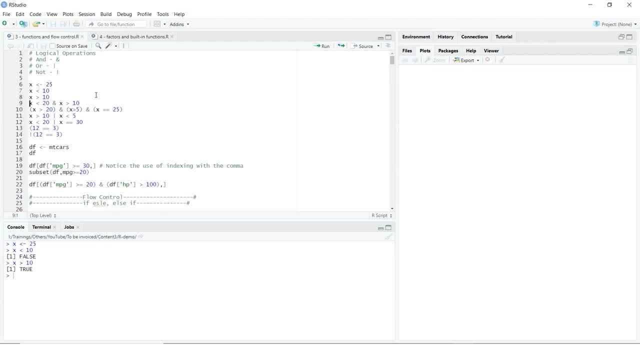 can use logical operations here. so i can say: and so i'm saying: is my x value less than 20 and is my x value greater than 10? now, both these conditions are not true, so in this case we can get the result as false. but if i say x is greater than 20, which is true, and i am saying x is greater, 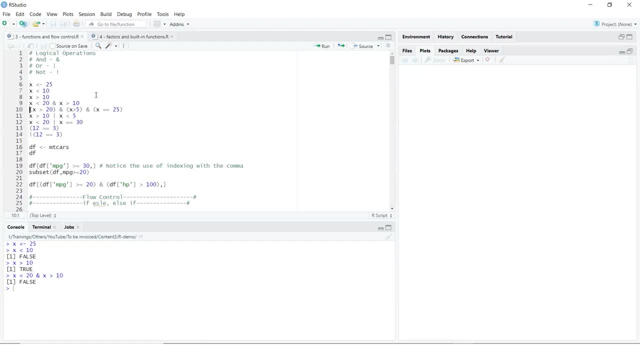 than 5. that's also true, and x is equal to 25. now, whenever we are talking about and we have to look at all the conditions have to be right. so let's look at this and we get the value as true. but if i say x is greater than 10 or x is later than 5, then one of the condition has to be: 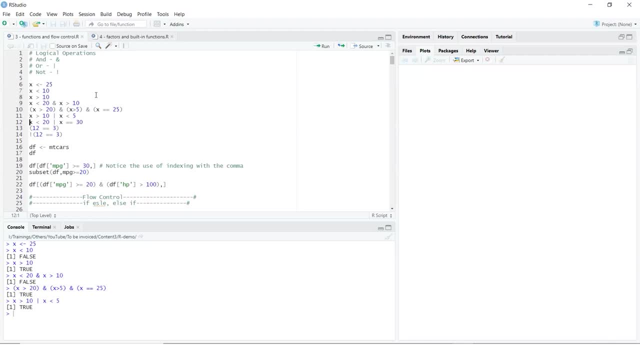 true, which is true in our case, so we get the result as true. we can take a different example. we can say: is x less than 20, which is not true, but is x equals to 30, and that's also not true. so in this case we get result as false. now we can straight away compare some numbers and we can say: 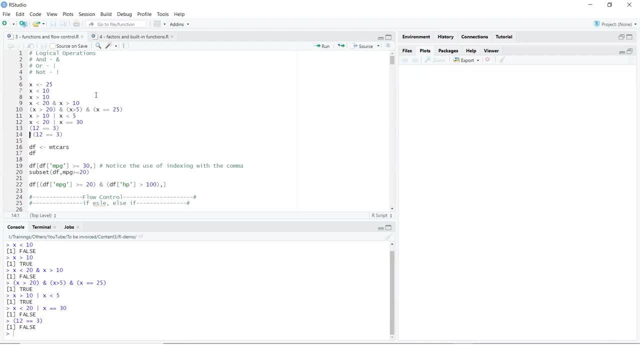 is 12 equals 3, and that's false. and if i say not, then that basically will give me the result as true. so these are some simple logical operations which help you when you're working with your data in r. now we can create a data frame by using an inbuilt data set: empty cars. and let's look at our data. 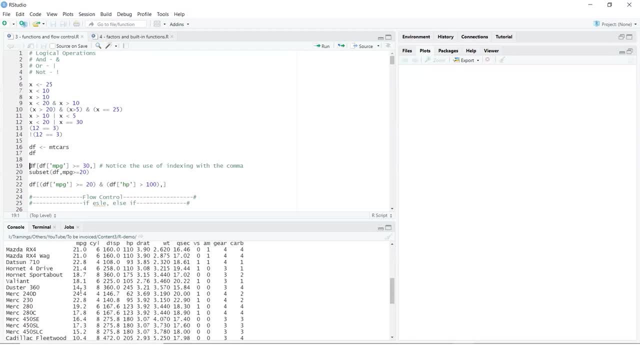 frame. so that shows us the values with all the different car models and the different column names. so car models are the row names and then you have other things like mileage and cylinder and so on, which are the specification for the data. now what i can do is i can filter out. 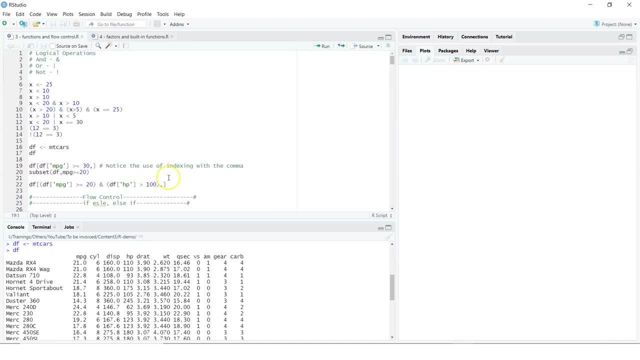 values here using indexing, so i can say data frame. now in that data frame i would want to compare the value of mileage which is greater than or equal to 30, and then i can end it with comma, so that gives me the value wherever the mileage is greater than 30. i can also do a subset on data. 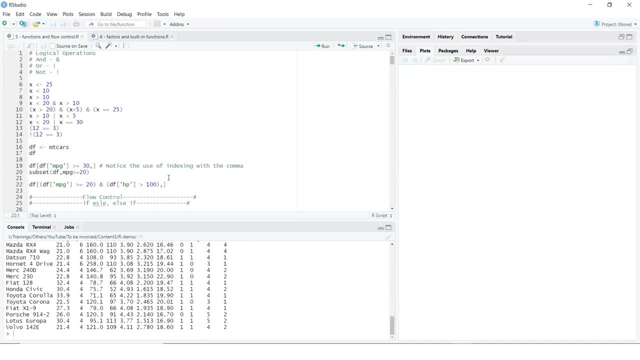 frame where i can select a particular value. so we can be doing this or we can be using square brackets. we can also do a dollar and compare the values. now we will use our logical operations knowledge here. so we will work on data frame where i am interested in the mileage which 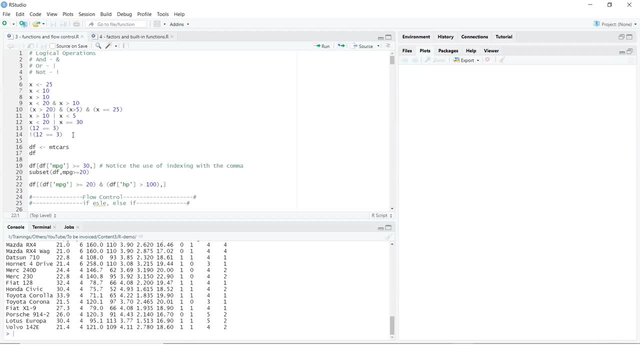 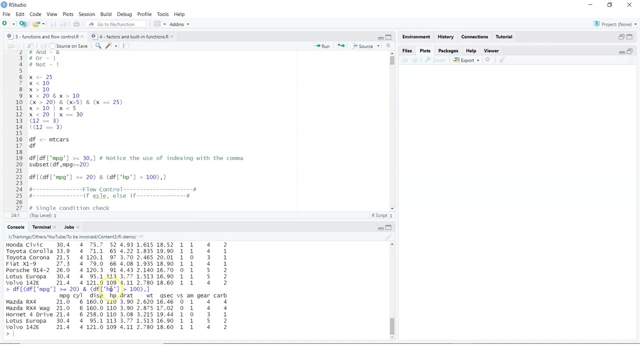 is greater than 20 and i am looking at the column- hp horsepower- and that should be greater than 100. remember, when we are doing a and both the conditions have to be met as true, and that shows me the result where you are looking at the mileage. 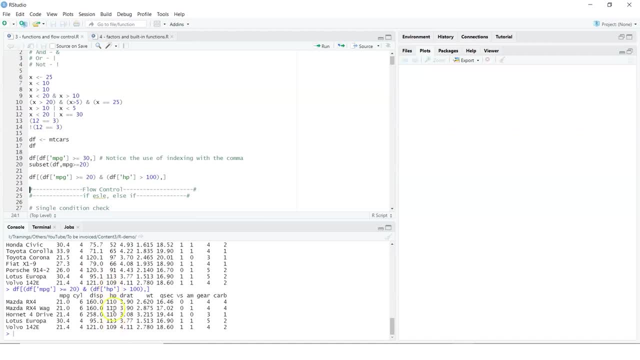 and you're looking at the horsepower column. both of these are met and that's why we get the result. so these are some simple examples of using your logical operations, either when you're working on a data frame, so same thing can be done on a matrix. same thing can be done on a list or a vector or individual values. 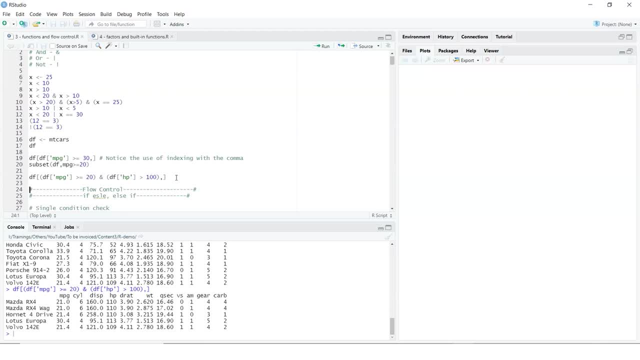 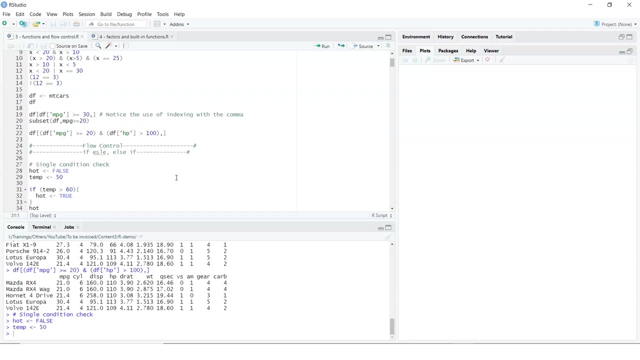 now let's also learn about flow control. that is how, if else, or else if is handled in R, so you can do a single condition check. so, for example, I assign a value to hot which is false and I am saying: temperature is 50. now what I 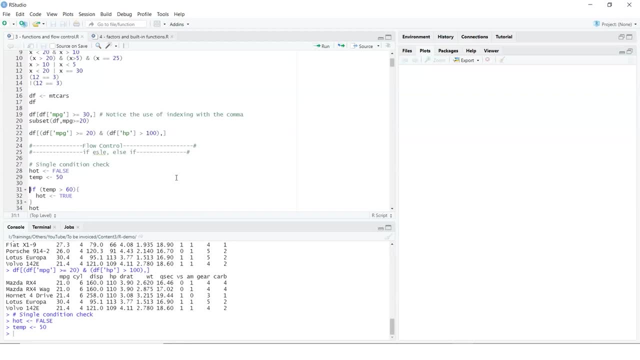 would want to check is if the temperature value is greater than 60, which in our case will not be true, which will not be true because temperature has been assigned 50. so is it greater than 60? no, so if I do this, if condition and I 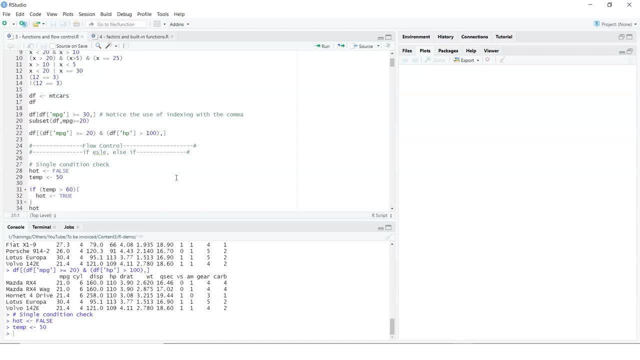 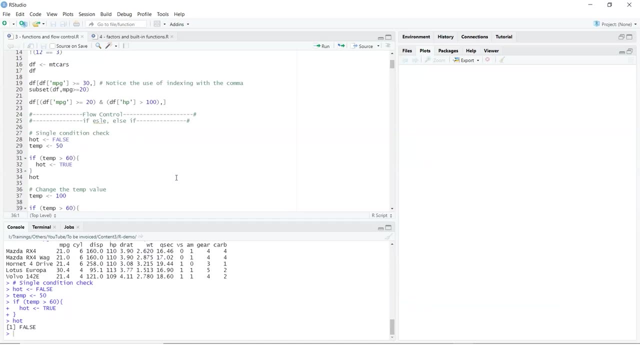 am saying: if the condition is true, then I would want to assign the value of hot to true. and now, if you look at the value of hot, it is still false. why? because the condition which we passed for our if is not true, it has not been met, so whatever. 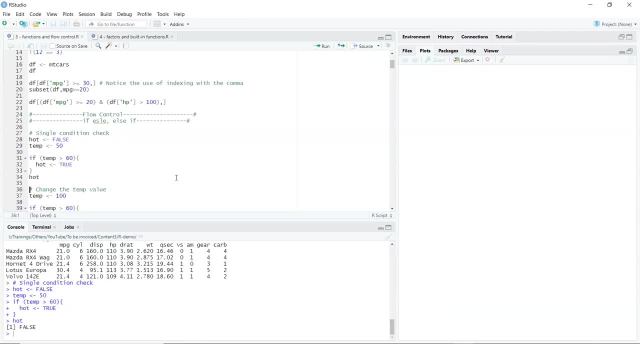 was passed within the statement has not been done. now let's change the value of temperature as 100, and now, if we do the same thing, we say: is my temperature greater than 60, which is right, so then whatever has passed in the bracket will be applied. so 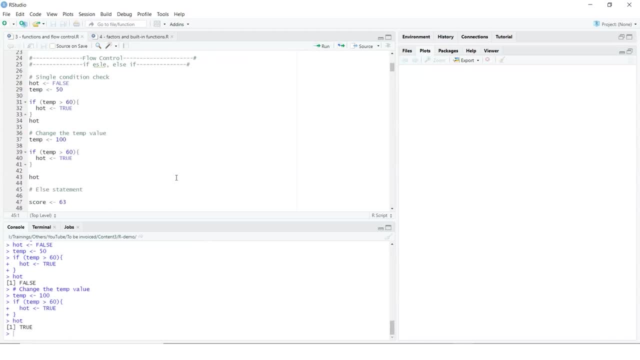 hot will be assigned new value. and now, if you see the hot values and set to true- so this is a simple single condition- check what you're doing. now, certain times there can be multiple conditions to check and that's where we use else. so in this case we go for assigning a value to score which is 63. 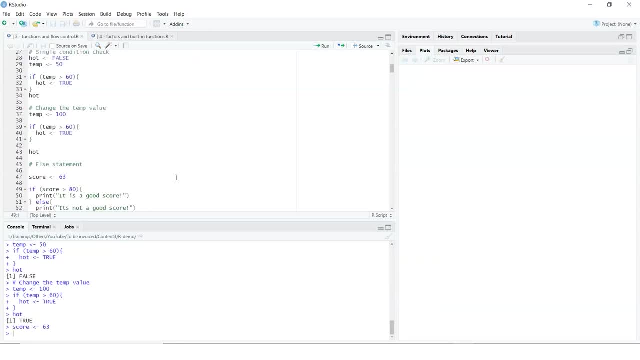 so let's do that. and now let's say: is my score value greater than 80, which is not true? so whatever is passed in here which is print it's a good score, will not be done, but it will jump to else. and then whatever we have passed in else will be done, so it will say it's not a good. 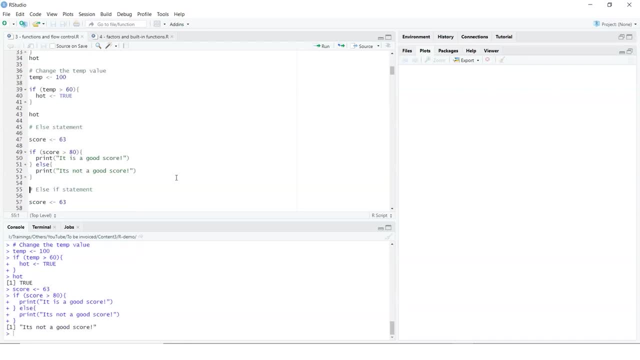 score. so let's do this if and it says it's not a good score. so this is a simple way of using if else, where you are checking two conditions, or you are checking the condition, but what if the condition is not met? then your control is passed to your next statement. now I 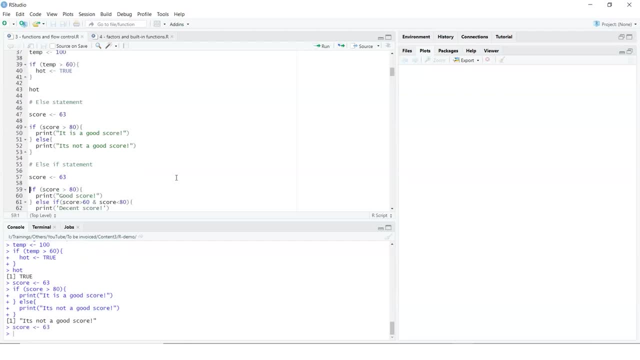 can also do a else. if so, I can say score is 63 and I can say: is my score greater than 80? that's my first condition. so it would print good score. but might be. I would want to check something else. so I'll say else if and I'll say is my. 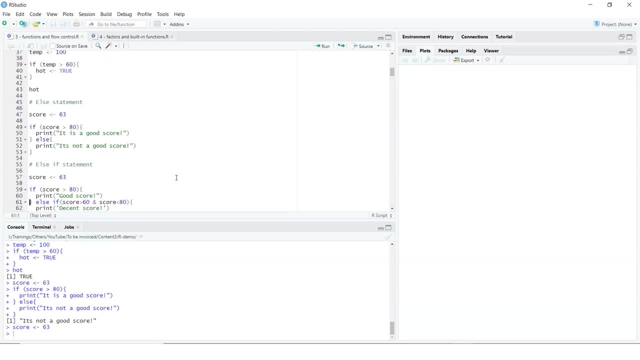 score greater than 60, yeah, and is it less than 80? remember the and which has to evaluate. and true for both the conditions. I'll say: print decent score. I can still keep on giving conditions here in, else, if score less than 60 and score is greater than 33, that would not meet, so that will be ignored. and then 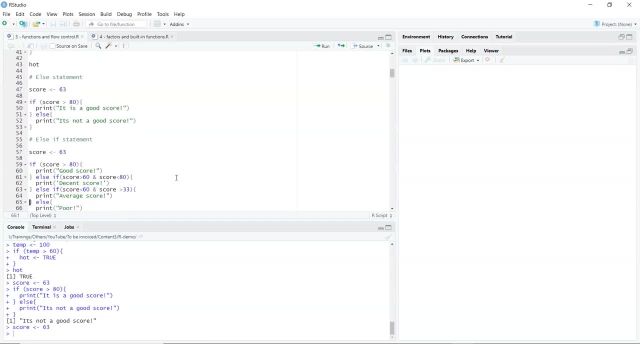 you have else which says print poor. so first it checks or evaluates for the condition which you have passed for if. if that doesn't work, then it goes to else, if and if anything in else if is met, then it's going to take that into consideration and it will not go for else if, if and else if conditions are. 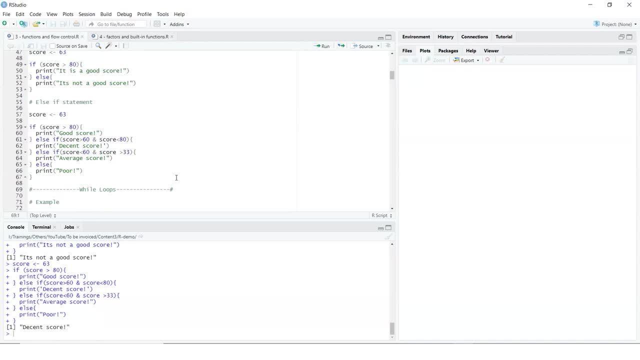 not met, then it goes to else and we see decent score already printed here. now that's a simple example of if else and if else. if, wherein we are evaluating a condition, but probably we have multiple other things to check. now how do you work with while loops in R? that's very simple. so what we can do is we can. 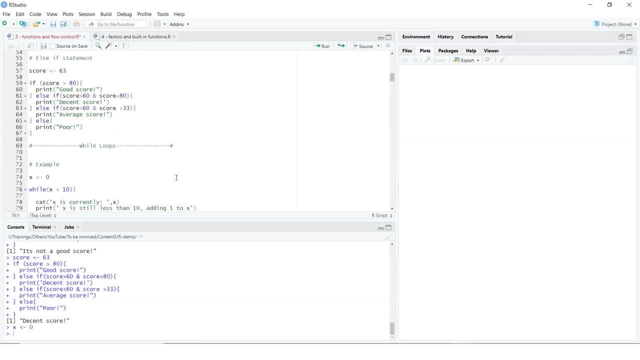 assign a value to X. and now I will say, while my X is less than 10, so I'm going to create a loop. so I have said my X has been assigned a value of 0 and that's fine. so this is going to be less than 10. but if we are going to just do this, then 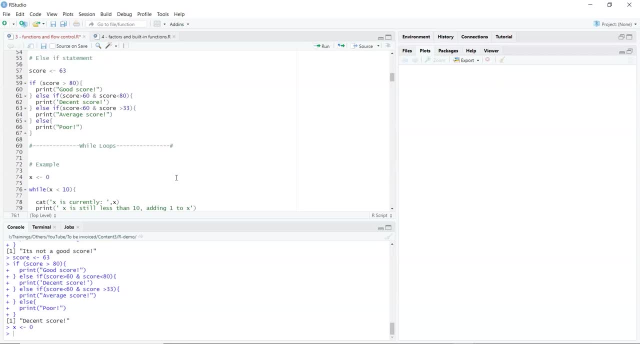 it will keep running and it will get into an infinite loop. so we'll see how we do that. so we'll say y, while X is less than 10. I would want to basically have the value of X. I would want to print: X is still less than 10, adding 1 to X, and what we are doing is: 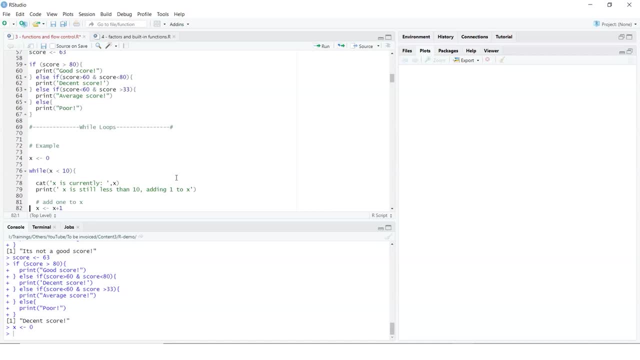 we are incrementing the value of X. now. if you do not do this step, then it will get into an infinite loop, because X will be always less than 10. so we are incrementing the value of X by 1 and then we are giving a condition. so if at 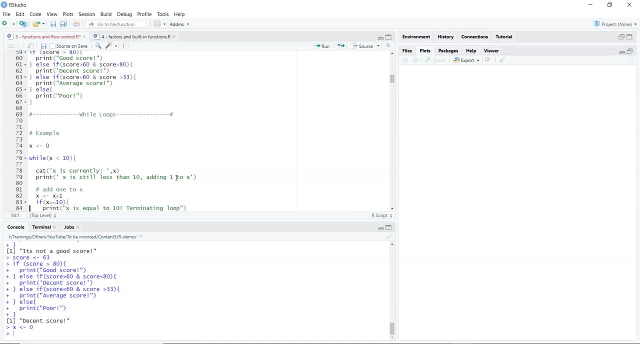 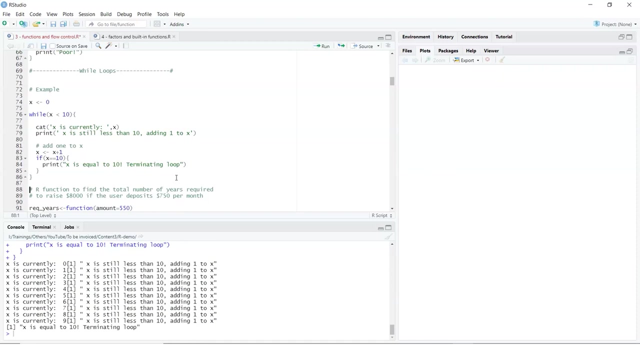 any point of time. X is equals to 10. I would want to say X is equal to 10, terminating the loop, and then basically my while loop ends. so we can do this. so let's say X is 0 and then do this while loop, and now you see, it is at every step. it is basically printing. 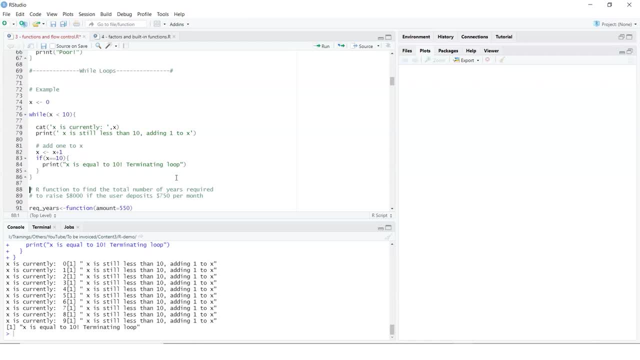 out the value of X, it is still less than 10 adding 1 to X and it also gives you the value of X. so when we do a, X is currently and I print out the value of X, so it shows me 0. next time you increment it, it becomes 1 and 2 and so on. so this is where you 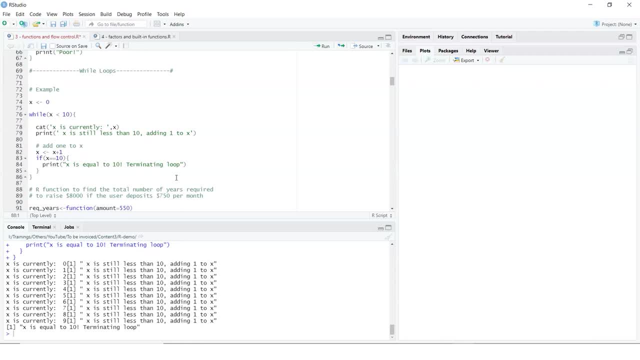 are using a while loop, where you are looping where based on a particular condition and then you basically have, once the condition is met, you are able to complete the loop. now let's look at a. let me take this one here. we look into functions in a later stage, so let me. 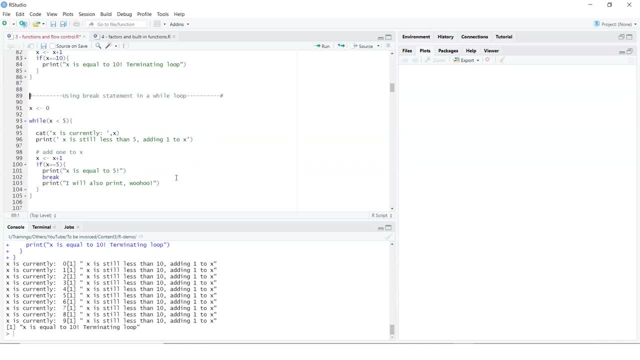 take this function and let's get rid of this one. I would also want to talk on break statements and while loop, and once we are done with the flow control on while loops, then we can look at the functions aspect. either we can look at how we control our functions or how we create built-in functions. so let's look at this. 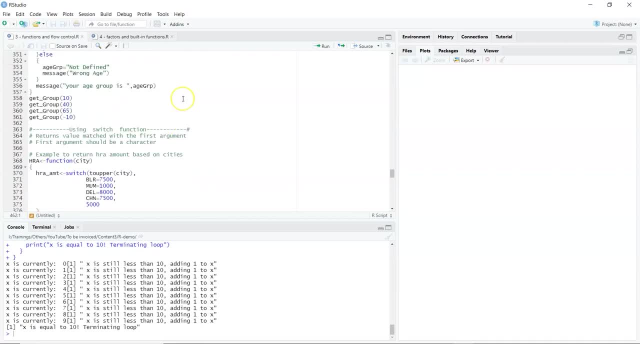 one and let's continue with our while loop. so we just saw a simple while loop here, and what we also want to see is: when you are working with your while loop, how do you break if a particular condition is met? so we saw a simple example of while. 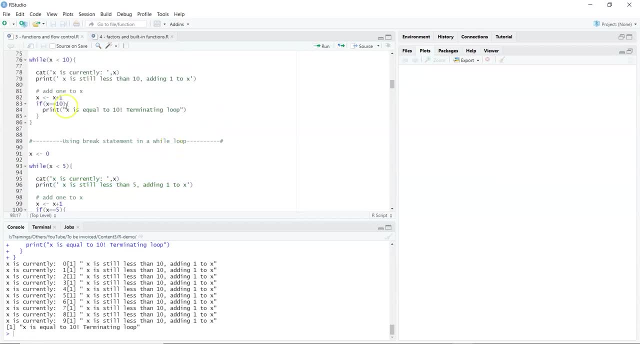 loop- and that's fine- wherein we were printing out something, we were auto incrementing the value of X. we were also checking at one point of time with the value of X and we were able to get the value of X within our while loop. if the value of X was met, we would say we are terminating the loop and it comes out of. 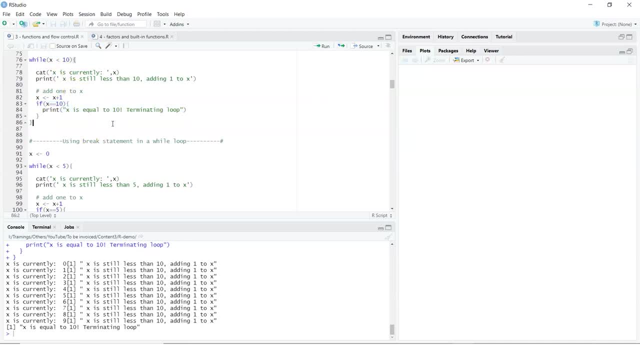 that now. if that does not happen, then we continue doing it. how about a break statement? so break statement is when you would want to end the while loop if a particular condition is met. so for example, here I assign a value to X which is zero. now I want to evaluate this. 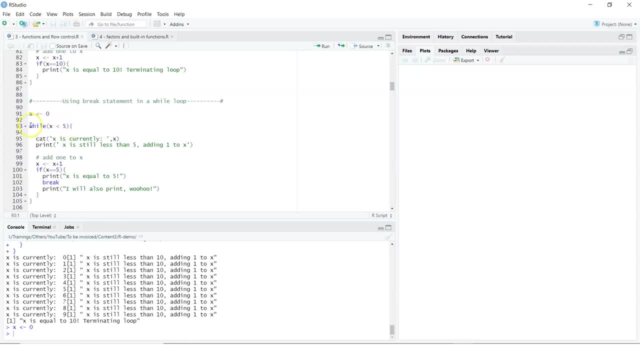 X is wheat, it will be permanent value in my value is then X will automatically be automatically work in itsayı Kiran positive. I mean when I print a value of x, I see that x is, for example, any of x. I will copy it out of the value of x. 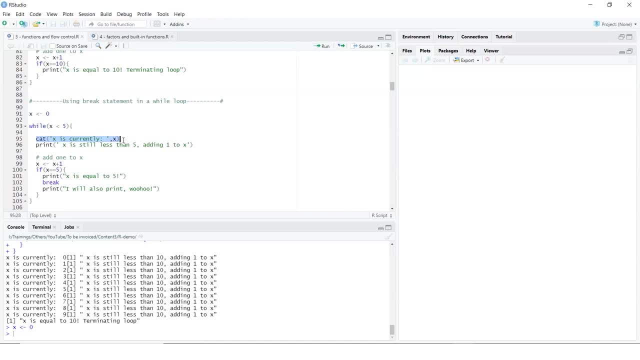 and I will be auto incrementing the value of x. so I will create my loop and given a condition that x is less than 5. now what I want to do is I want to use the cat function, which will print the value. so I'm saying x is currently sen. 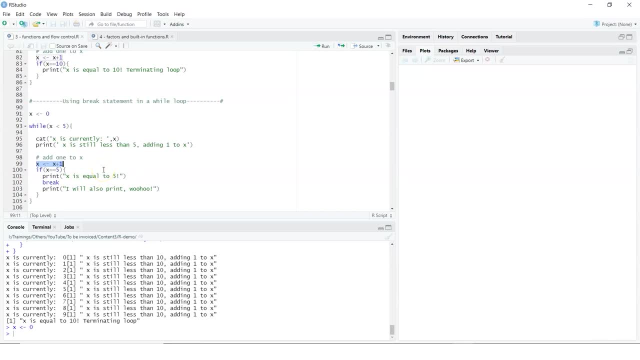 I'm then increment it by 1, and here I am saying if x reaches 5.. So while we keep incrementing the values within the file loop, we will see if x's value is 5, we will print it is equal to 5 and we 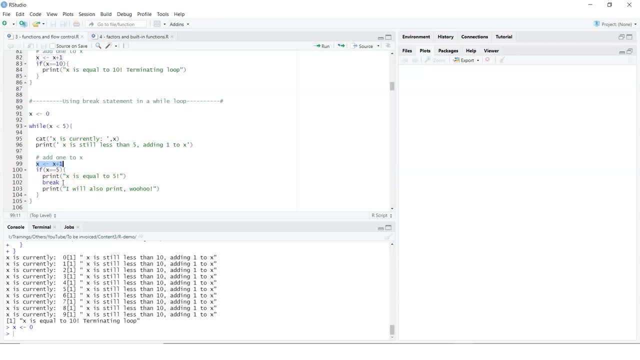 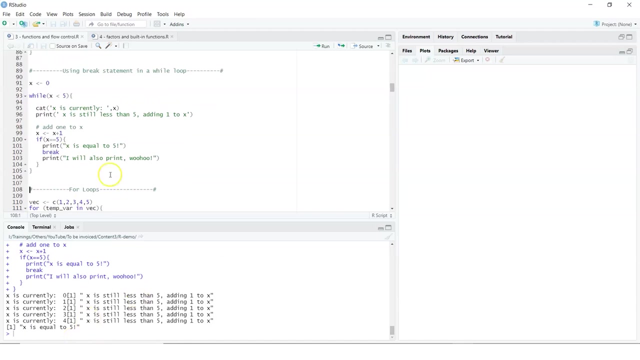 can just do a break. Now, if you do not use a break, you can still end the while loop, but break is basically to end this loop here based on condition which is met, and we can do this and then run this while loop. So you see, here x was met as 5 and we just broke out of the loop. So that's your simple. 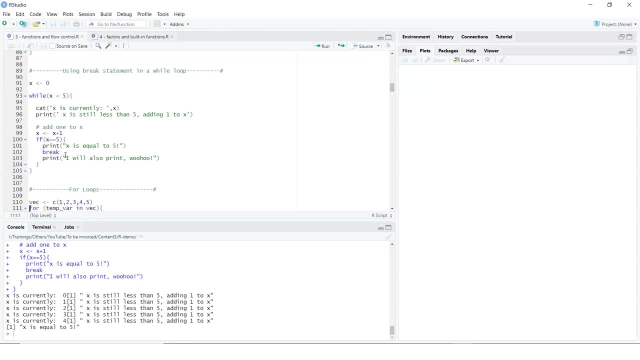 while loops, what we are seeing. Similarly, we can work on for loops, So for loops can also be useful. so your conditionals, what we saw as if else, or else if your while loop is, while a condition is not yet met, you keep looping and keep doing some actions. Now what you can do is you can. 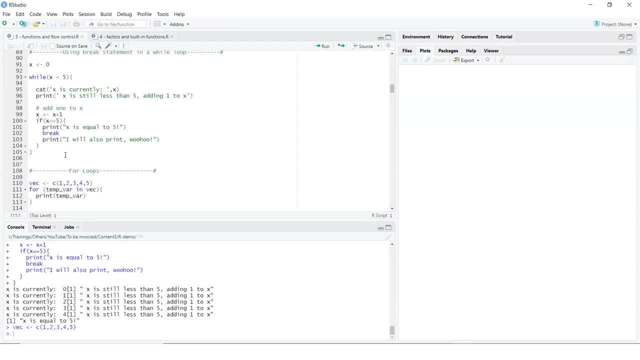 also work on for loops. So here I am creating a vector and then I am going to loop, that is, I am going to iterate through every element. So I'll say for, and when you are using for loops, you'll say for, and then you can give in anything. you can give in any value. I can say i. I can say x. 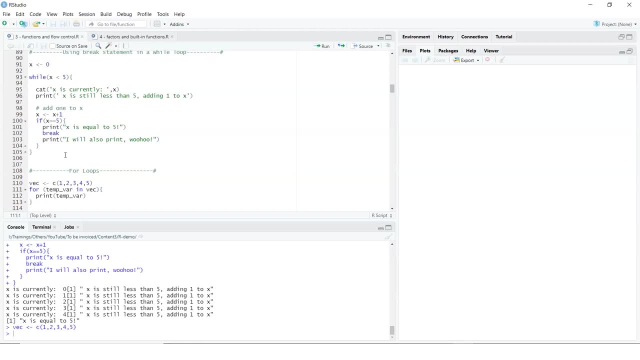 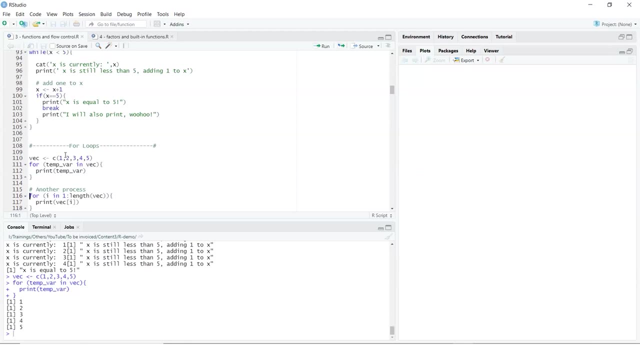 So I'm just giving temporary Variable in vector and then I'm printing it out. So this basically prints all the values one by one. So there is one more way to do it. You can say for and you can say I in and I would want to. 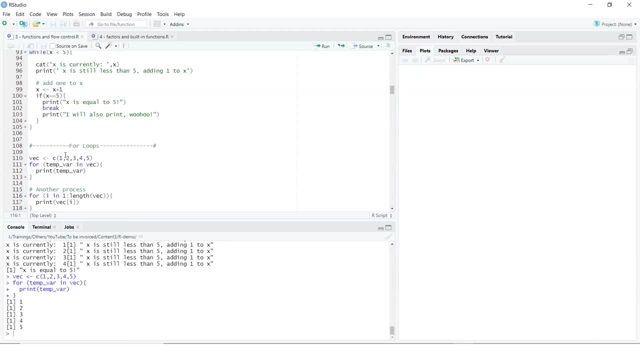 take length of the vector, So one to the length of vector, that is, till the last element is reached. I would want to print the vector elements using the value of i. So what is i here? It's the index position, and I can do it in this way. So if you are looping over a list, So I'm creating a. 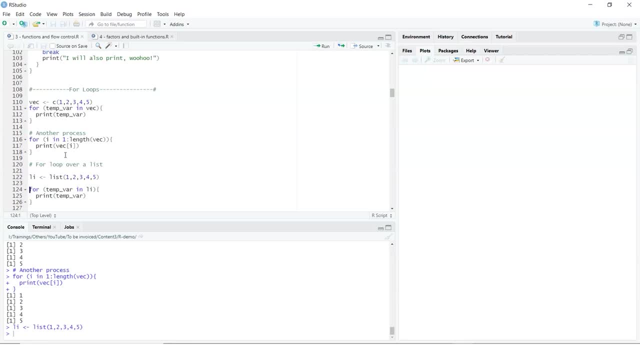 list and it's very simple. So you can just do a for loop where you can say for i in list, I want to print the i and that gives me the list elements. or you say for i in and you give from starting position, that is one till the length of list, and you would want to print every element. So here we. 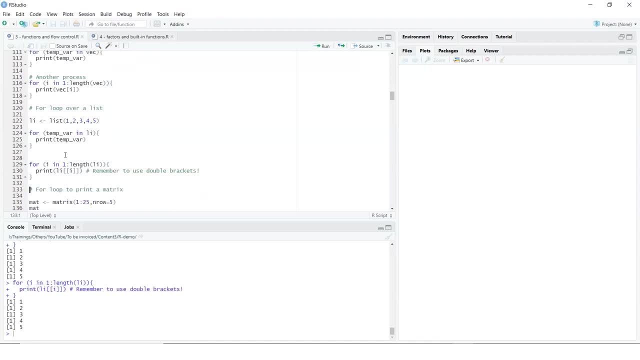 can also use double brackets. So if you would want to loop through a matrix, So sometimes that might be required. So let's create a matrix which has 1 to 25 values around by row, and you look at your matrix and now what you want to do is you want to iterate through a matrix. So you want to do. 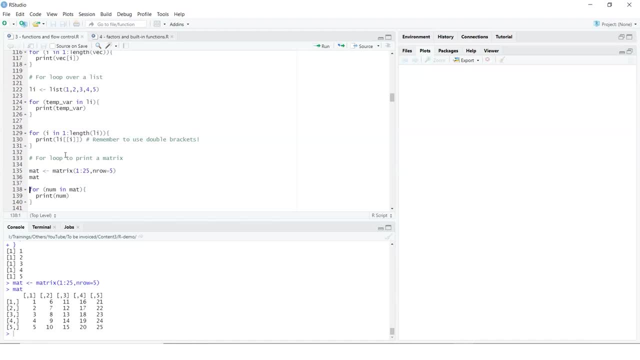 a looping. So I'll say for: i in matrix I would want to print out the values, and that prints out all the values in matrix. Now what if I want to print the square and square roots of numbers between 1 to 25.. So I can say for: 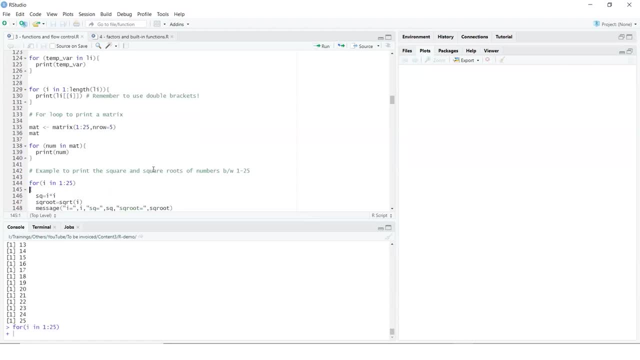 i, wherein the value starts with 1, ends with 25, and then within my for loop, I can basically give this condition where I'm saying: get me the square root that is i into i, or get me a square root of i and just print it out. So I'm saying: message i. 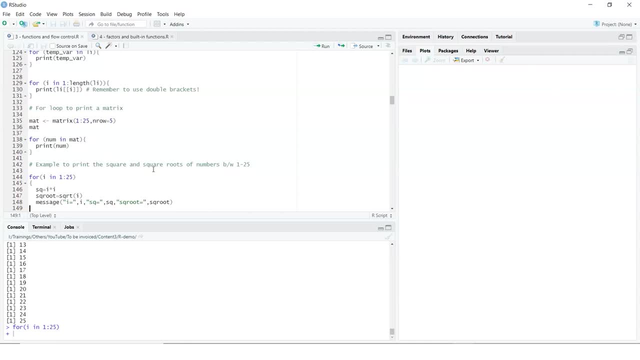 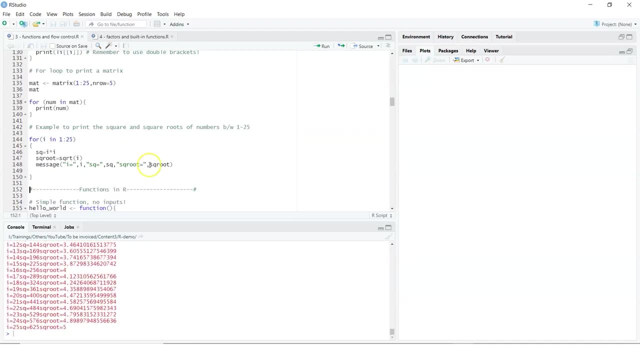 is this. one square root is this and my square is this and square root is this. So if I look at this values here now, I am looking at all the values from 1 is to 25.. I'm looking at the square of the values and I'm looking at the square root. So what we did was we did a for we passed in the elements.